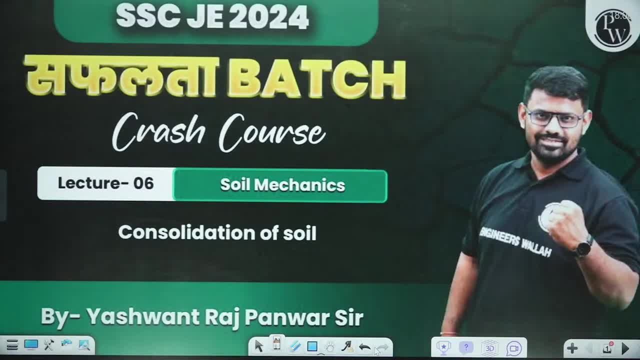 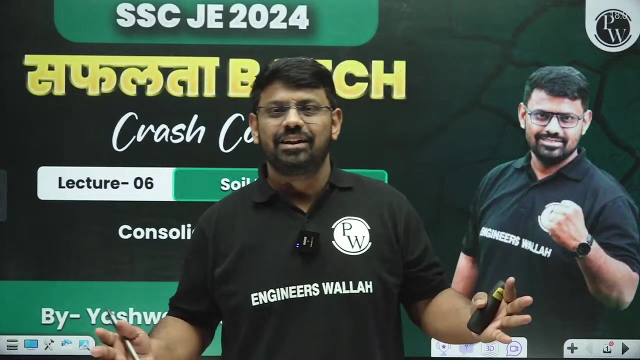 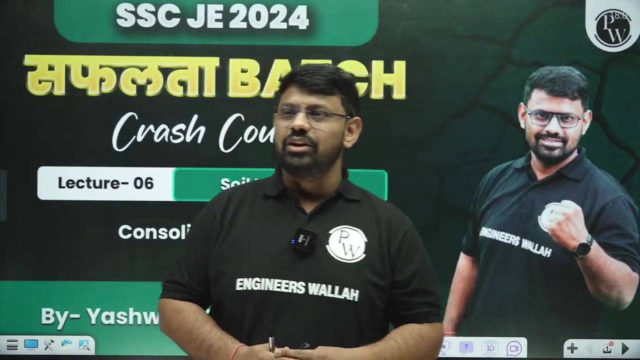 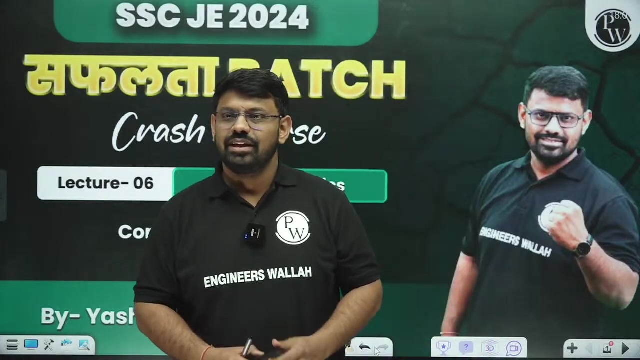 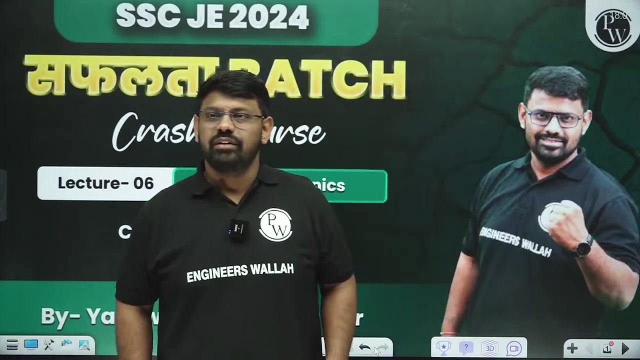 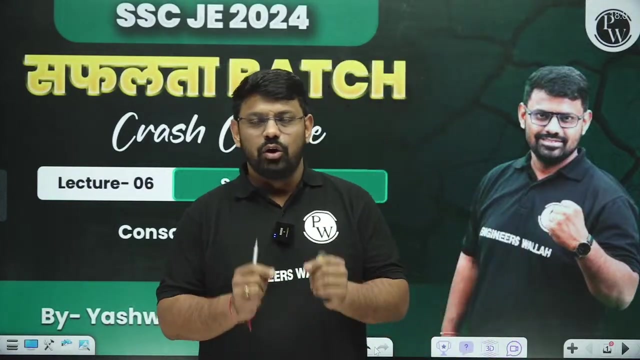 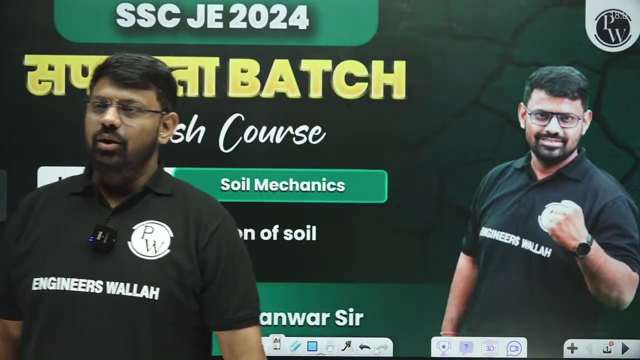 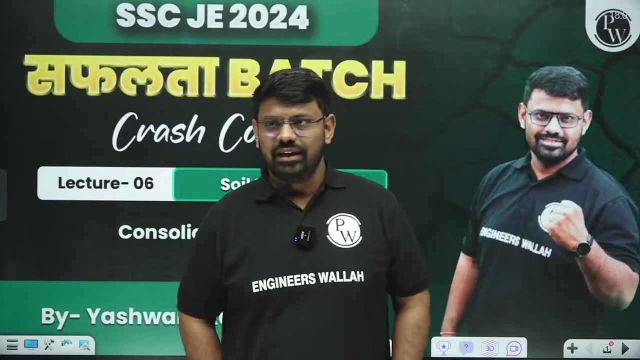 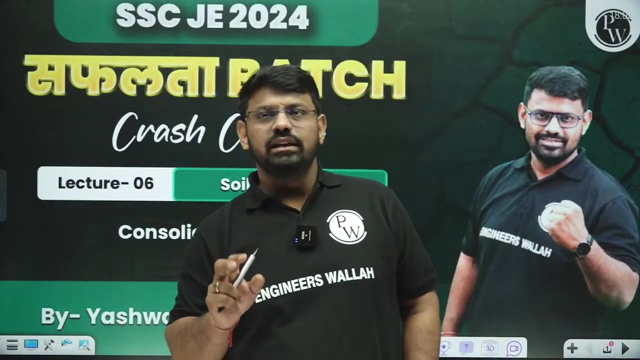 Thank you, Thank you, Hello everyone. A very, very good evening to all of you. A very good evening to all of you. A very, very good evening to all of you, Hello everyone, A very, very good evening to all of you. 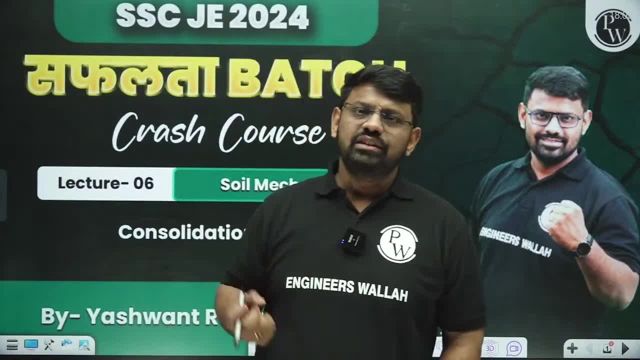 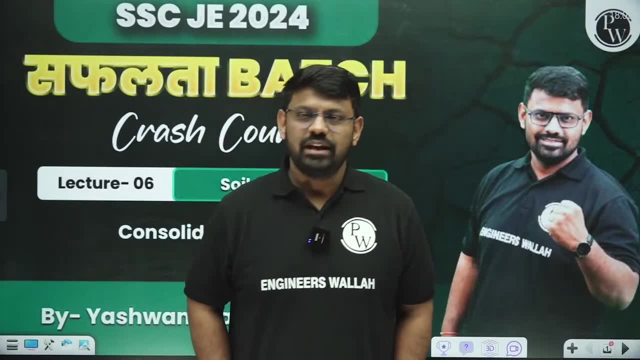 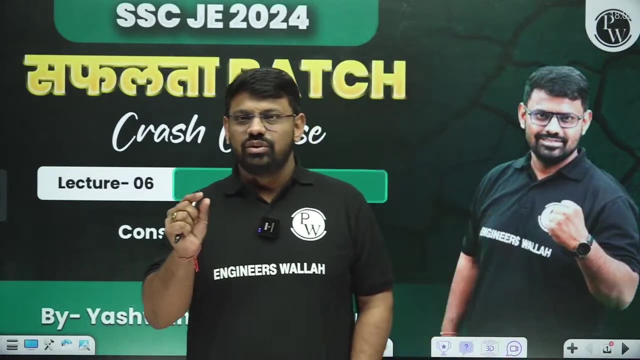 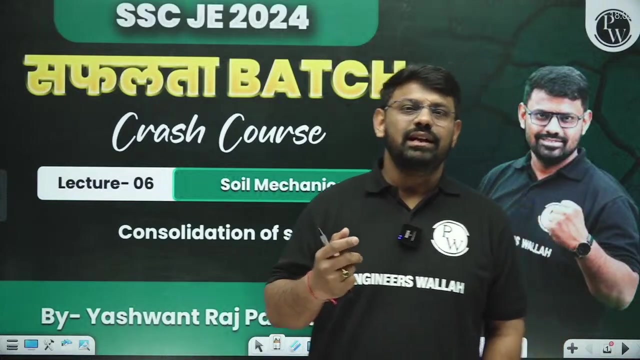 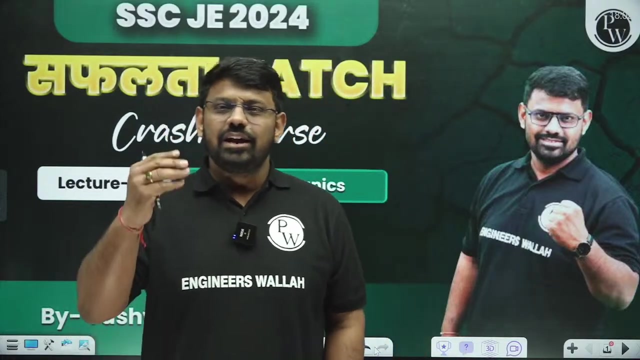 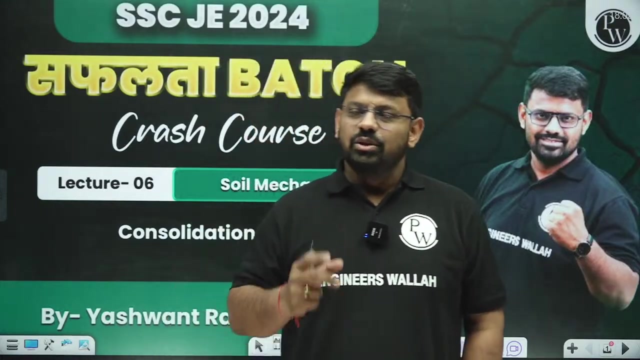 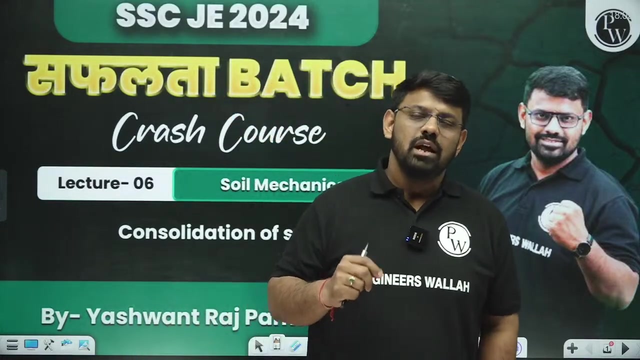 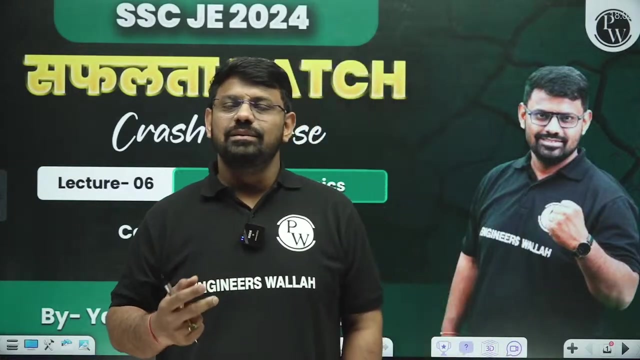 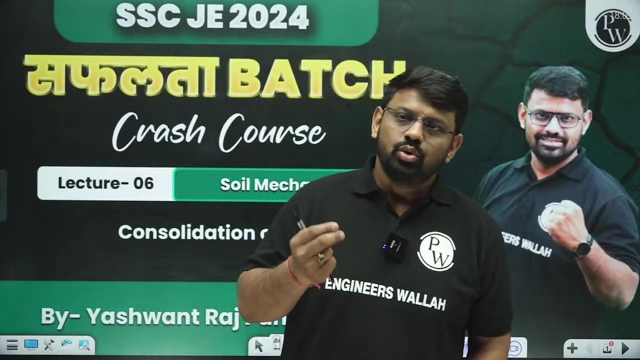 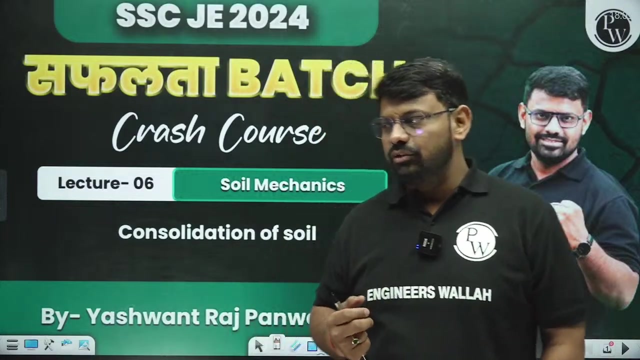 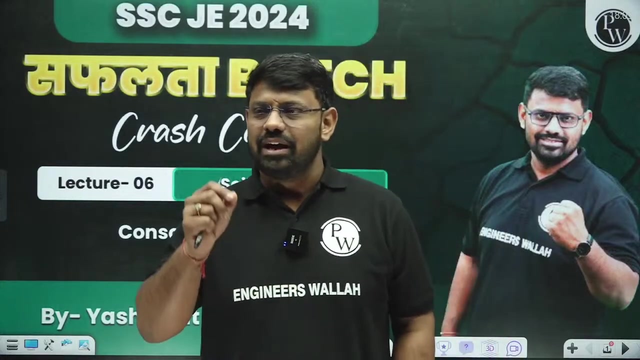 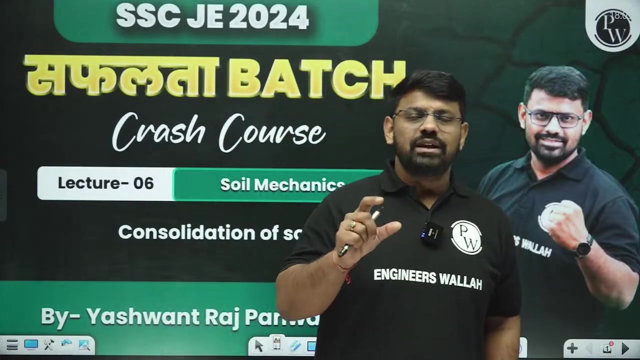 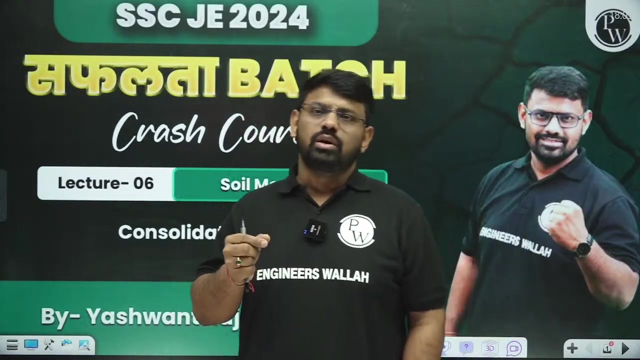 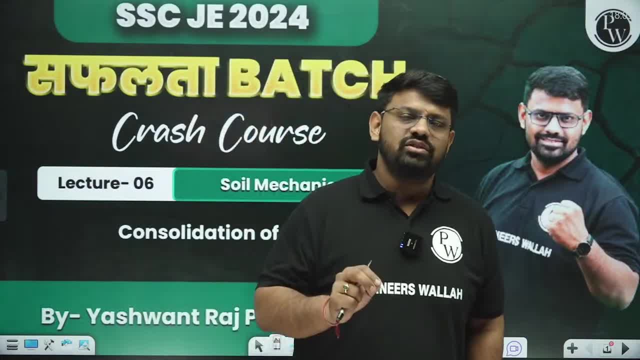 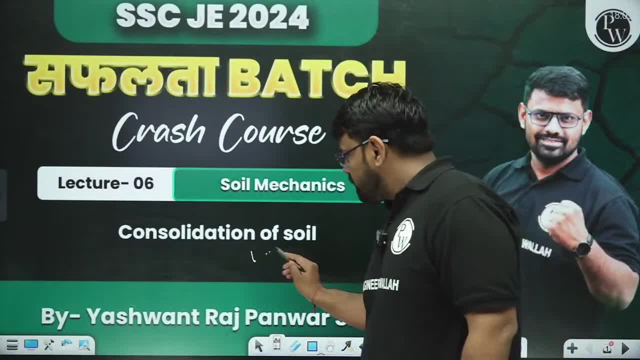 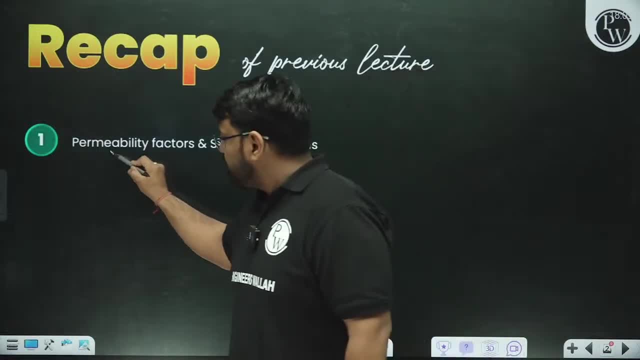 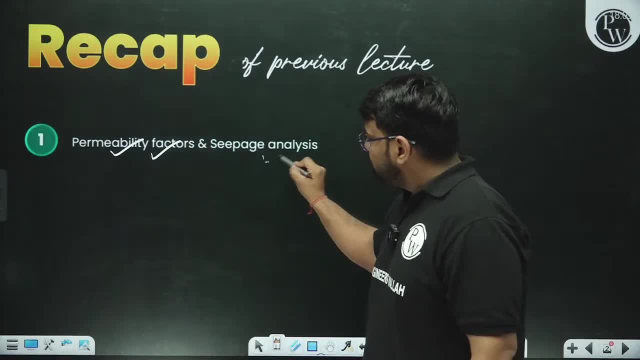 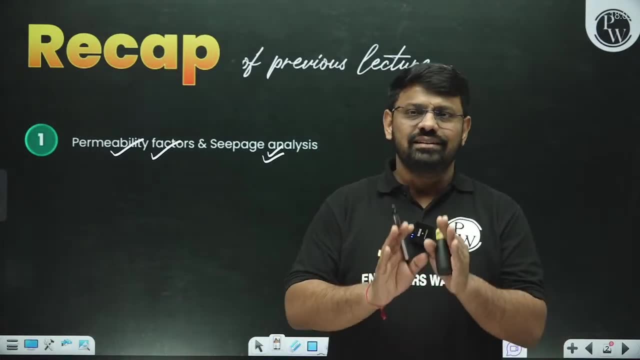 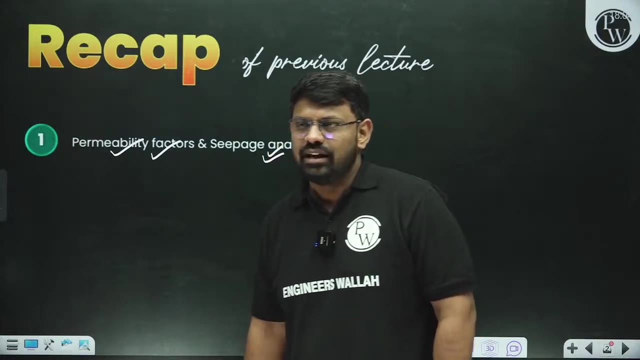 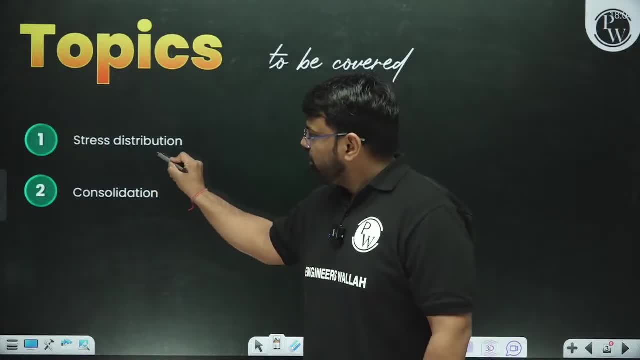 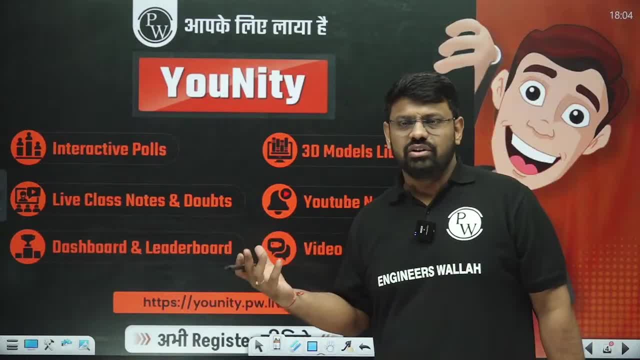 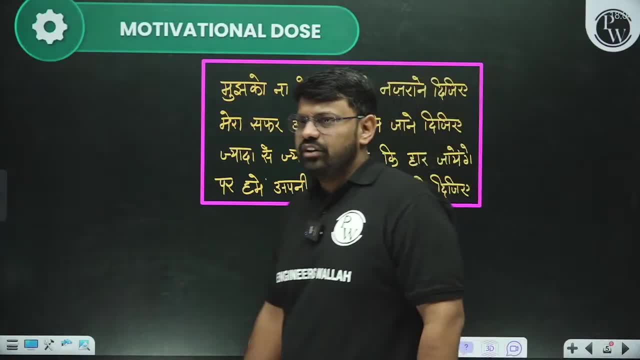 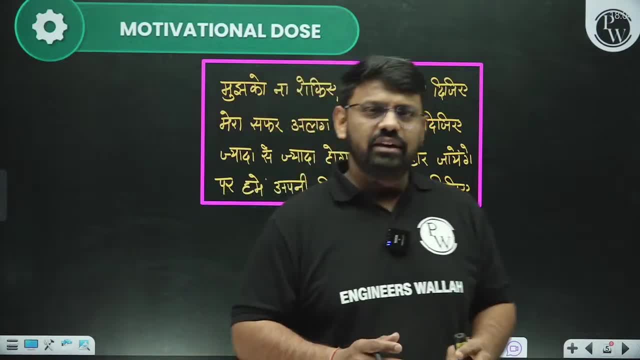 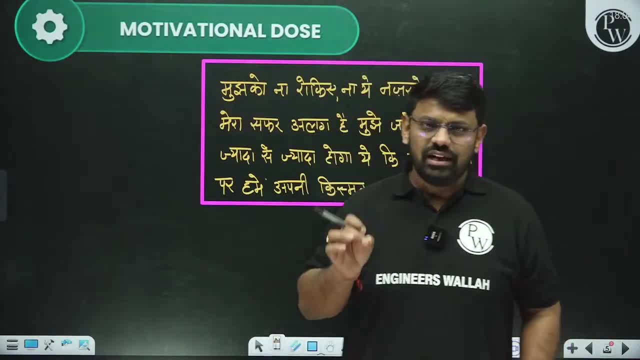 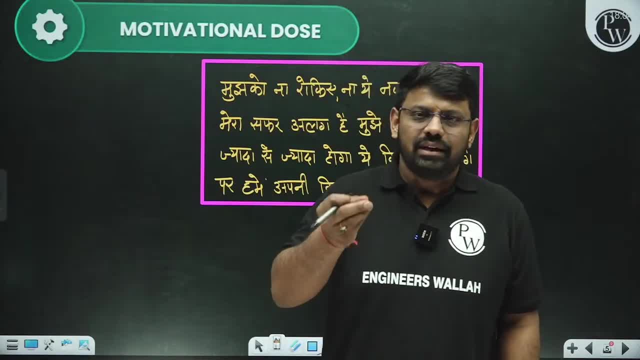 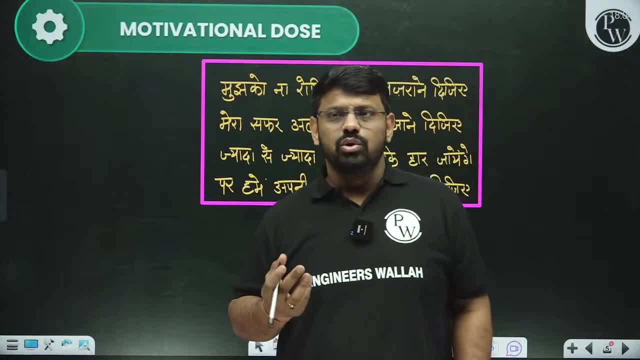 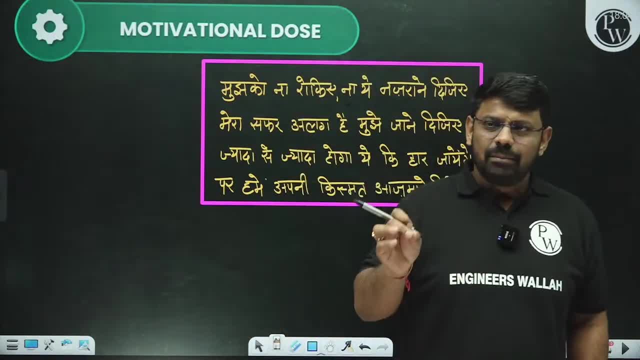 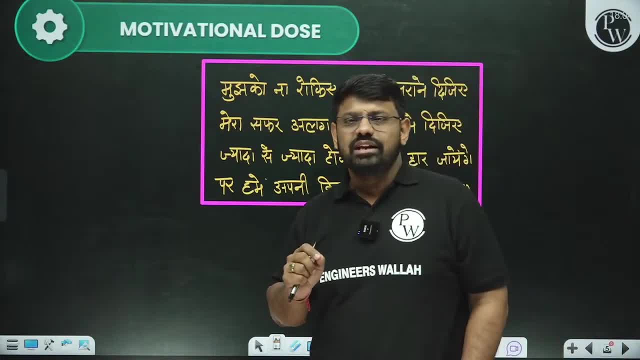 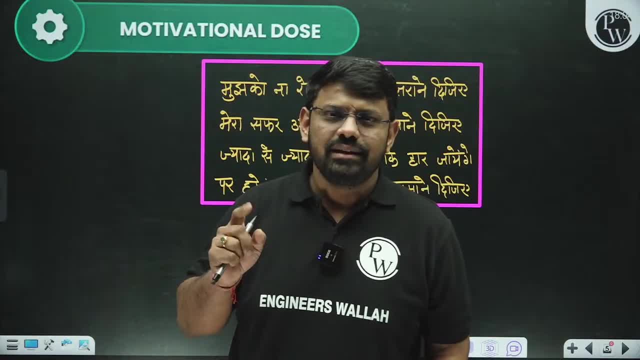 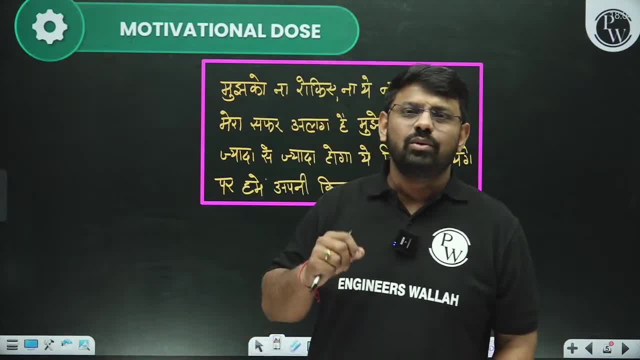 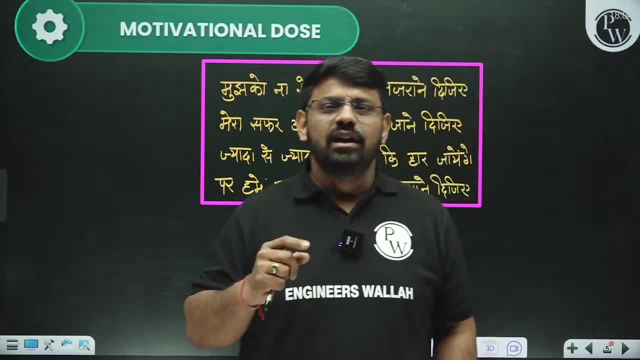 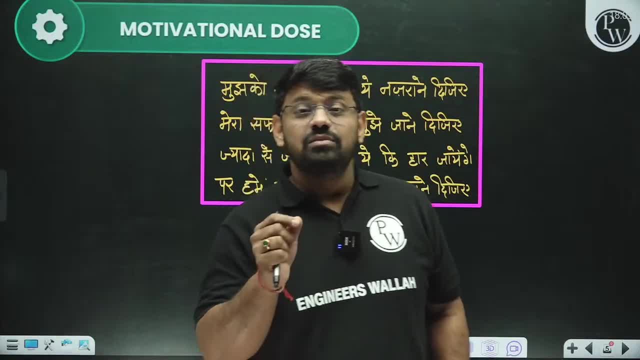 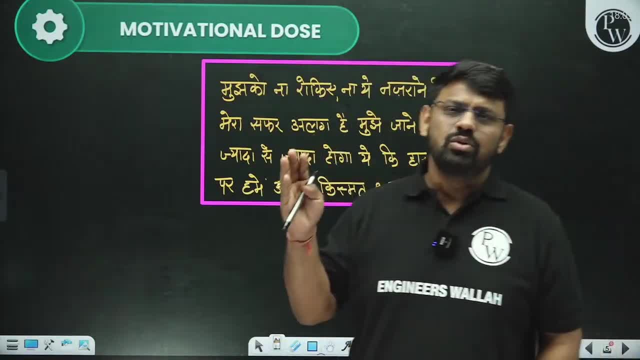 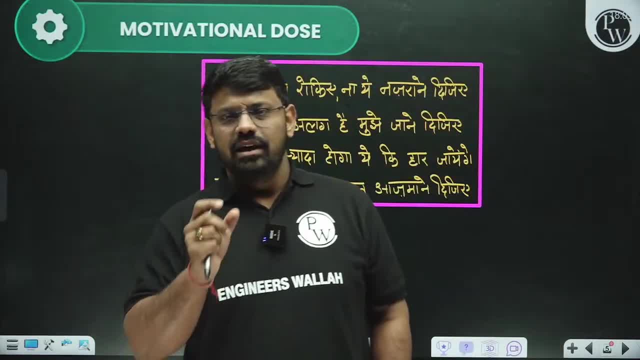 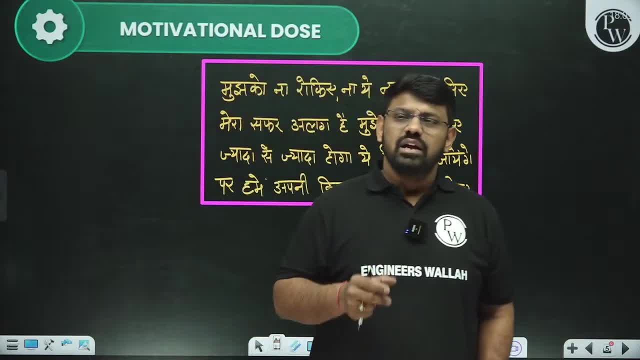 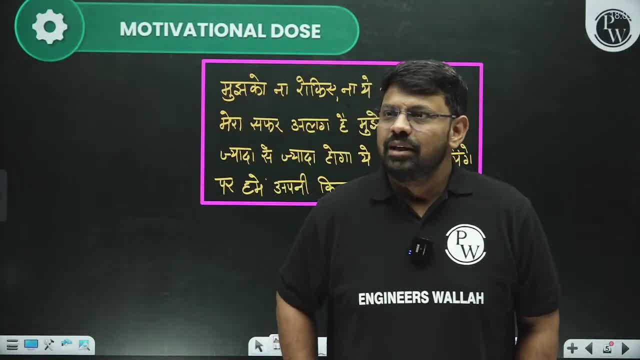 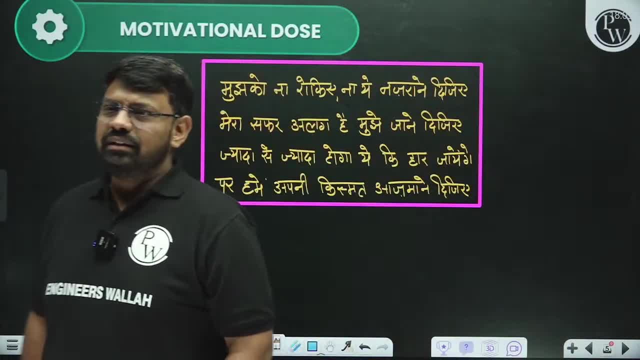 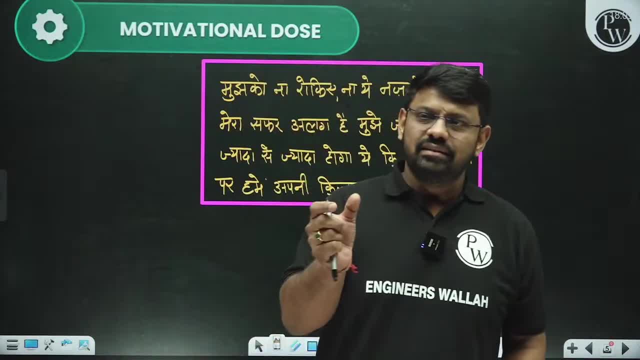 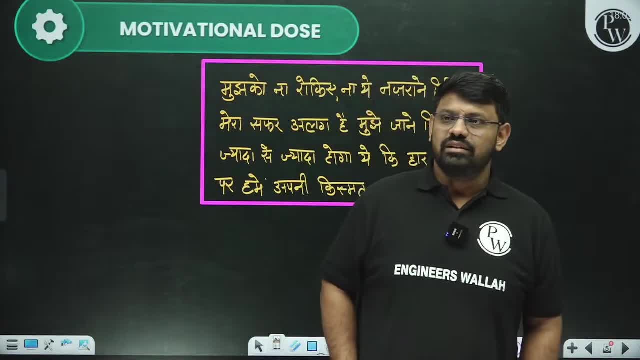 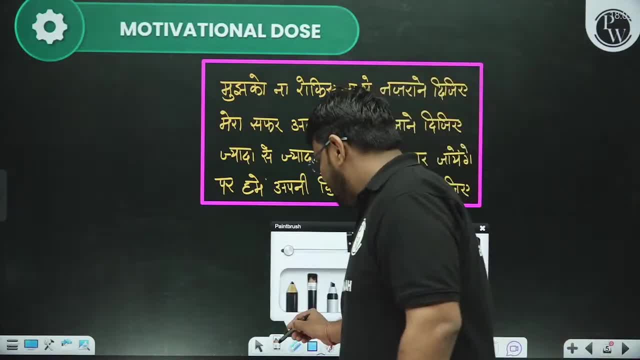 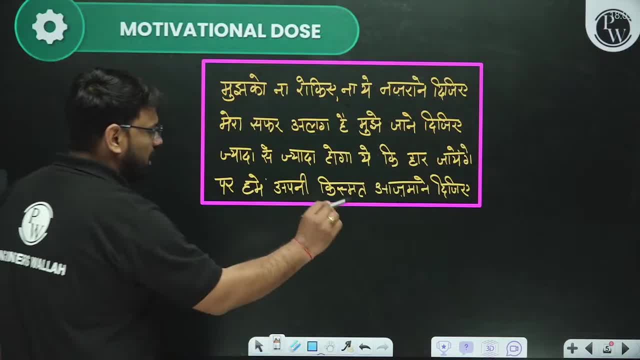 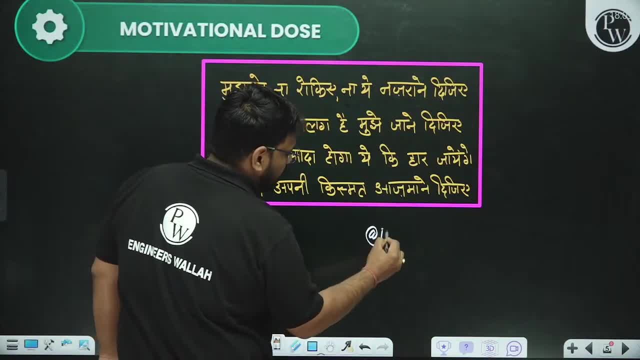 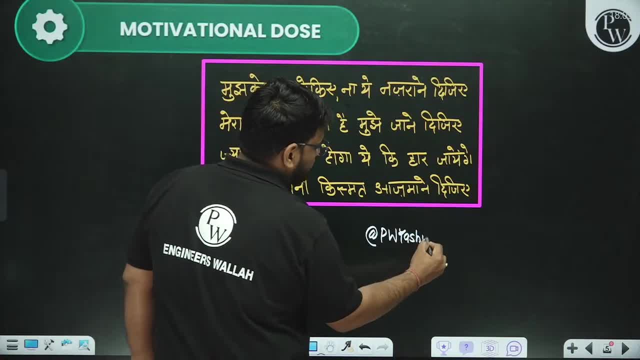 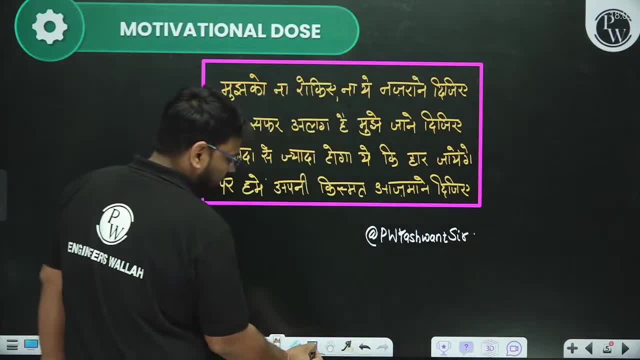 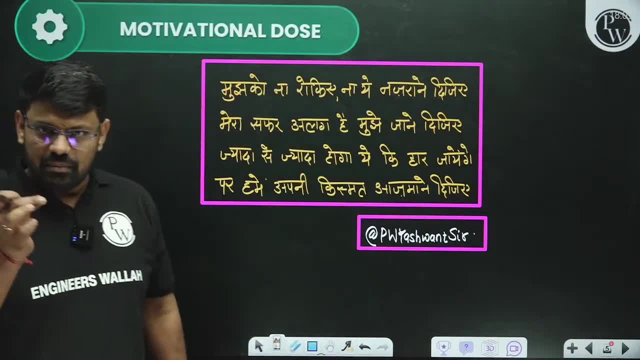 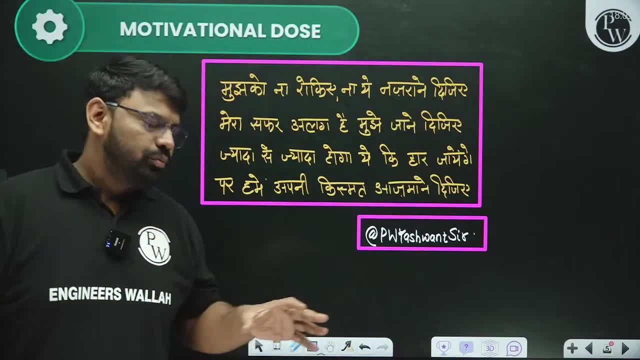 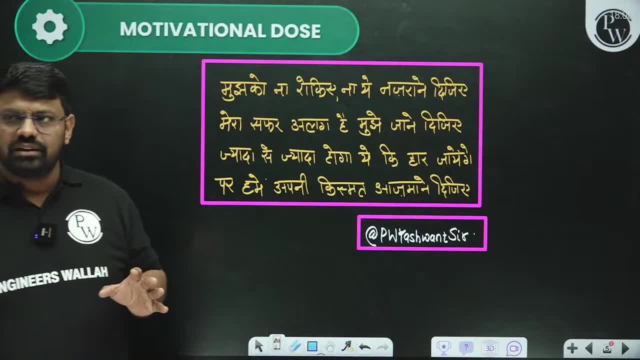 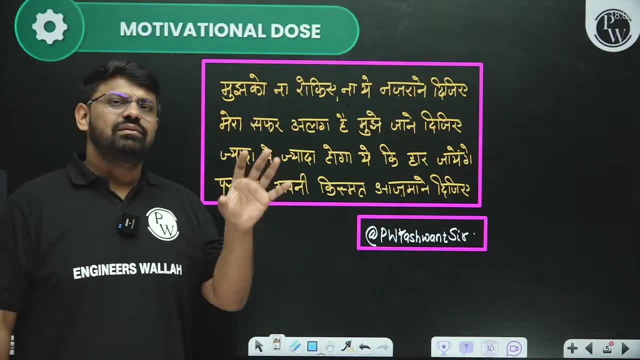 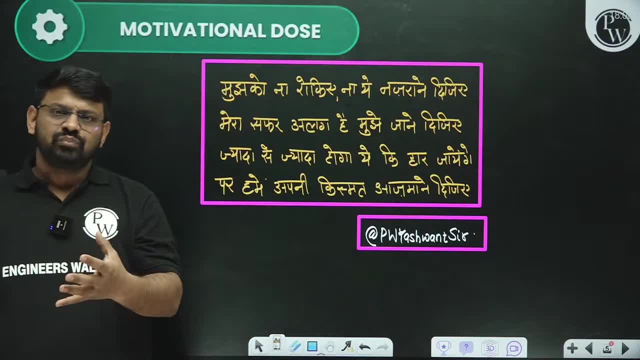 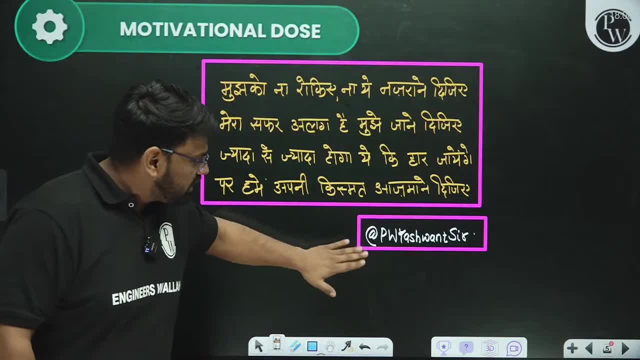 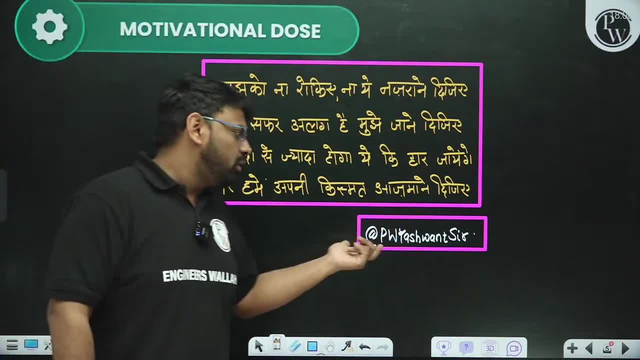 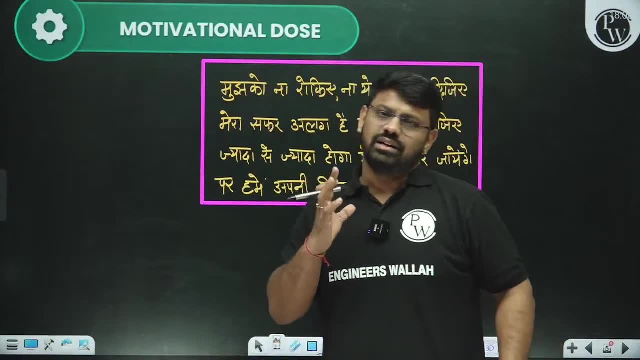 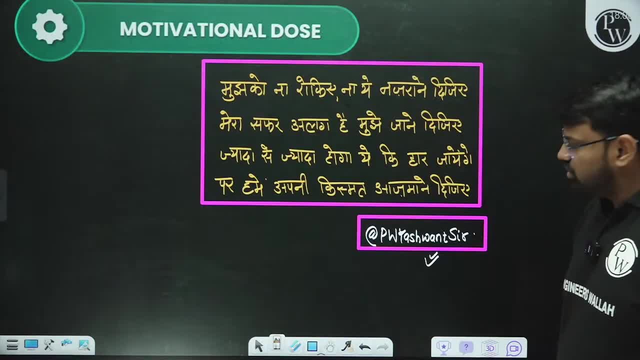 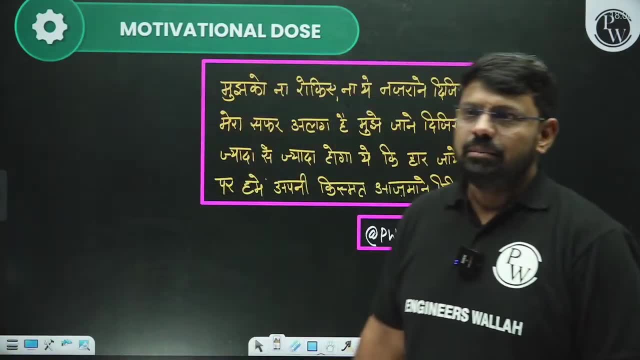 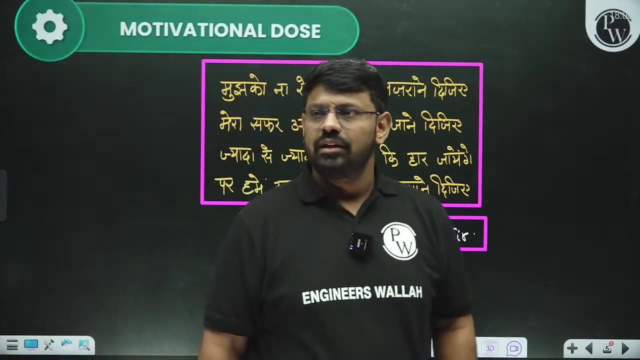 So you can come here at the rate PW Yashwant says you can join on the official telegram channel and here all your doubts, with reference, will be clear. Very good, Son, I have replied to everyone. Yes, let's start today's class. stress distribution in soil. 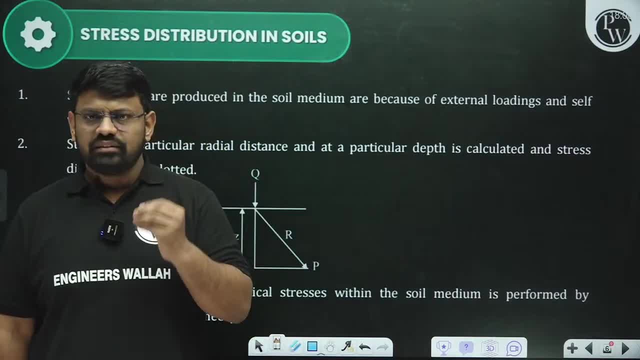 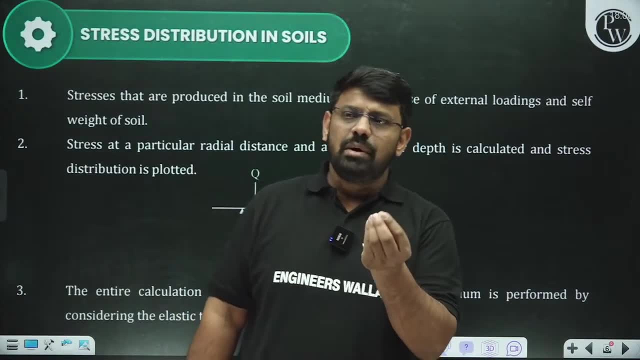 I have already shared the notes of this topic with you so that you can read a little about it, Because this particular topic, this particular chapter, does not have a lot of heavy weightage. There are only a few amounts of formulas in it. We have to keep looking at some small formulas here. 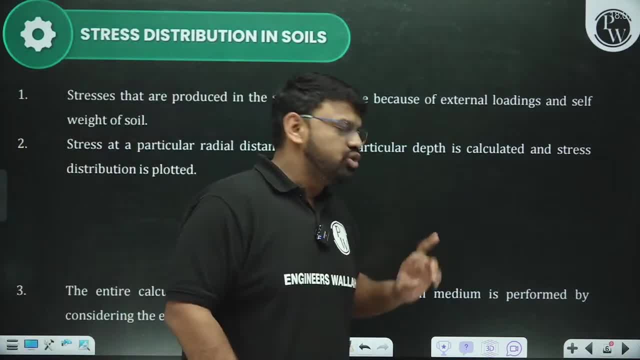 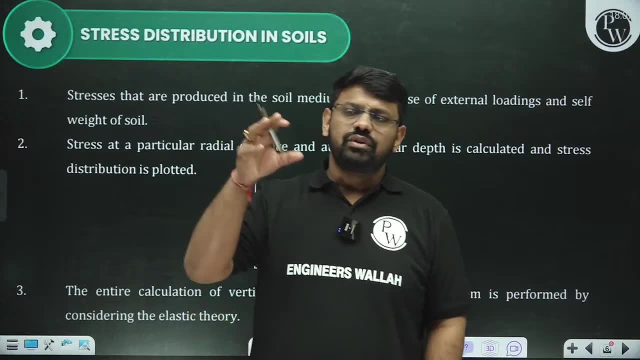 So, first of all, you will see what stress distribution means, Sir. we have read stresses in soil. Then what is this stress distribution, Sir? this stress distribution is basically a vertical stress distribution. You have to keep in mind that whenever you have a load, 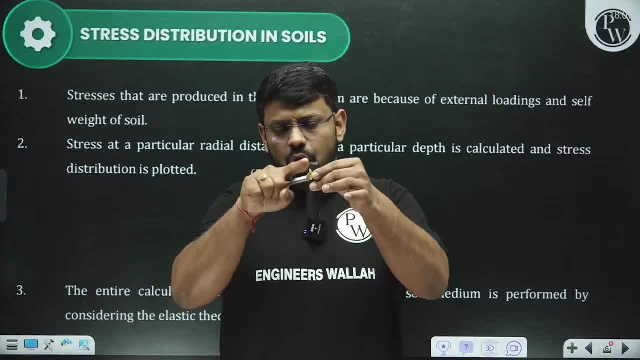 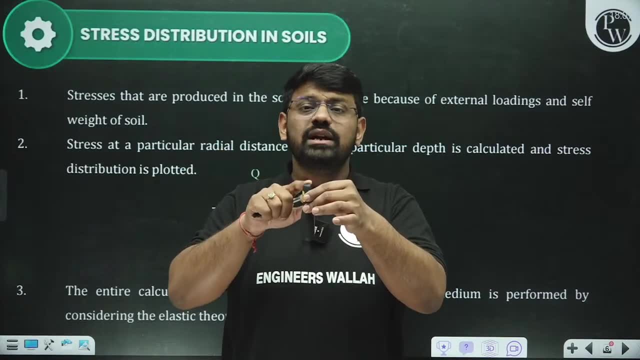 So, for example, a load is applied here And you have a layer of soil at this depth. There is a mass of a lot of soil here. So if you have a load here, then how much will the effect of this load come on a particular depth? Z? 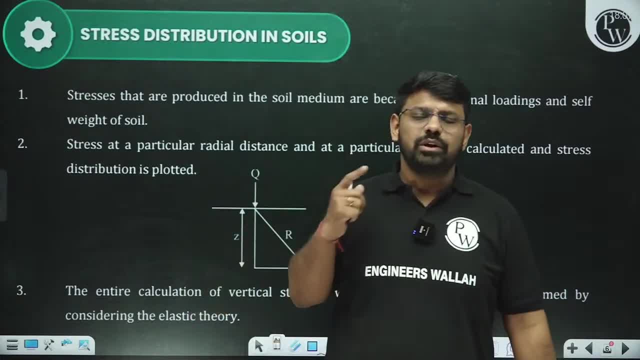 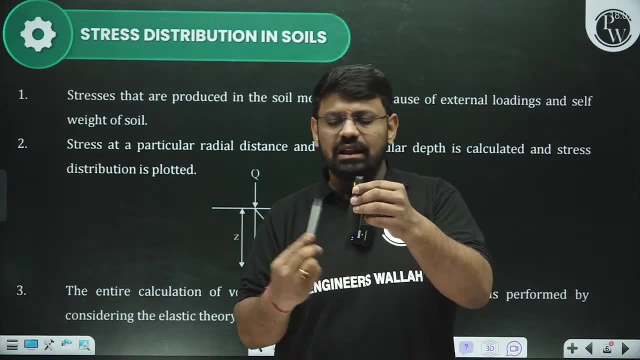 So we read the effect of that depth in this particular chapter. Okay, depth is fine. Along with that, what effect will it have on a particular radial distance? Sir, this stress distribution is basically a vertical stress distribution, That means in this complete periphery. 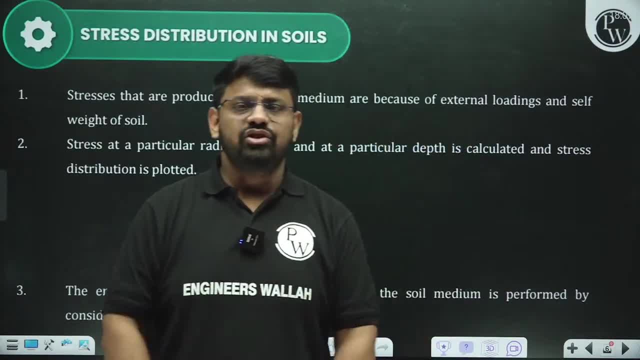 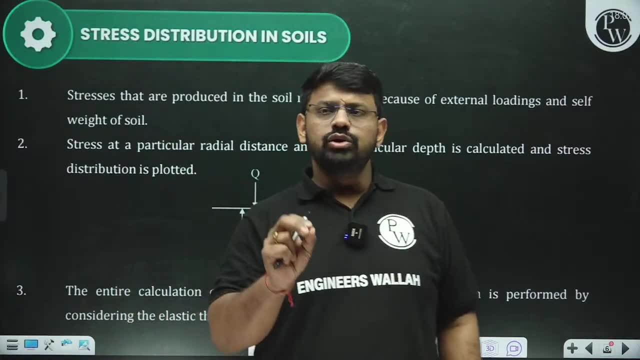 what will be its zone of influence. We talk about this in vertical stress. Basically, we have two types of theories in it. If you understand it carefully, then everything will go in your mind. We have to keep in mind the assumptions of both the theories. 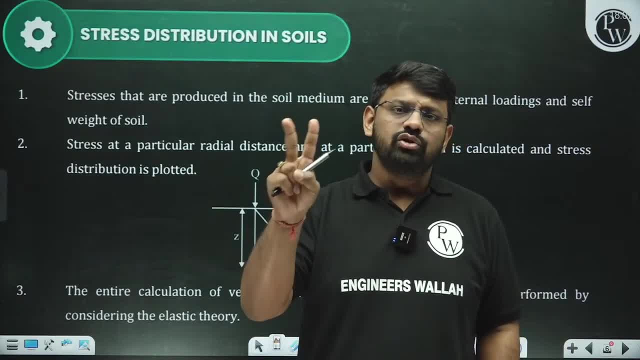 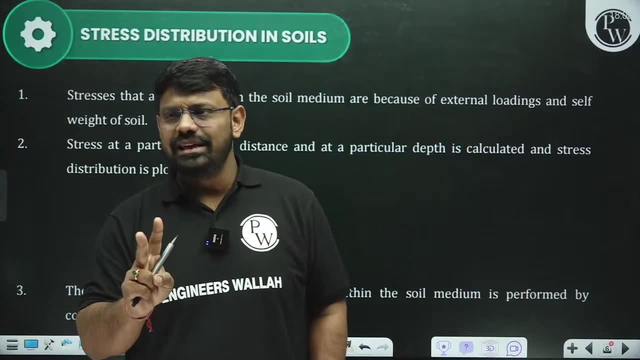 So all the children comment and tell me Which of the two theories is the most important in vertical stress. I hope you have read this chapter a little bit. I have told you two theories. We have two theories which are the most important. 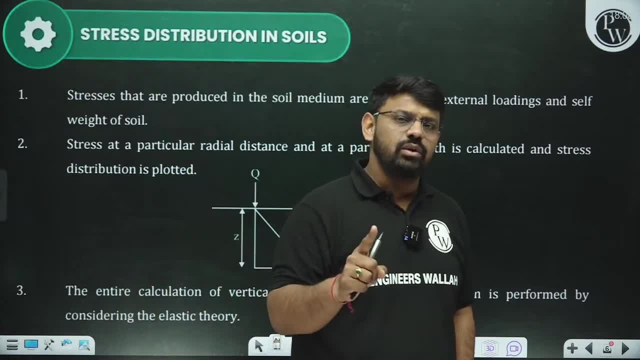 Sir, the first one we have is the Bosnian theory And the second is your Westergaard's theory. So Bosnian and Westergaard's theory are two theories by which we define our entire vertical stress. 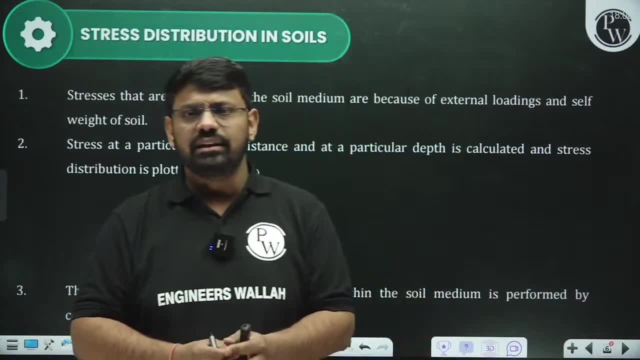 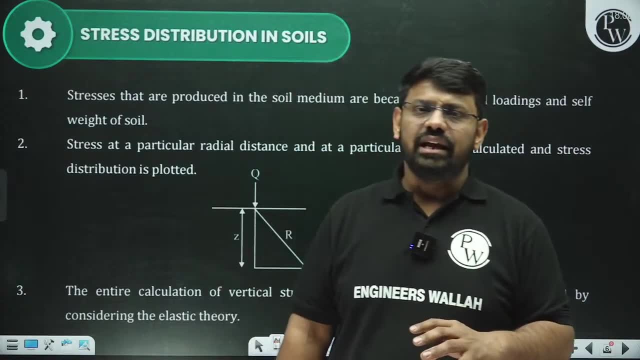 And these are the things in our syllabus Regarding this, the assumptions, the calculations, the formulas. we just have to remember them. And here your stress distribution chapter will be covered. very well, Okay, Look, sir. first of all, 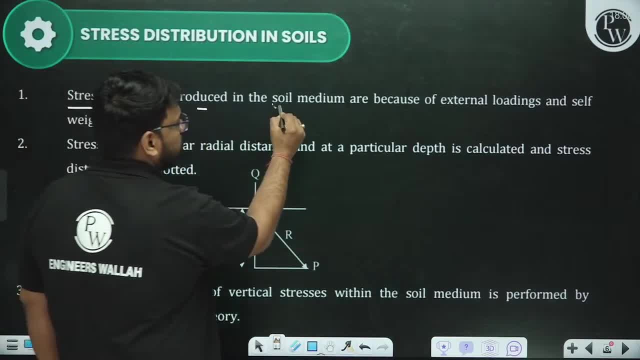 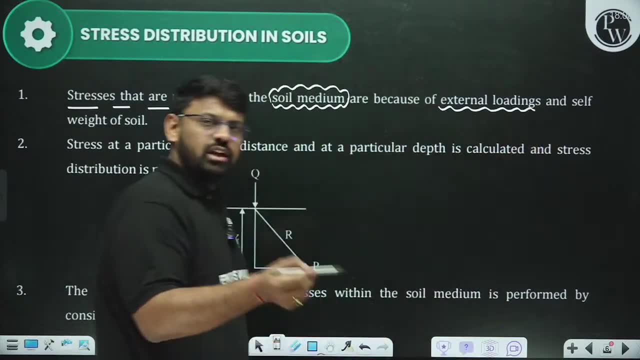 the stresses that are produced in the soil medium. in any particular soil medium, the stresses that are produced are basically the same Because of your external loadings. because of external loadings and because of the self-weight of the soil, they are produced. Okay. 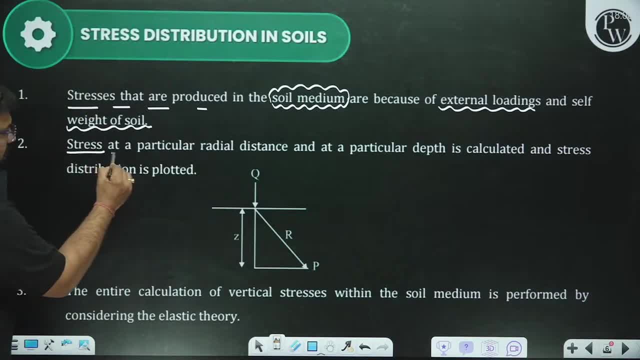 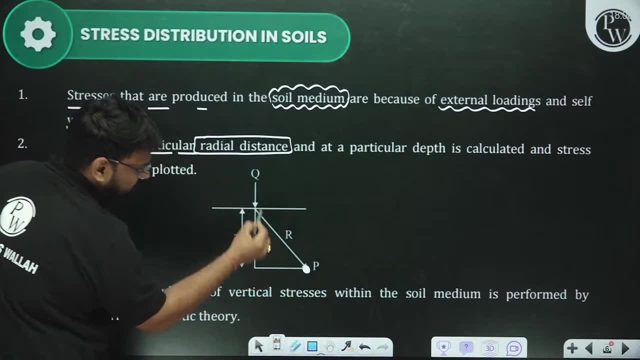 Either there is an external load or it can be produced because of the self-weight- Look ahead- Stresses at a particular radial distance, any particular radial, suppose this is the point. Now, what is the whole story, sir? The whole story is that you had this ground surface. 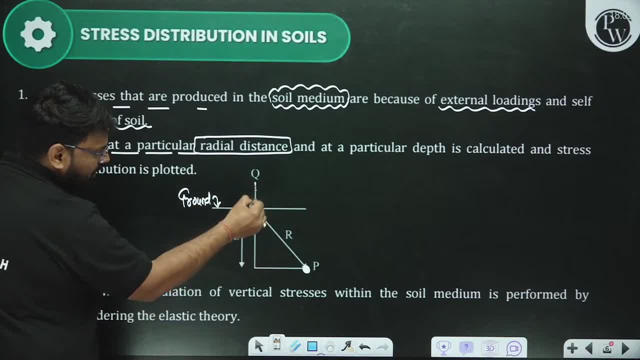 Sir, we have this ground surface And on this ground surface, somewhere here, you have a point load. Now, this point load, its effect, where will it come From here to here? the radial distance, ie look at its axis. 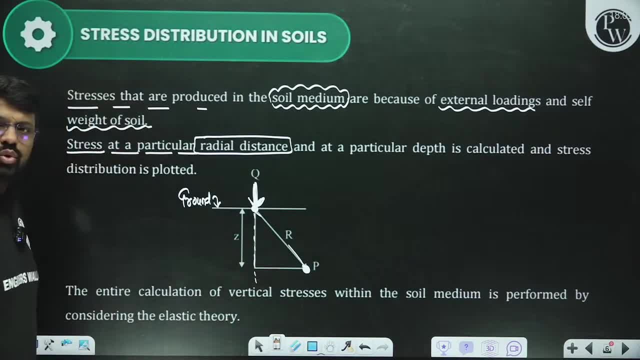 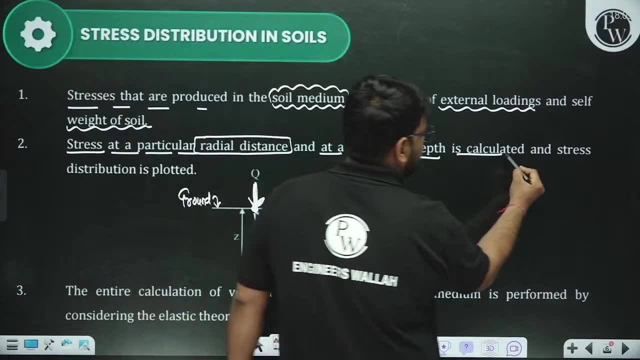 This load of application is here. So this much radial distance is far away from you. So how much effect does it have there? We will generally see this here. So at a particular depth is calculated. we will calculate that. 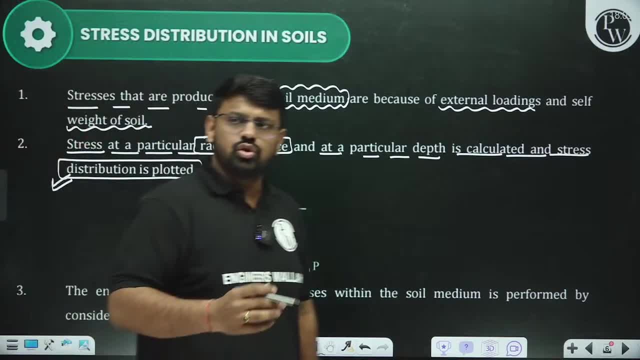 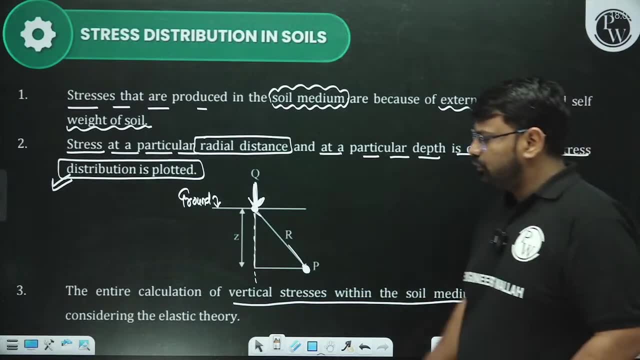 and we will plot the stress distribution. And from here we also plot the stress distribution. This is the most important thing, sir. And the entire calculation of vertical stress within the soil medium is performed by considering the elastic theory. Keep in mind that. 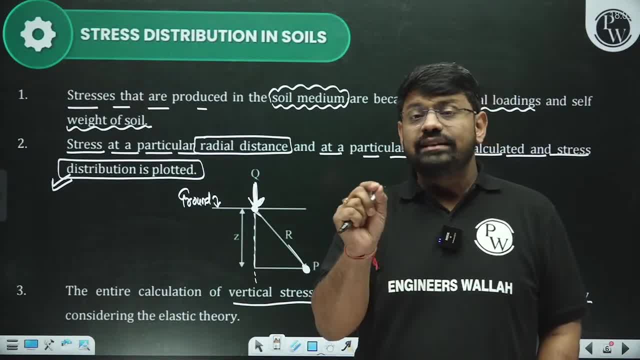 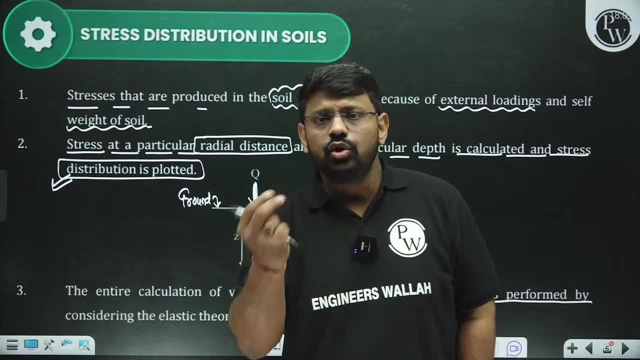 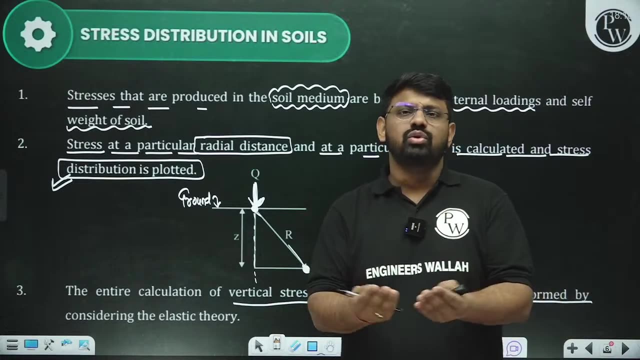 whenever we talk about vertical stresses, one thing may be asked. in the statement, It is asked that in the complete vertical stress distribution that we see, which theory do we generally apply? So keep in mind, by applying the elastic theory, based on the elastic theory. 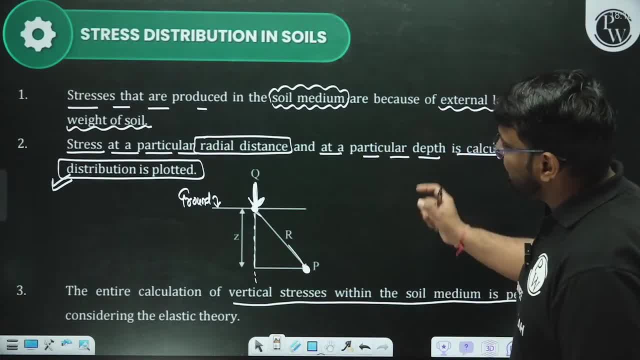 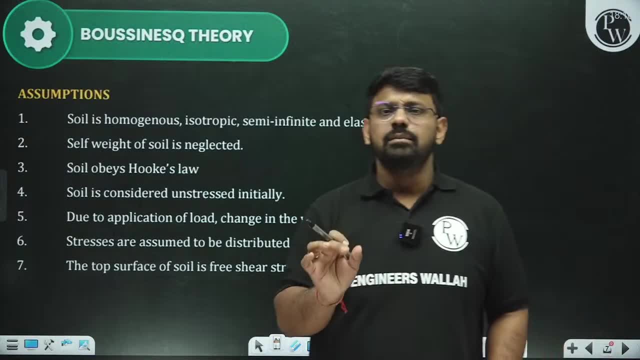 you discuss both these approaches, whether it is Bosinex or Westergaard. Let's move ahead, sir. The first theory is the Bosinex theory, And the most important part of it is its assumptions. So what did Bosinex say in the assumptions? 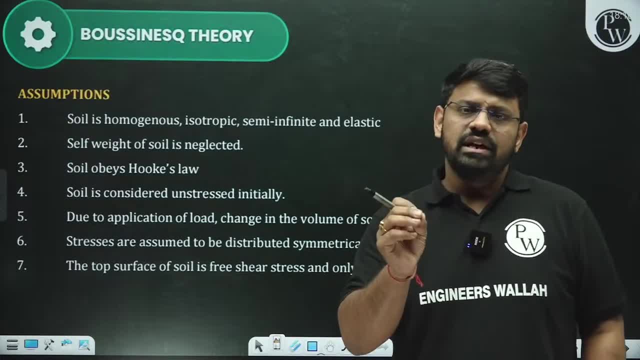 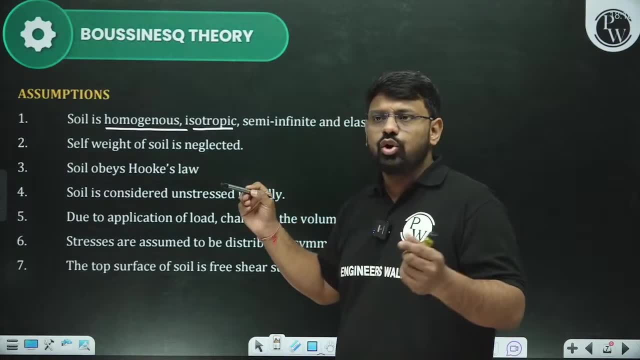 And what did Westergaard say? in the assumptions, You have to note all these points. well, First of all, we have homogeneous soil. You will have isotropic soil. These are common assumptions we have. After that, we have semi-infinite soil and elastic soil. 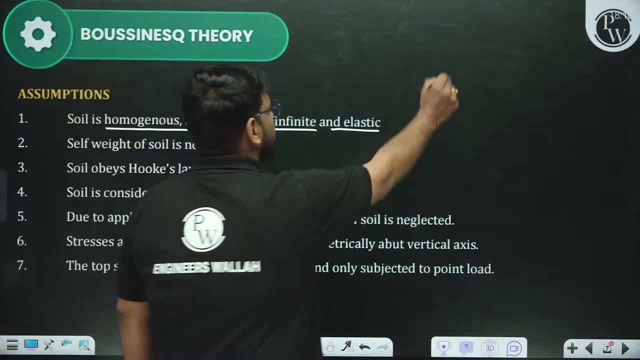 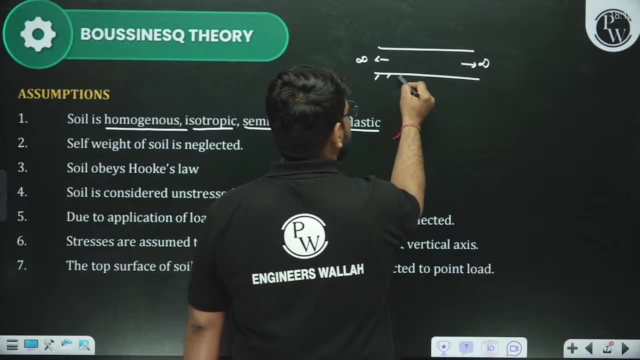 What does semi-infinite mean? Semi-infinite means that in one direction you have a good extent. Suppose from here it is in an infinite direction, And here you have a ground condition. So, sir, you know this depth. 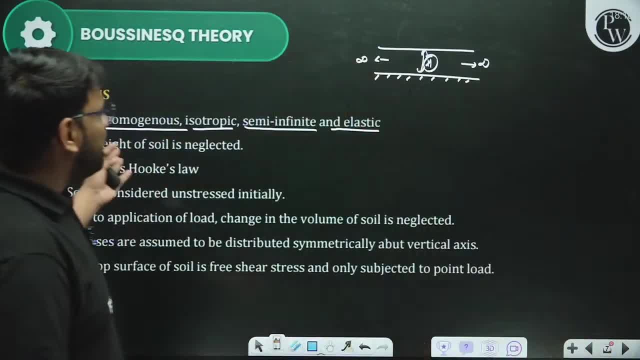 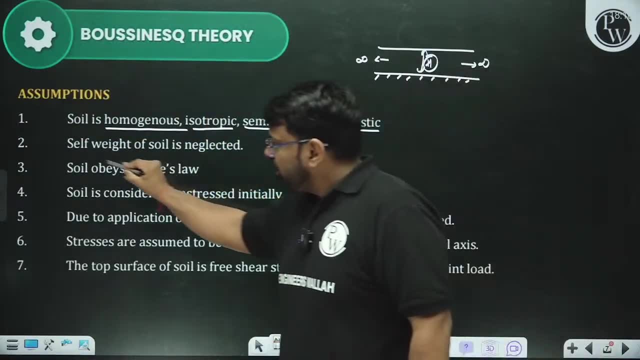 but it is infinite in one direction. So this is known as your semi-infinite medium. So it is assumed that we will have semi-infinite elastic, homogeneous and isotropic soil. We neglect the self-weight of the soil, So understand this thing carefully. 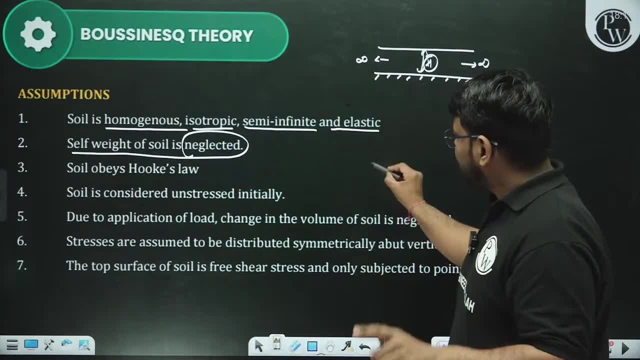 Sir, when Bosinex said in the theory, because I have told you that on any particular depth- suppose this is a particular depth or this is a particular radial distance- then, on any particular depth or on any particular radial distance, when you will have any load, 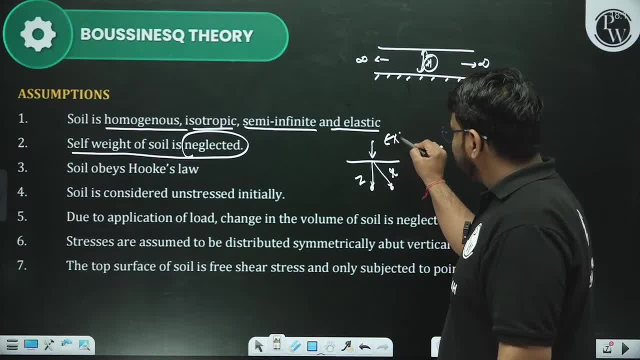 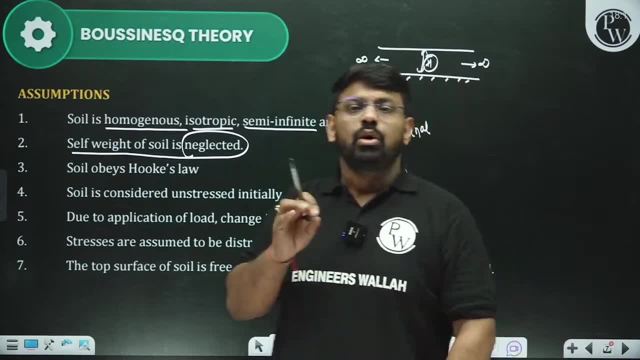 then here two types of vertical stresses can be produced, Sir. one is because of the external load and the other is because of the weight of the soil. But what did Bosinex say, Sir? the weight of the soil. you have to neglect it. 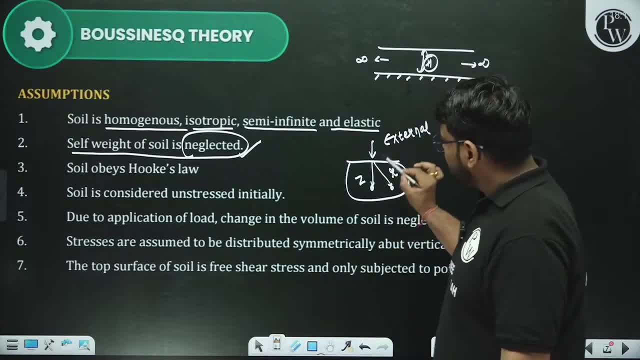 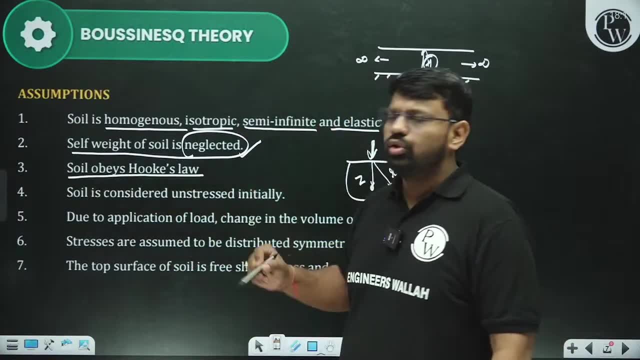 So the self-weight of the soil is neglected. This is the thing. This means only if the external load is applied. we will consider the effect of this. Look ahead. Soil obeys the Hooke's law. Soil will obey the Hooke's law. 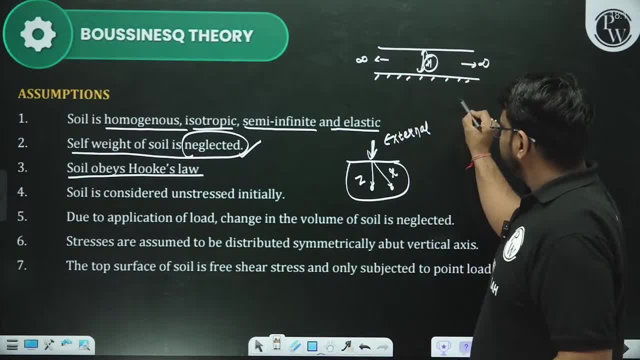 Obviously, the elastic theory is applicable here, So the Hooke's law will also be applicable here, That is, stress is proportional to your strain. This Hooke's law will also be followed here, So this point is also clear to us. 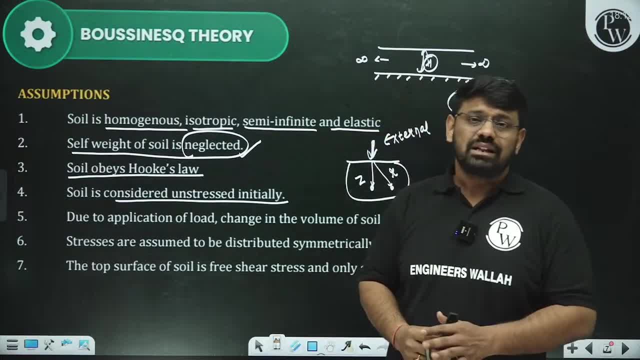 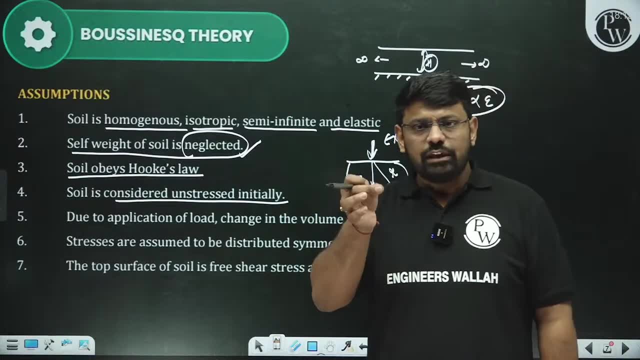 Soil is considered unstressed initially. Means Bosinex says that if you want to see the effect of any load on any point, if you want to see the effect of any load, then you have to keep in mind that before this load, 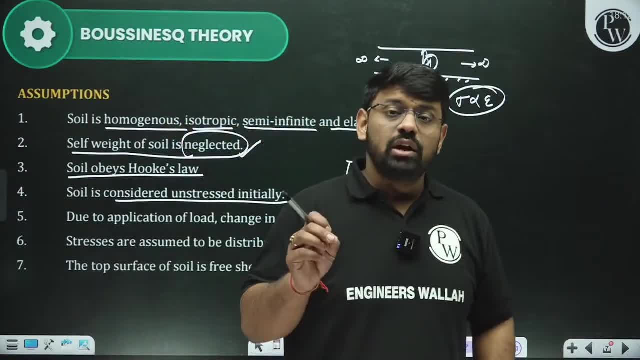 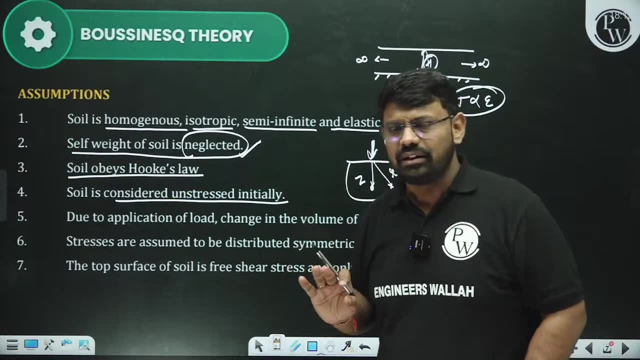 there should not be any other load on that particular soil Means. soil should be unstressed. initially. The load you are applying is the first load that is applied on the soil. Only then we can consider that effect from there, Absolutely clear. Next, due to application of load, 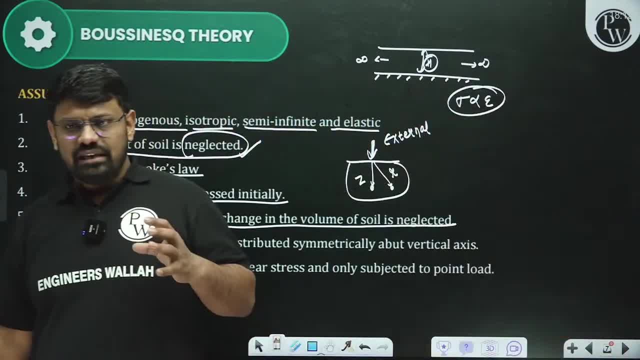 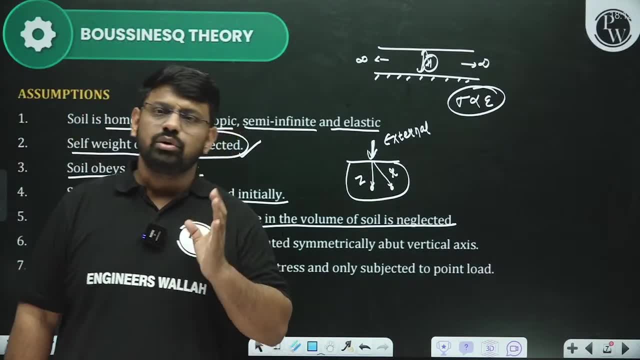 change in the volume of soil is neglected. Now, when we are applying the load, as soon as you apply the load on any particular soil, you get to see its volumetric changes. So what did Bosinex do? He ignored the volumetric changes. 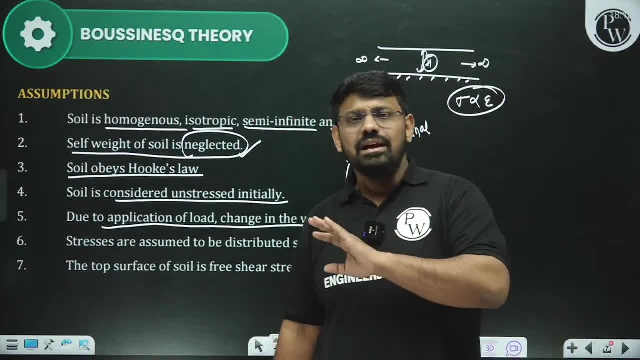 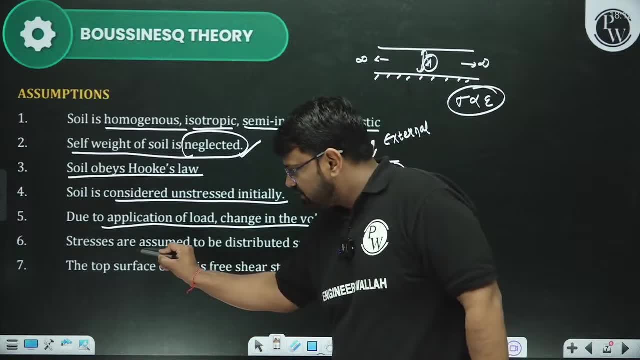 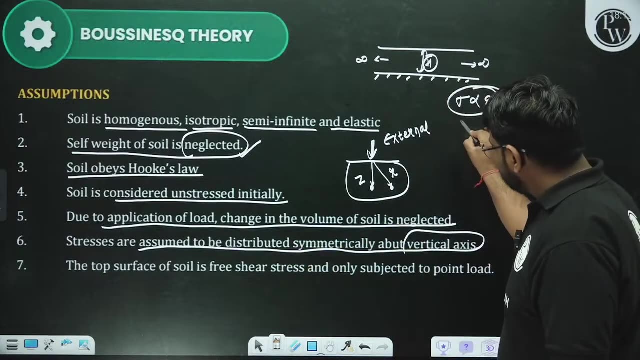 So what will be the volumetric changes? It will be completely ignored. We are not assuming that you are getting to see any kind of strain in your soil. Next, stresses are assumed to be distributed symmetrically about the vertical axis, And we are also assuming that. 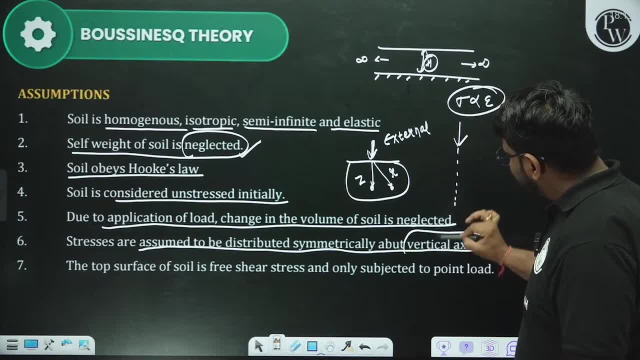 you will get to see the vertical axis. Suppose this is the load. Now, this is the vertical axis. So the effect of the load on this particular point, suppose this distance is here and this distance is here. So if I see its second point symmetrically, 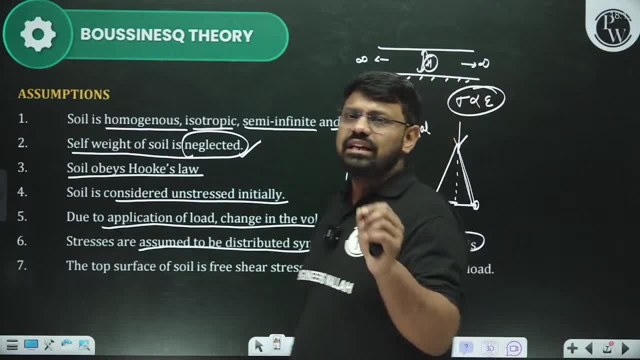 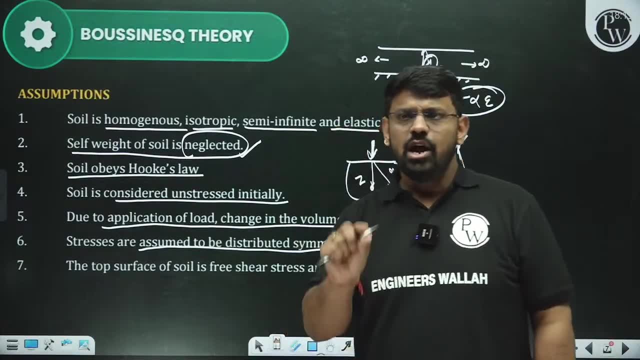 on this side, then its effect here and here will be exactly the same. So here you can understand that, to justify your theory, Bosinex has neglected a lot of things and put a lot of things into assumptions. So what will be here? It will be symmetrical. 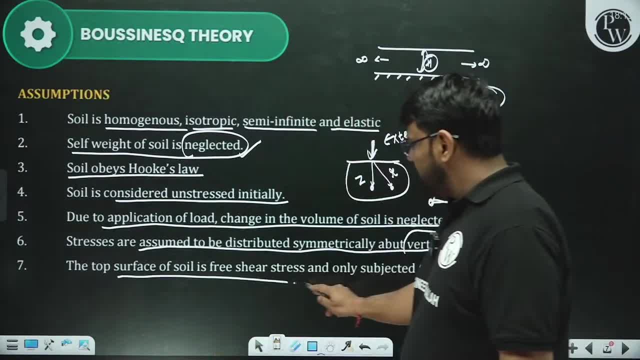 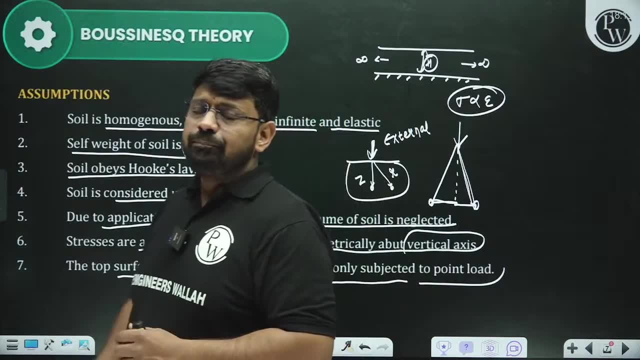 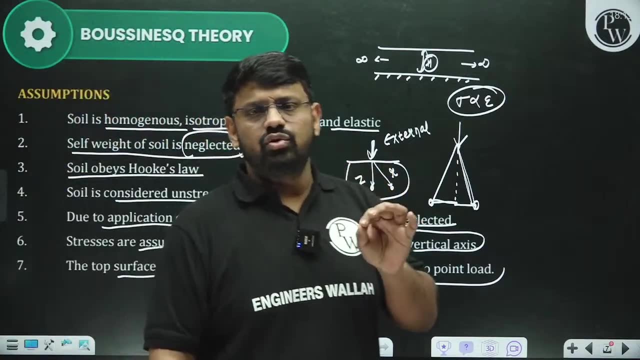 The top surface of the soil is free from shear stress and only subjected to point load. Now you must be thinking that it can be a shear component. Shear component or shear stress is also neglected. So we have to remember all these assumptions. 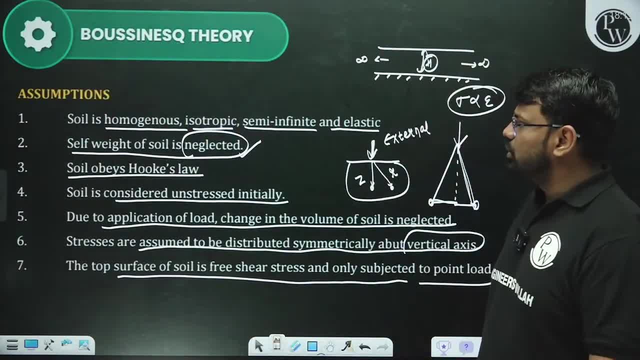 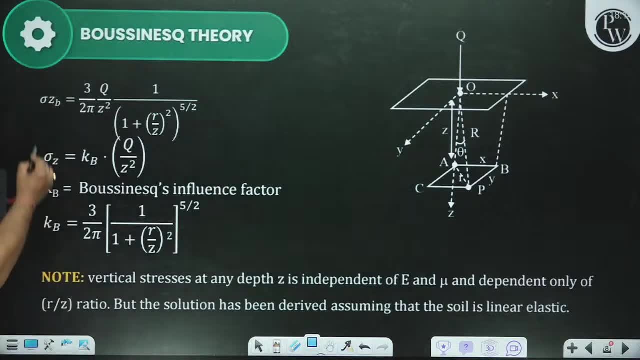 very well. The first point is clear. Now, using these assumptions, he has given a formula and you can be asked that sigma z, the vertical stress that we have, that will be equal to 3 upon 2 pi q by z square 1 upon 1 plus. 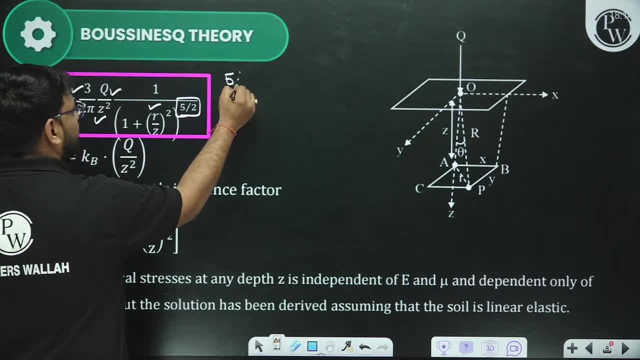 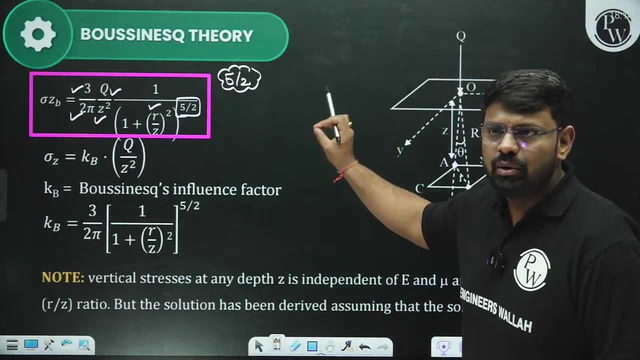 r by z, square power 5 by 2. Remember in Bosinex that this power will be 5 by 2.. You have to remember this. r by z, power, 5 by 2.. So we have to remember this formula very well. 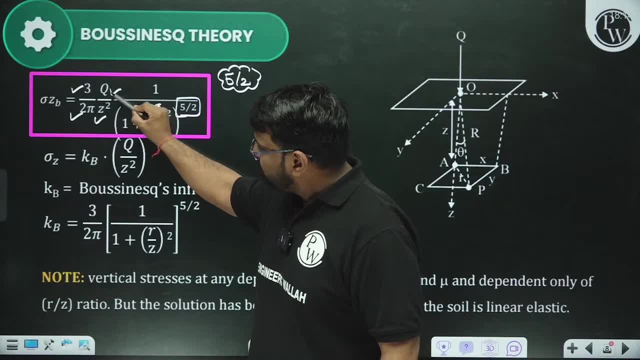 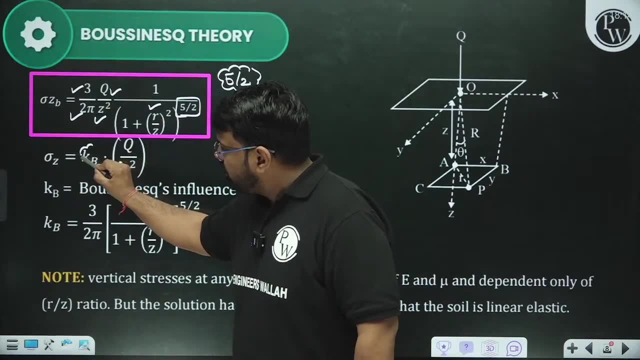 Now see here: what will you do from here? q by z square that we have? if I separate q and z square, whatever the term is, you have made it a constant- and that we have kb- kb means Bosinex constant. 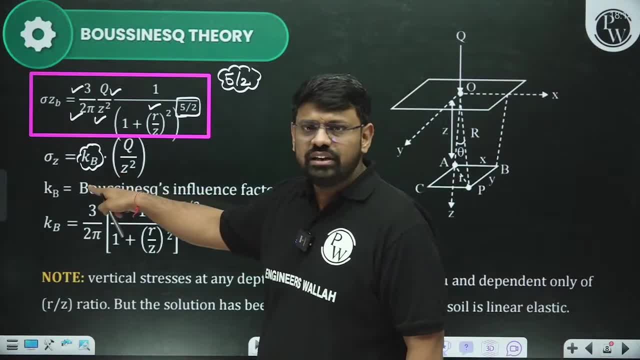 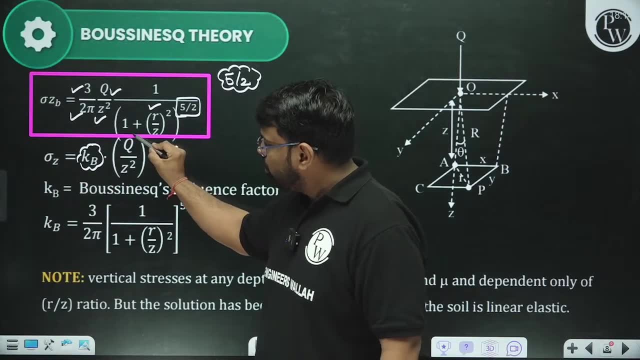 What happens, sir? Bosinex is a constant. So here, kb is the Bosinex constant and q by z square you have. So the vertical stress that we have is directly dependent on us, The external load you have applied. if you increase the external load, 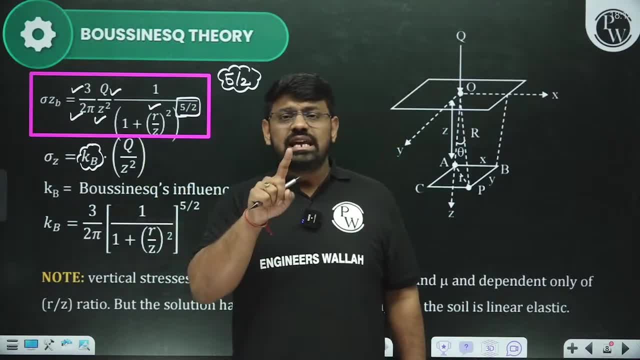 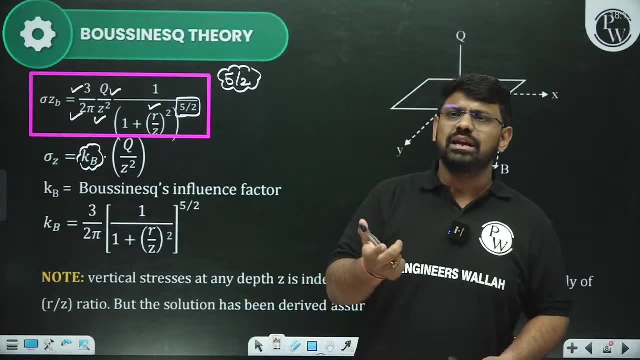 the vertical stress will increase. Similarly, z square is inversely proportional to z square. So the more depth you apply, we know that the point of application- like in SOM you must have read something- that the particular point of application on which the load is applied. 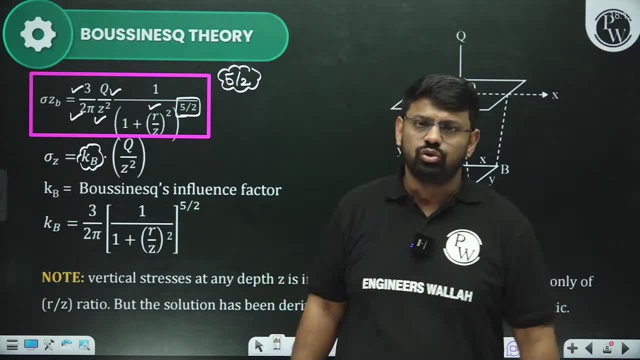 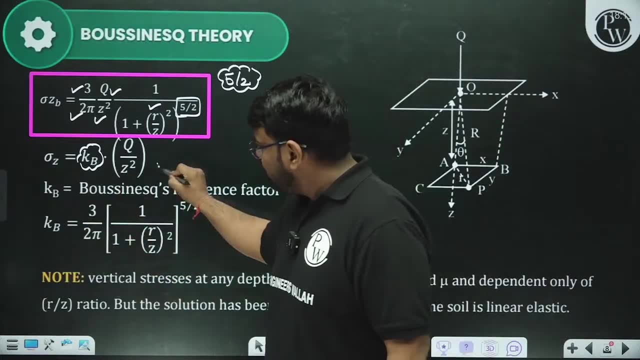 if you go far from it, then the effect of the load starts to decrease slowly. So definitely, as the depth increases, its effect will decrease. So you are also getting to see this in the formula. So you just have to remember this direct formula here. 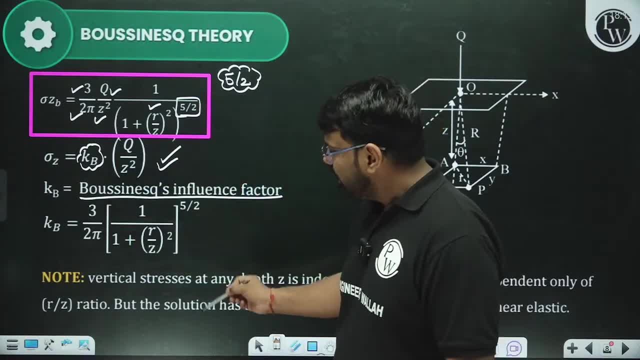 So kb equal to Bosinex influence factor. we call it Bosinex influence factor and you see separate q by z square rest. this whole term is called kb, That is, Bosinex influence constant. Okay, sir, it is clear till here. 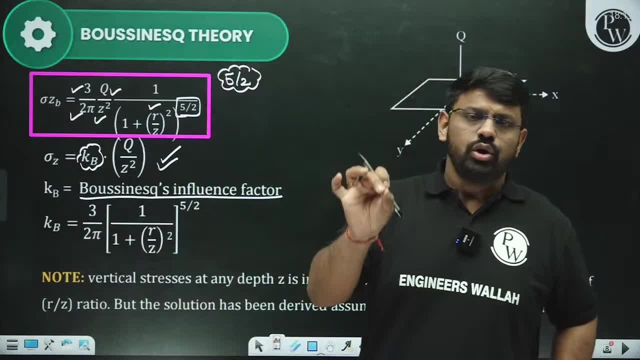 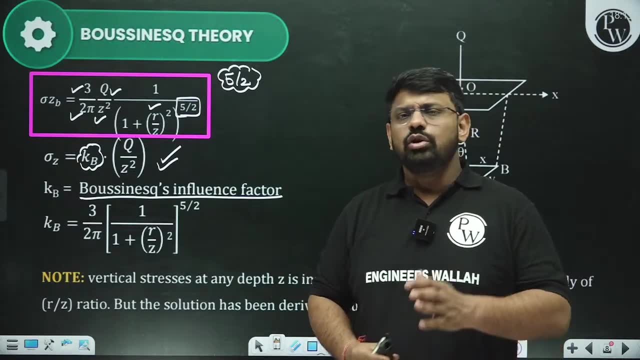 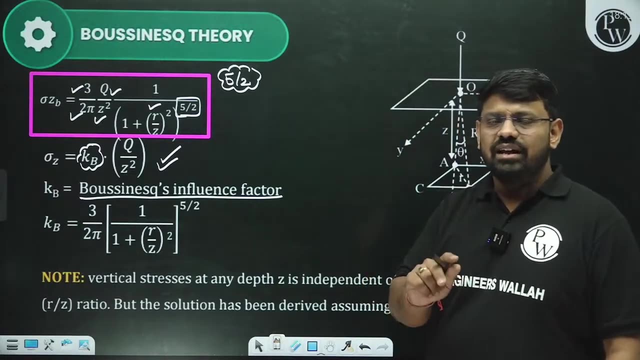 Now from here. I had told you, that it depends on elastic theory. So, sir, if elastic theory also depends, then in our mind one thing is clearly printed: then modulus of elasticity, then the Poisson's ratio, all these factors should also depend. 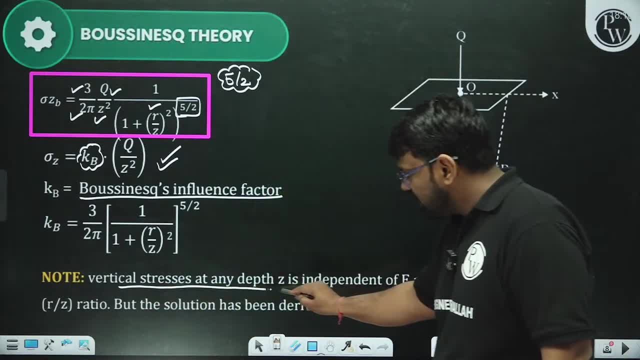 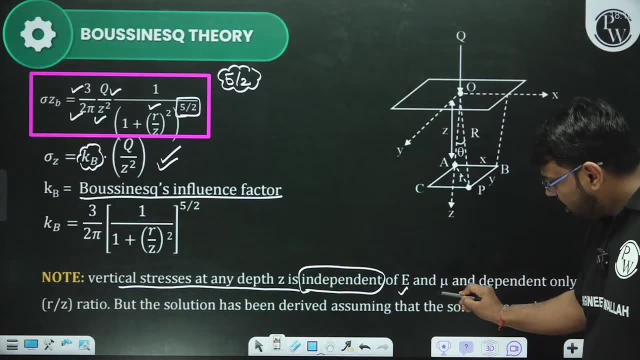 So see here, understand this clearly: The vertical stress which we have at any particular depth, if I am talking, is independent From whom? it is independent From modulus of elasticity and Poisson's ratio. It is independent, Although you have calculated, from elastic theory. 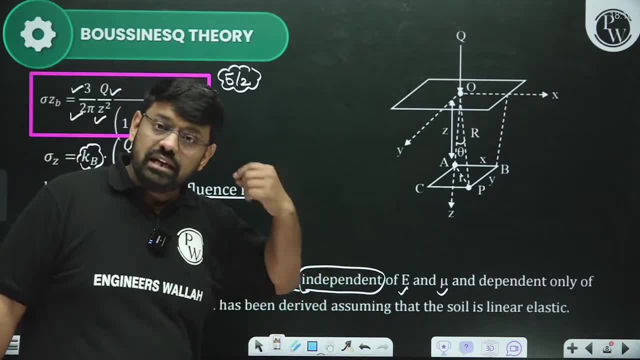 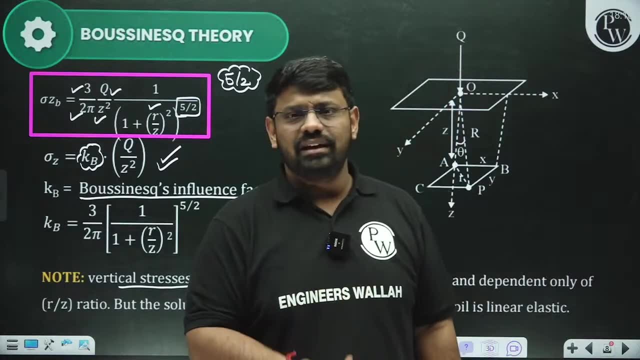 still, this modulus of elasticity and mu will be independent. Why? Because, sir, first of all, volumetric strain is neglected, Sir, when volumetric strain is neglected, then all other things of elasticity are finished, Sir, lateral strain etc. are finished. 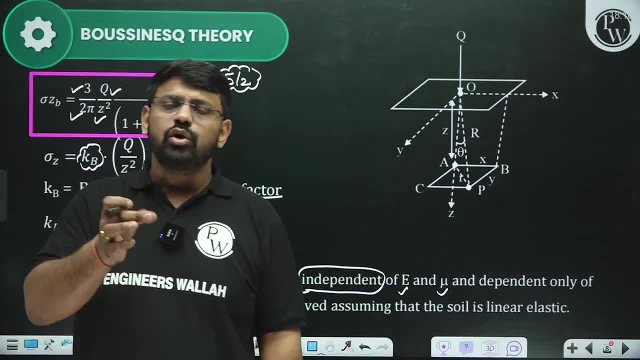 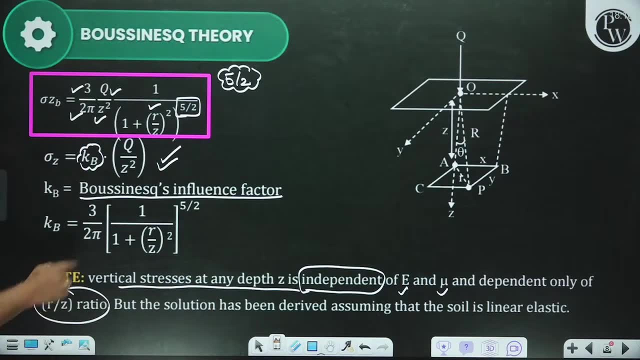 So because of this modulus of elasticity and mu, there is no dependency here. But on whom it will depend? It will only depend on the ratio of r by z, which you can see here. This is the ratio of r by z. 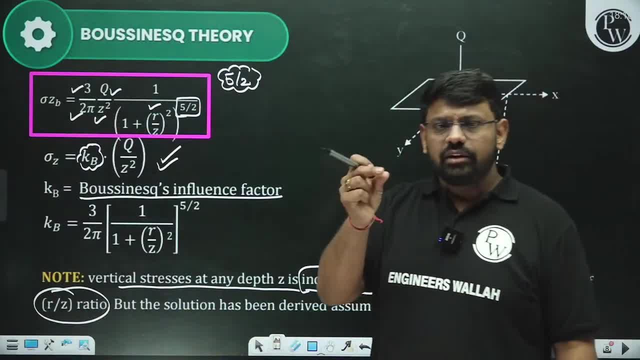 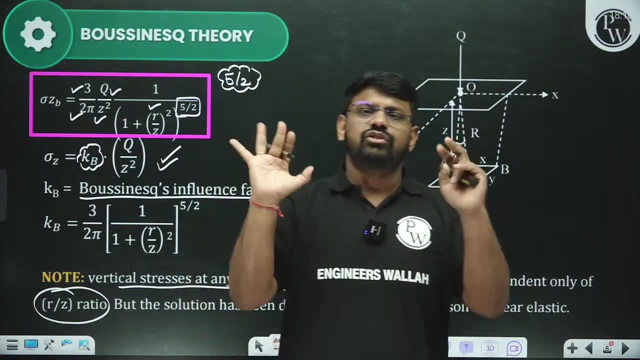 And it depends on this. So, this common sense, it can be a tricky question from you, Because when you remember the assumptions in your mind, then it will be clearly in your mind that elastic theory, And after elastic theory it will write E. 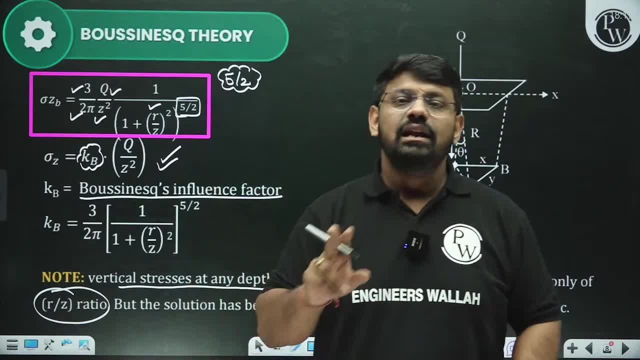 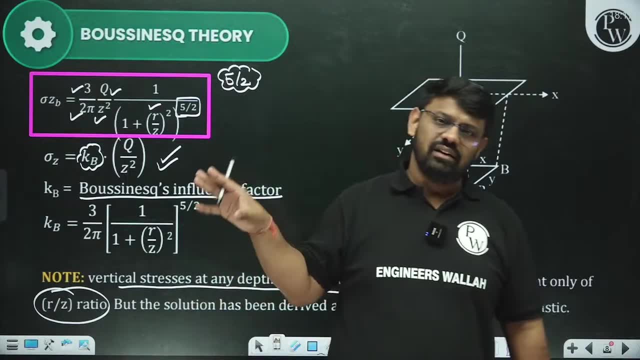 E will come in your mind as soon as you write E. It means it should depend on modulus of elasticity. Modulus of elasticity is independent Because Bosinex has ignored a lot of things. That is why you have to keep this assumption in mind. 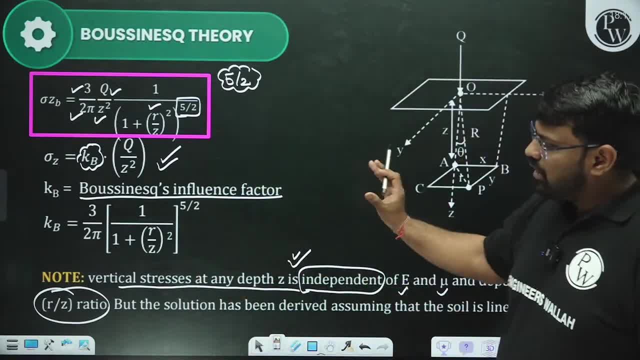 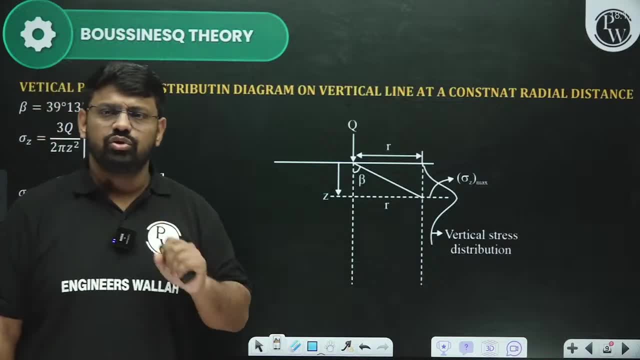 You have to keep this note in mind, Sir. in a very good way, we have remembered the formula. We have remembered the influence factor of Bosinex. Now look ahead. You have to remember one more data which was asked once. 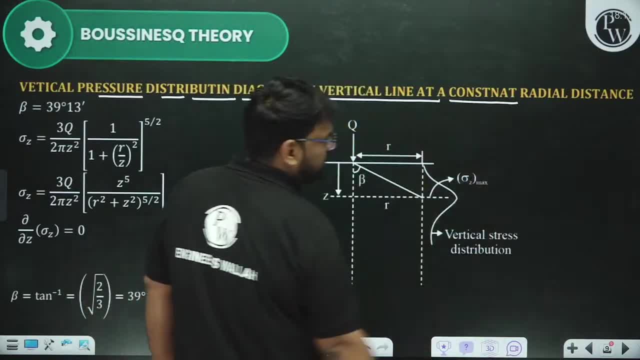 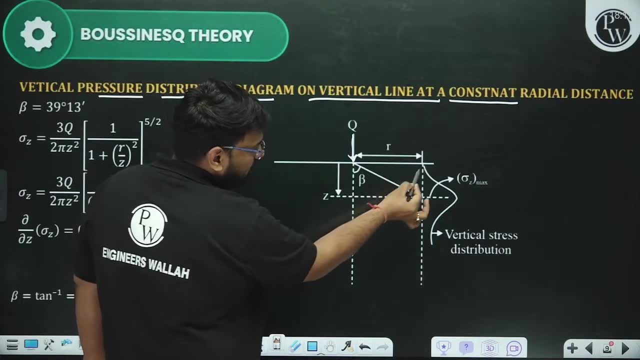 What was asked, sir? That vertical pressure distribution diagram on vertical line at a constant radial distance. Sir, this is a load on a particular point And this is depth z. So this is a vertical stress diagram. It means in this direction, this is your diagram. 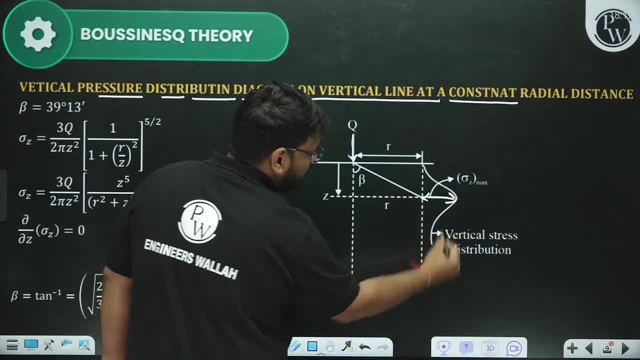 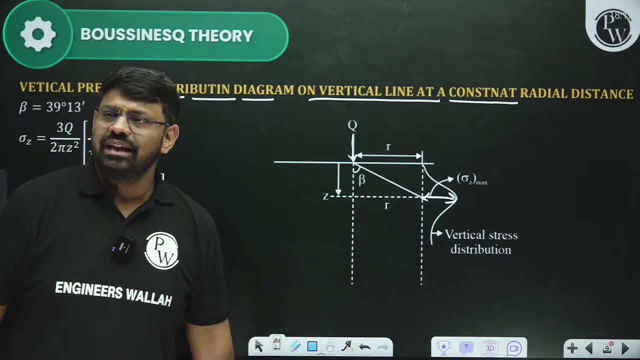 So, on this diagram, the maximum value of pressure at which particular angle, you get to see. this is also asked by you. And, sir, they say: what is the meaning of r by z Son? if you ask such questions, if you ask such questions, 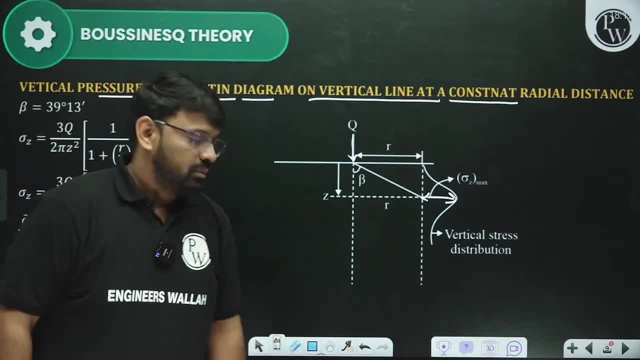 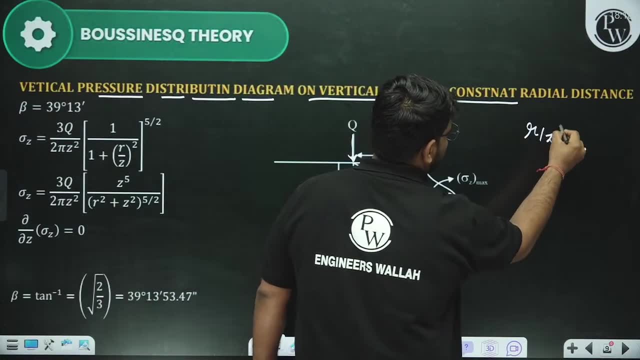 then what will be done? What will be done? Tell me What will be done If I say r by z. Now I am writing again and again and you are asking, son, what is r by z? r is radial distance. 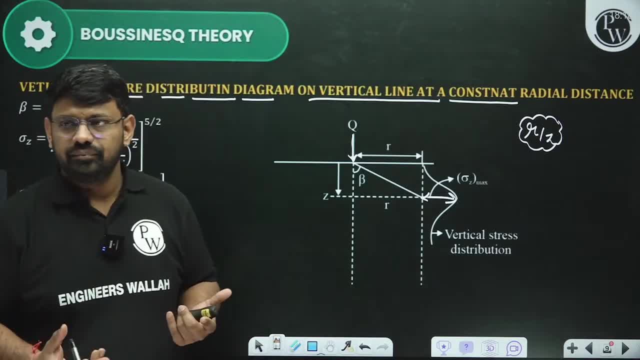 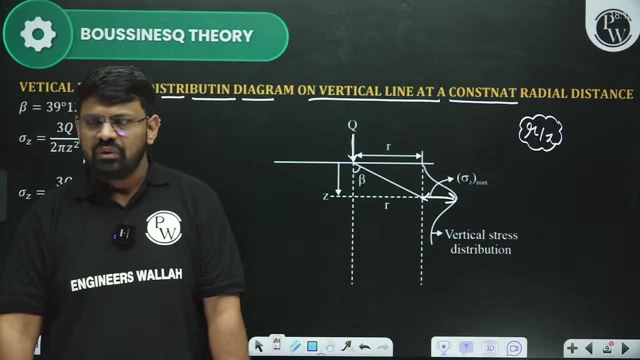 z is depth. This is the matter, Isn't it? This is the matter. It was a simple thing, Okay, sir. So look here. No problem, sir. Focus a little, son. Focus a little, You will understand things. 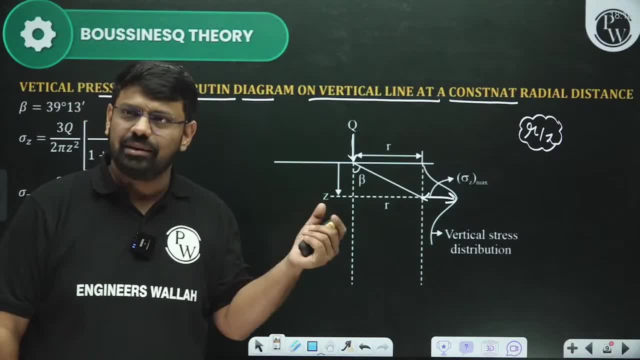 You are studying for the first time. I know this thing, But you keep this in mind. Focus a little. I had just written: r is radial distance, z is depth. I have written this. Okay, Now look here, sir. 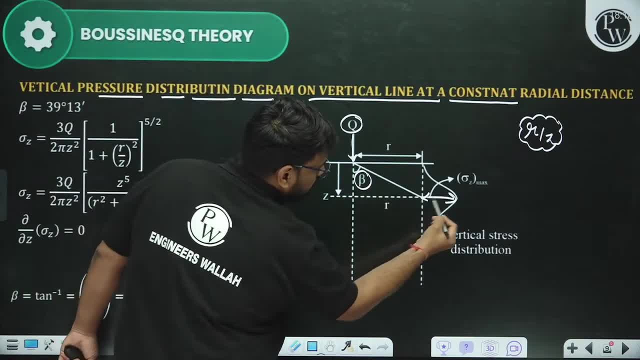 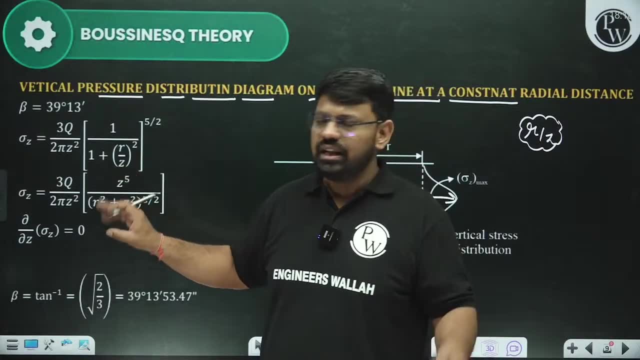 If you are having vertical stress, then b means at which angle will you get to see this maximum value? You can derive this very easily from the Bosnian theory. Look, there is no big way to derive it. For example, we have sigma z. 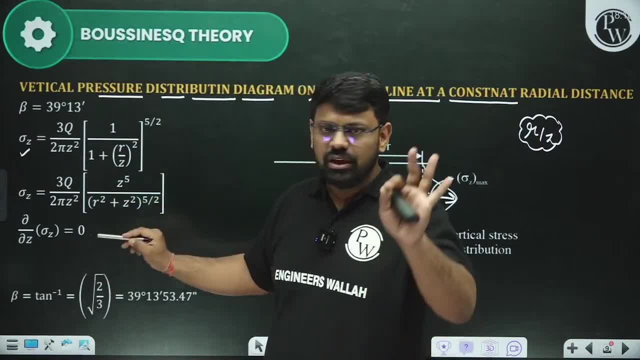 So everyone remembers this formula In the mind: 3q upon 2, pi z square 1 upon 1 plus r by z square power, 5 by 2.. 5 by 2.. 5 by 2.. You will remember, sir. 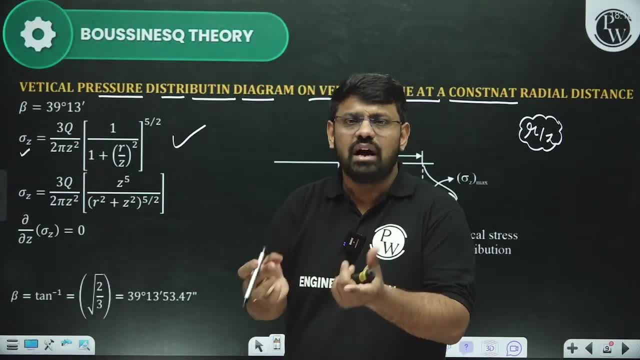 It is a simple question. Now, what will you do from here? Maximize, See where the maximum stress will be. So what did we do for maximum and minimum? in childhood We used to do partial differentiation. So, sir, what will you do after partial differentiation? 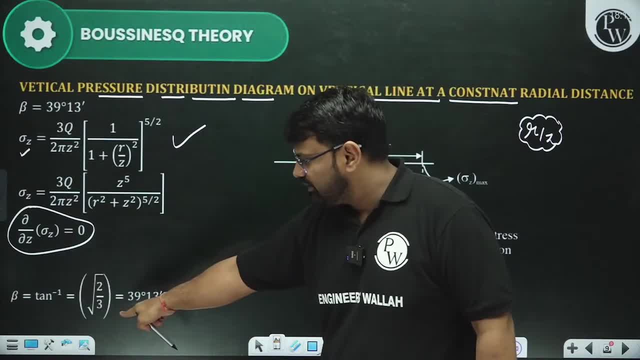 You will make it equal to zero. And from there, when you make it equal to zero, then from here you will get the value of beta. in this way Means 10 inverse under root of 2 by 3. So from here, 39 degrees. 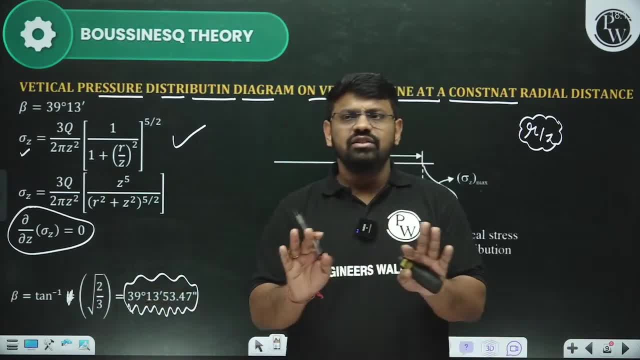 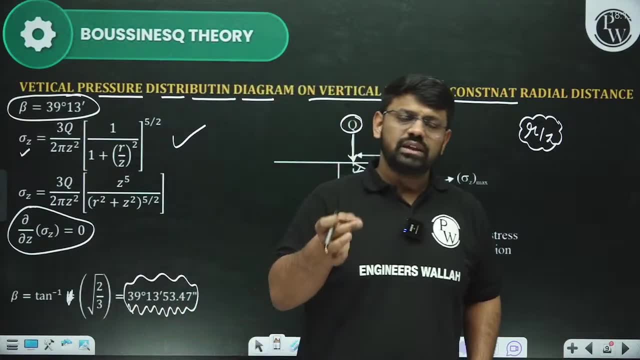 13 minutes and 53.47 seconds. So you don't have to remember the derivation, You have to remember this final result, Which is 39 degrees 13 minutes. And what happens, sir? This happens that whenever you have any vertical load, 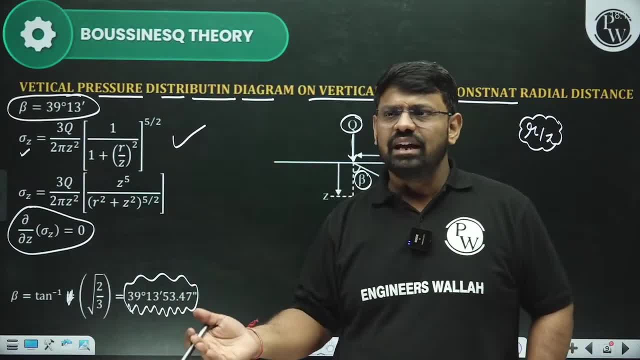 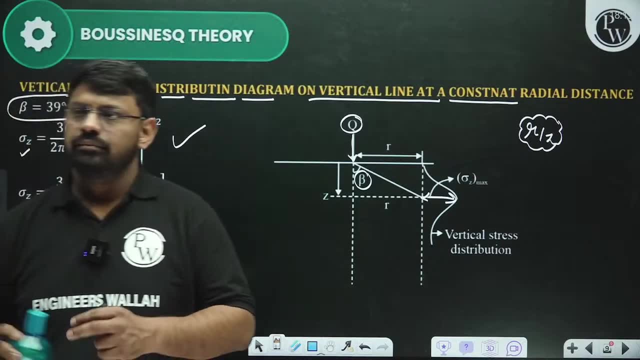 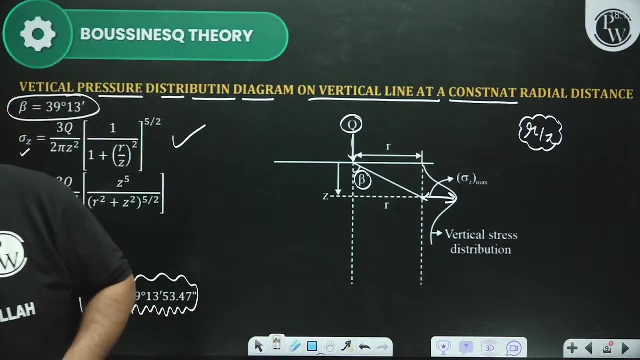 then if I take the vertical see, if I take the vertical see, see Hathim. Hathim has come to us Absolutely. son, All the children of Hathim will listen to you And open your heart and ask your doubts. 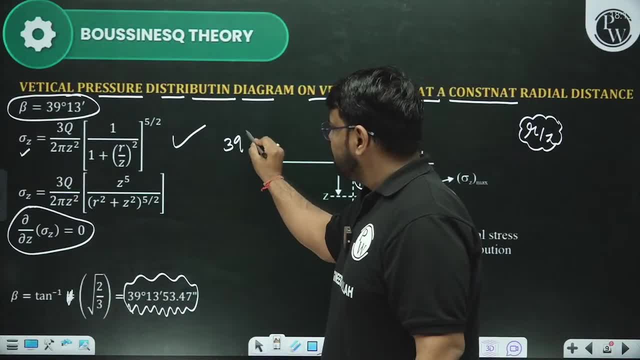 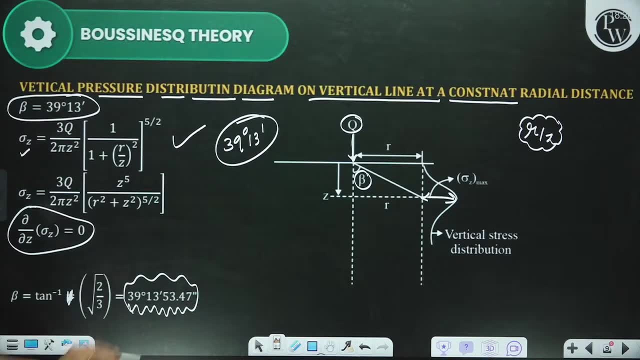 Open your heart and ask your doubts. Very good. So, sir, here we have 39 degrees and 13 minutes. This is beta. This is the beta. Okay, sir, This is your beta, So you just have to remember this value. 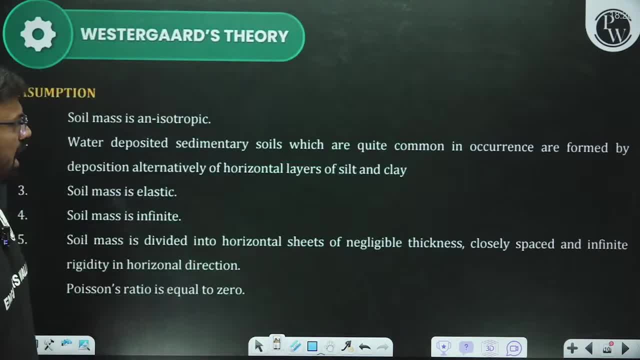 If the question can be directly asked, then it can be asked. It is a very clear thing, sir. Now look ahead. Sir, the first theory of Bosin-X has become very clear to us. The second theory is sir Westergaard's theory. 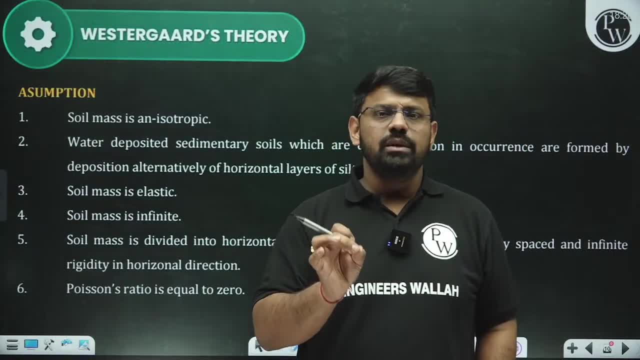 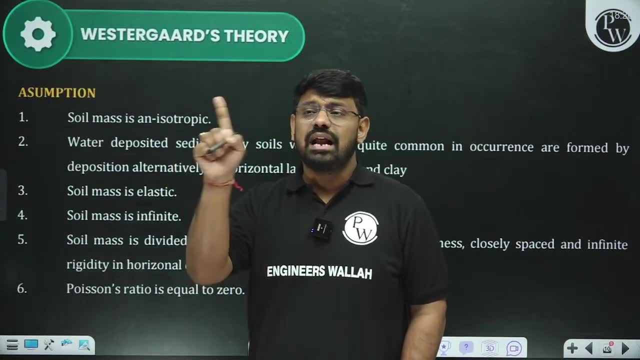 Now, sir, the Westergaard theory that we have. we also have some assumptions of the Westergaard theory. Now, what is to be understood in assumptions, Sir? the first assumption, the most important assumption, which is asked to you many times: 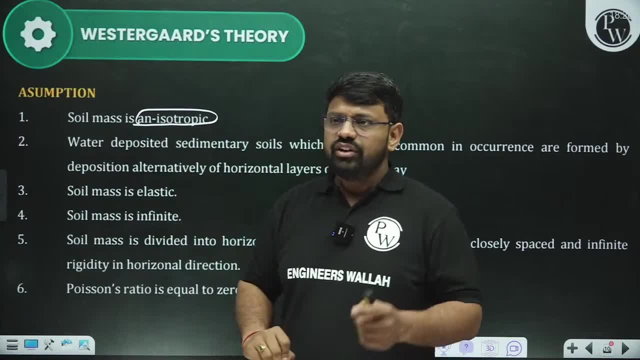 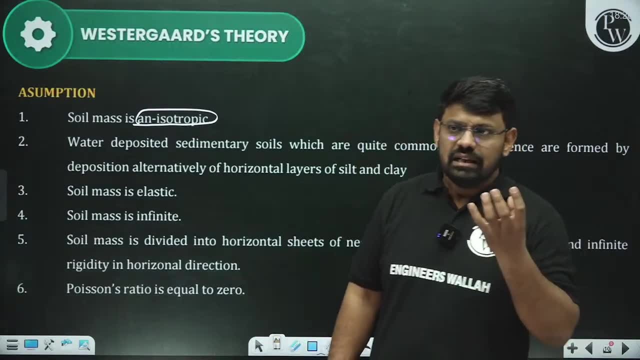 that is, sir, soil mass is anisotropic. Okay, Because generally it will be said that soil mass is always considered to be isotropic. Whenever we take assumptions in every way, then we take isotropic, But but here we have anisotropic condition. 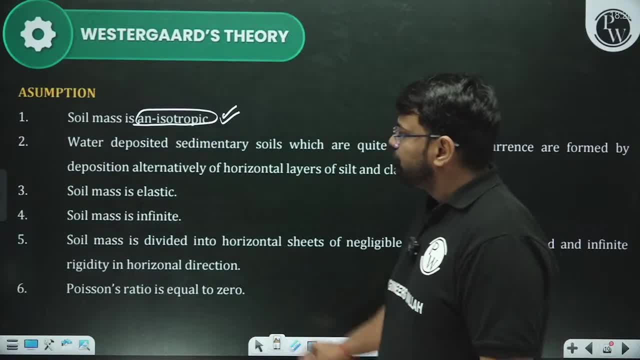 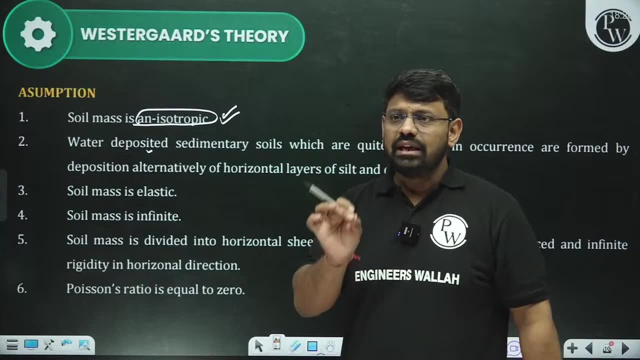 So soil mass is anisotropic. This will be the first thing. Now I am telling you this line first. I am telling you this line first. Slowly, slowly, understand this first line, Because this line is a little difficult. 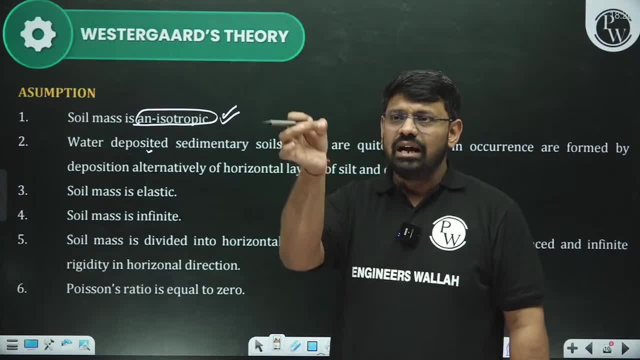 Isn't it? The line is a little difficult, So I am telling you first What was his name: Mr Hatim, you also understand, And Mr Arshad, you also understand quickly. So you have to focus a little, Okay. 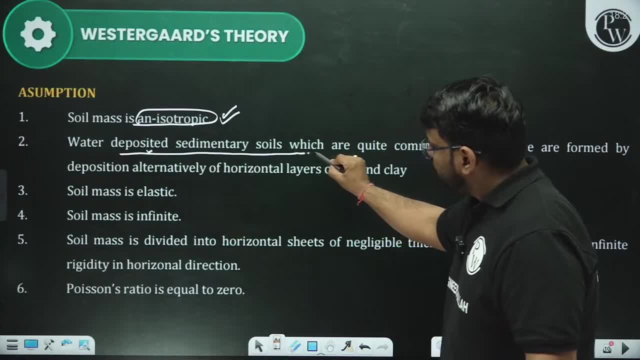 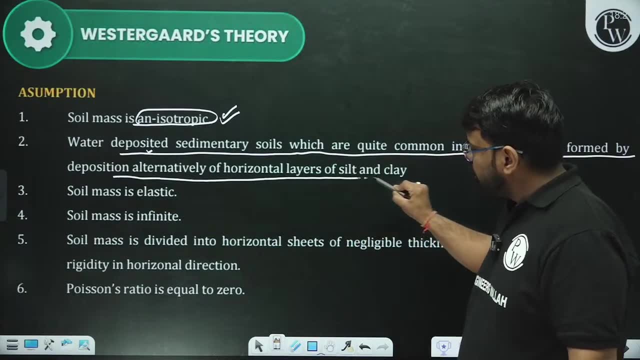 Now look, sir. Water-deposited sedimentary soils, which are quite common in occurrence, are formed by deposition of, alternatively, of horizontal layers of silt and clay Means. generally, when we talk in general, in general, when we talk in general, 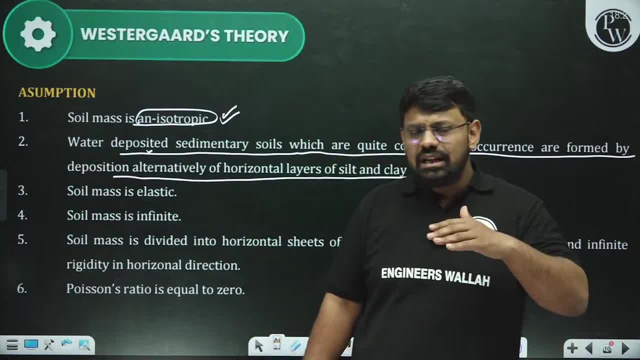 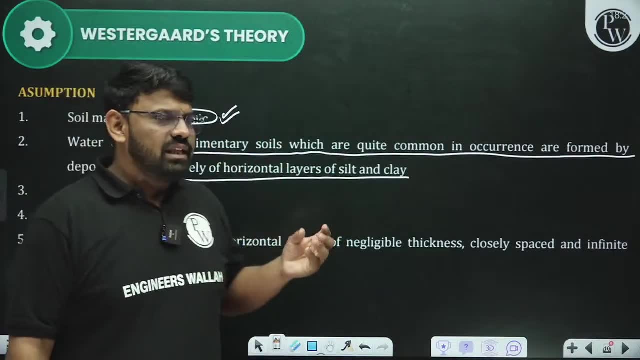 then all the soils we have, sir, they are formed in layer by layer, stratification. And sedimentary deposits are also formed in stratification. So Vestergaard theory wants to say that general common occurrence means generally what you see. 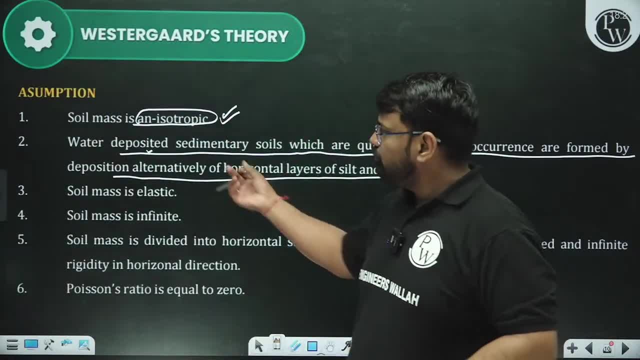 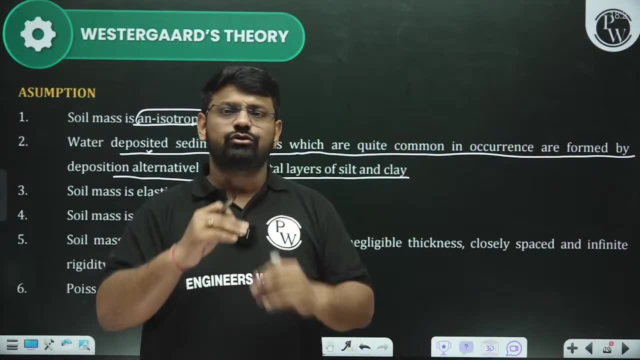 we have sedimentary deposits, Okay, And that sediment deposit is water-deposited, So we get to see those sedimentary deposits through water, And in these deposits you will have alternate layers of silt and clay, So you get to see these alternate layers of silt and clay. 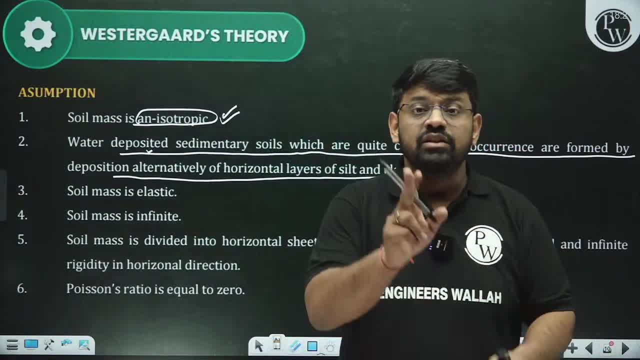 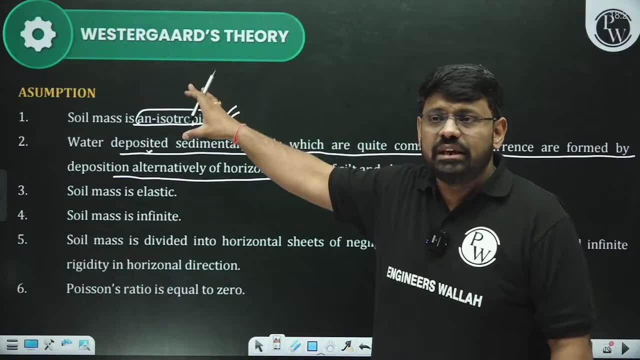 here This kind of soil condition is there. What is this kind of This kind of soil condition is there? First thing is clear Now: if you see, here this is the soil condition For that Vestergaard is applicable. So when Vestergaard 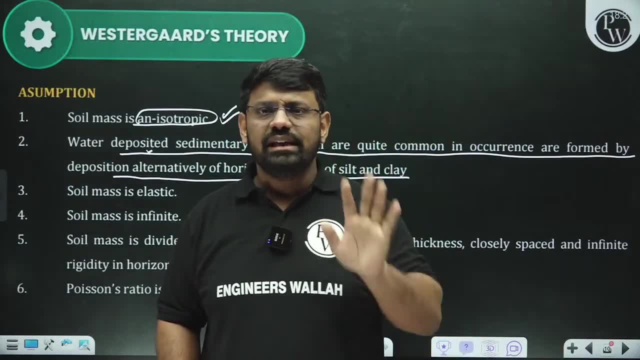 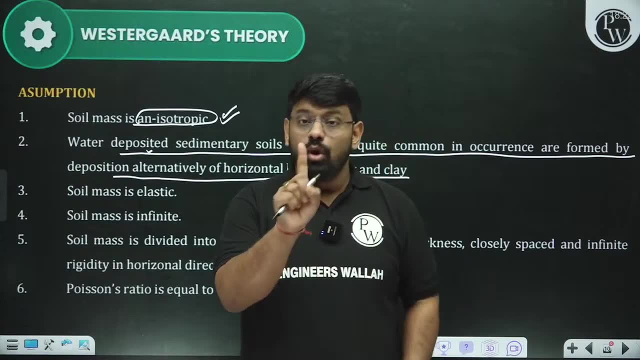 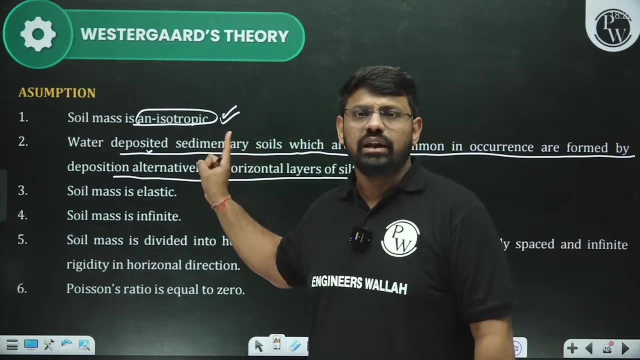 said this, sir, we are commonly occurring soil. This means, sir, that Vestergaard theory is more general in comparison to Bosinex theory, Because Bosinex had ignored a lot of things. He did not ignore everything. He has considered a lot of things. 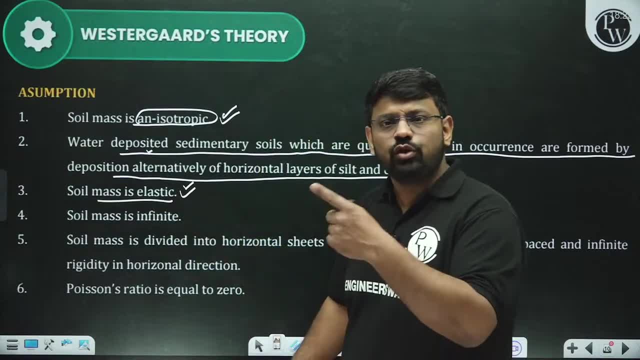 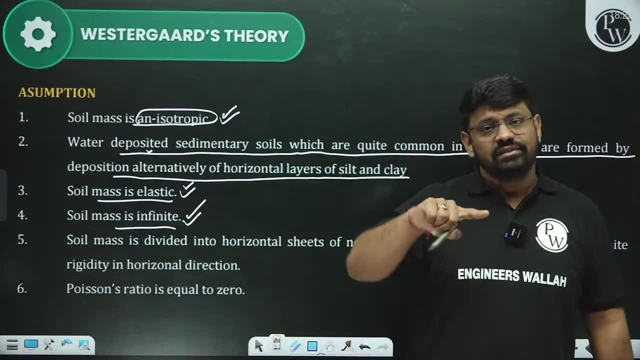 He said, sir soil mass is elastic. He said, sir soil mass is elastic, Elastic soil mass. Okay, sir Soil mass is infinite. Here it is not semi-infinite. He said, sir soil mass is infinite. 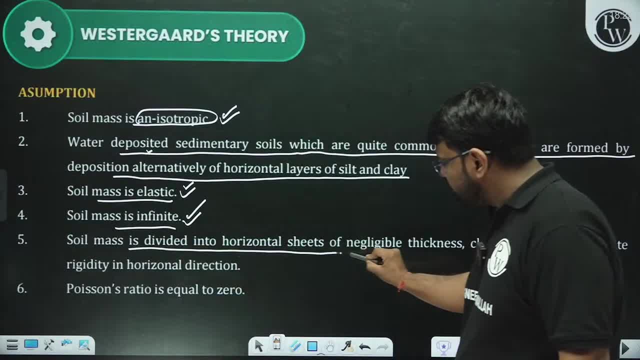 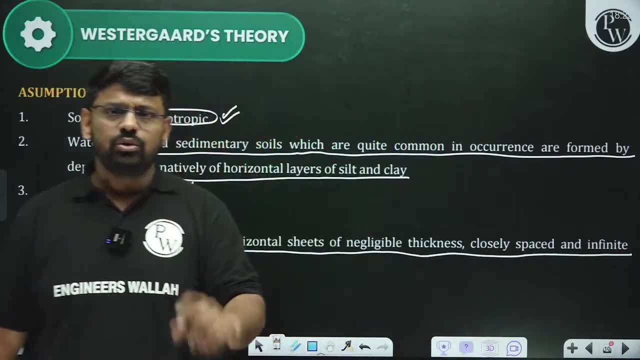 After that, see, soil mass is divided into horizontal sheets of negligible thickness, closely spaced, and infinite rigidity in the horizontal direction. Both of these are fine here because, sir, he said sir, the layer that we have will be in the horizontal direction. 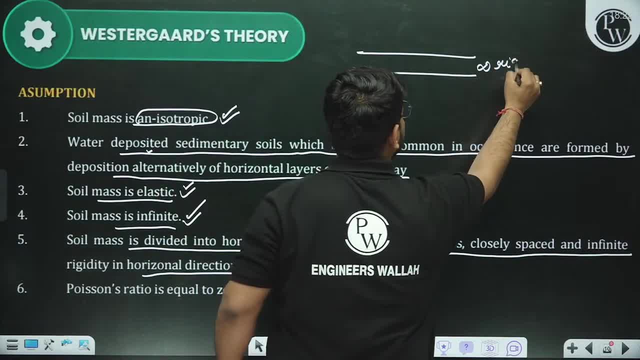 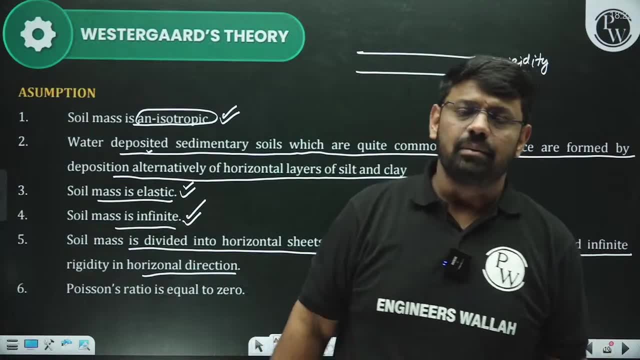 and in the horizontal direction we will get to see infinite rigidity. Sir, what is infinite rigidity? Rigidity means that, sir, you cannot do deformation there, And infinite rigidity means that, sir, there will be zero strain in that direction. 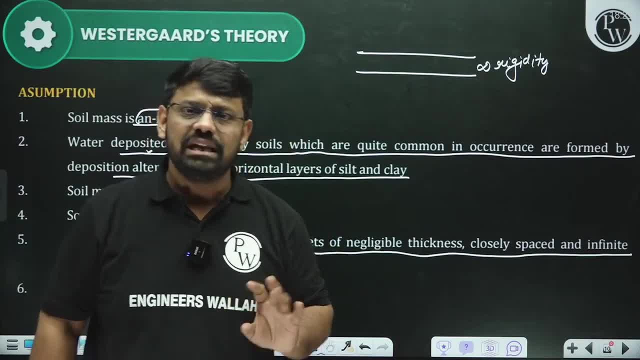 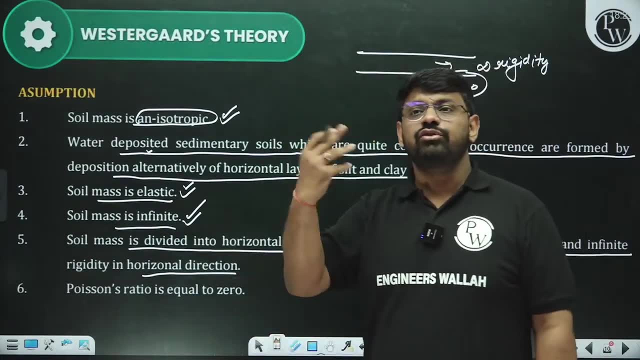 It means that you cannot see any kind of deformation in that direction. It means that, sir, if you see in this direction, then, sir, what strain will we have? Sir, it will be zero. This means the meaning of being infinite rigid. Okay. 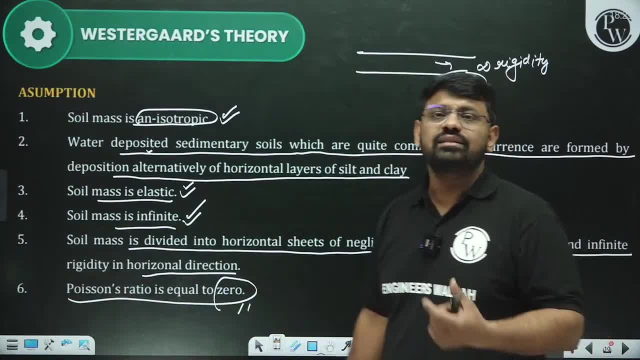 Now look ahead, sir. Poison ratio is equal to zero. That means, sir, the poison ratio is zero. The point is also absolutely correct, sir. When lateral strain is not happening, then where will the poison ratio come from? 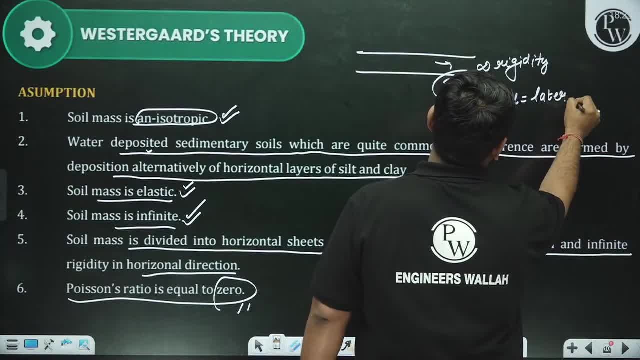 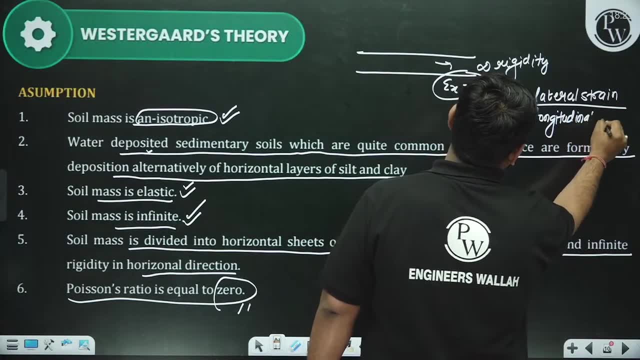 Because you all know that, sir, the poison ratio that we have, that is basically your lateral strain divided by the longitudinal strain. So lateral divided by longitudinal strain is what we have. So if we do not allow this, then what will be equal to mu. 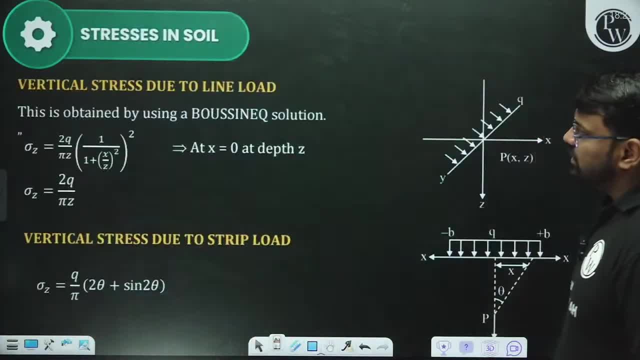 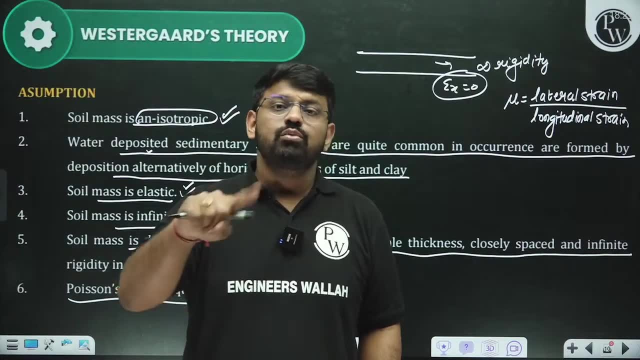 Sir, it will become zero. The soil becomes completely rigid, Mu becomes equal to zero. So we have all these assumptions of Westergaard. So do write in the comments once and tell me which theory is more general, Bosinex or Westergaard. 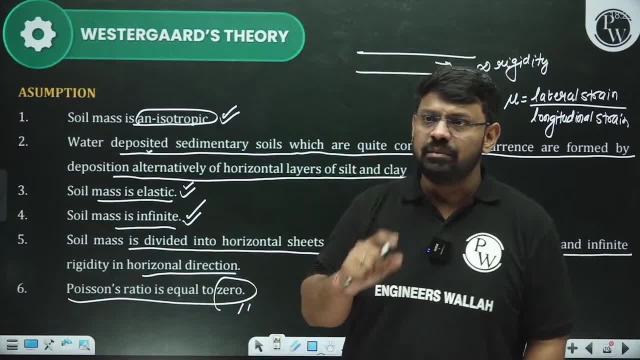 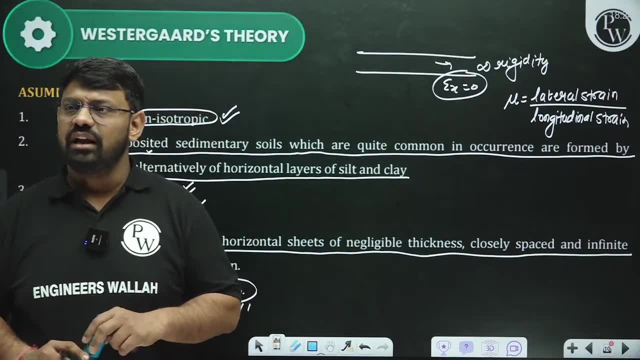 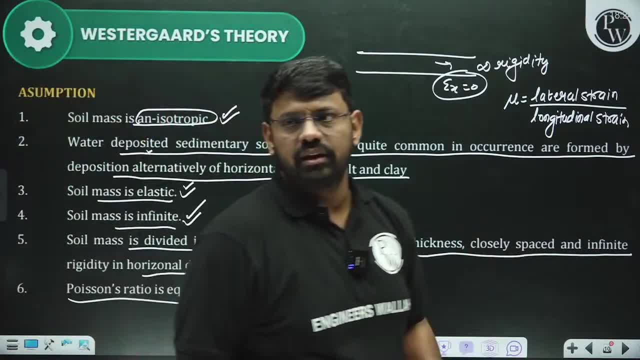 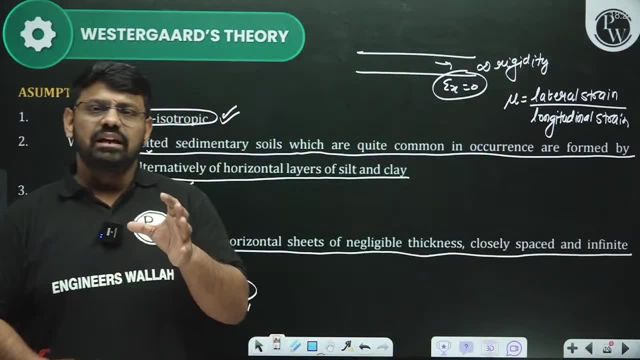 What is anisotropic? A child is asking: sir, what is anisotropic? Look here, what is the meaning of anisotropic? Try to understand carefully. Isotropic means that the properties in every direction are similar. okay, I told you about anisotropic yesterday also. 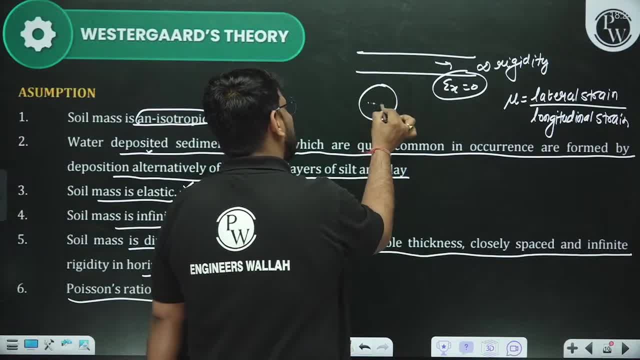 I told you about anisotropic yesterday also. For example, this is soil. Now, if you go in the direction of x, let's assume that I have assumed a property as permeability, So this is permeability. and if you look in the direction of x, 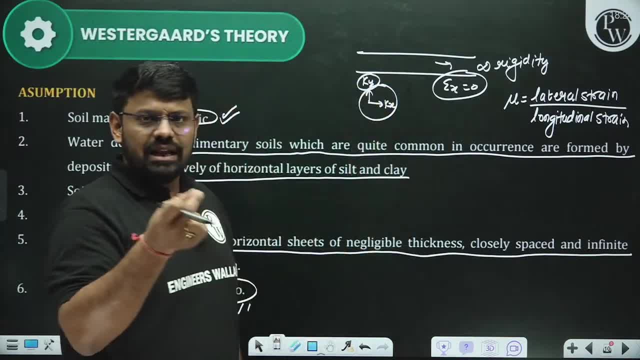 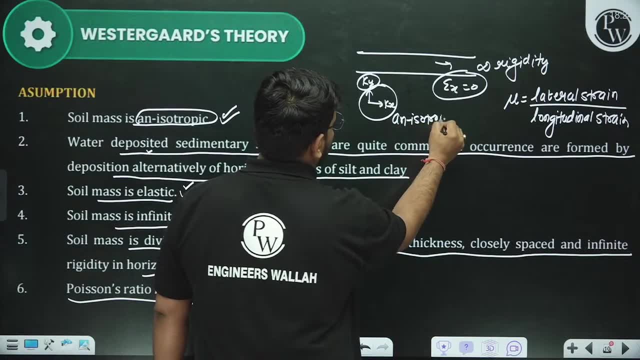 it is kx, and if you look in the direction of y it is ky. So in different directions the permeability is different. This means: how did this happen to you? This soil is anisotropic. The properties are not the same. 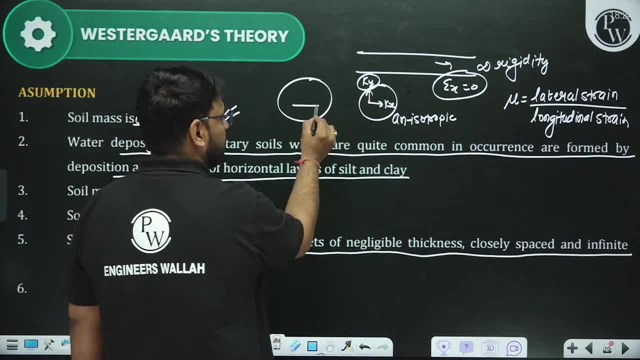 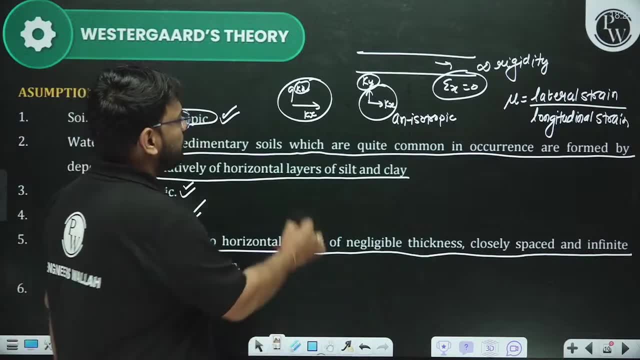 If this soil is isotropic, then, if I am taking an example of this, okay, If I took permeability, then this would also be kx, sir, And this would also be kx. Both would be equal. Both would be equal. 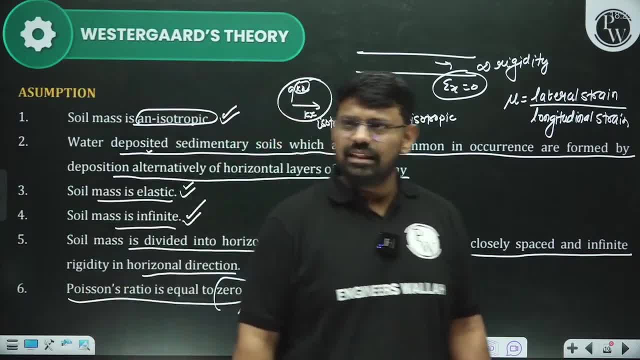 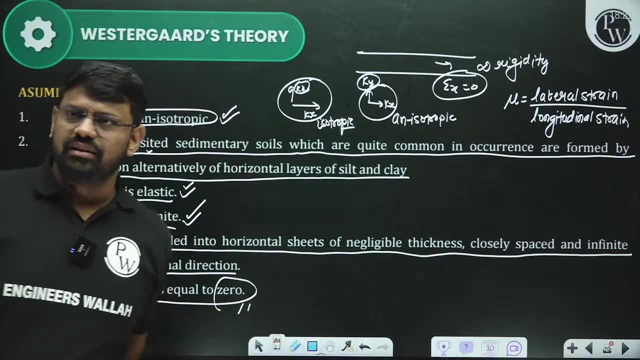 This kind of soil is called anisotropic soil. Is it clear? Is it clear It is isotropic. Okay, sir, Very good, Westergaard, Westergaard, Westergaard, Westergaard is everywhere. It is very clear, sir. 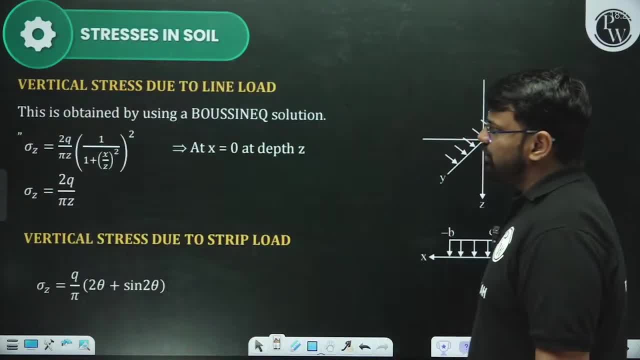 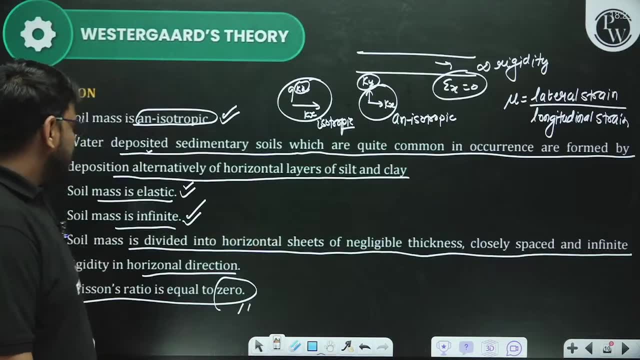 Now look here, If I talk about vertical stress due to a line load, Look when we talk about vertical stress due to a line load and before that, understand. one more point. Okay, Sir, here we have a Westergaard influence factor. 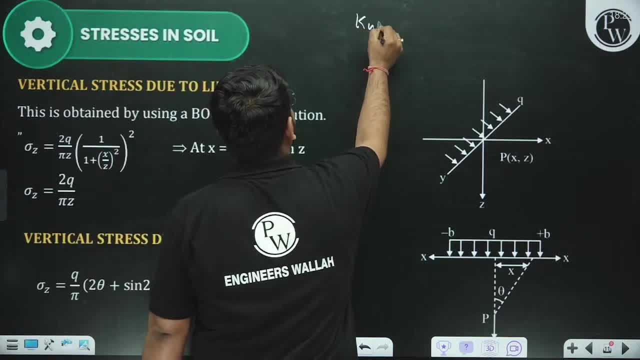 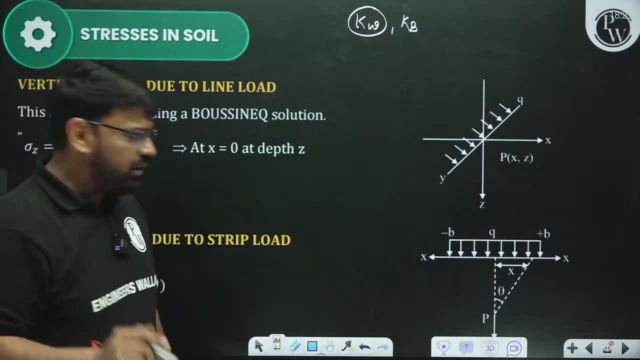 which is known as your Kw. Okay, So Kw is the Westergaard influence factor And Kb, which we have, is the Bosinex influence factor. Okay, Both are the same. Now, here means both of you have the influence factor. 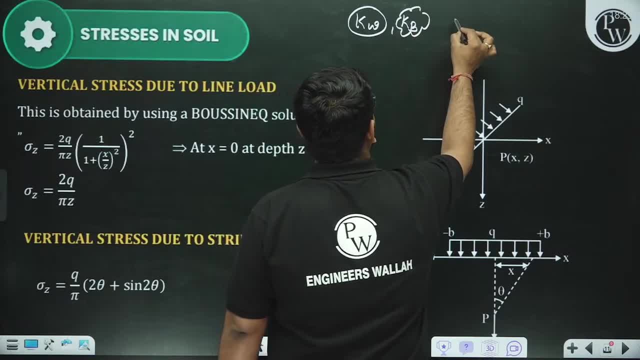 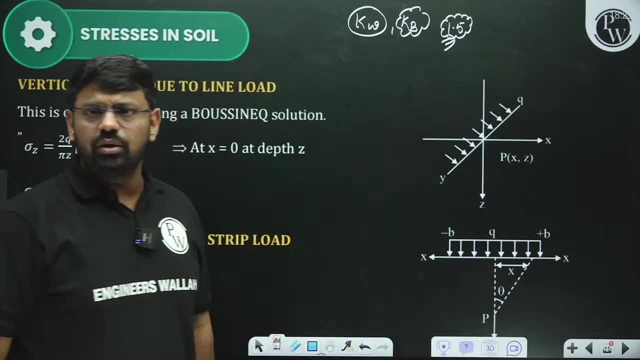 Both of these factors are the same when the value you get is 1.5.. When their ratio is 1.5, then both of them are equal. When the value of r by z is 1.5, then both of them are the same. 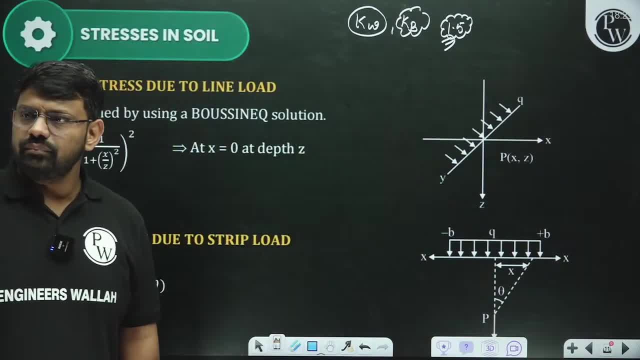 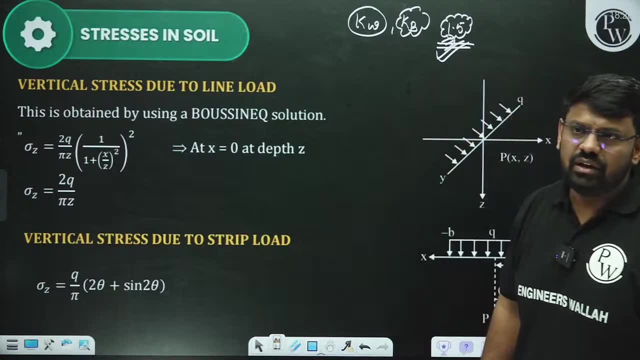 Is it clear? Is it clear: When the value of r by z is 1.5, then both of them are the same. So sometimes this question is asked to you: When will both be the same When the value of r by z is 1.5,? 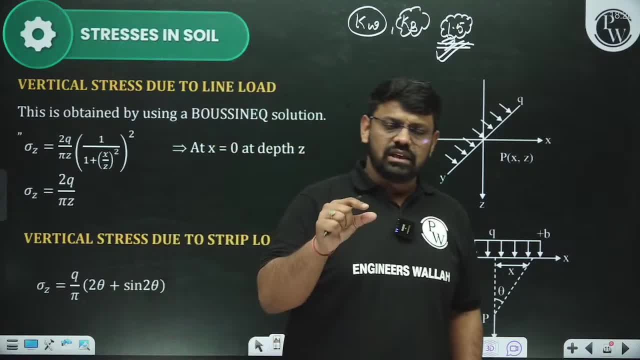 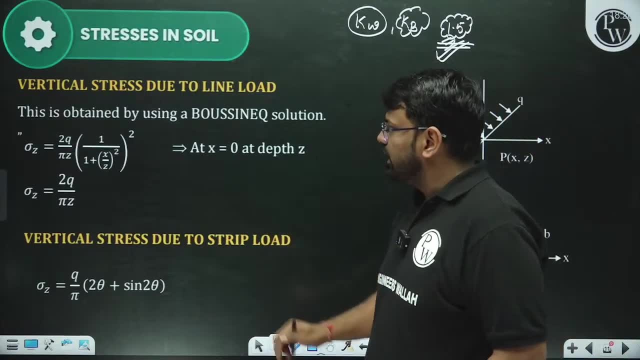 then both of them are the same. So this is a small point that you have to remember Now, sir. in different, different, different types of loading conditions, how will stresses be generated? How will stresses be generated? We will talk about that. 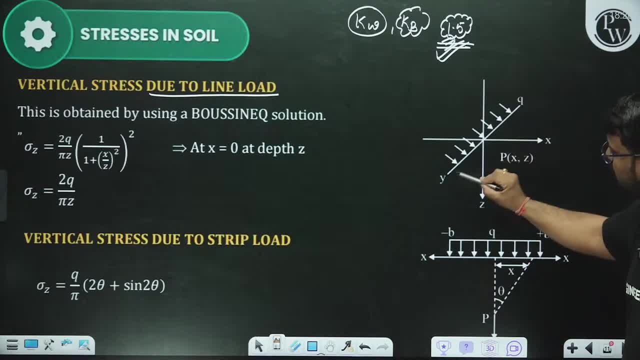 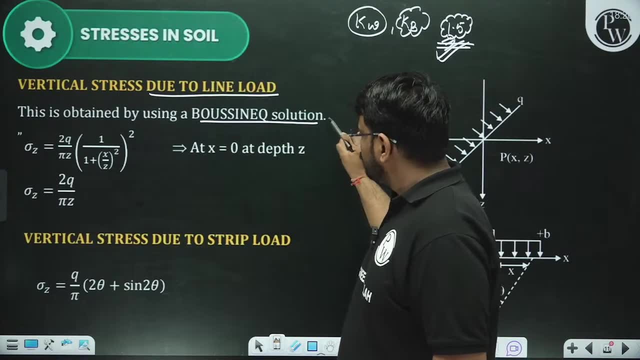 First of all, sir, vertical stress due to a line load. What does line load mean? This is the complete line load that we have here. So how will you obtain this? Using the Bosinex solution. So we obtain using the Bosinex solution. 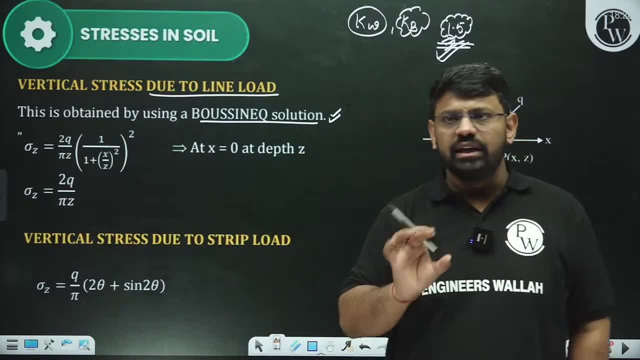 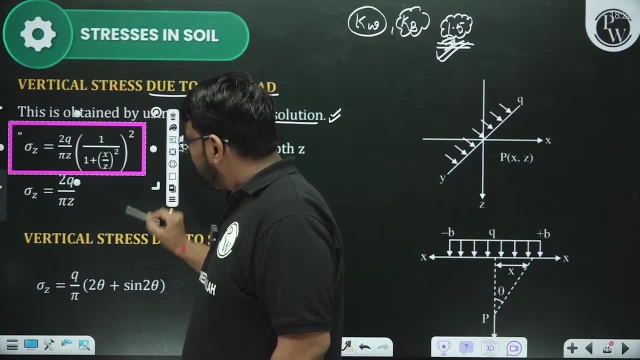 What do you have to do here? Here you just have to look at the formulas. So the first thing we have is that if you look at the formula here, then sigma z equal to 2q pi z. sigma z equal to 2q pi z. 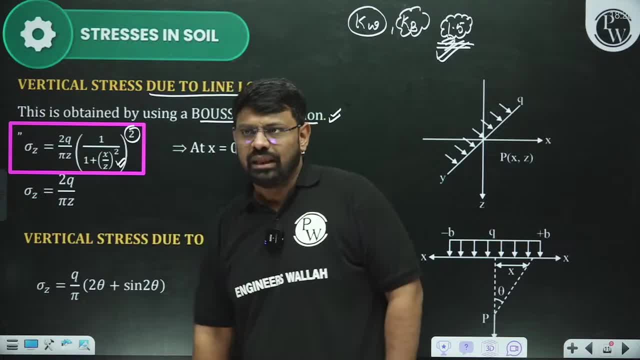 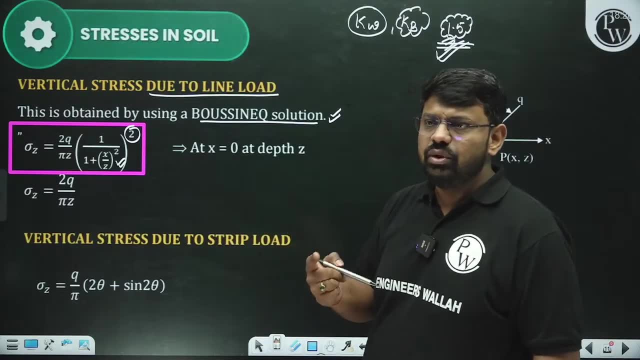 1 upon 1 plus x by z, square, whole square, x by z square, whole square. this is what you have, But what will you be asked in the exam when it comes to line load? what will you be asked in the exam? In the exam, you are asked, sir. 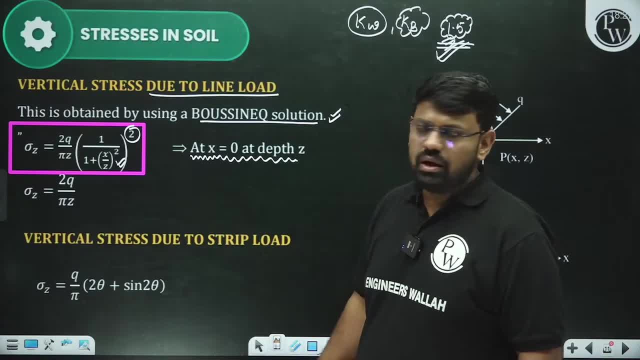 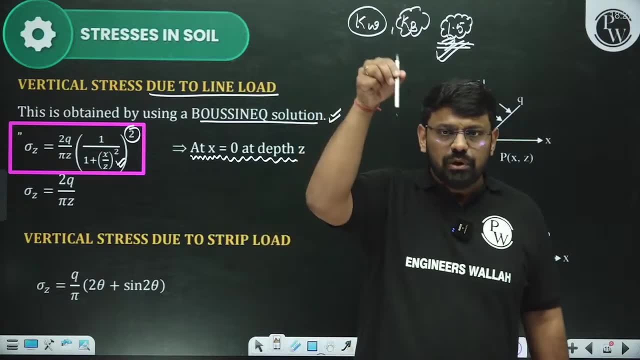 when x equal to 0 happens, then what will be the depth? That is, when x equal to 0 happens, then this formula becomes 0.. This whole term is removed from you, So we ask you that. just below the load. 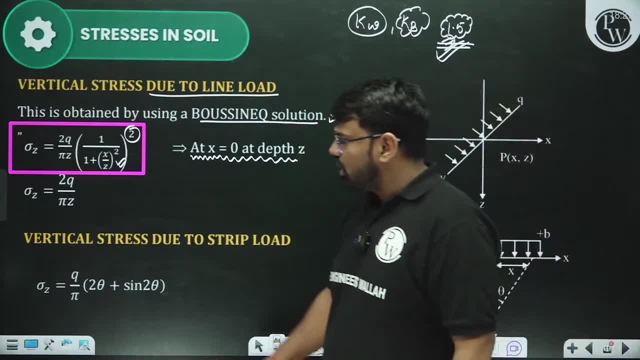 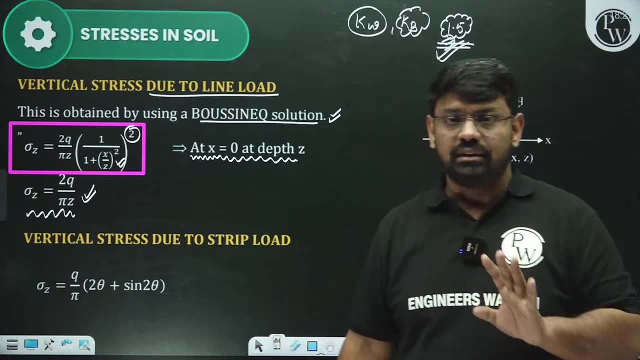 just below the load tell us how much stress will be developed. So from there you have to remember this formula: 2q upon pi z. If we talk about line load, then this formula is also remembered to us in a very good way. 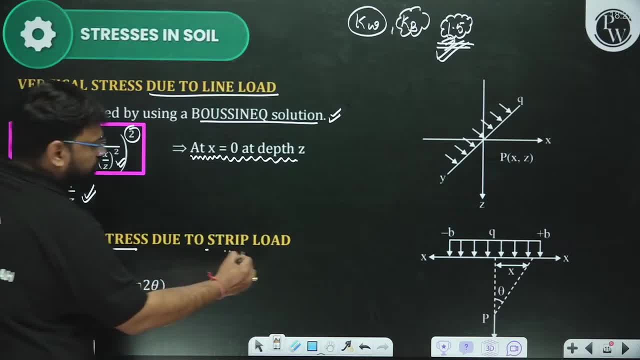 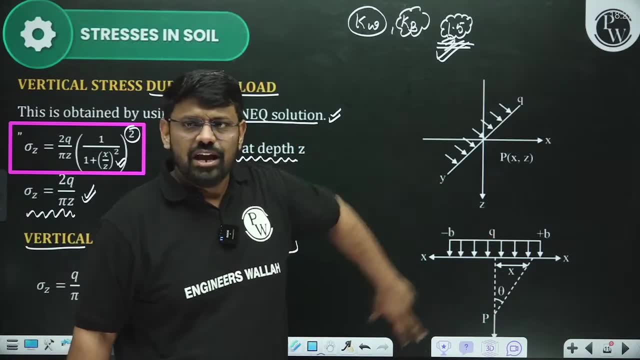 Similarly, sir, vertical stress due to strip load. So, sir, we have this type of line load. If I talk about strip load, then there will be a small strip in the strip load. A small strip means from minus b to plus b. 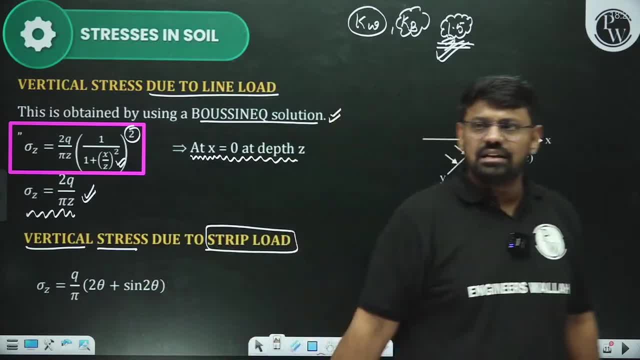 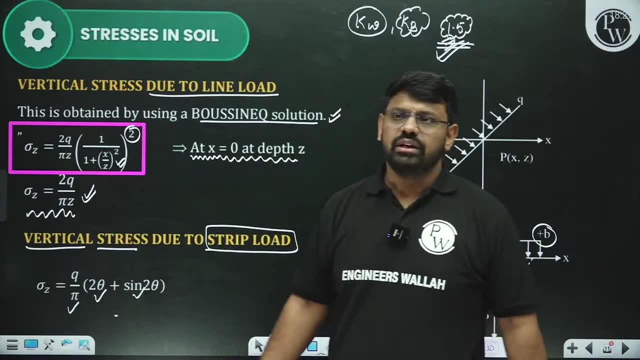 this much load is being applied to you Now because of this. how much vertical stress will you get? That will be q upon 2 pi 2 theta plus 2 pi 2 theta. The question has never come from this, but you just have to remember this formula. 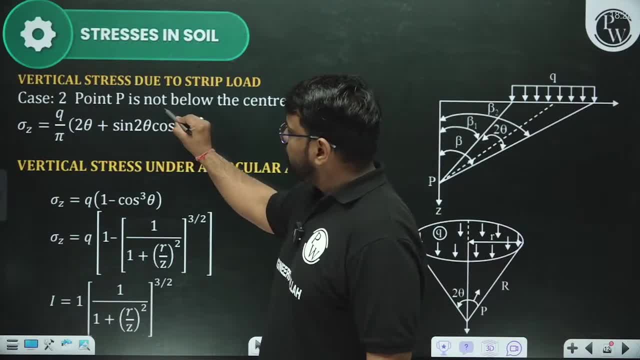 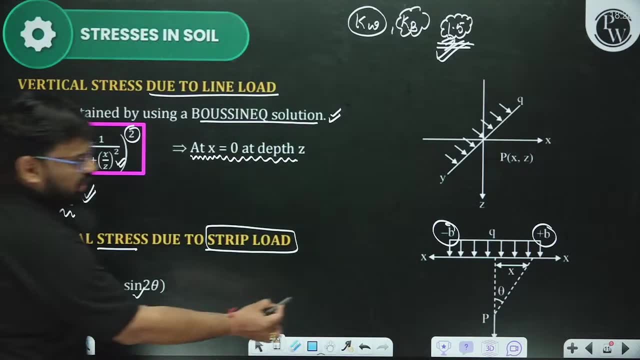 Look at the next point, sir. If we have case 2, when point P is not below the center of the strip, Look, we have this formula. This formula is valid when what is happening to you, Look, this strip is from minus b to b. 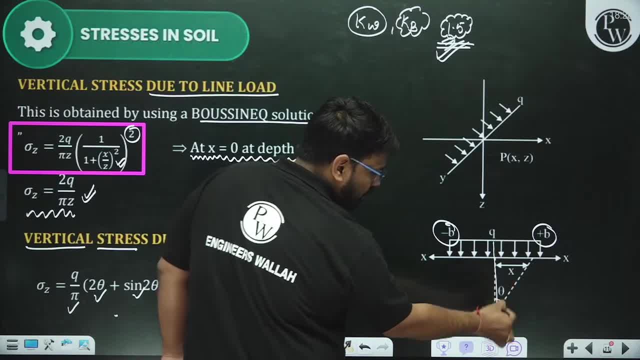 So we have taken a point below its center, So we took a point below the center of the strip. When we took a point below the center of the strip, then we got sigma z like this: So when will this happen to you? 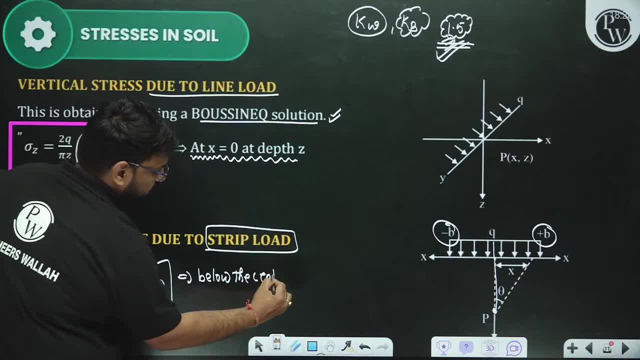 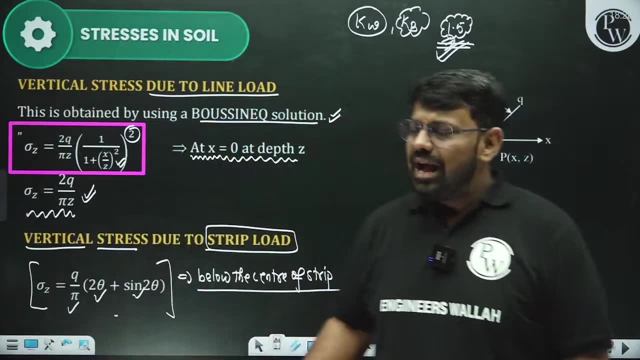 When it is below the center of the strip. When it is below the center of the strip. So when it comes below the center of the strip, then we call this formula x If it is not below the center. like, look here: 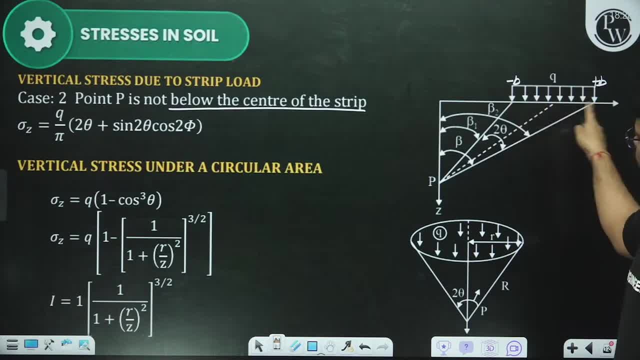 The strip load is here. So this is minus b to plus b. Now its center is here. This time the point is not here. This time the point is somewhere here, So it is away from the center. So the formula changes here. 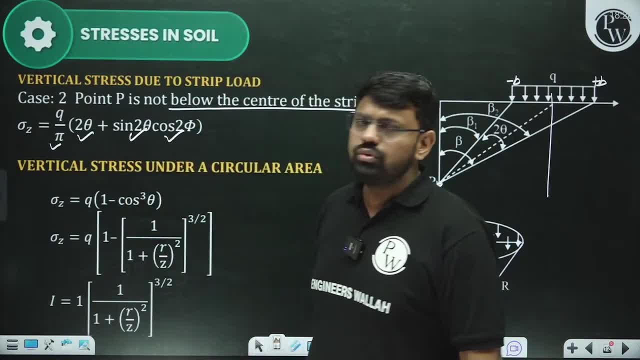 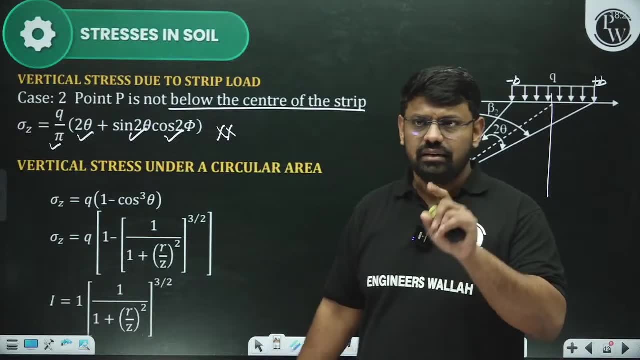 So it becomes q by pi 2 theta plus sin 2 theta cos 2 phi. This is the formula you have here, This formula also, you don't have to remember. Ok, You don't have to remember. Ok, I am just asking you to write it down. 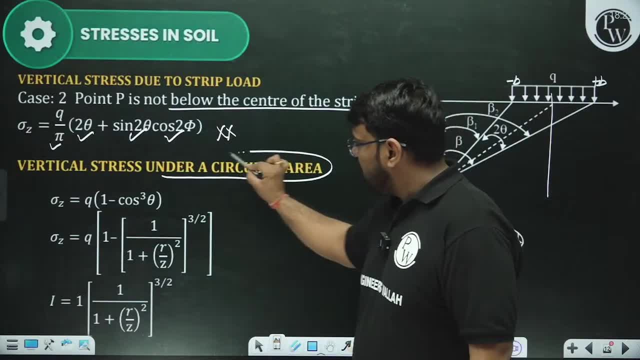 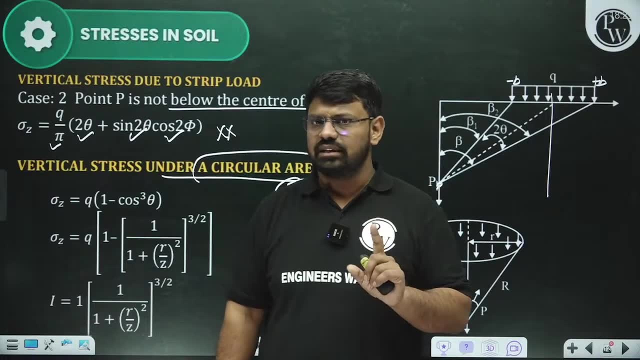 Now look ahead, Sir. vertical stress under the circular area. Yes, Ok, You have to remember this formula. This is important. Ok, What will you remember in this? Just remember a small relation in this And the question will be 100% in the exam. 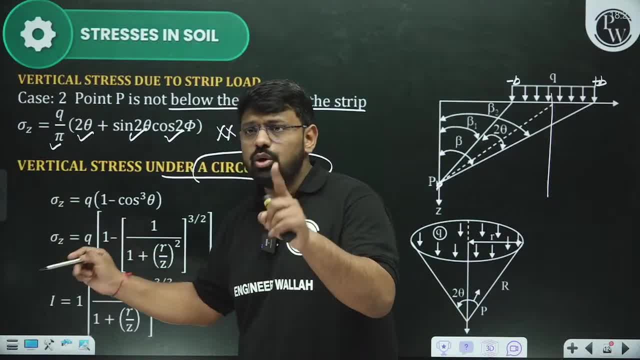 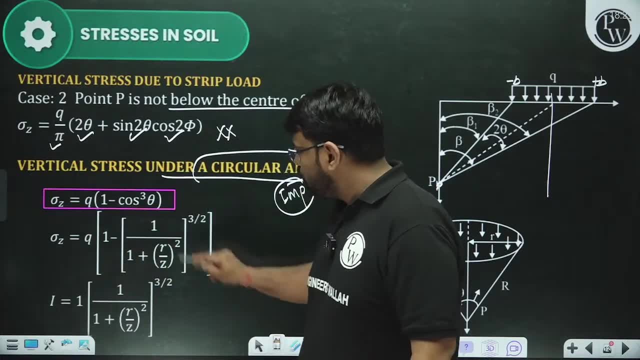 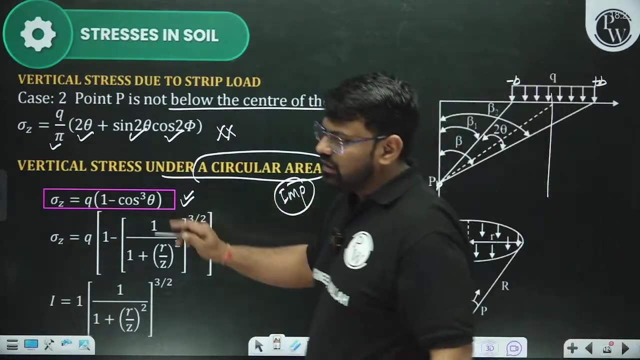 If it is asked. Look, You have to remember this. The stress caused by this is q multiplied by 1 minus cos 2 theta. You have to remember this formula. That is ok. Ok, You have to remember this formula: q into 1 minus cos 2 theta. 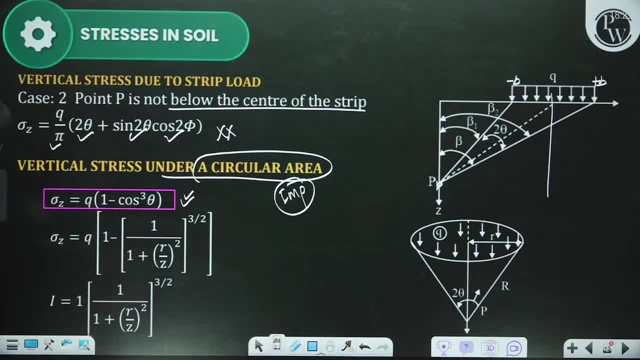 From here, your question will be solved. Ok, From here, your question will be solved. Ok, sir. When does this work? sir, When we have this circular loading, You have to remember this formula. Sometimes it is possible to ask the formula directly. Ok. 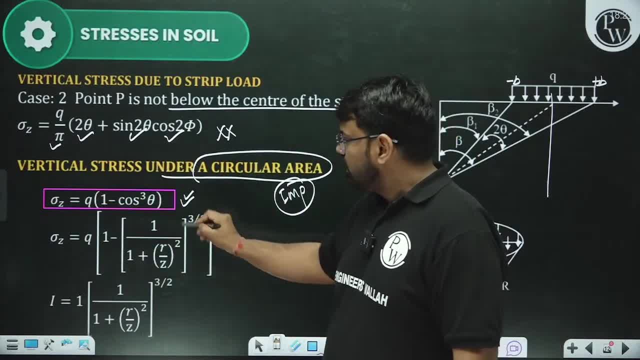 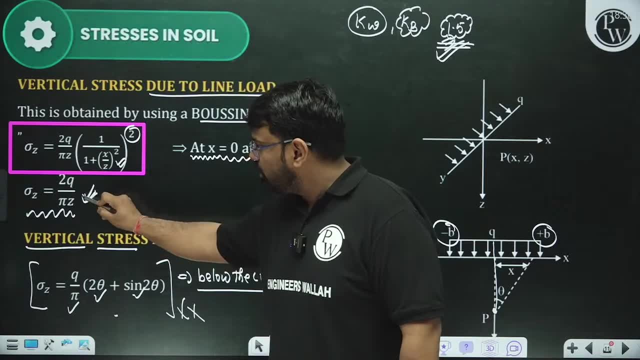 So just remember the formula that I have told you, Sir. you have to remember this one. You don't have to remember this one. You don't have to remember this one either. Ok, Remember the one below, You don't have to remember the one above. 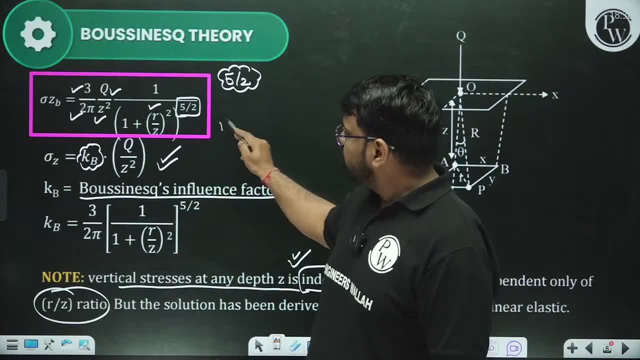 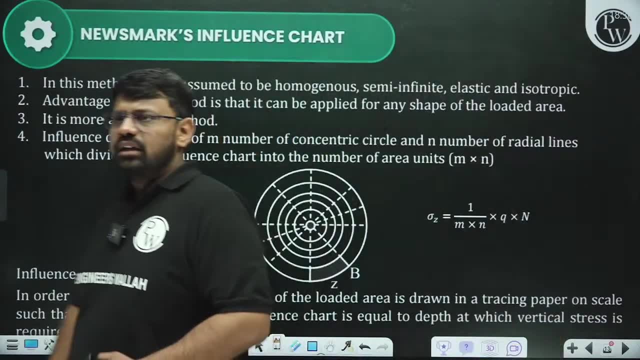 And, apart from this, remember this value. Before that, you have to remember the whole bosin x. Ok, You don't have to leave the bosin x, Ok, sir. Now look, sir, The most important part of this chapter. 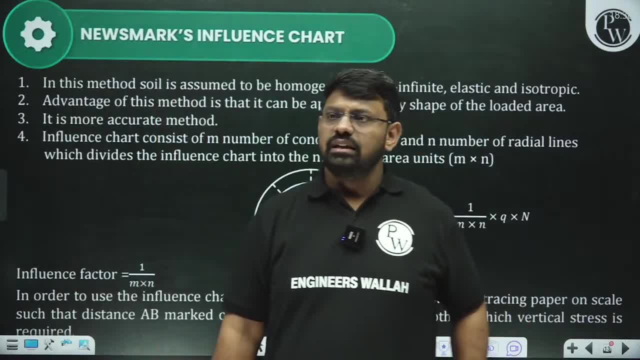 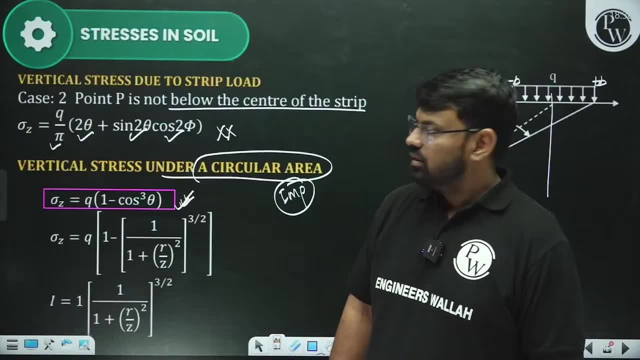 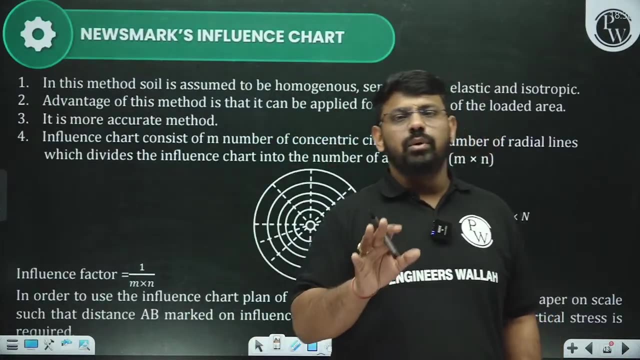 Sir, don't remember the small one, Remember the big one. Yes, Only q and q square Here. Here. This is q into 1 minus cos 2 theta. Ok, Now come forward, Sir, the most important point that we have. 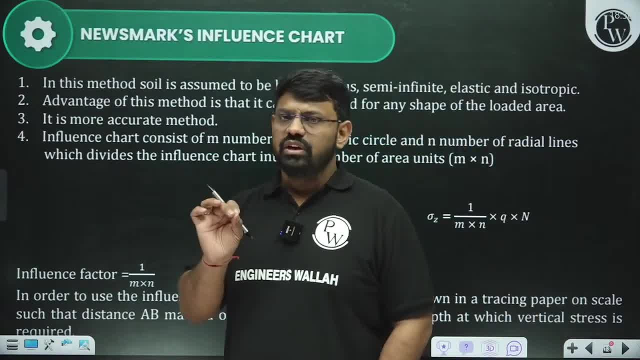 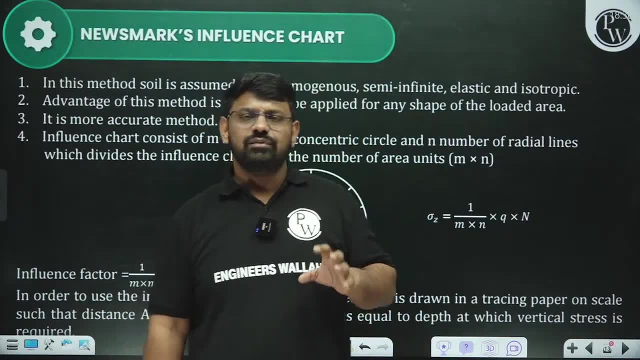 is the Newmark's influence chart, And from here you will definitely get to see the theoretical question. Understand one thing here: When we have vertical stress distribution, then for any kind of shape of area, for any kind of shape of area, 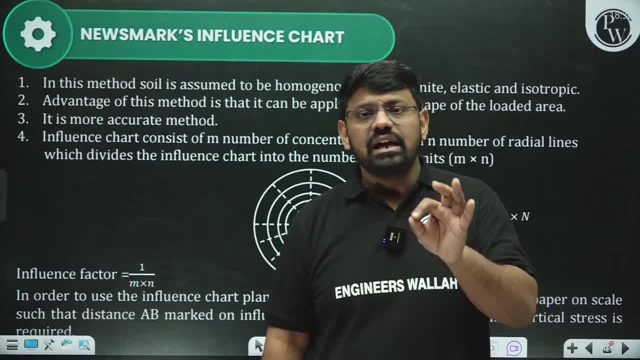 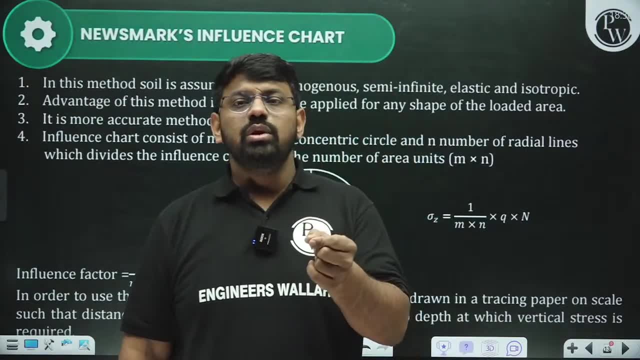 or for any kind of loading, we have a graphical representation, And for that graphical representation, which is dependent on the theory of bosin x, we call it Newmark's influence chart. Now, how is the Newmark's influence chart basically made? 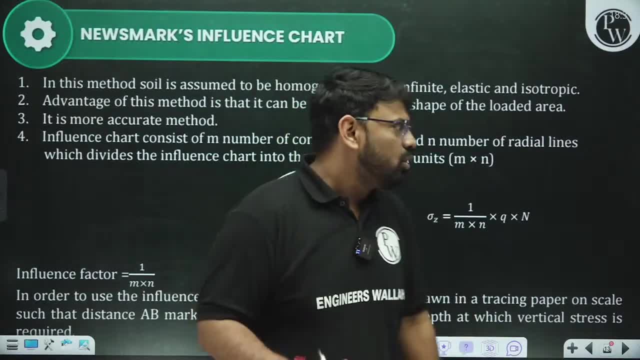 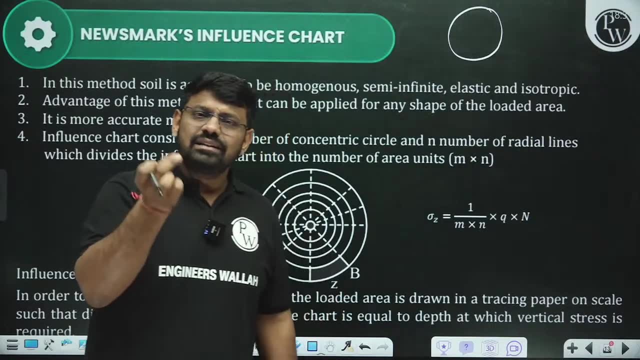 It is basically made by a concentrated line. That means, if you see, here there are concentric lines, So you have these concentric lines Con-centric. Con-centric means that it has one center, a single center. Ok, So here, single center. 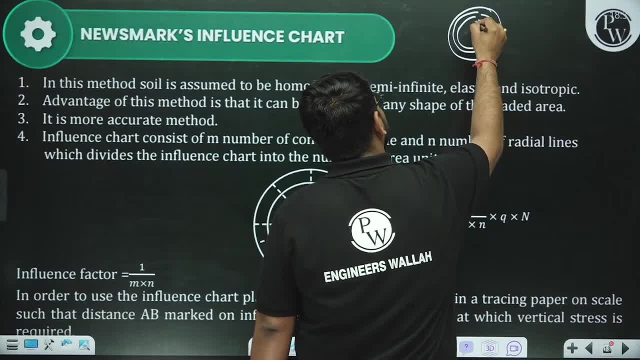 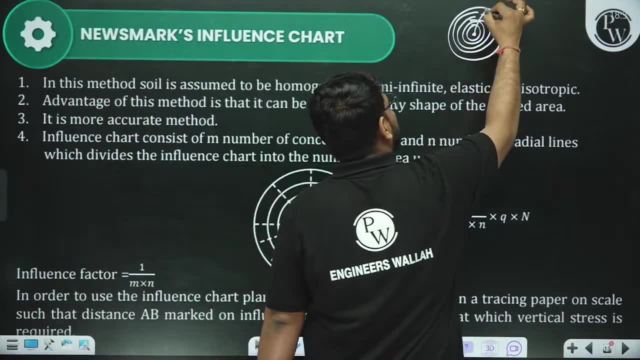 and on this single center all these circles are made. So you have these concentric circles. So, sir, we have concentric circles. First thing, sir, concentric circles. Second thing, we have radial lines. So you will have all these radial lines. 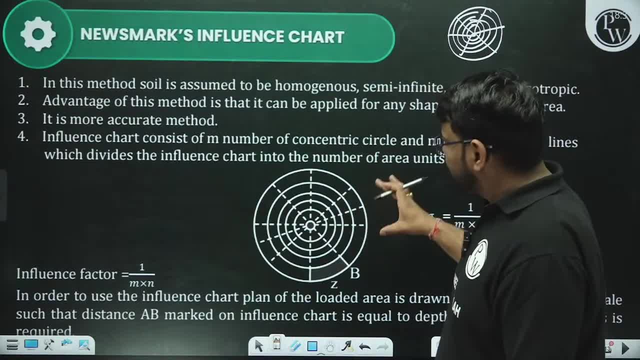 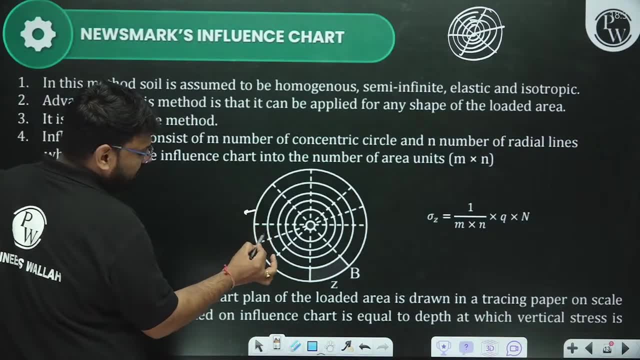 So, like timber, the internal structure of timber, you get to see the same structure in a way. Ok, So here tell me, sir, when you have these concentric circles and these radial lines, how do we use them? 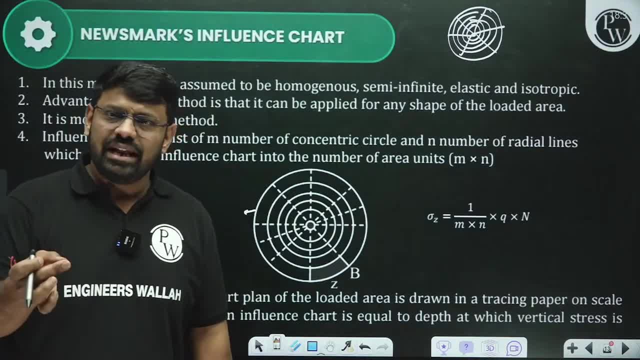 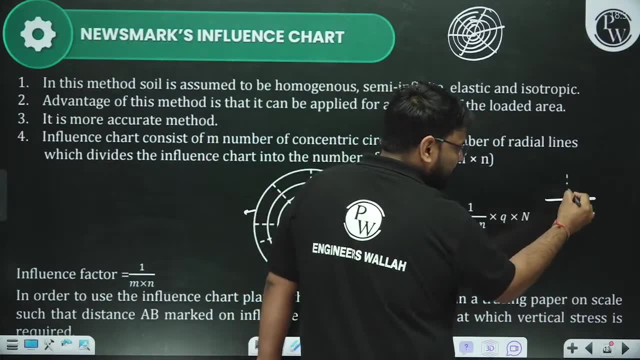 See, this is a graphical representation. And what are we doing with this, sir? What we are doing with this is that, sir, we have, for example, ground, Sir, this is for example ground, Vertical force is applied on it. 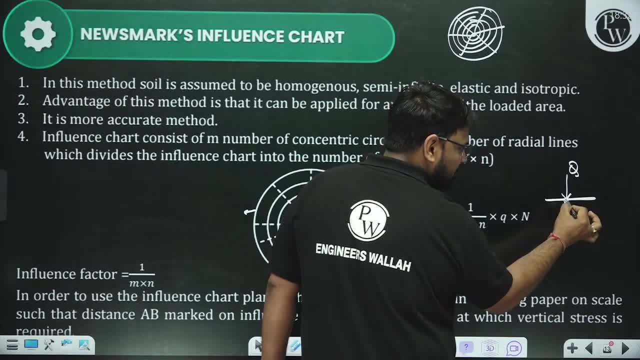 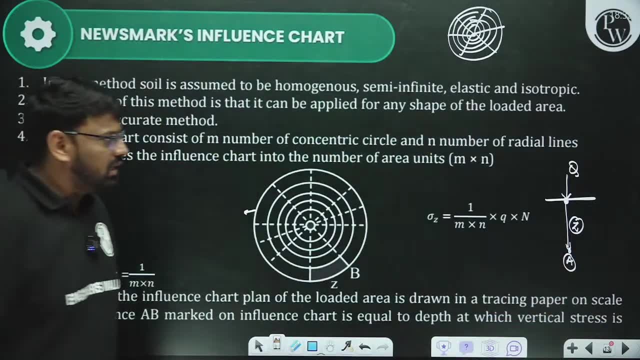 Ok, And why is this load applied? I have to remove stress on a particular Z depth on this particular point. I have to remove depth on this particular point. So I mean, sir A and B, let's assume this point. 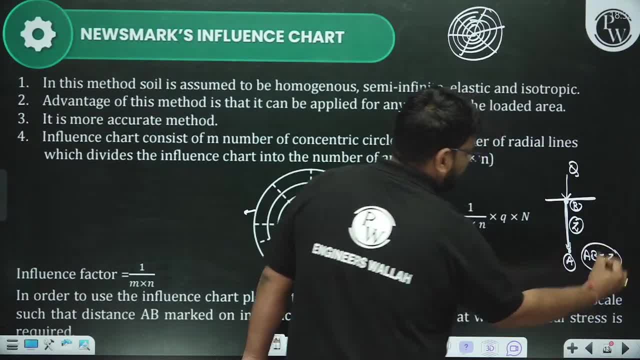 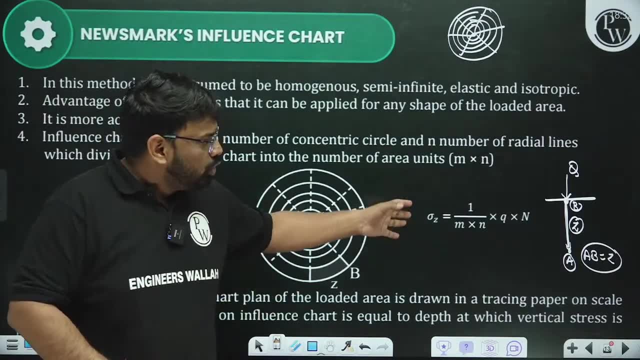 So I have AB depth. Ok, This is equal to Z, This is our depth, And this is the point. So what will you do? You will take the stress distribution chart of that particular area, sir, and you will place it. 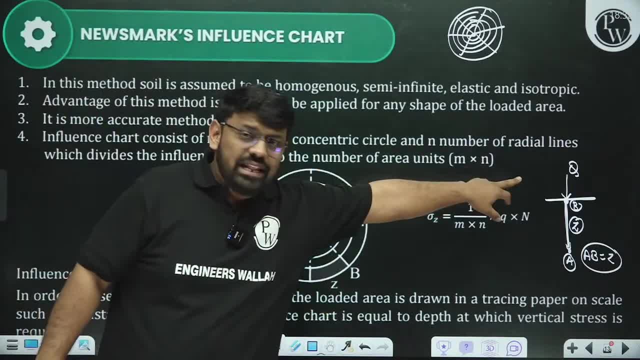 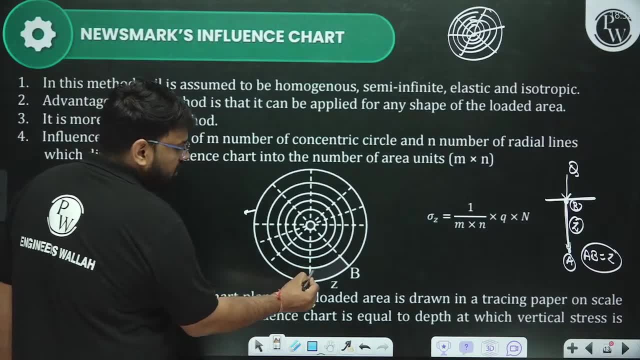 on the Newmark's influence chart. So this point, the vertical one, you will place this point on its center And the depth that you are getting you have to match that depth here. For example, this is point A, this is point B. 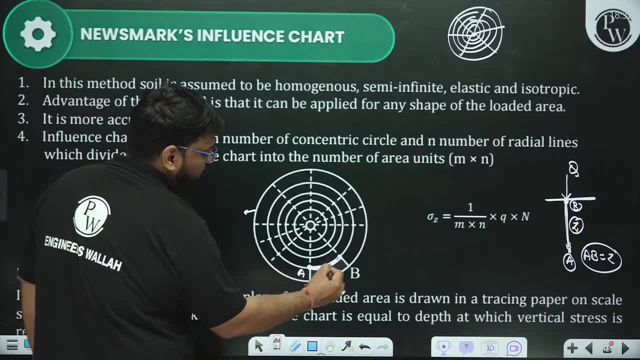 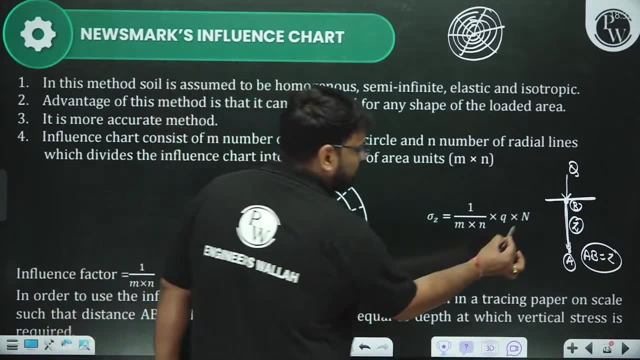 So you will match this line of depth here. the radial distance On the concentric circle, So the area that it will acquire. here we call that area, sir N Ok. So number of equivalent areas, So the area. 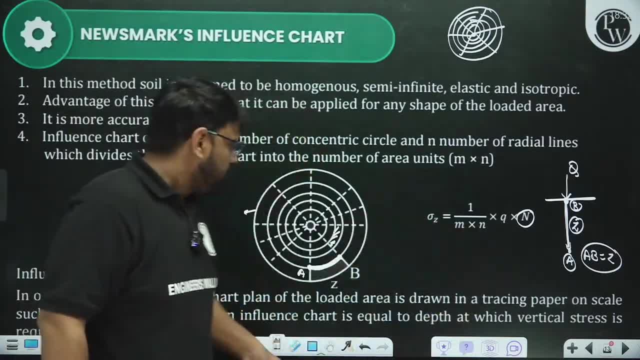 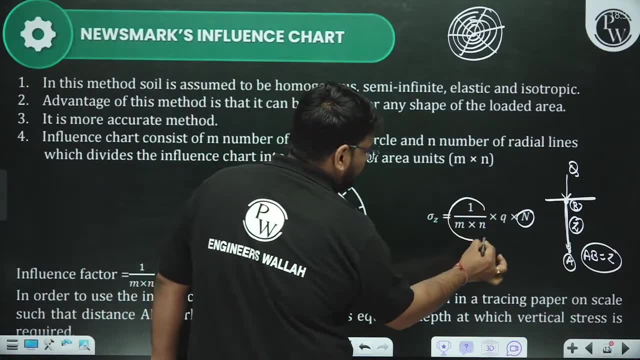 that it covered. you have the number of equivalent areas- Q is the force- And at the same time you have 1 upon M by N. This is your influence factor developed here. With this we take out a formula And with this formula we calculate. 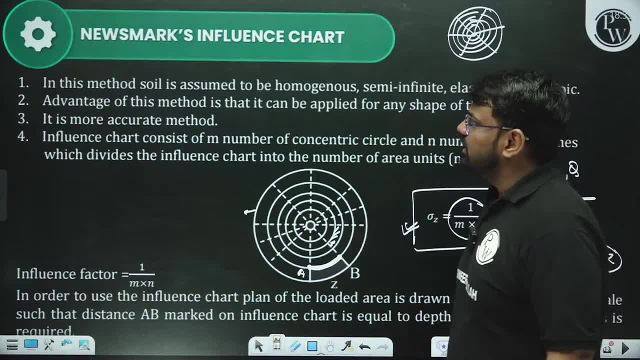 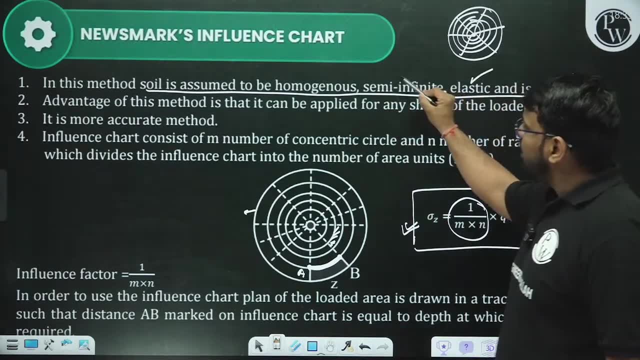 the vertical stress. So look, sir, In this method soil is assumed to be homogeneous, semi-infinite, elastic and isotropic. These four things you have to consider as soil For the first time. What is M and N? 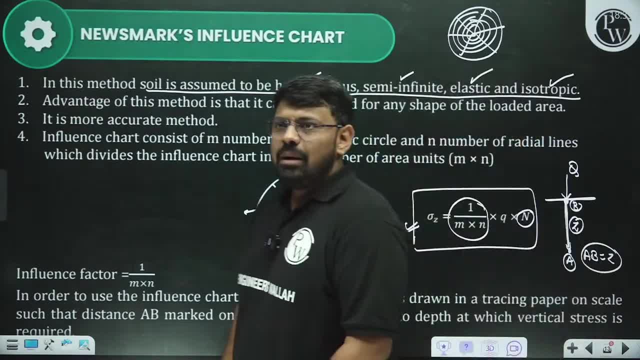 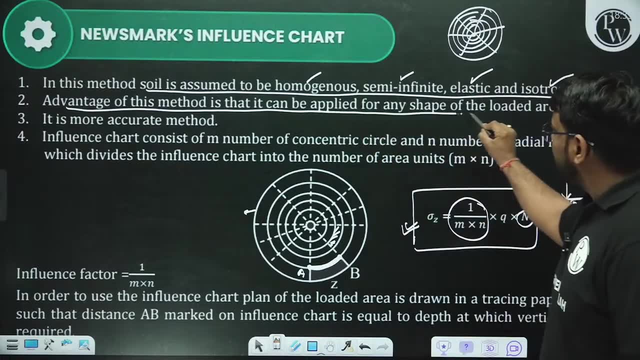 Now let's tell its study. Now look ahead. Ok. Advantage of this method is that it can be applied for any shape. So the second thing that you have to keep in mind, sir, is that this particular chart is applicable. 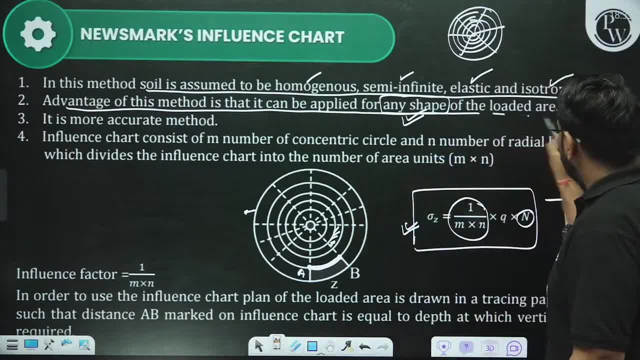 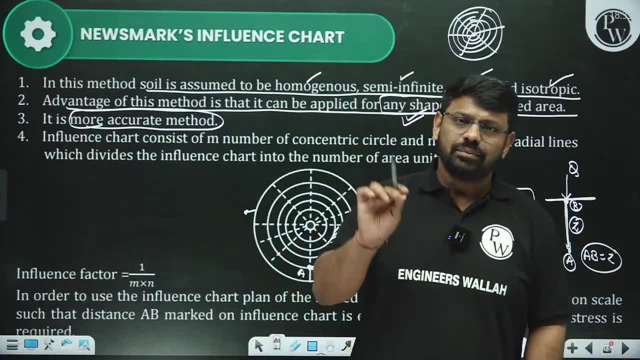 for any type of shape of loading- This is also remembered, sir- Offloaded area. Look ahead, It is more accurate method. Absolutely, This method of yours is the best accurate. Ok, The best accurate method, or the best method is the best accurate method. 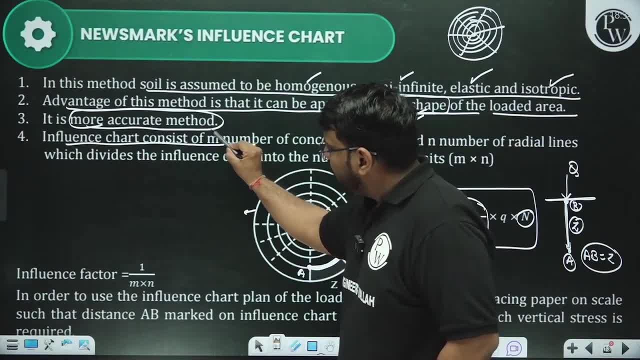 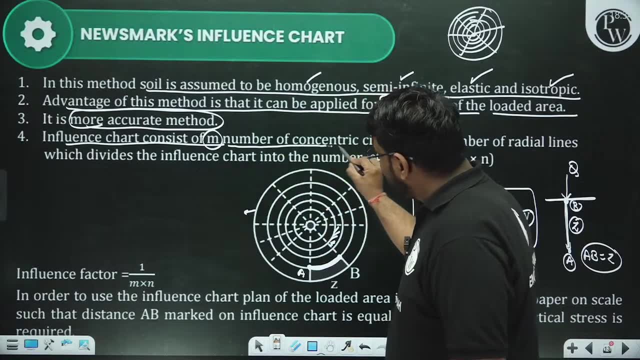 Look ahead, sir. If I am talking about influence chart, then M The M that we have. The child asked: sir, what is M and N? Ok, What is M and N? So we have M, sir. Number of concentric circle. 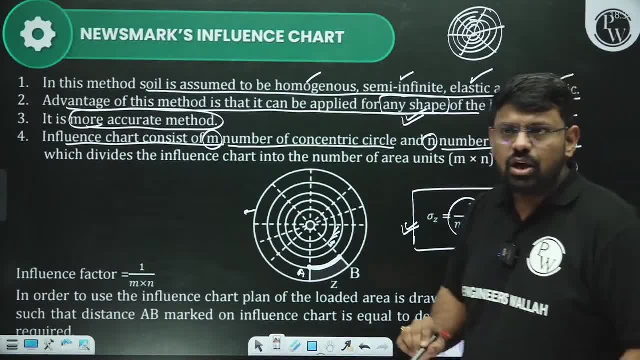 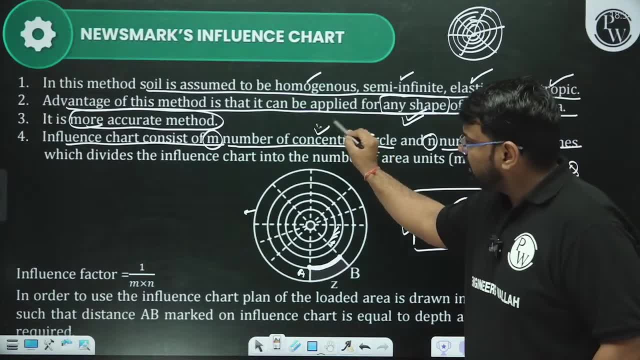 And, sir, we have N Number of radial line. Ok, So number of concentric circle and number of radial line, We understood both of these things, sir. So you have number of concentric circles, Means look one, two. 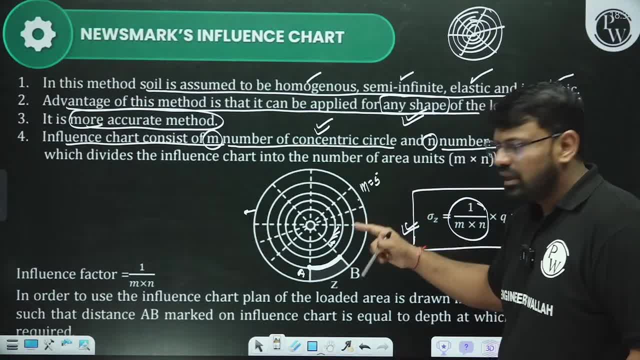 three, four, five. So here the value of M is five. Concentric circle is formed. Concentric circle is formed Similarly, N is your radial line. Means one, two, three, four, five, six. 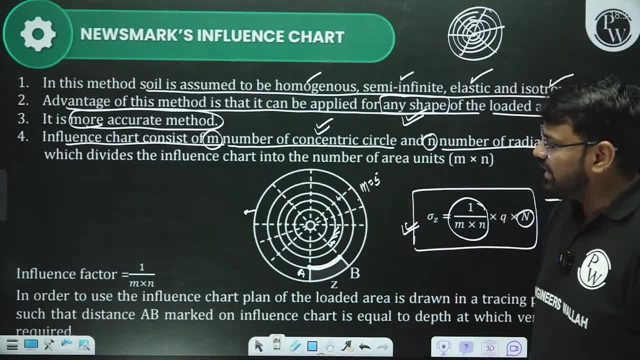 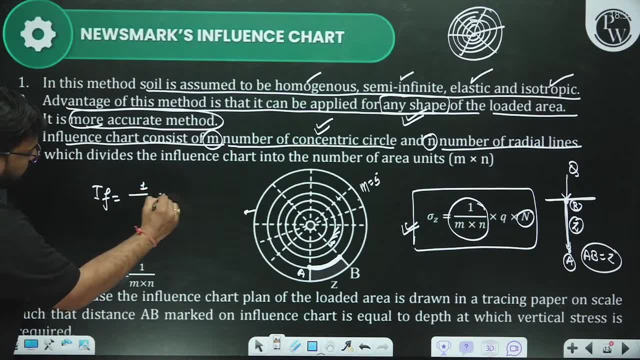 seven, eight, nine, ten, Whatever is given to you, That much radial line you will have. So the influence factor that we will have, So, sir, the influence factor that we take out, we take out one upon M multiply by N. So this too. 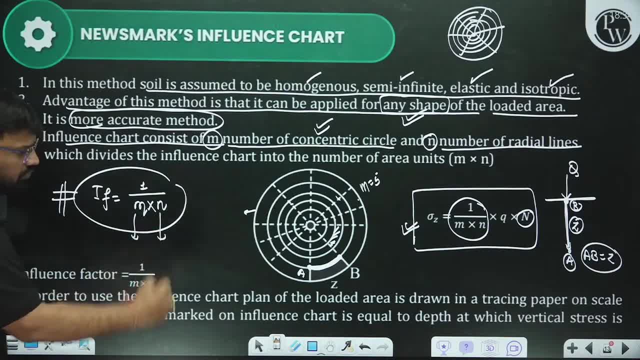 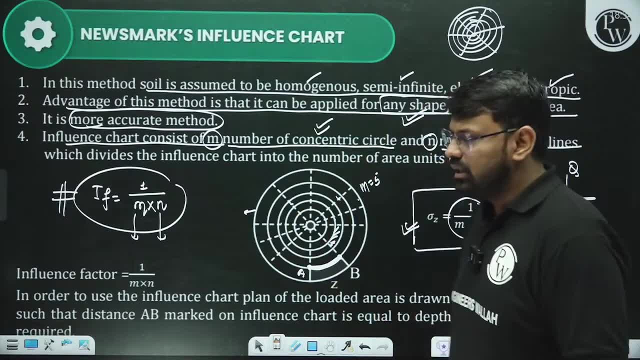 can be asked in the exam: M: concentric circle, N, number of radial line And concentric circle and radial line. both will be given to you in the exam. Ok, Both will be given to you in the exam. It is clear, sir. Now look ahead. 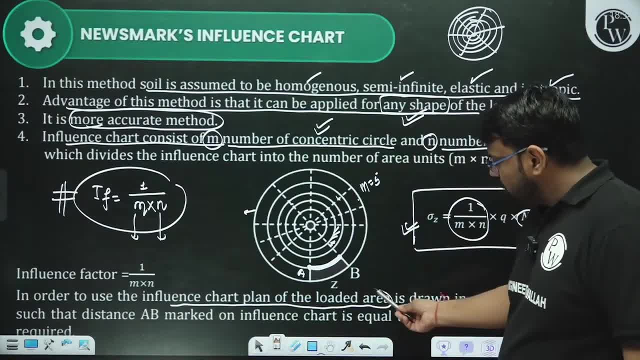 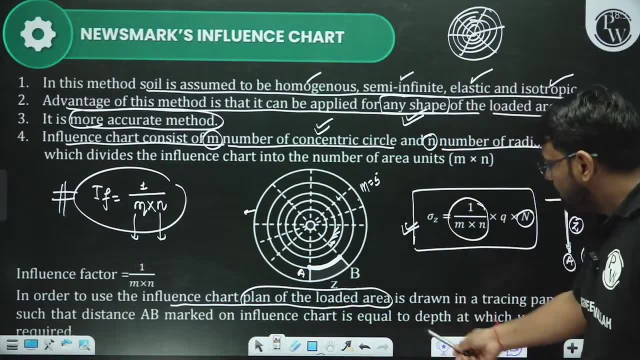 In order to use the influence chart. what did you do? Plan of the loaded area In the area where your loading is done in the ground, the loaded area that we are getting to see. what will we bring? We will bring a plan of that. It is clear. 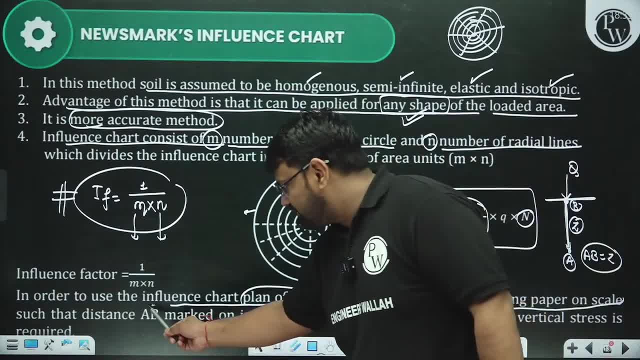 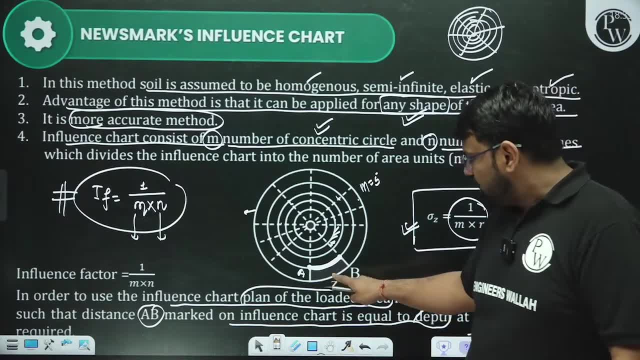 It is drawn in a tracing paper and on a scale such that distance AB which we have, is marked on the influence chart equal to depth at which vertical stress is calculated. So the distance here. you will keep the depth of that plan here. 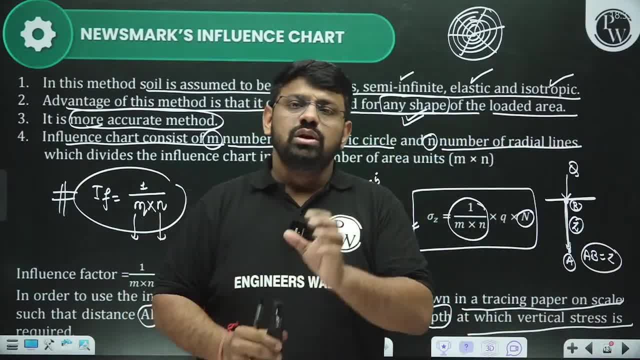 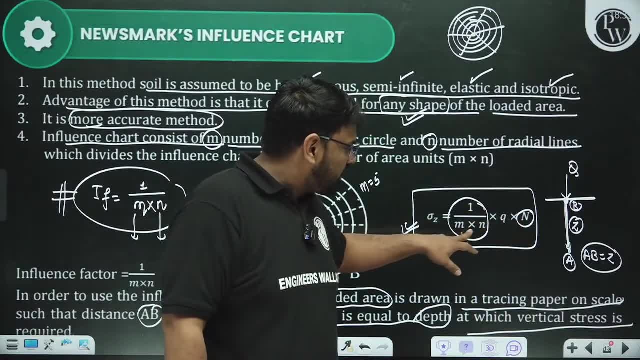 How much area is being influenced by that? So you take out the number of equivalent areas. How much was covered in your plan? So, sir, here comes N. This is the influence factor. This is Q. So much vertical stress. 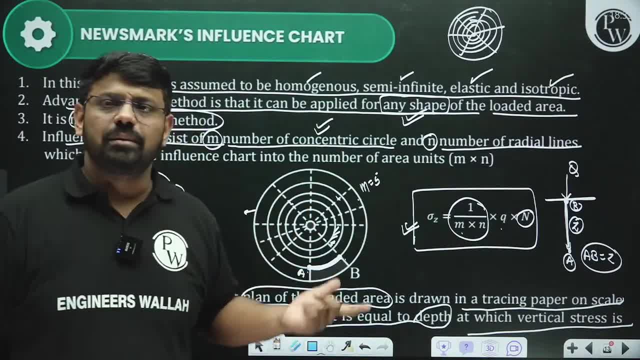 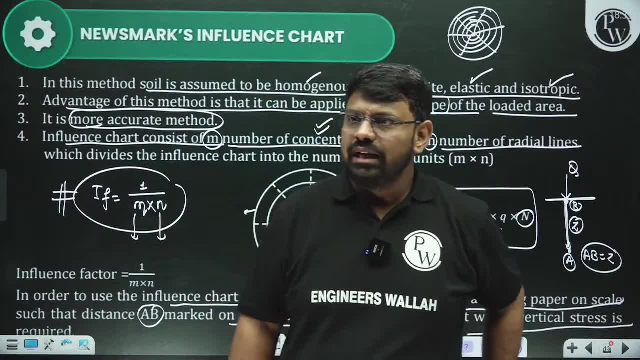 what do we have? So much vertical stress is taken out, Sir. from whom did it come out? It came out from your Newmark's influence chart. It is absolutely right. It is absolutely clear, sir. It is absolutely clear. That means, that means. 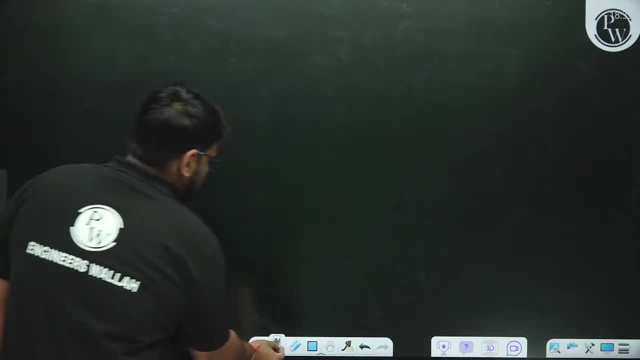 if you see here, that means, sir, if you see here, then you have to keep one thing in mind, sir. You have to keep one thing in mind, sir. If I talk about the Newmark's influence chart, then in this: 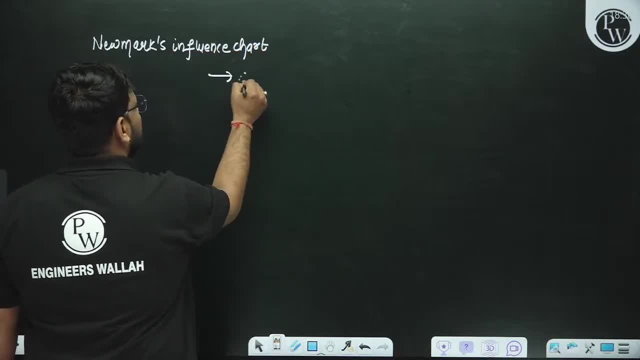 you have to keep two or three things in mind. The first thing, sir, is any shape. It is useful for any shape, The loaded area. The second thing, sir, we have is that it is more accurate. It is a more accurate method, sir. 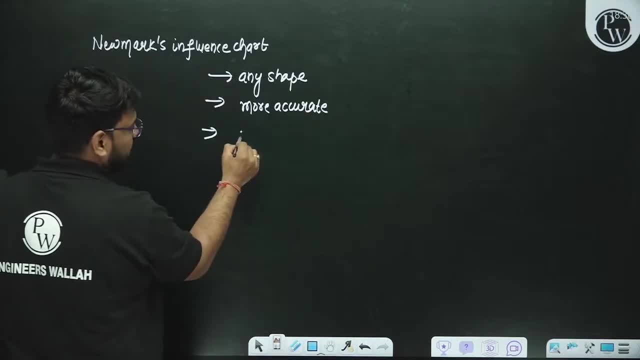 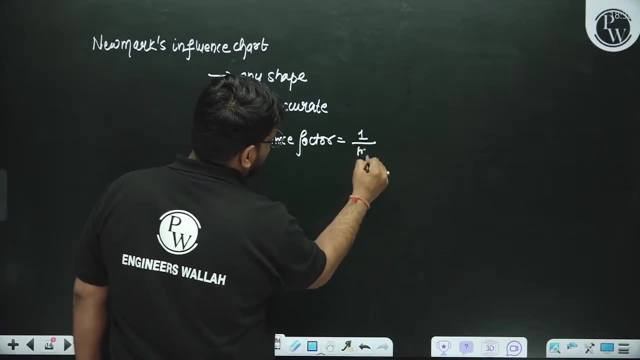 It is a more accurate method. The third formula to remember is of the influence factor. So, sir, we remember the formula of the influence factor in a very good way: 1 upon M into N. Sir, what did we have? You have the number of. 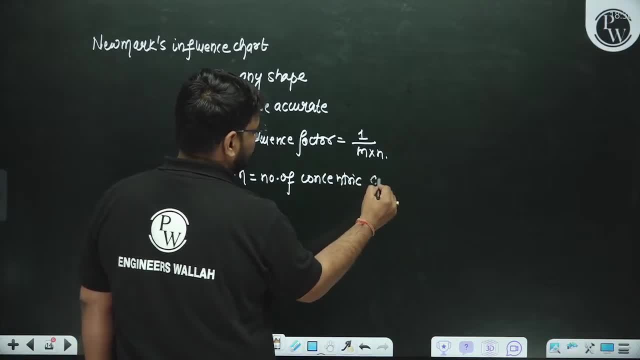 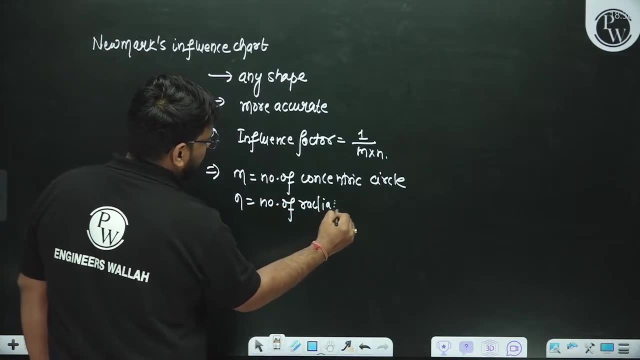 concentric Concentric means the same center, So concentric circle. And N, sir, we have the number of number of radial lines. So these are the number of radial lines. Similarly, sir, N, you have capital N. 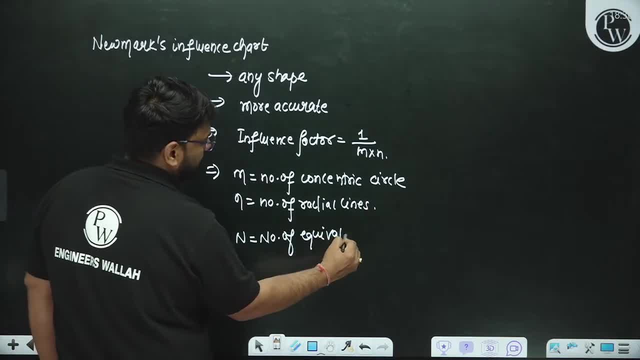 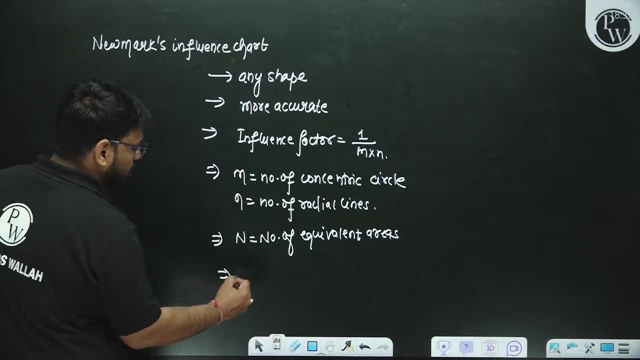 That number of equivalent areas, right, So the number of equivalent areas which are covered on it, which are covered on the chart. we have that. So from here we calculate the stress at any particular depth, that 1 upon M into N. 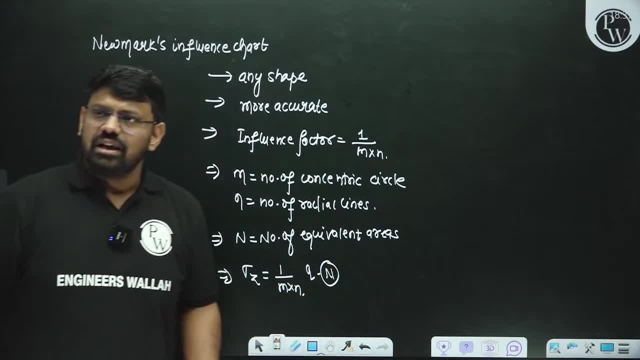 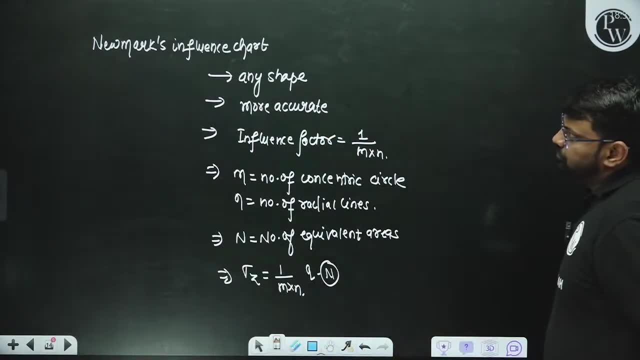 Q multiplied by N, You can generate this much stress here. It is a very simple thing, sir. It is a very simple thing, sir. Now look ahead, sir. What is happening Now look ahead, sir. The Newmark's influence chart. 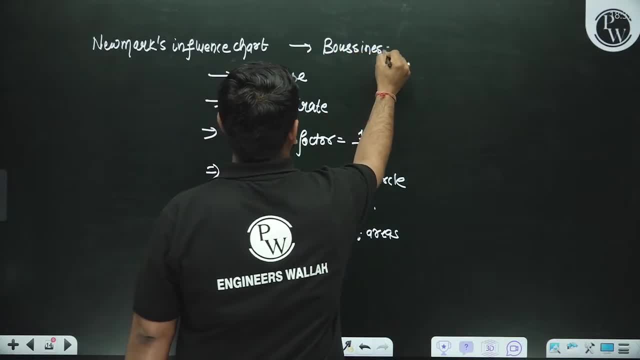 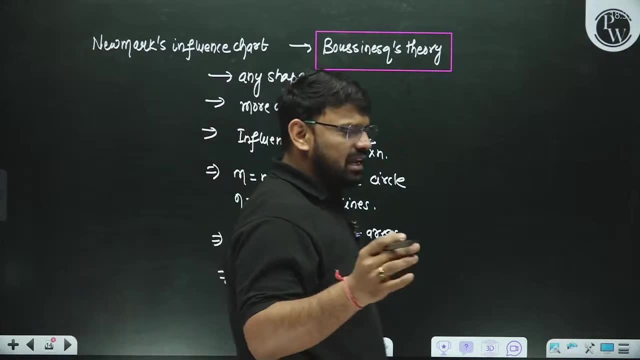 keep in mind, sir, that it depends on the theory of Boise-Nex. It depends on the theory of Boise-Nex. This is the first thing. So, just like this, just like this, we have another chart. Just like this, we have another graphical representation. 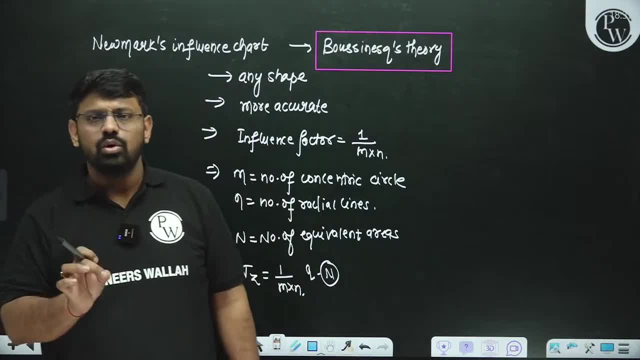 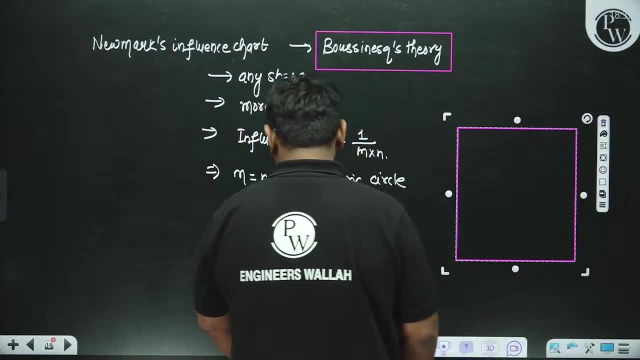 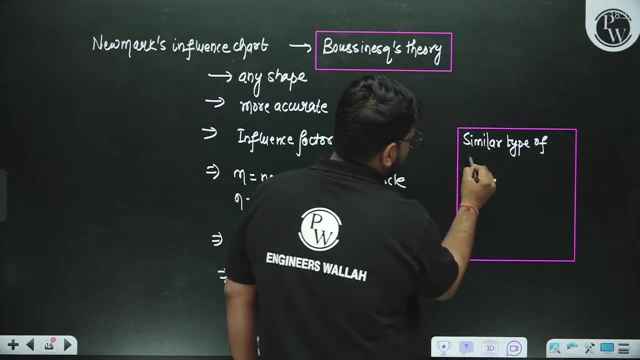 That is the Fenske's chart. Just remember the name: Fenske's chart is, which depends on the Westergaard theory, Right, Which depends on the Westergaard theory. So look, similar, similar type of similar type of. 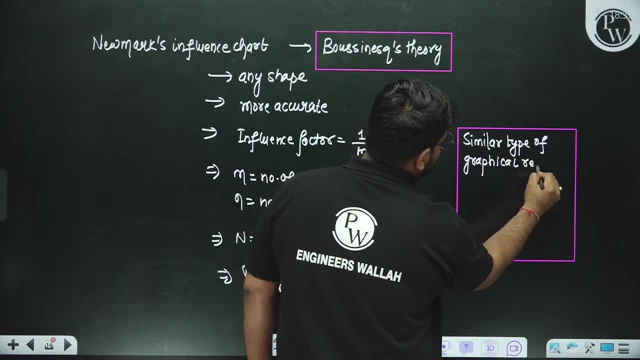 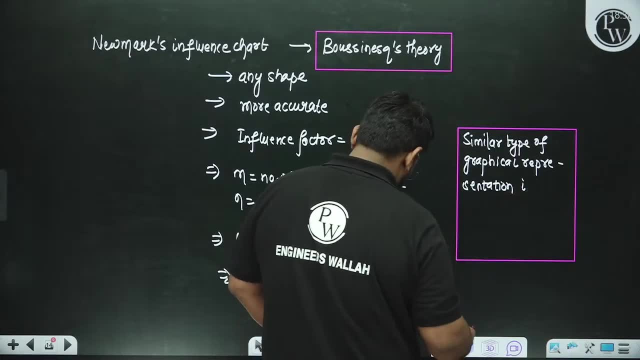 graphical representation. similar type of graphical graphical representation: representation based on on whom it will be based. Based on? based on Westergaard's theory. just remember the name. based on Westergaard's theory is: is Fenske's chart? Which chart? 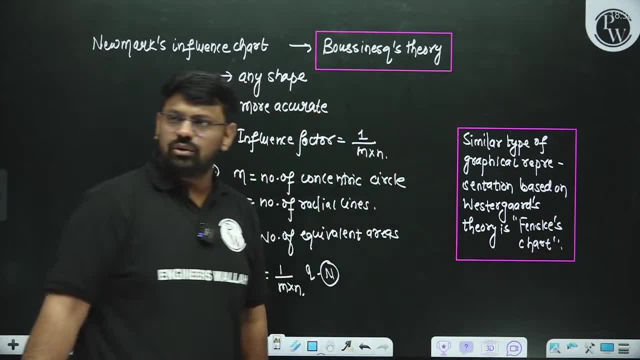 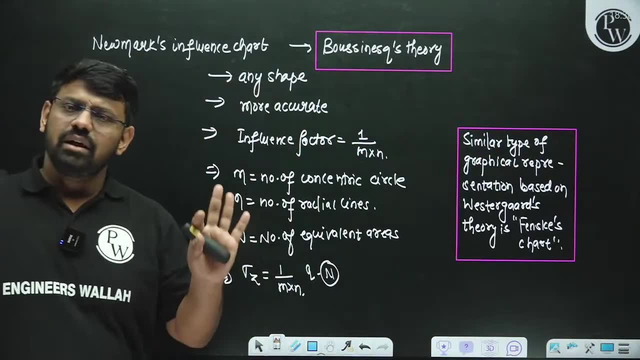 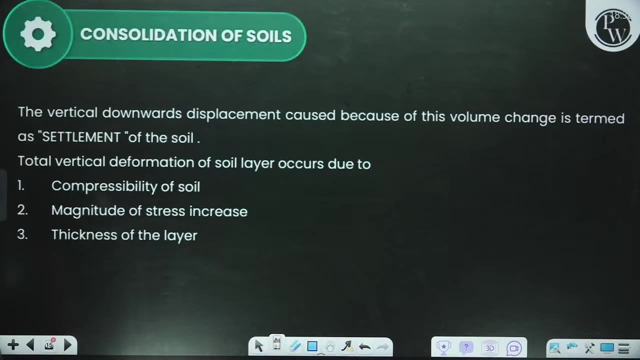 Sir Fenske's chart, Right. So this is Fenske's chart, which depends on Westergaard. Very clear, clear things, right, Very clear things we understand here, Right. So here your stress. distribution chapter ends here. 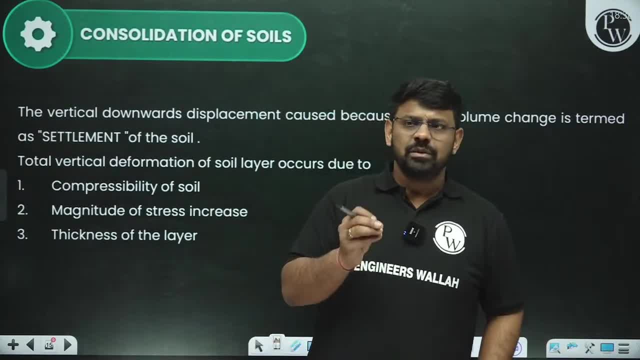 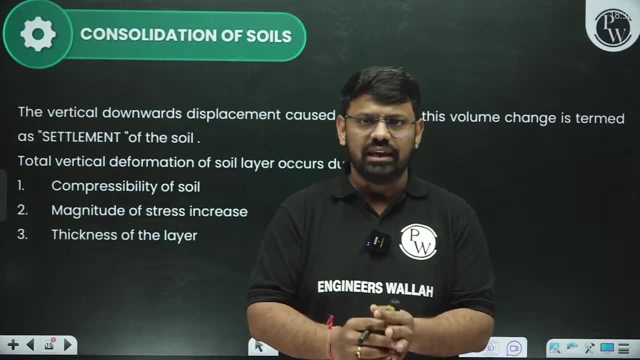 It is a small chapter. It is a small chapter in which, whatever I have told you, if you read it seriously, seriously, then in a very good way, in stress distribution, you will not face much problem. Sometimes one or two questions are asked to you. 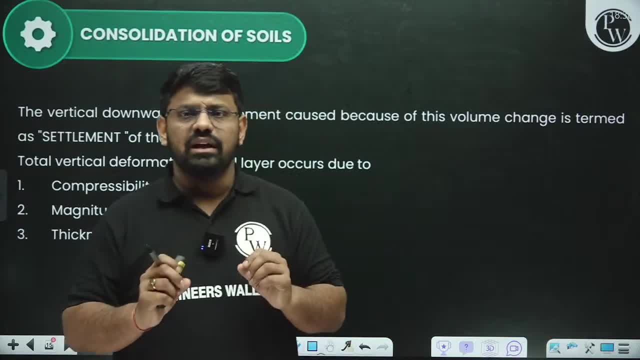 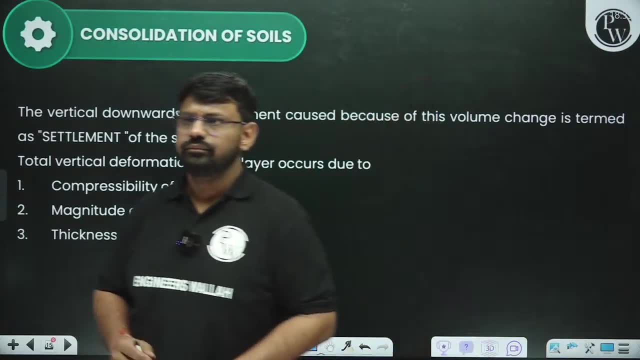 Those one or two questions have been told to you. What are the important points that you have to keep in mind and what are the important points that you have to understand? You will understand it in a very good way, Right, Right sir. 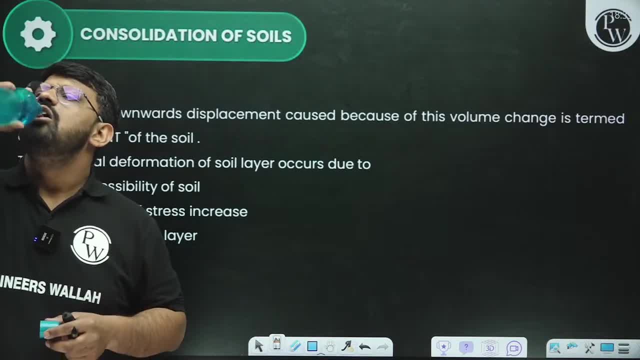 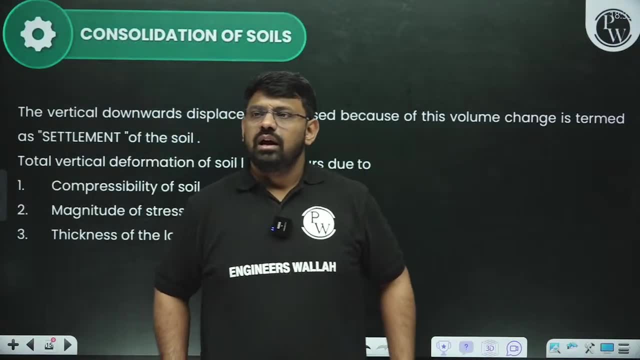 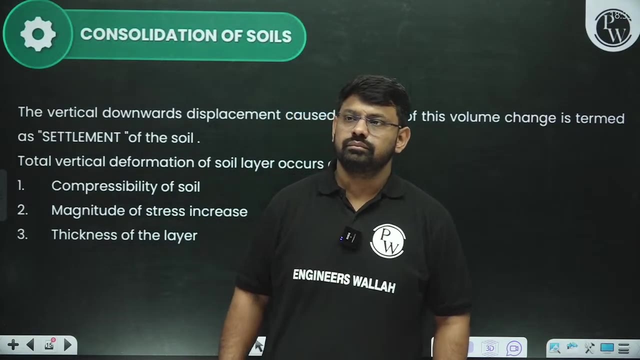 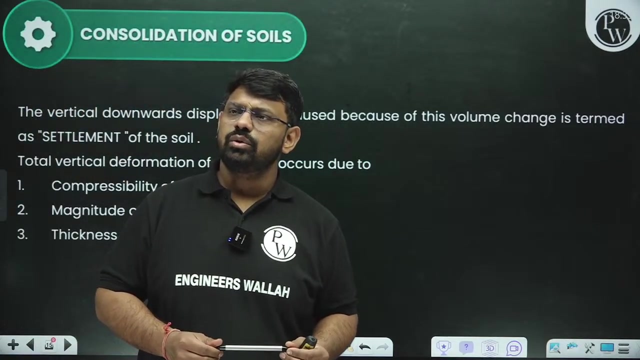 Right, sir, Son load intensity. There is load intensity. Right, Yes, There is load intensity. And sir Vishu Bhai is saying: Sir, do you have to give a complete learning and theory exam to the syllabus? What do you mean? 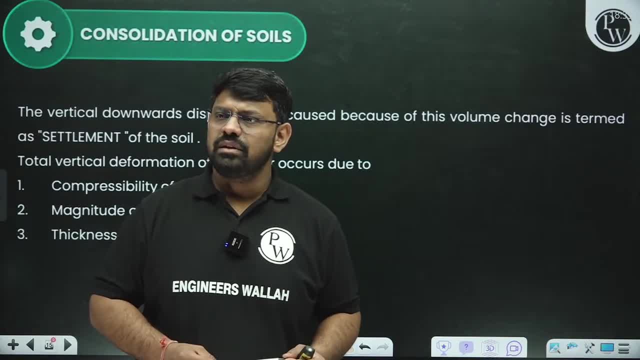 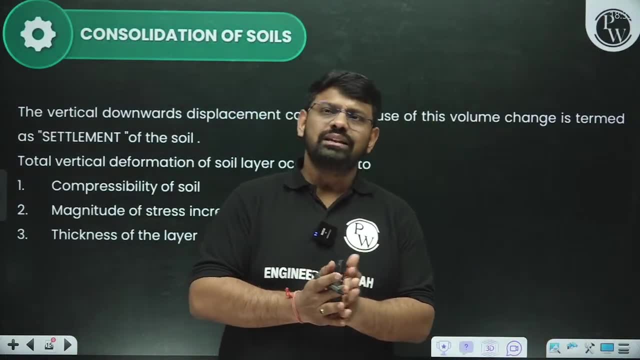 What do you want to say? I don't understand, Sir. I am telling you all the questions in a very good way. Okay, sir, Now let's start. Yes, Now let's start the next and most important chapter. 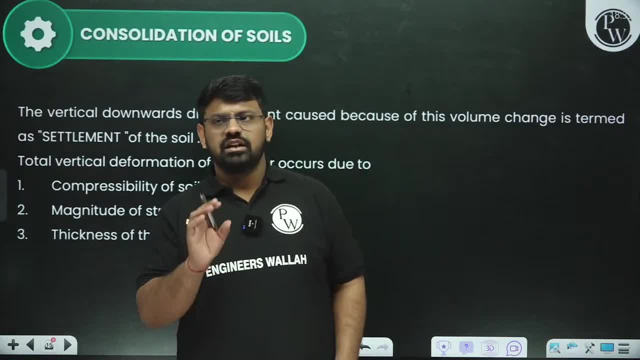 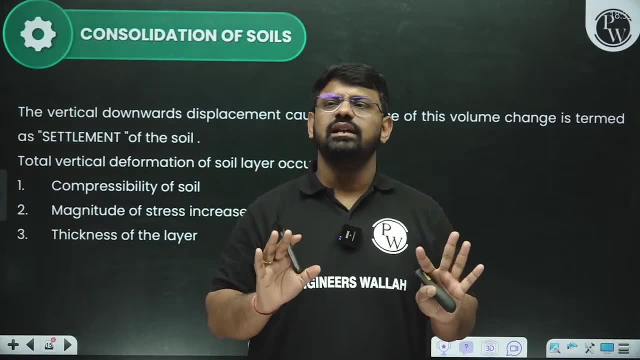 which is going to be the best chapter of today's class. Sir, you have that Consolidation of soil Right. Consolidation of soil Now, in a very clear way, with full focus, with full mind, in a good way, if you are reading it for the first time. 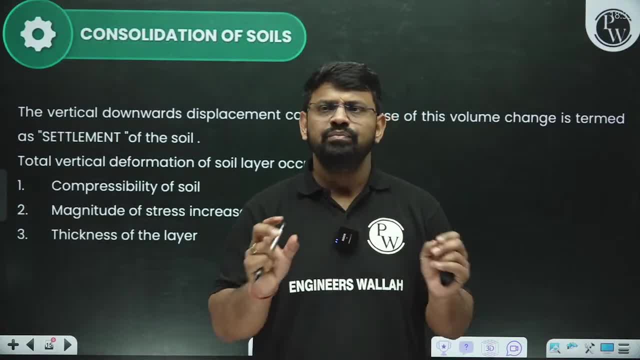 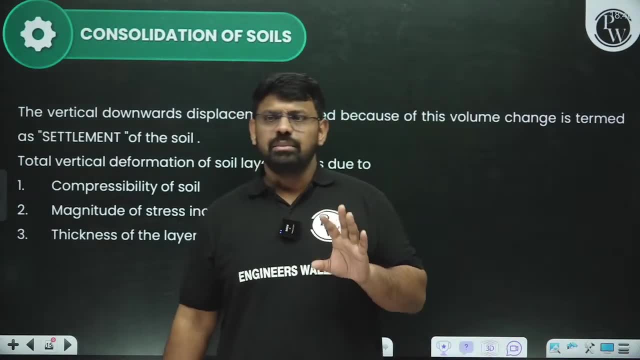 if you are reading it for the last time, if you have never read it in your life. whatever it is, just try to understand it once. We will make the basics of it. After that we will work on it. Okay, Consolidation means the consolidation of soil. 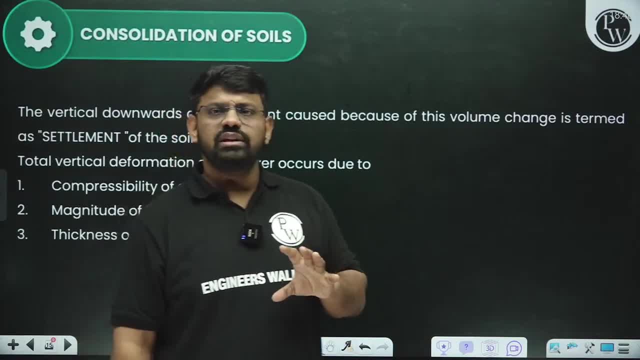 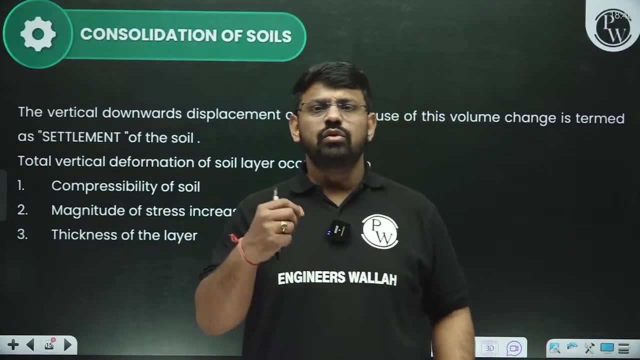 Now one thing: you know that by giving the theory of consolidation. the theory of consolidation was given by Dr Carl von Terzaghi And because of this theory he is also called the father of soil mechanics. What is said? That's why he is also called the father of soil mechanics. 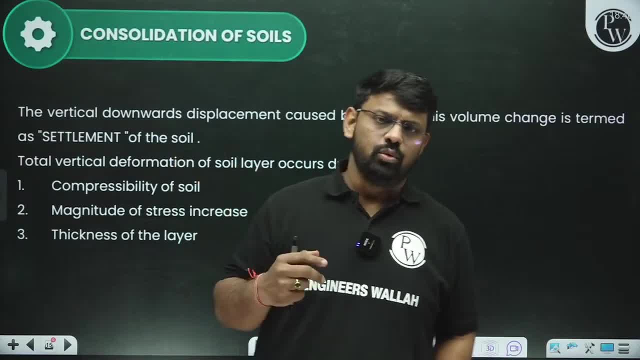 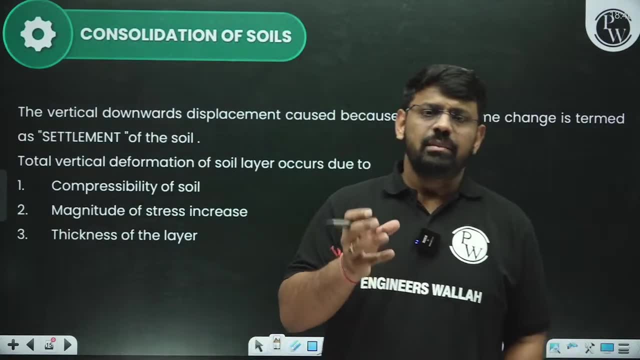 Dr Carl von Terzaghi. He gave you the theory of consolidation. Now, the theory of consolidation means basically the consolidation of soil. So, sir, how does the consolidation of soil happen When I had taught you the compaction chapter? 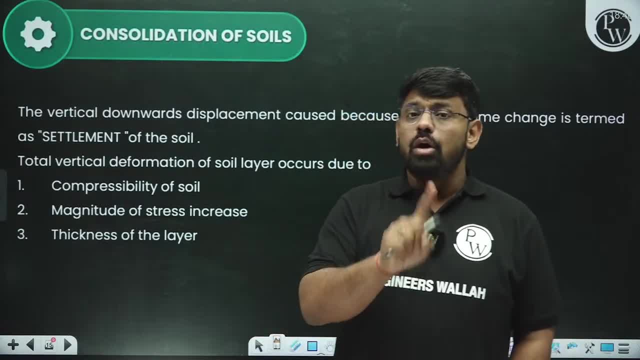 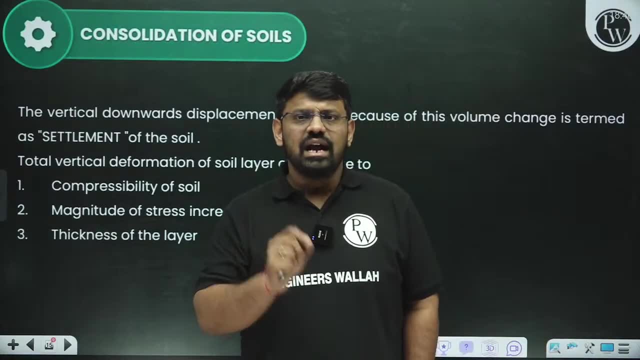 I had told you the difference between compaction and consolidation. What is the difference? So, in consolidation, I had told you that when you have to apply load, you get to see volumetric changes in a particular soil. What do you say, sir? 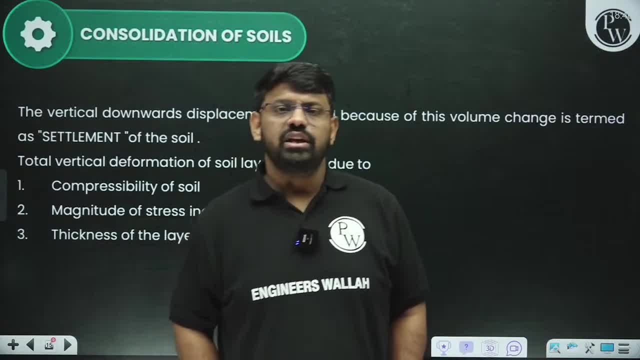 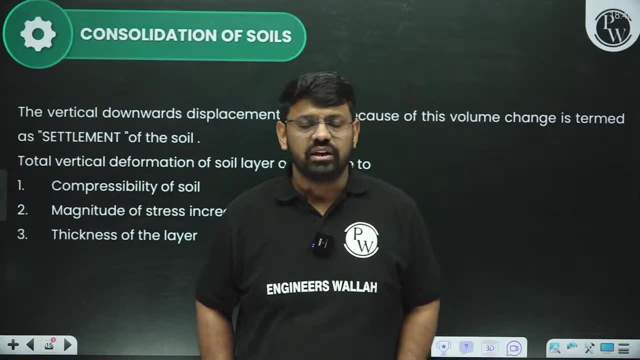 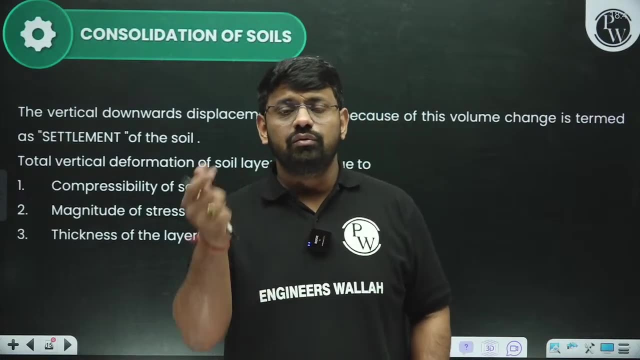 When you apply load, you get to see volumetric changes in a particular soil by expulsion of water. By expulsion of water, then we call it consolidation. Compaction is that, sir? by expulsion of air, when the volume is decreasing, then it is called compaction. 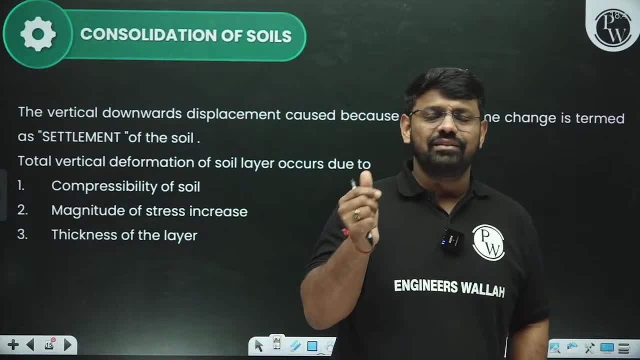 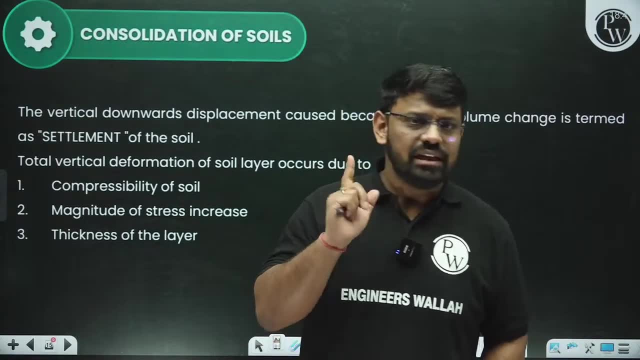 And by expulsion of water. expulsion means the outflow of water. So by the outflow of water, you get to see the difference in the volume. Sir, we call it consolidation of the soil. Is it clear, sir? Now, sir, why is the water expel out? 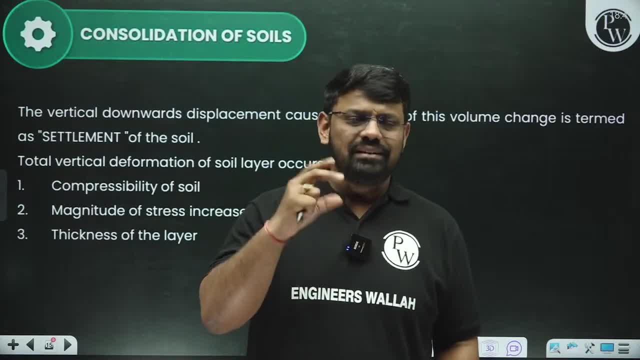 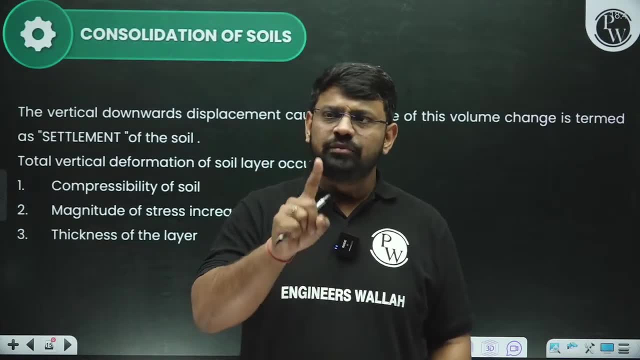 Why is the water expel out? Listen to this, Sir. imagine a soil mass in your mind, Sir. there is a soil mass, It has solids present in it. So first of all, when we apply load, then first of all the air will escape from there. 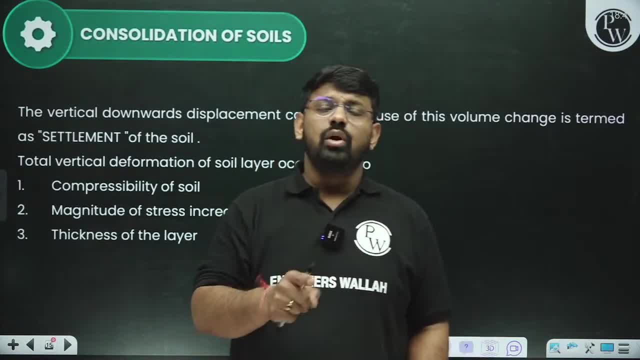 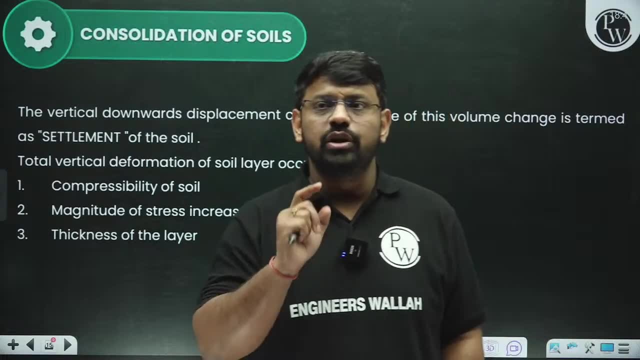 So the air will escape from there. Consolidation happens only when the soil is completely saturated, Means when the soil is completely saturated with you. So when the soil is completely saturated with you, it means, sir, we have removed the air. 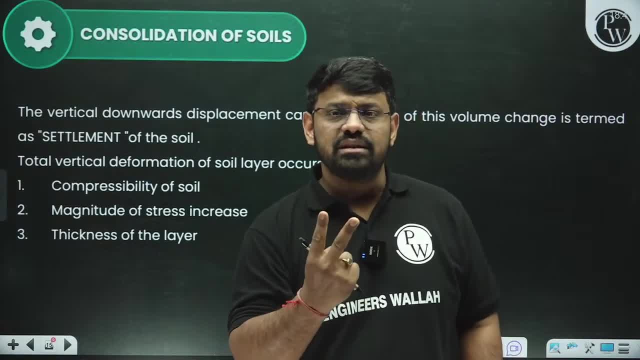 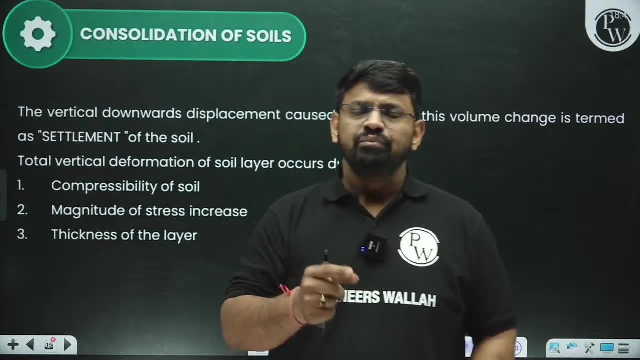 So when the air is removed, then what is left? A two-phase system is left. I had given you a special condition, So a fully saturated system is a two-phase system in which there will be water and solids. Now I will give you a statement. 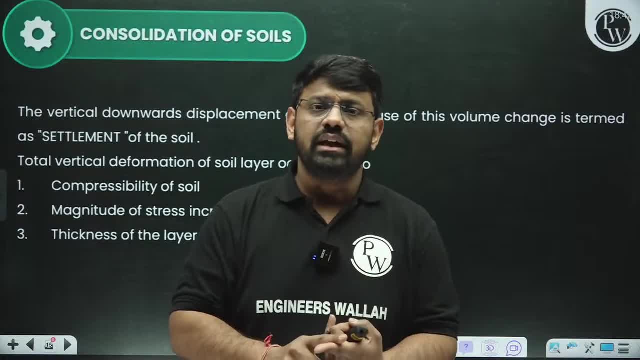 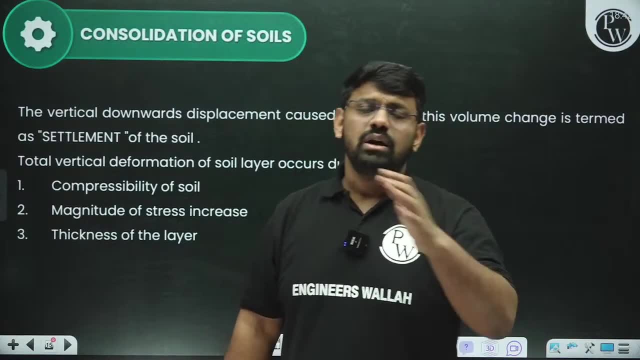 What did I show you? What did I show you, sir? That the solids and water in the soil are always incompressible. Incompressible means: if you apply load, then there should not be any change in the volume, So it will be incompressible. 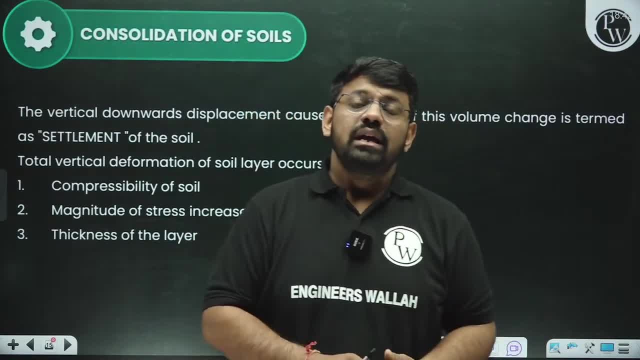 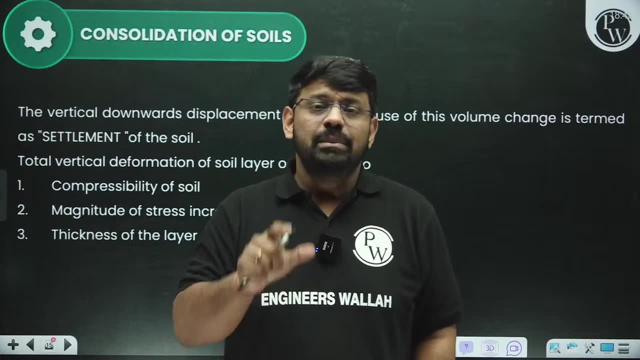 It will not be compressed Means. by compressing them, you will not be able to decrease the volume. What does this mean, sir? Now you are applying pressure, Neither water nor solids can be suppressed. So even if you have to reduce the volume, 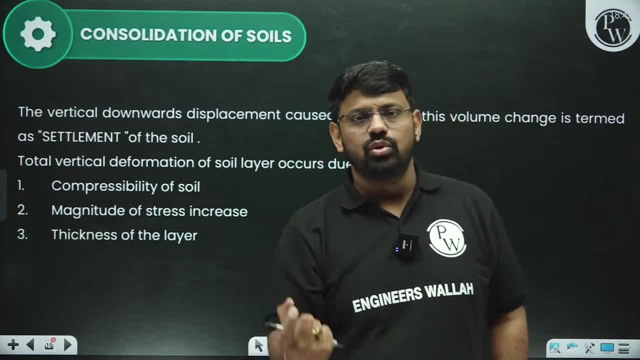 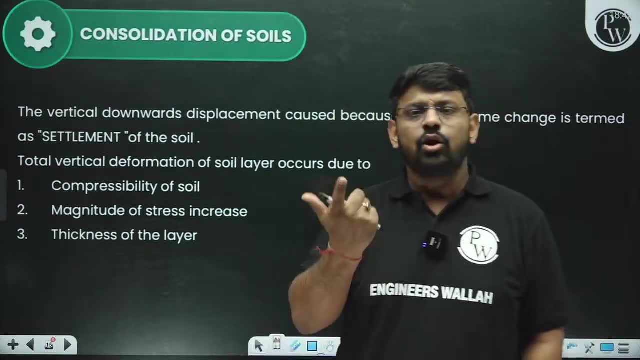 what should be done from there. Water should start coming out slowly. So what does water do, sir? It starts coming out slowly from there. This is what we call expulsion of water, And this is the only option that is available in the soil. 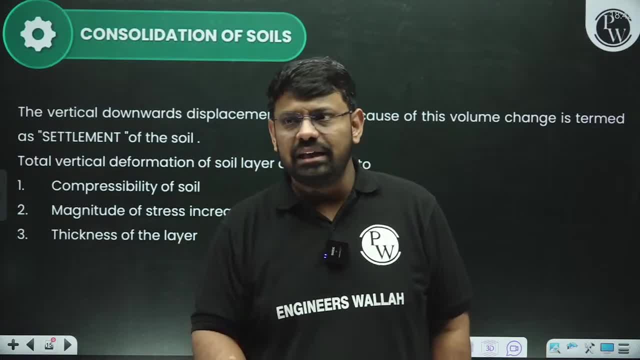 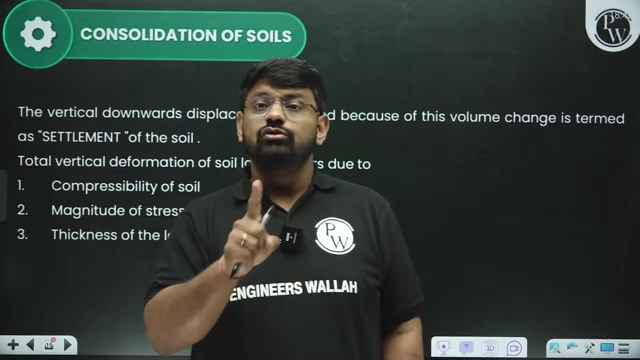 So the other option that is available is that water will come out from there And because of this expulsion of water, because that load has been applied on it for a long time, that is why I had told you that consolidation is a time-dependent process. 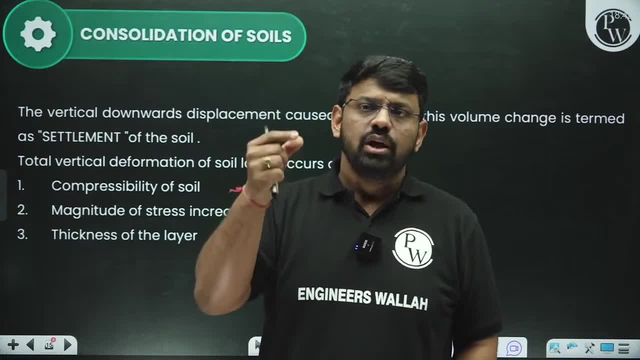 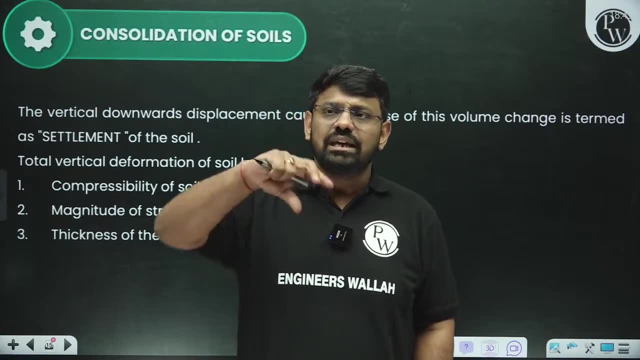 It takes time. It is not that it will happen immediately. It will take time. It will take time, For example, when the load is applied there. then we have a time-dependent phenomenon: that water is coming out from there And slowly we are getting to see. 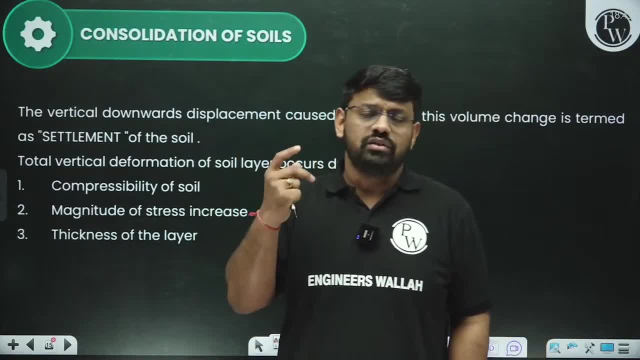 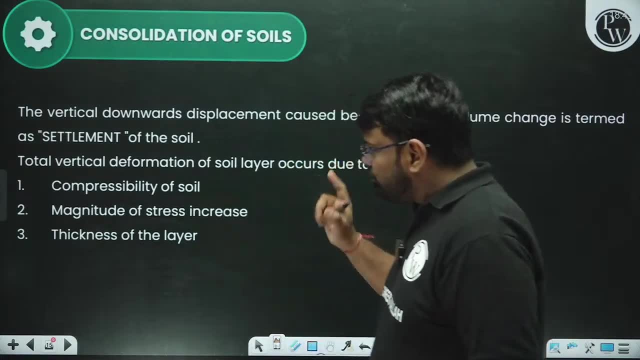 a change in its volume, We have a slow process. This is what we call consolidation. So, sir, we are clear about this. Now look at this consolidation: If you have applied the load due to the change in the volume, 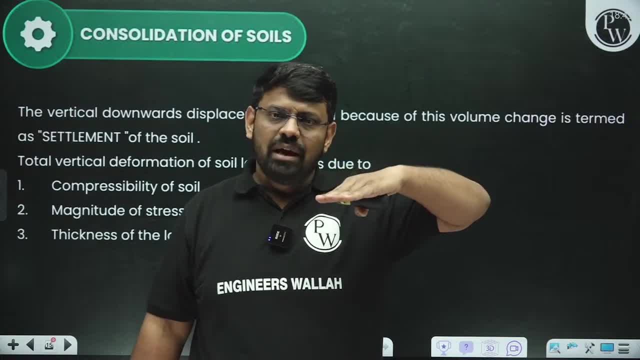 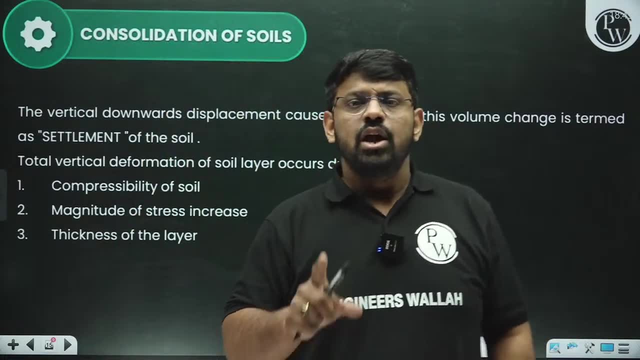 you will get to see that the volume has changed in the soil. so you will get to see some amount of settlement in the soil. So the vertical deformation that we get to see, that is what we call settlement in this. What do we call it, sir? 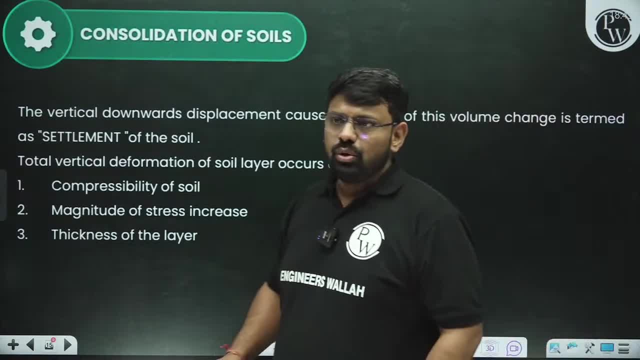 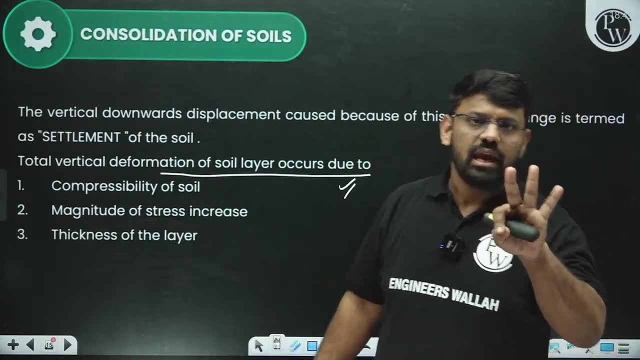 We call it settlement. So this is known as settlement. Now look here. So the total vertical deformation that we have in this particular soil layer is due to three reasons. The first reason, sir, we have, is compressibility- That there is compressibility in the soil. 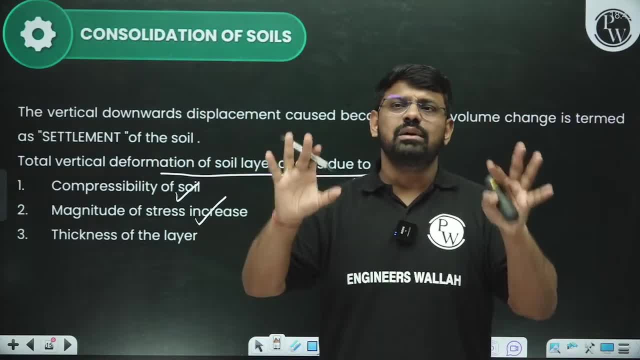 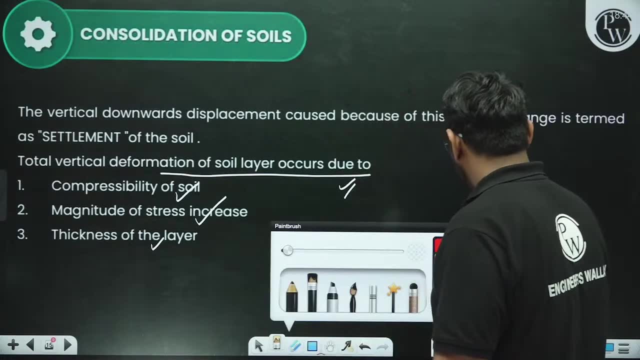 That is why it is happening, That is why we are having an increase in stress. And the third reason, sir, is the thickness of the layer. That means, sir, the first property- see, the first property- is the property of the soil. 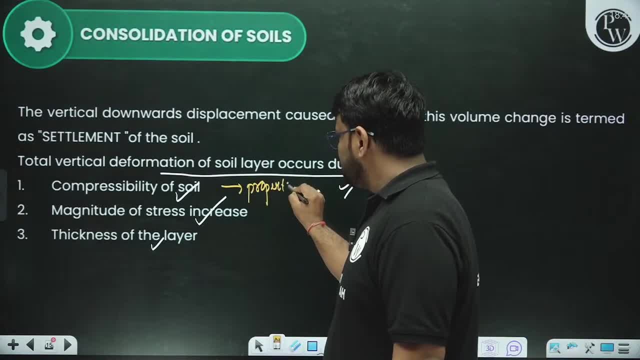 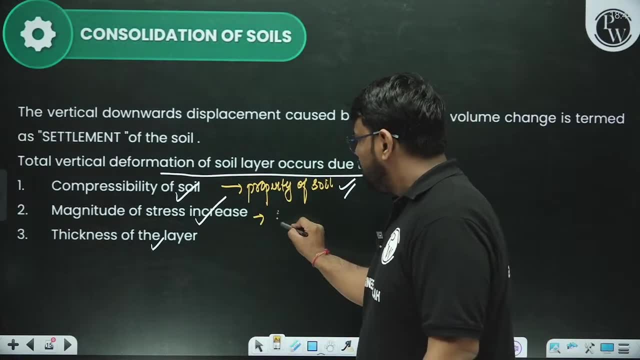 So, first is the property of the soil. The compressibility, sir, is the property of the soil. So first we have the property of the soil. Second, sir, we have depended on the loading conditions, That means the magnitude of stress. 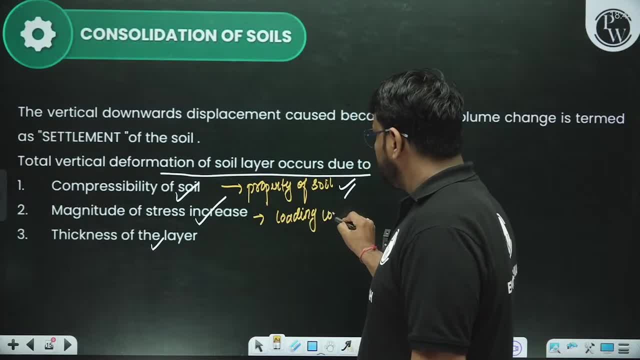 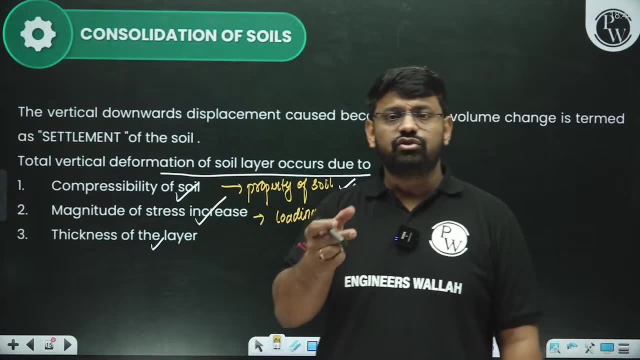 What does this mean, sir? This is basically dependent on the loading conditions. After that, you have the thickness of the layer. The thickness of the layer means the sub-strata. How is the sub-strata? It depends on that. This means, sir, the nature of the sub-strata. 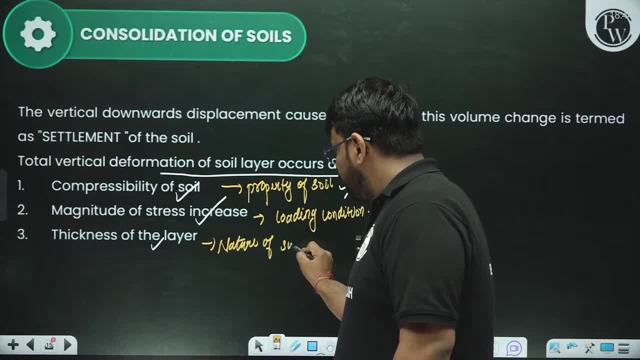 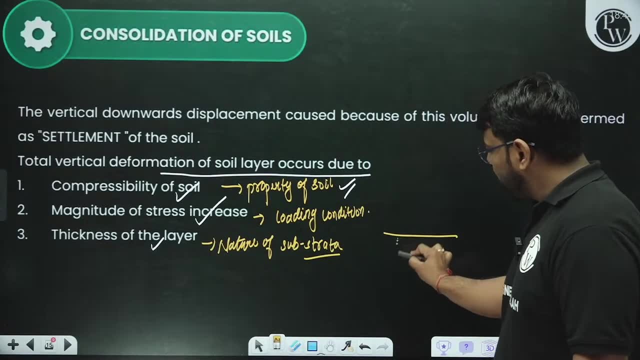 Whose nature, Sir? the nature of the nature of the sub-strata, The nature of the sub-strata. The strata means the layer and the sub-strata means the soil below the ground. So this becomes the sub-strata. 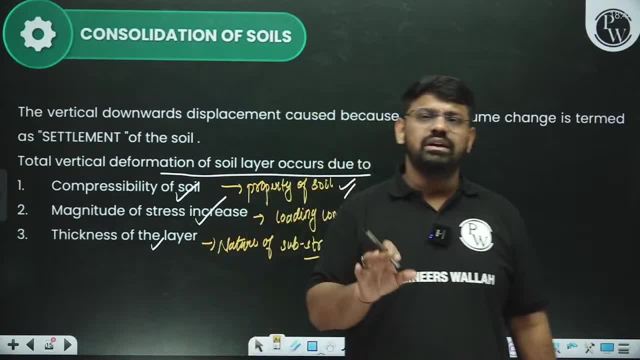 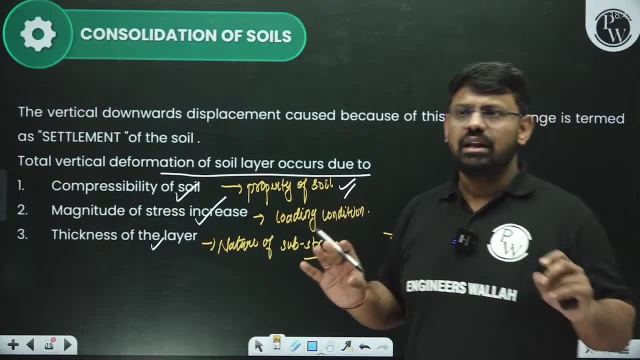 So it depends on its thickness. So these are the three parameters that we have to keep in mind, due to which we get to see this vertical deformation or settlement. Tell me, is it clear up to here? Is the basic concept clear up to here? 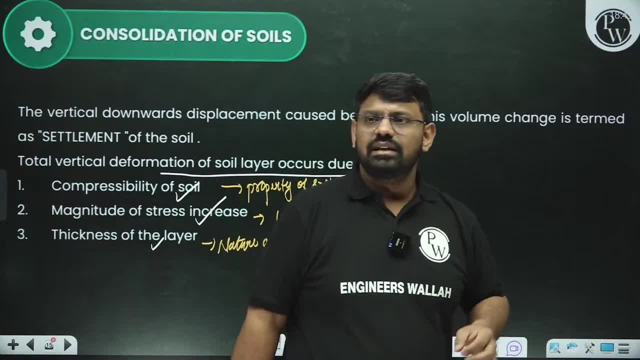 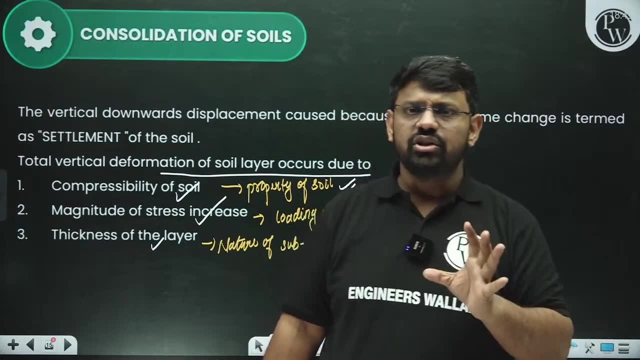 Tell me quickly All the students please comment and tell me. Put the heart symbol in the comment box and tell me, sir, is the point of consolidation clear up to here? You might not have studied it in a crystal clear way or understood it. 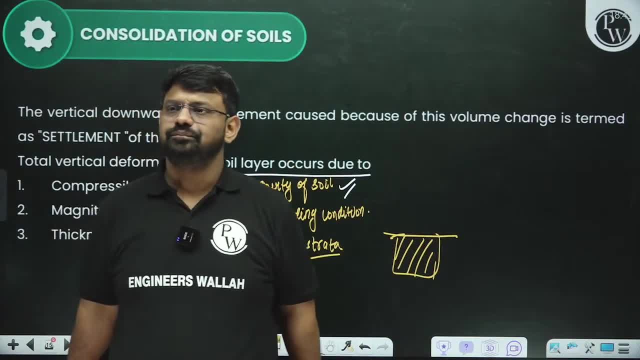 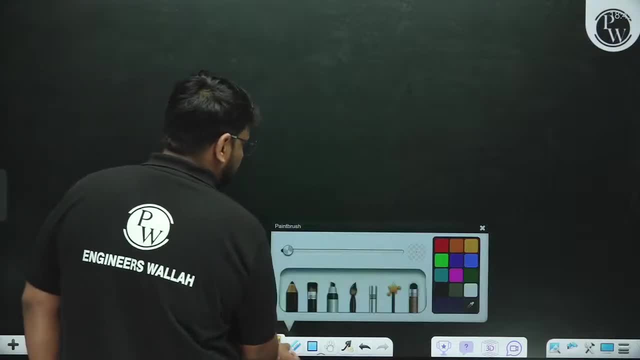 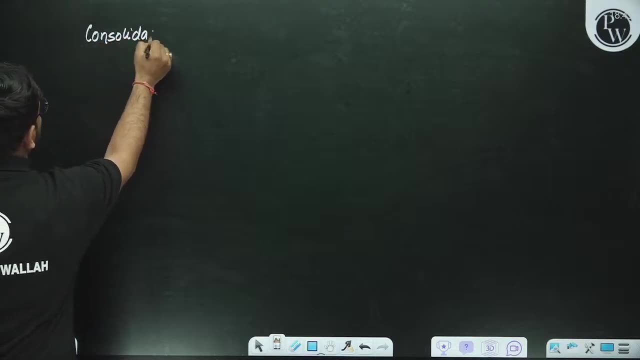 Quickly comment and tell me: Sir: yes, it is clear. Very good, Now look further here. Very good, Now look further here. Whenever we talk about consolidation, you have to understand some things. What do you have to understand, sir? 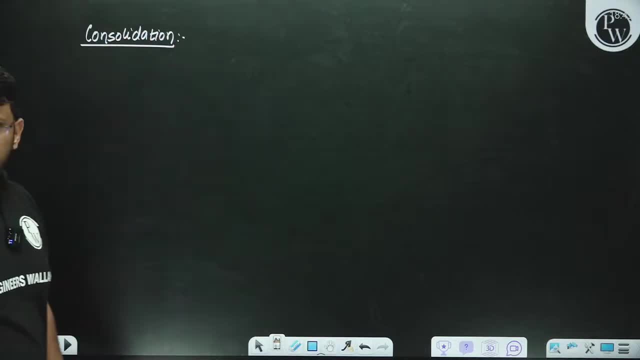 Quickly tell me, Sir, when I talk about consolidation, you have to understand two or three things. in consolidation, Sir, the first thing we have to understand is initial compression. What do you have to understand, sir? First is your initial compression. 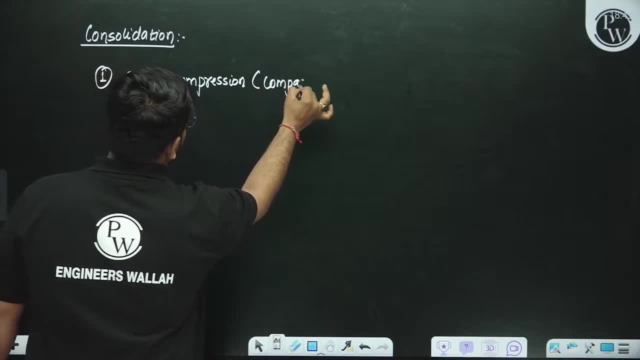 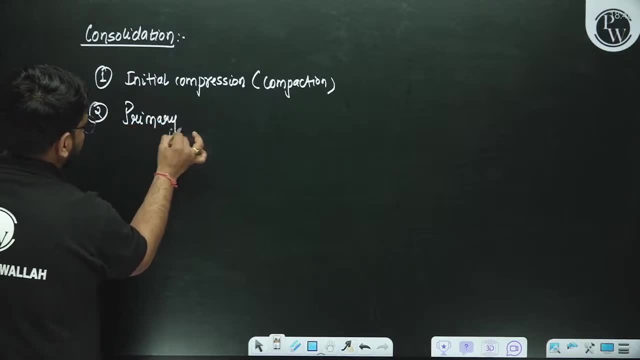 The first stage is initial compression, Sir. we also call it compaction. I will explain it now, Sir. the second thing we have is primary consolidation. Okay, Primary consolidation. We also have this, sir. And the second thing we have is: 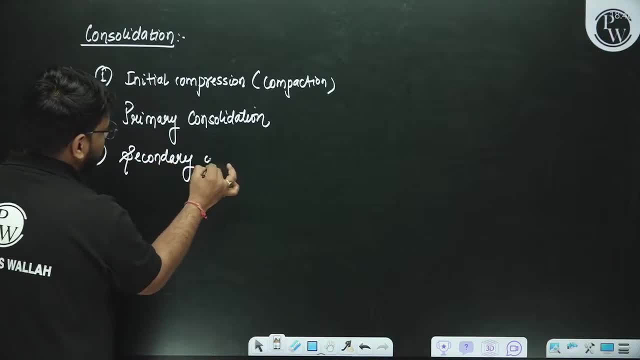 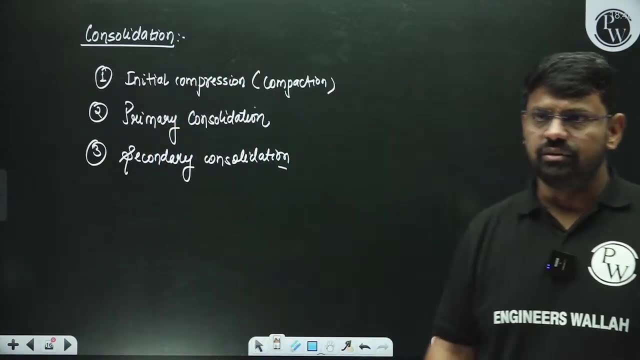 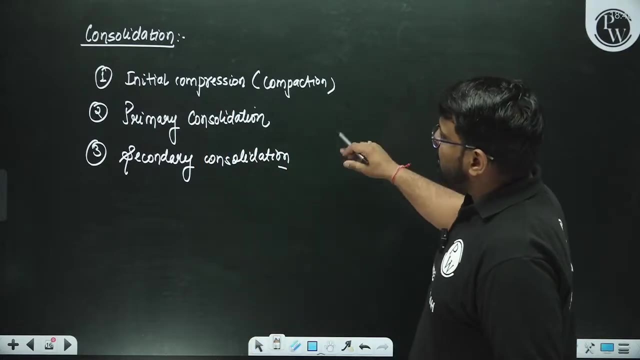 secondary consolidation. Try to understand it well. Second we have is secondary consolidation. The second thing we have is secondary consolidation. Very good, Now look, sir, What are the stages? The stages that I have explained to you. they are all there. 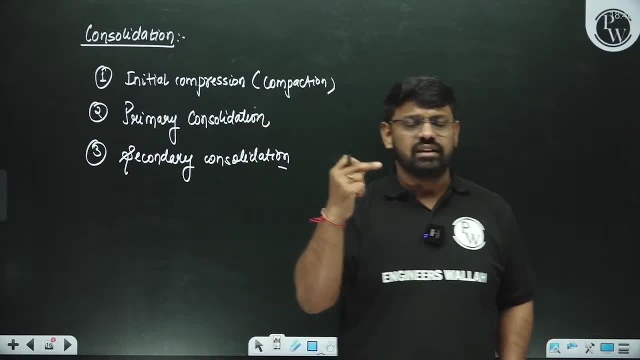 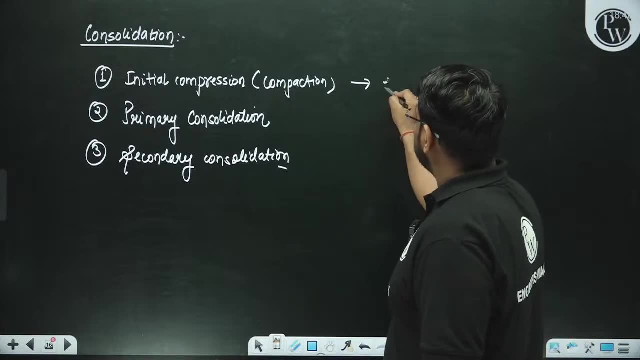 First of all, whenever you put a load on us, there will be initial compression. Initial compression is instantaneous, It is instant. It is instant We call it compaction. So, sir, initial compression is the compaction process. only What is happening here, sir? 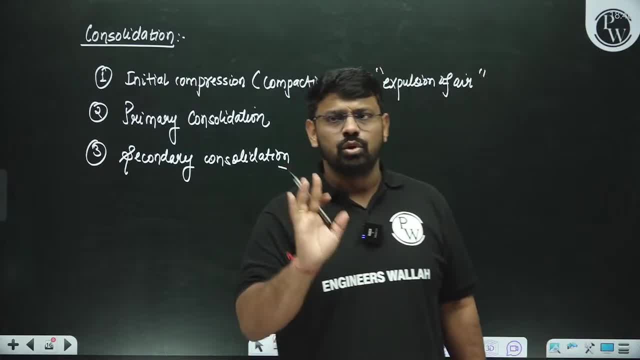 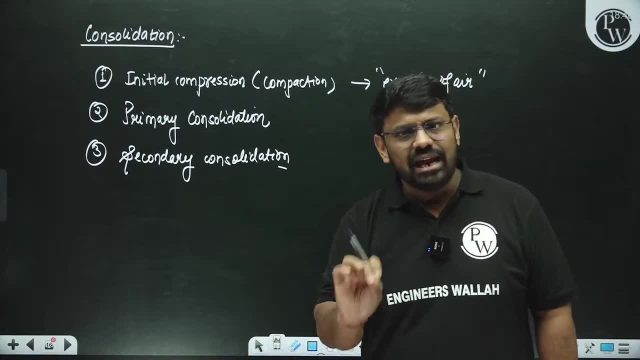 We call it compaction. We used to call it sun-hannan. Now, here, because of this expulsion of air, the volume will decrease. sir, There will be a change in the ayatan. The air will also come out. 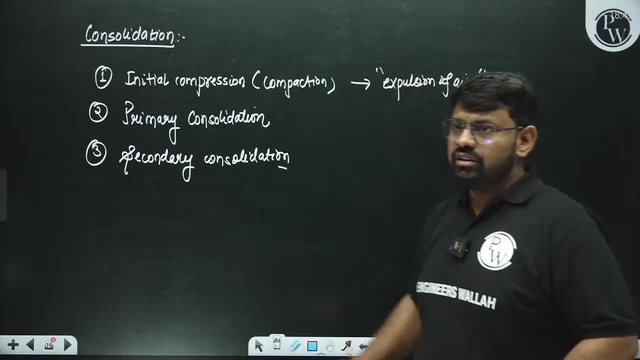 So the air has come out of the voids. That means, sir, there will be a change in the ayatan. That means we will see volumetric changes. Now, because of these volumetric changes, we will see vertical deformation. 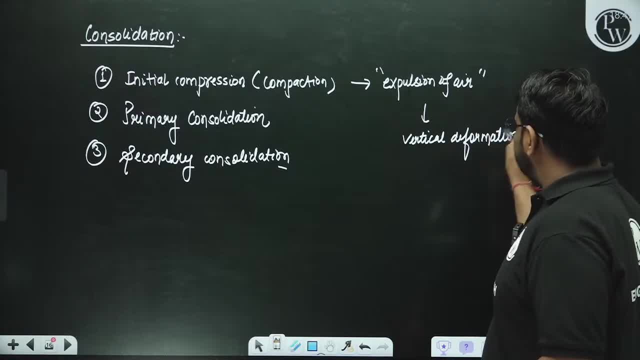 So, sir, this is also very clear: If the air comes out of there, then the compressibility property of the soil. what did you get to see because of that? Because of that, you got to see vertical deformation, This same vertical deformation. 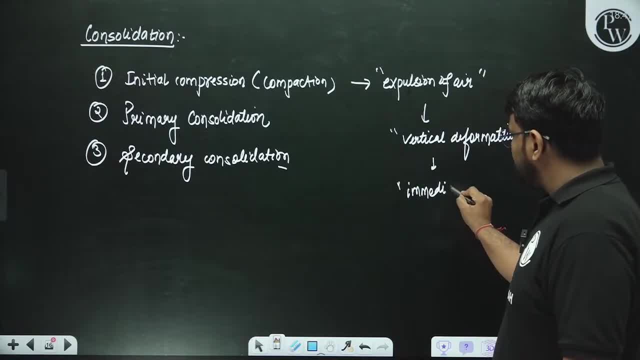 we call it here, sir, immediate settlement. What do we call it? This is known as your immediate settlement. So if you are ever asked the definition of immediate settlement, this is what it means. So this is your immediate settlement. 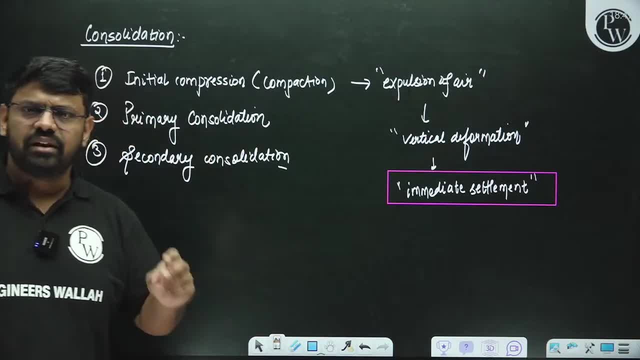 What is it called, sir? We call it immediate settlement. It is instant settlement. It is instant settlement. The air came out of there: Vertical deformation. Let's move ahead, sir, Now, after immediate settlement, when this initial compression has happened. 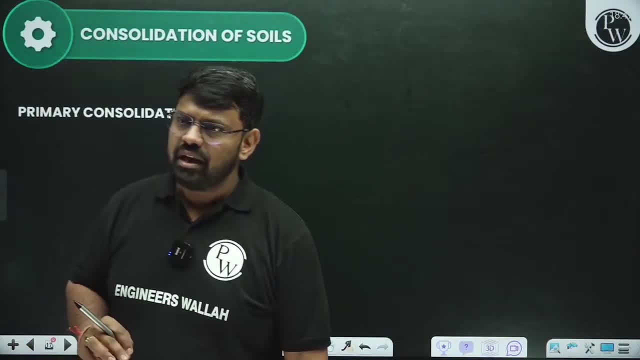 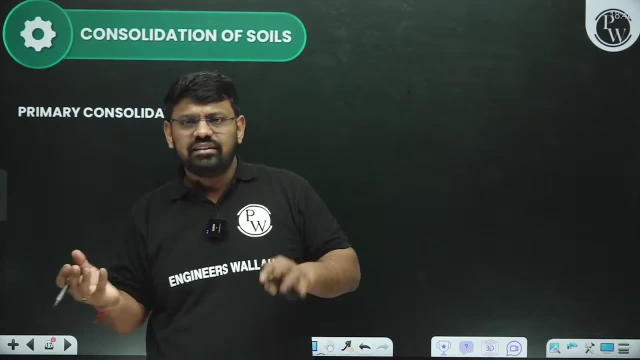 Sir, is compression and expulsion the same Son? I have told you the secret That compression means the change in the volume, Expulsion means to come out And because of coming out there is a change in the volume. There is a slight difference in both. 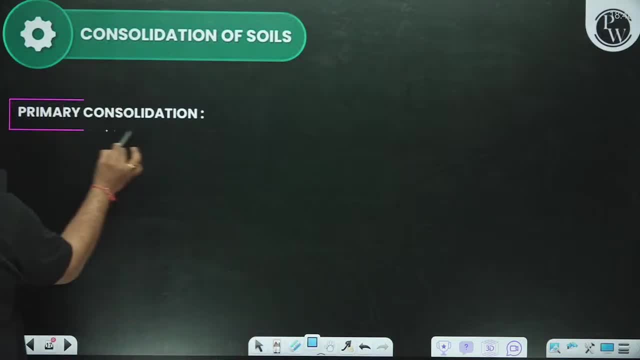 Now look here. Second, we have primary consolidation. So, sir, primary consolidation happens first when your initial compression is over And the soil that you have, that will be completely saturated. Okay, For saturated soil, you will get to see primary consolidation. 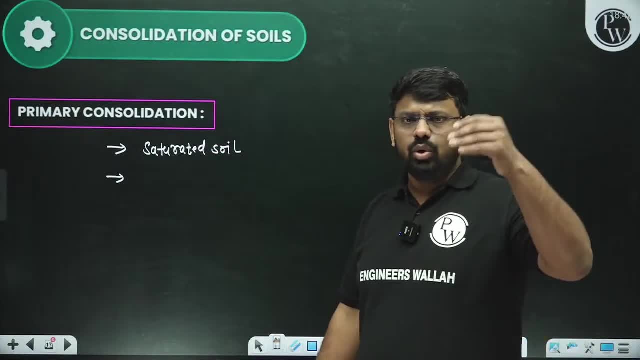 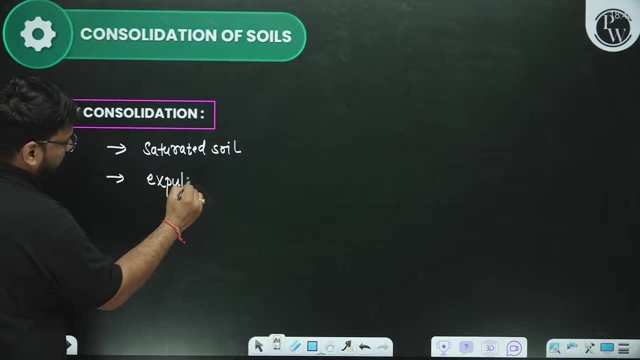 Now, primary consolidation means that you applied load and you got to see expulsion of water, Which I have explained to you. So, sir, in this case you will have expulsion of water And, because of this expulsion of water, you will get to see volumetric changes. 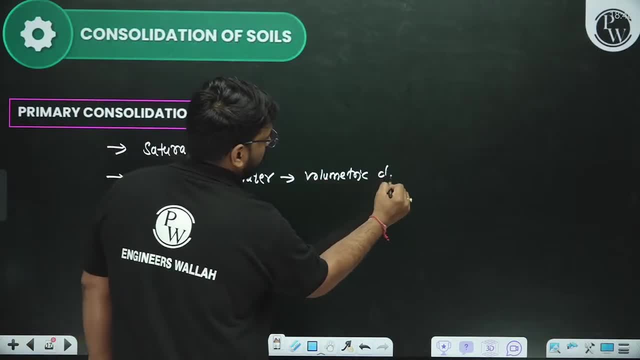 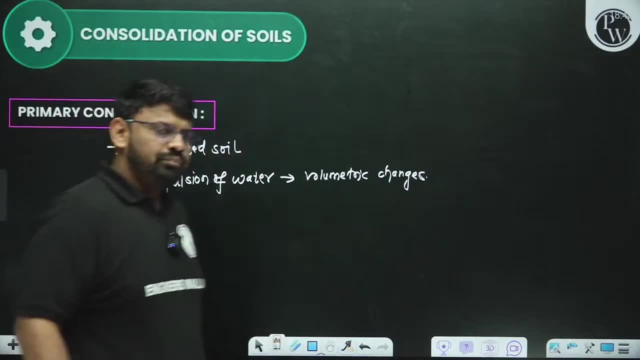 And because of this expulsion of water, you will get to see volumetric changes. And because of this expulsion of water, you will get to see volumetric changes Now. similarly, you can say one more thing here, sir, Sir: expulsion of water means. 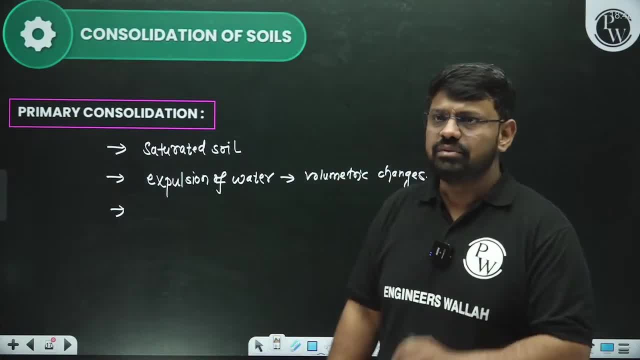 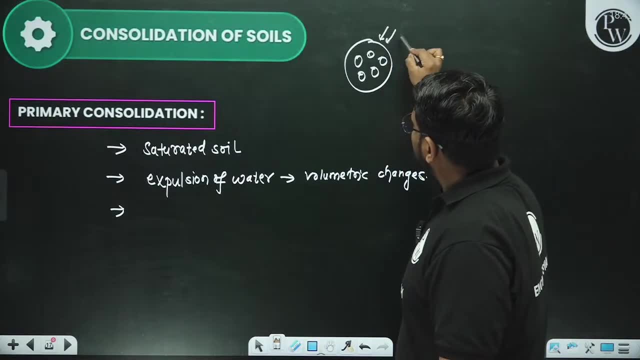 that whenever we apply load. I had explained to you one thing, Sir, when I was teaching you in Effective Stresses. Sir, look here When we have solids, etc. Now, when we apply pressure on the soil, then the water present in it. 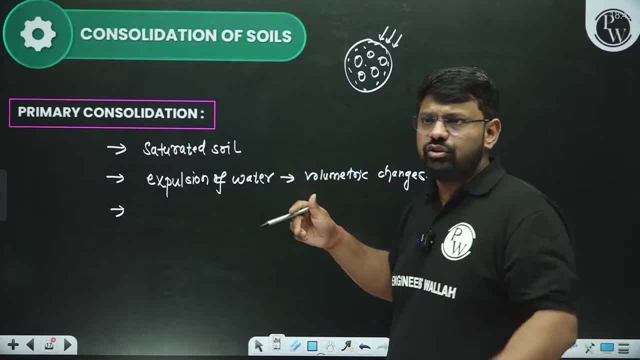 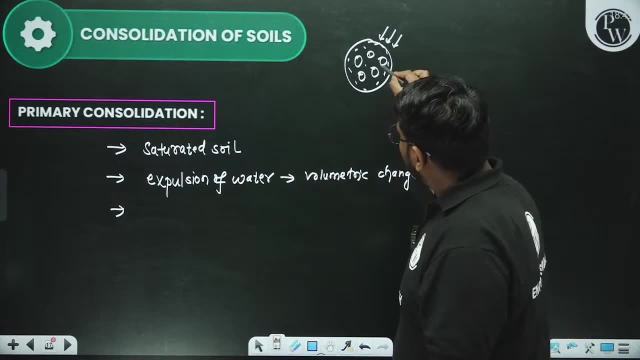 does it apply pressure on it? That is our pore water pressure. So, sir, pore water pressure will be developed in an amazing way. So, sir, the pore water pressure will be developed. So, sir, the pore water pressure will be developed. 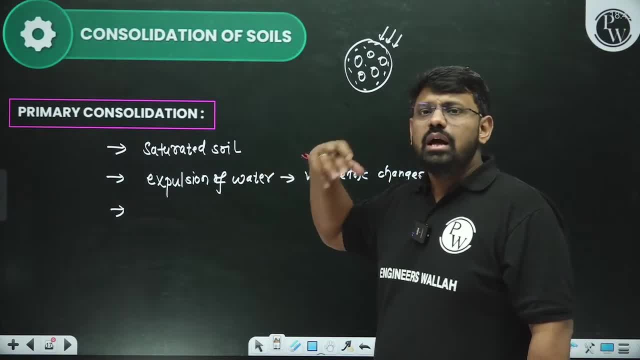 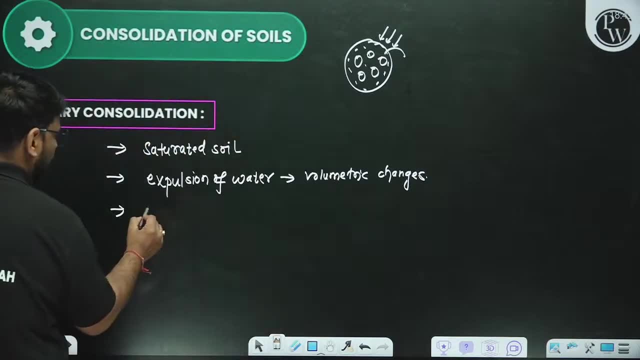 Now this pore water pressure will have to be dissipated, Means it will have to be released. Only then there will be volumetric changes. So how will it be released? By coming out of the water. So, sir say expulsion of water. 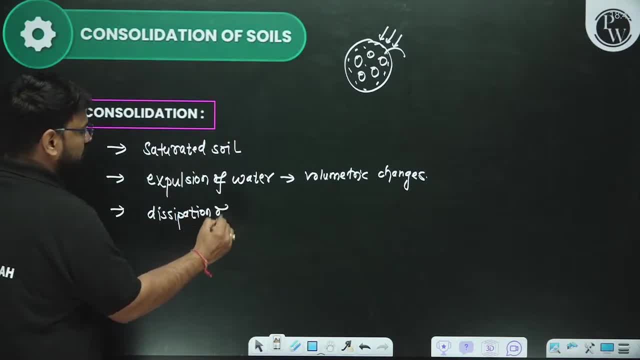 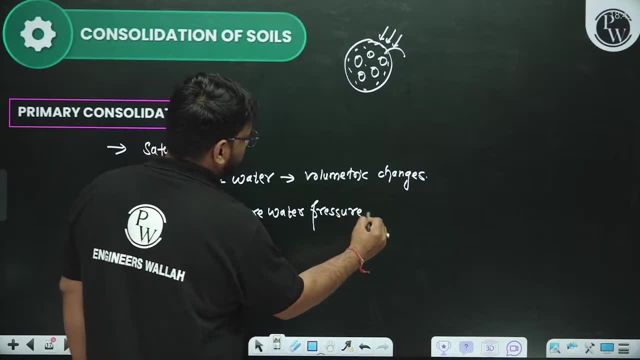 Or, sir you say here dissipation of pore water pressure. What do you say, sir? You say dissipation of pore water pressure. So it is exactly the same, sir. So this is because of the dissipation of pore water pressure here. 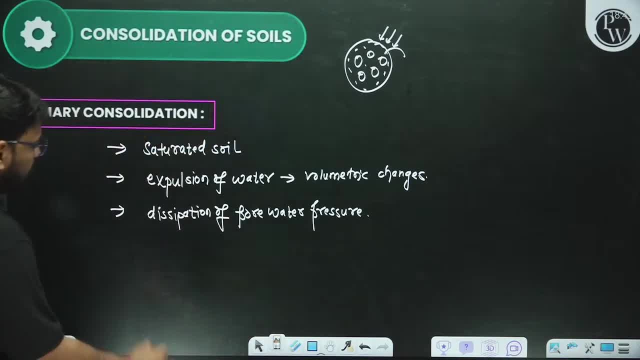 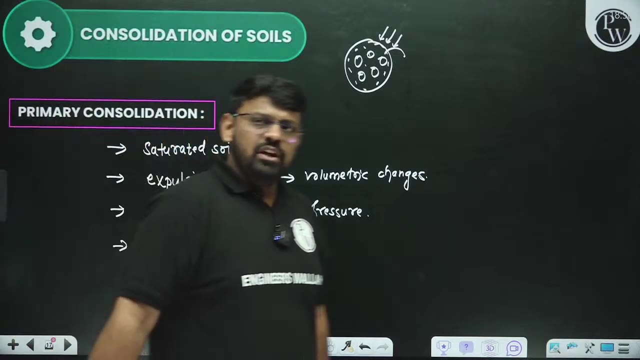 So we get to see consolidation. What is consolidation, sir? This is called primary consolidation or one degree consolidation. Sir, we call this one degree consolidation or primary consolidation. This is known as your primary consolidation. Now, because of this primary consolidation, 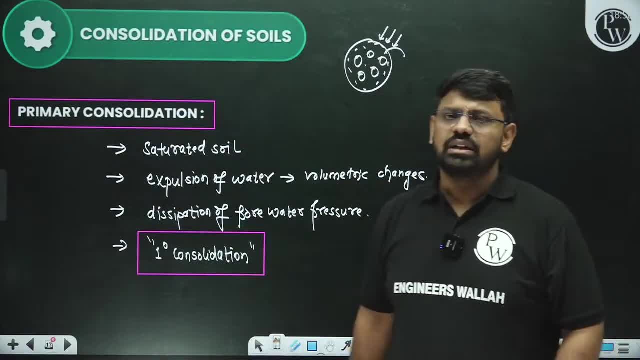 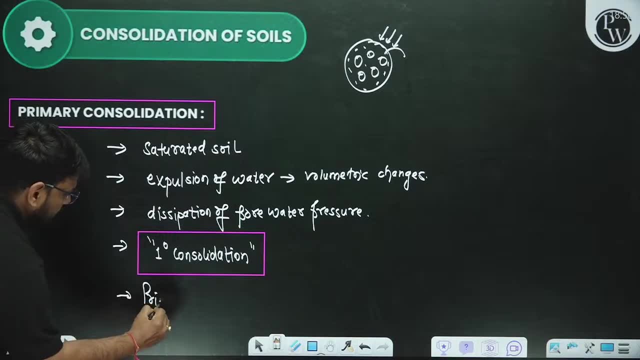 the settlement that we get to see. we call that settlement primary settlement. That particular settlement is known as your primary settlement. What we will call this settlement, sir? We will call it primary settlement. It is absolutely clear. There are time-dependent phenomena. 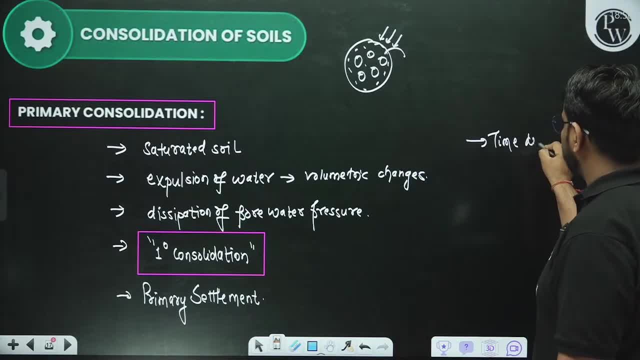 It is absolutely correct. So here you can understand, sir. this is a time-dependent phenomenon. We are getting to see this because of static loading. I have told you all these points earlier, That time-dependent static loading. I have told you all the things. 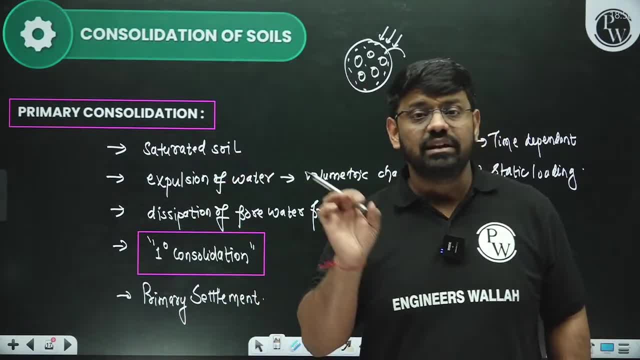 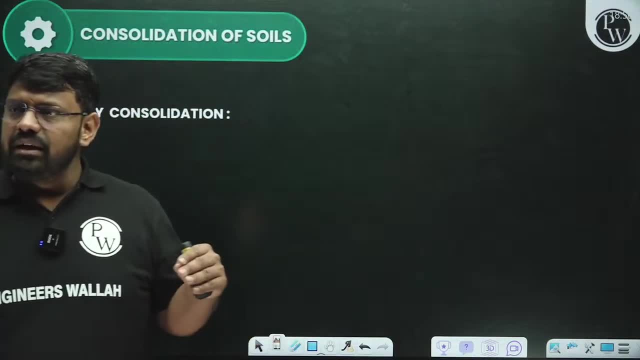 So, through this primary consolidation, the settlement that you get to see first of all, this becomes clear to us Now, sir. what will happen When you have a primary settlement in the soil right, When the primary settlement in the soil 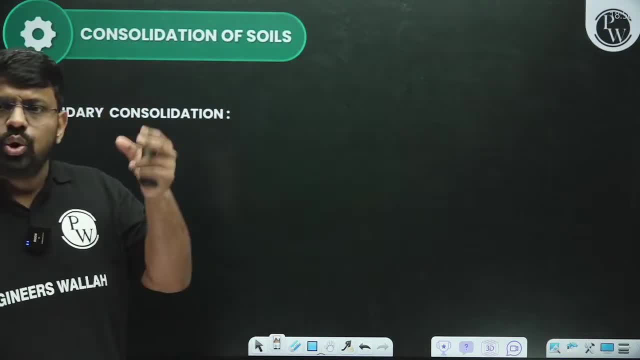 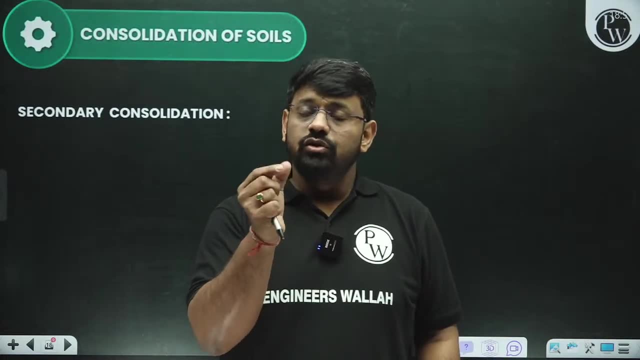 ends at the end of the primary settlement and your load is still attached, then what will happen, sir, Then? the particle rearrangement in the soil means when the particles in the soil reorganize themselves, then you get to see particle rearrangement. 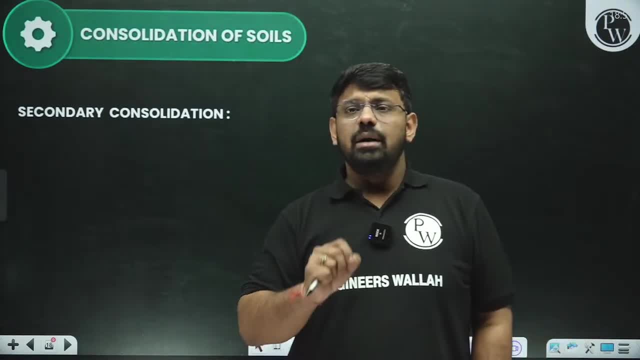 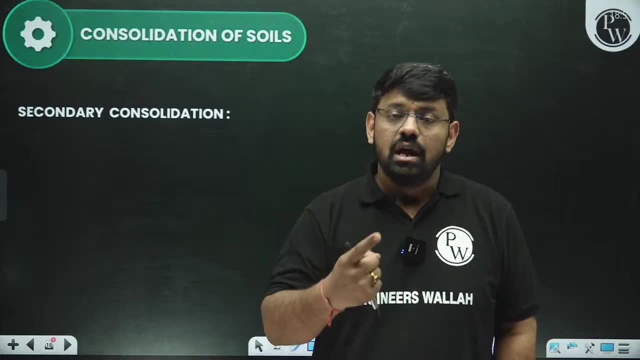 So, because of that particle rearrangement, you get to see some amount of volumetric change. And this volumetric change that you got to see because of the particle rearrangement, what do we call this? We call this, sir, secondary consolidation. 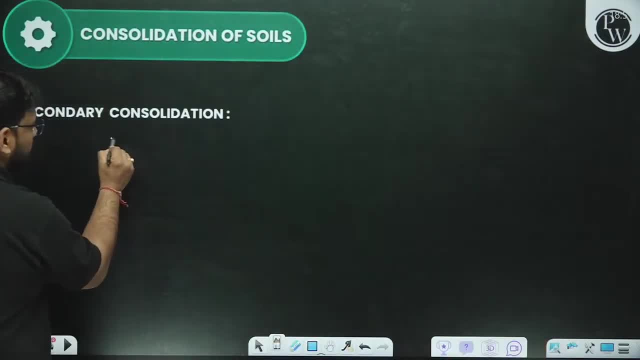 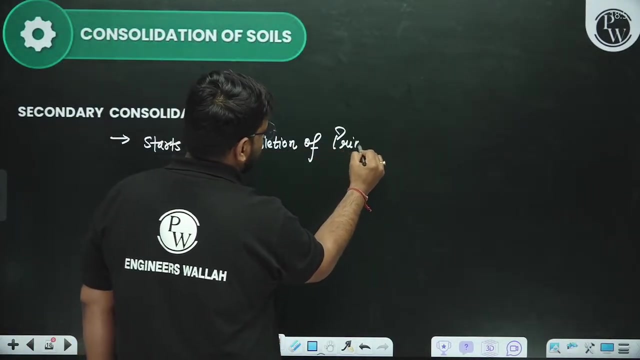 This is known as your secondary consolidation. Now, one thing to understand here is that the first thing is it starts after completion of. So, sir, it starts after completion of, after completion of primary consolidation. So, sir, when your primary consolidation is completed, then only. 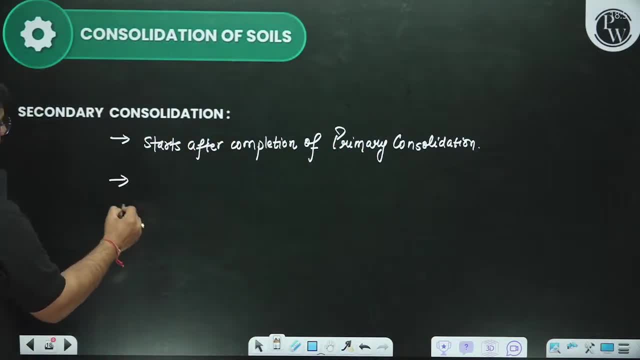 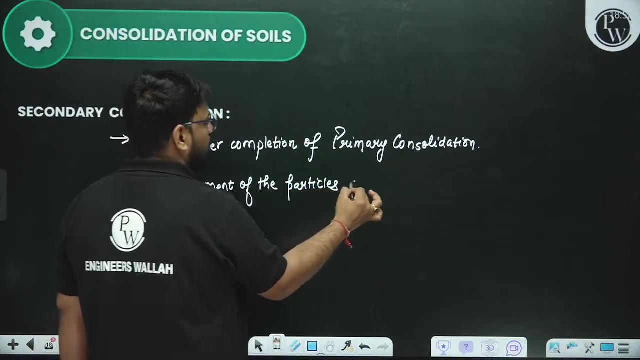 secondary consolidation starts Now, sir, after completion of primary consolidation. when the load is constant, then rearrangement of the particle, rearrangement, rearrangement of the particles or readjustment of the particle that we have causes because of this, what happens? 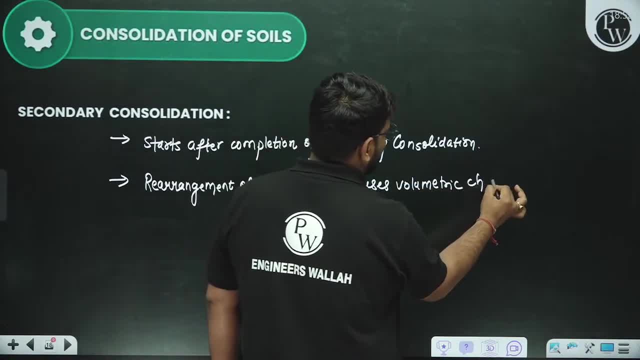 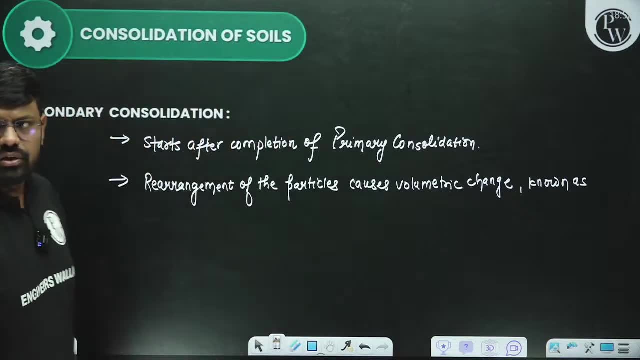 Causes volumetric change. Because of this, we have some volumetric change, volumetric change which is known as, which is known as secondary consolidation. And what do we call this, sir? This is what we call secondary consolidation. So, sir, one thing has been understood. 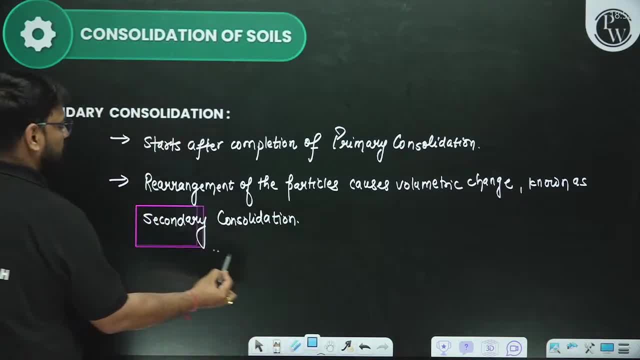 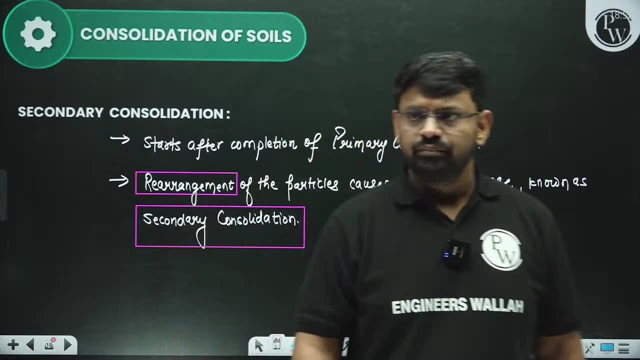 that here, expulsion. expulsion is nothing, sir. Here we have particle rearrangement. What is the particle, sir? Rearrangement is happening. Particle is readjusting itself. Right, Particle is readjusting itself. It is absolutely clear. 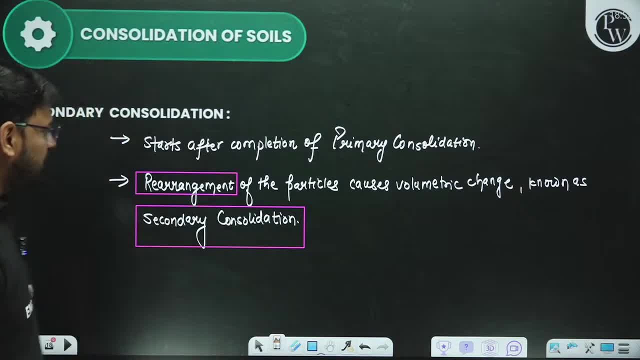 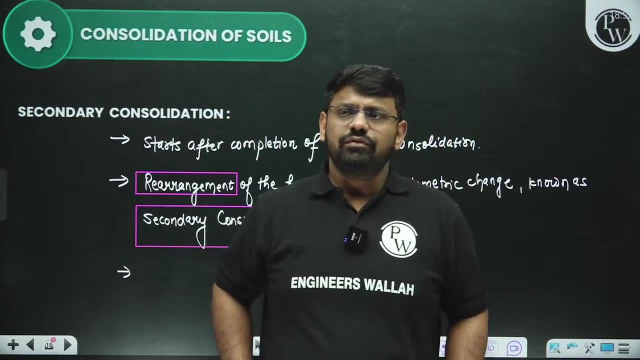 Right, It is absolutely clear, sir. Now, after this, sir, when we talk about secondary soils, secondary consolidation, then, sir, the rearrangement of the particle is important. Now you will see further, sir, that once all the children comment and tell. 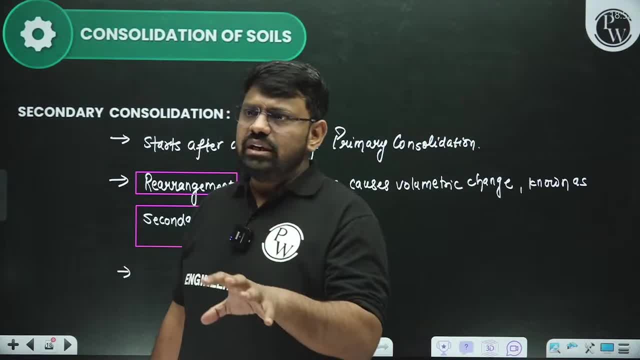 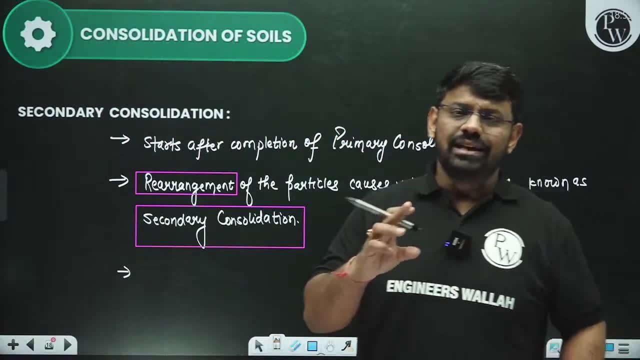 that secondary consolidation. you will get to see more in cohesion-less soil or you will get to see more in cohesive soils. Think quickly and tell. You have to think and tell this thing that, sir, when I talk about secondary consolidation, then secondary consolidation. 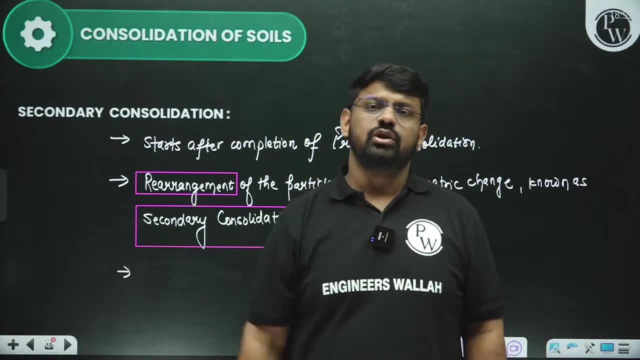 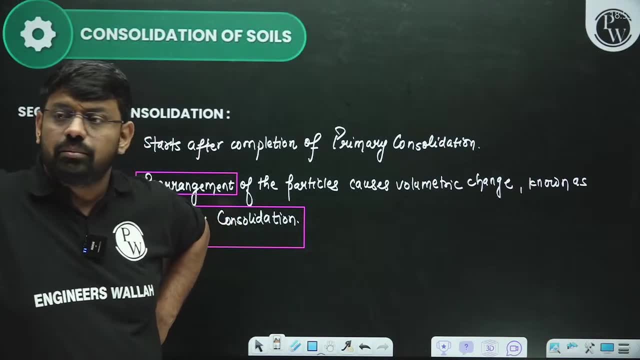 you will get to see more in cohesion-less soil or you will get to see more in cohesive soil. All the children will comment and tell once. All the children will comment and tell: And why? Why do you have to write, son? Look sir. 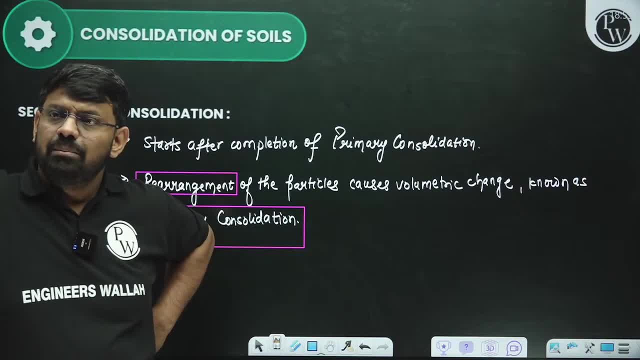 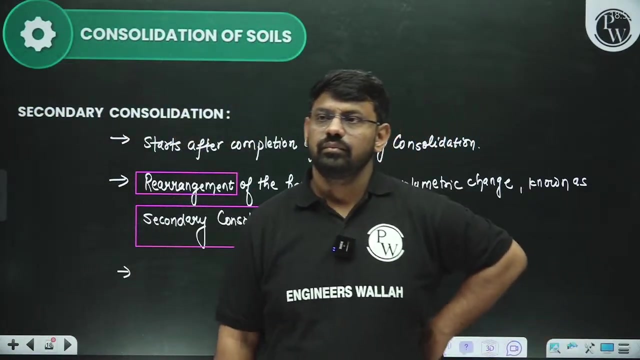 they are telling: cohesion, cohesion, cohesion, cohesion, cohesion, cohesion. That means secondary consolidation, as you are telling. some children are saying: cohesion-less, Look, cohesion, less cohesive, cohesionless, cohesionless, cohesionless, cohesionless. 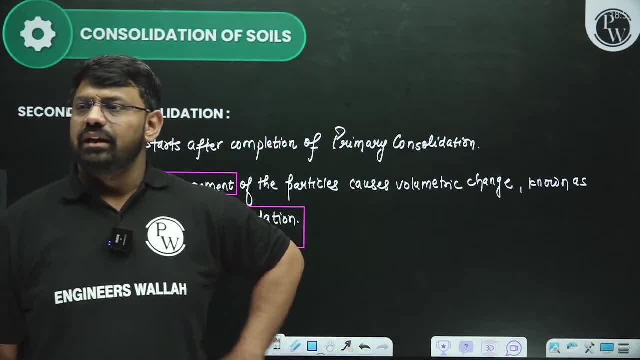 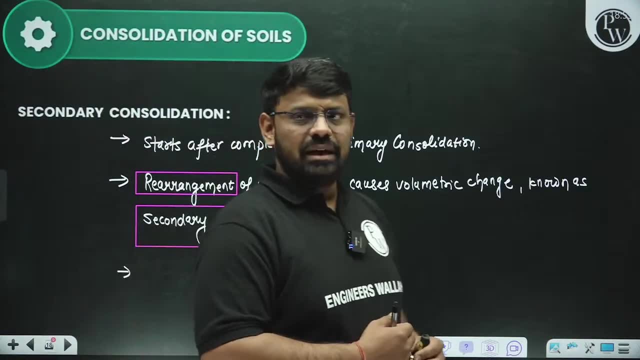 cohesive comigo nothing. no, my child, it is not like that. okay, now you have to understand that here. when we have cohesion-less soil, when you have cohesion-less soil, sir, what will happen in cohesion-less soil, In cohesion-less soil? 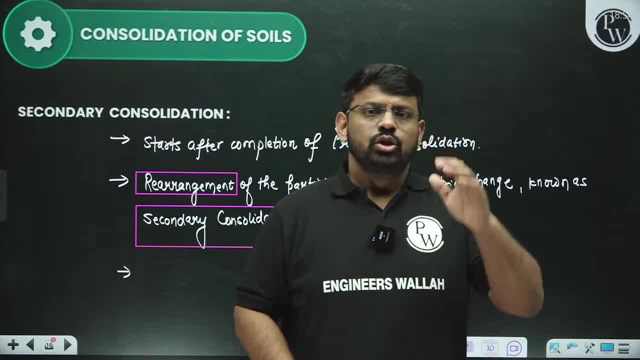 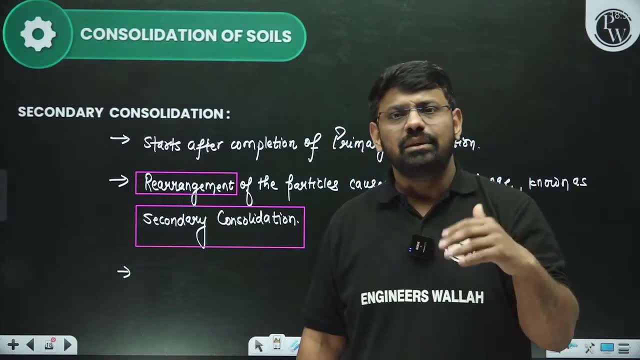 There is no bonding between cohesion-less soil and each other. So when you will load the particle will be very easily there, You will get to see the primary consolidation of that particle there. That means initially only volumetric changes will be observed there. 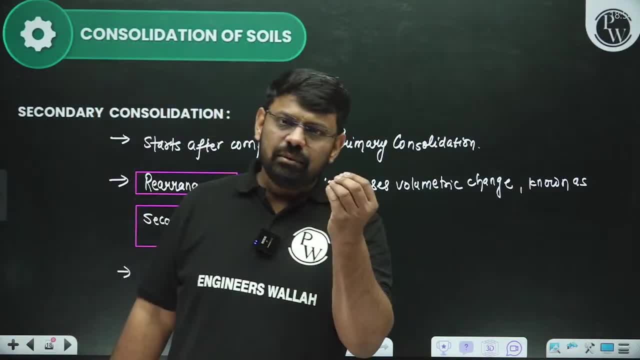 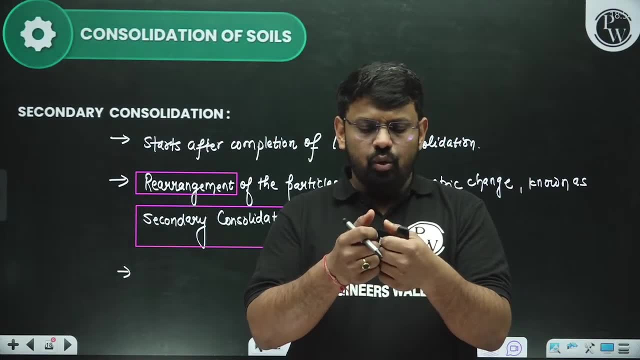 But if you have cohesive soil, then initially when you will load, then you will not get to see the change so quickly there, Because the water that you have, that water will be strongly bonded with the surface of the cohesive soil, Like we have clay particles. 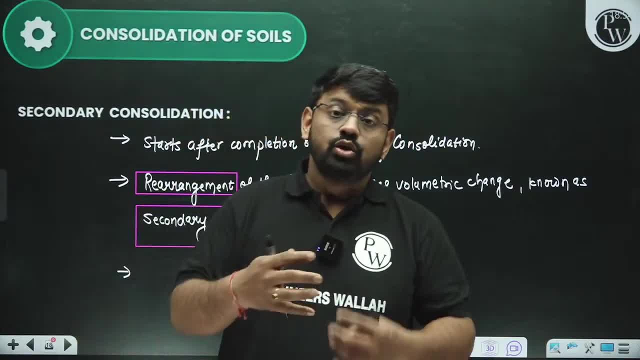 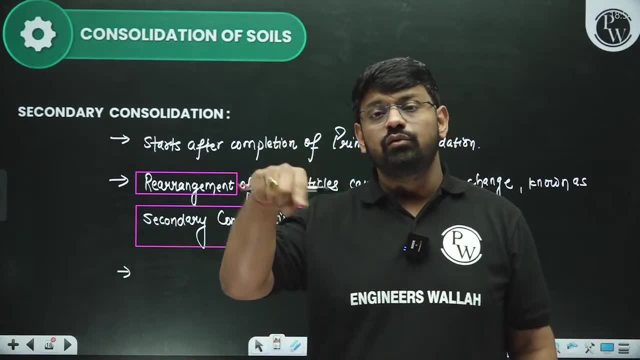 Clay particles are of cohesive nature. They have negative charge on the surface, So the water retention capacity, or bonding capacity, is very good. So it will not let the water come out. So the primary consolidation used to happen due to expulsion of water. So that one we cannot get to see much in cohesive soil. Cohesion-less soil will let the water expel out easily. Cohesive soil will not let the water expel out easily, So the primary consolidation does not happen in cohesive soil. 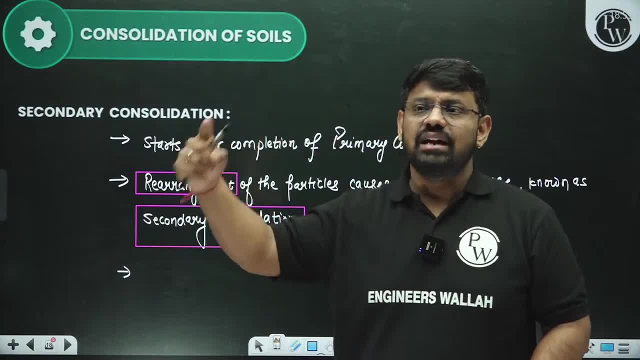 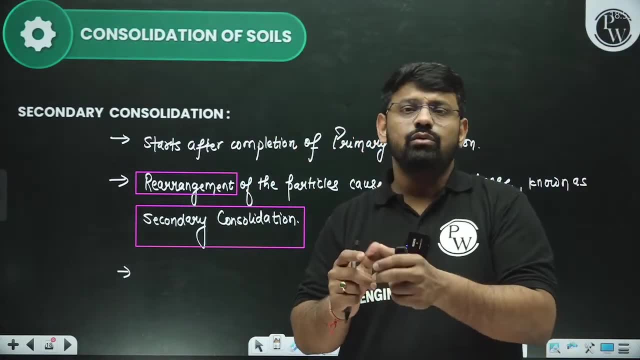 But when the load is there for a long time, it will go on continuously. The load will continue to be applied on it. Then you will see, Sir, when we have cohesive soils, you will get to see that small particle rearrangement in it. 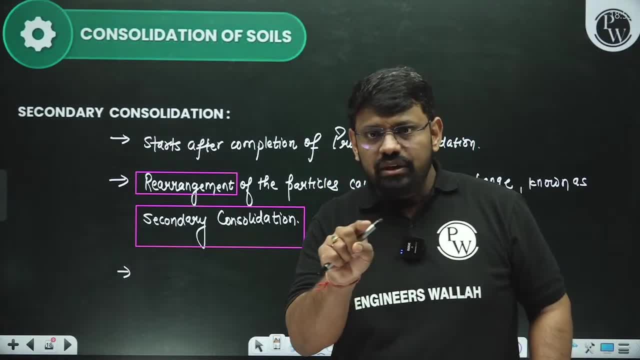 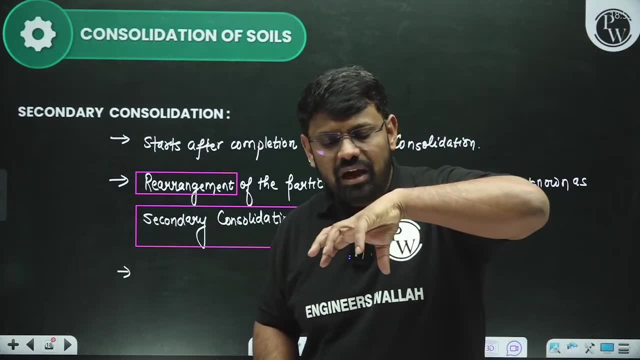 Because the clay around, you get to see the adsorbed surface water, which we call the aqueous layer of water. Because of that aqueous layer of water, the aqueous layer around the particle, you get to see that readjustment. 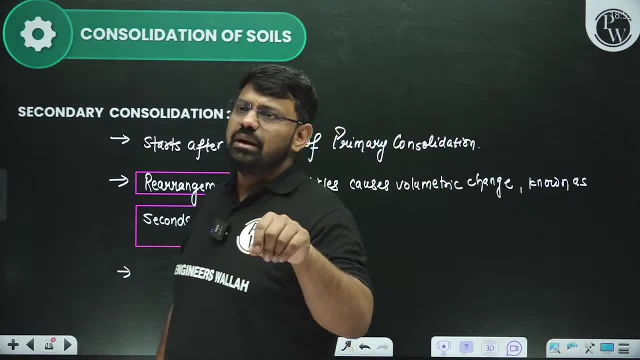 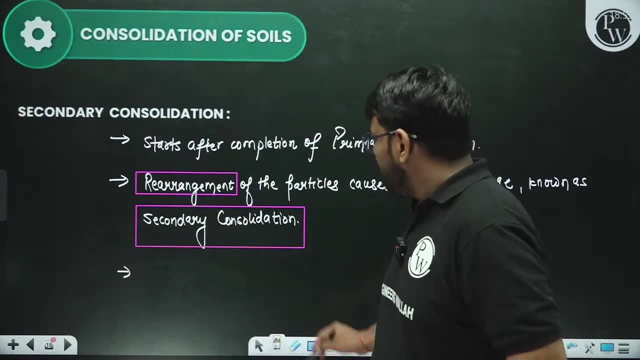 That is why we say, Sir you have particle rearrangement, Sir, you will get to see more in cohesive soils. That means what. That means, Sir, what will happen to us? The secondary consolidation: Sir, we get to see more in cohesive soils. 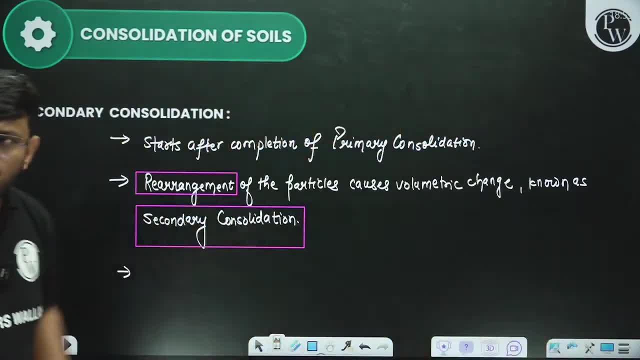 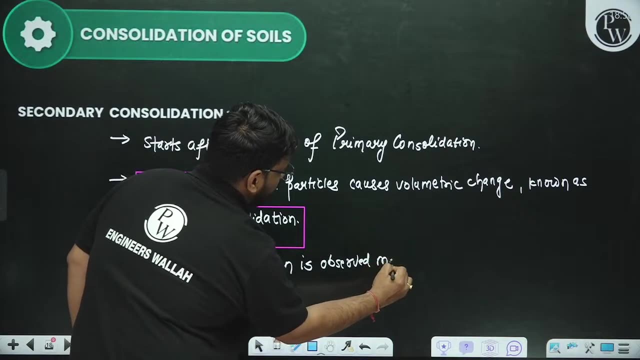 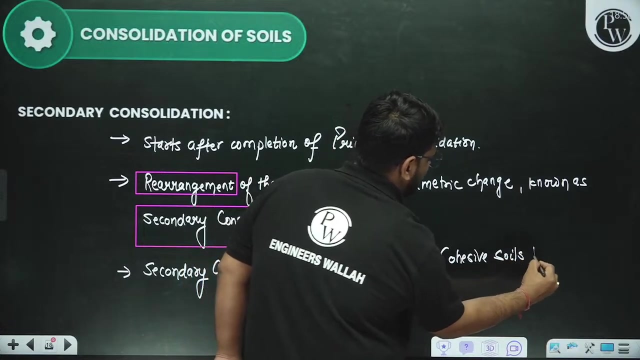 instead of in cohesion-less soils. We have to write this point here also, Sir. secondary consolidation: Sir, secondary consolidation is observed. secondary consolidation is observed more, more in cohesive soils. it is observed more in cohesive soils. cohesive soils, then cohesion-less soil. 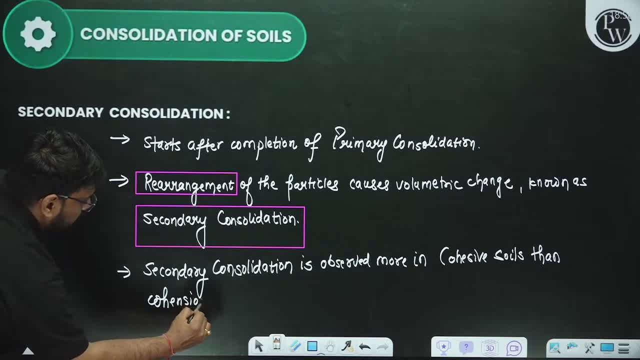 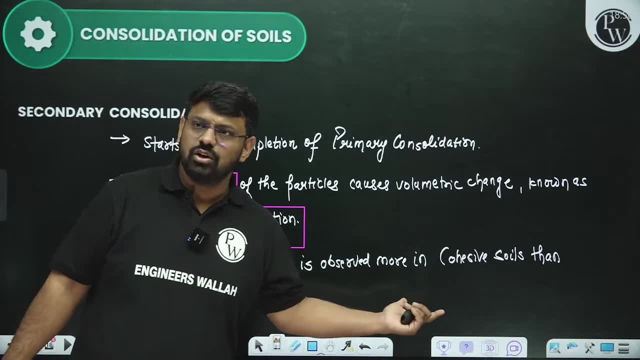 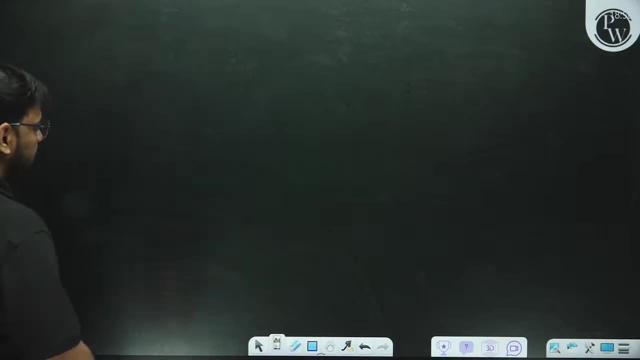 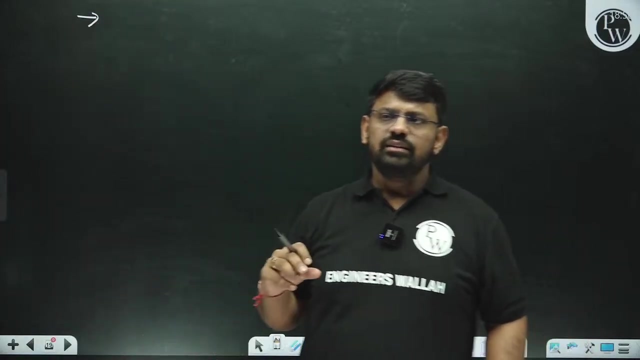 then cohesion-less soil. You will get to see more in cohesive soils instead of in cohesion-less soil. it is absolutely clear. instead of in cohesion-less soil, Sir. keep one more point in mind here, Sir: if you look at the secondary consolidation, then 20% extra is there in cohesive soil. 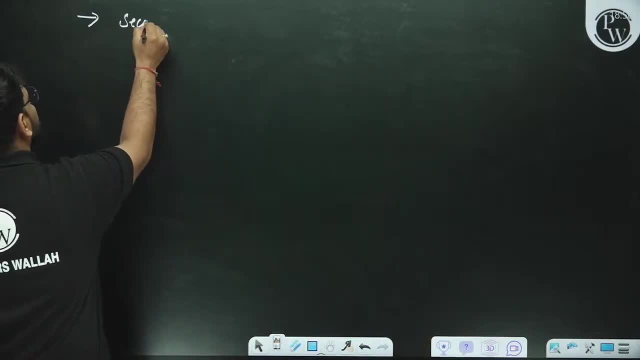 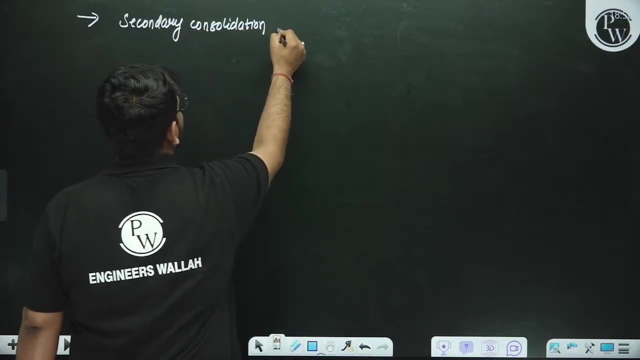 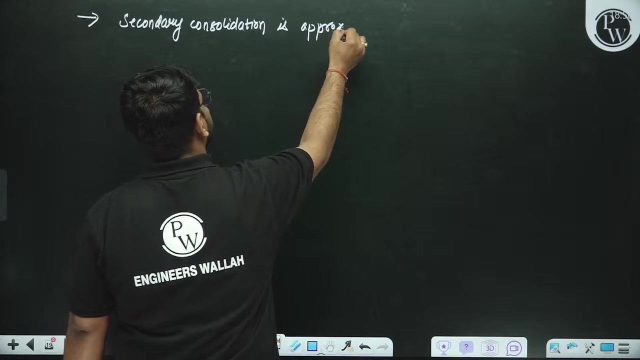 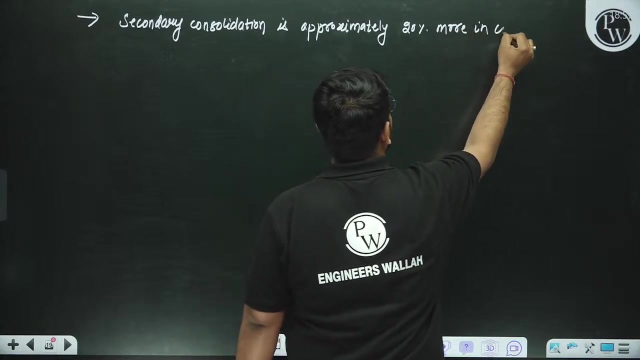 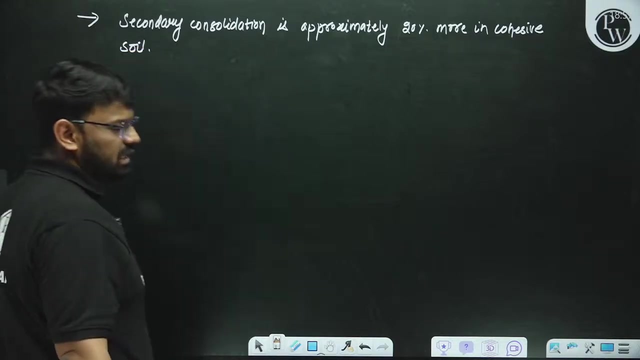 Sir, secondary consolidation is approximately 20% more than cohesive soil. Sir, cohesive soil is approximately 20% more than cohesive soil. Sir, this is what we call 2 degree consolidation. This is known as your 2 degree consolidation, And the settlement that we will get to see here is called secondary settlement. 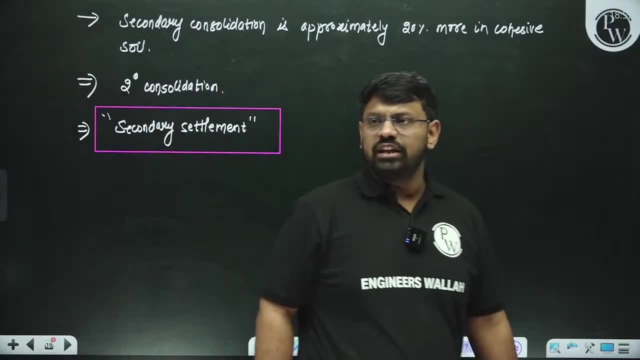 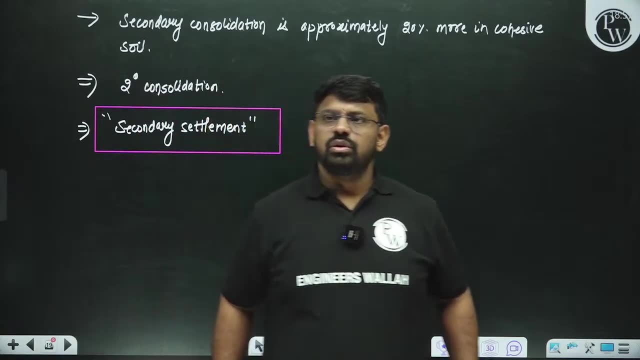 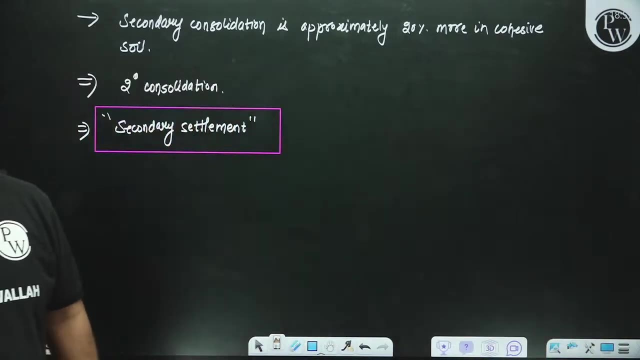 Sir, we call this settlement as secondary settlement. That's what we understood here. This is known as your secondary settlement. This is known as your secondary settlement. Secondary settlement. Sir, you can write in Hindi also. Son, I am not the Viru-Sahasra Buddha that I can write two languages quickly with one hand only. 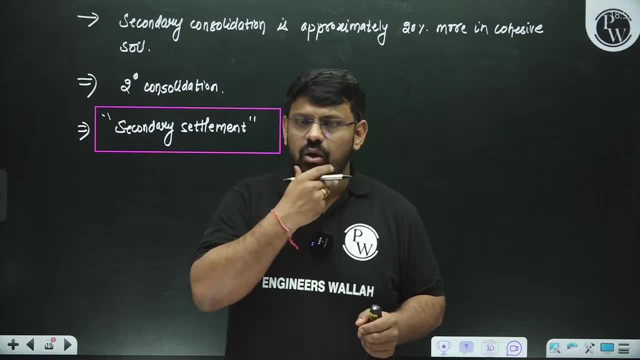 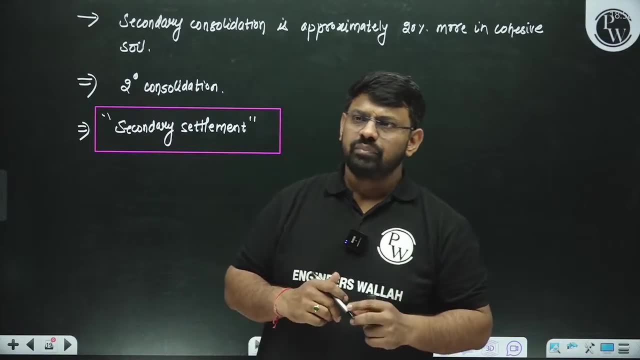 You have to teach consolidation in 2 hours also, And you also need both languages in 2 hours. One thing I work on is that I try to write in Farsi language also. I try to write in different languages too. What I do is with both my hands. 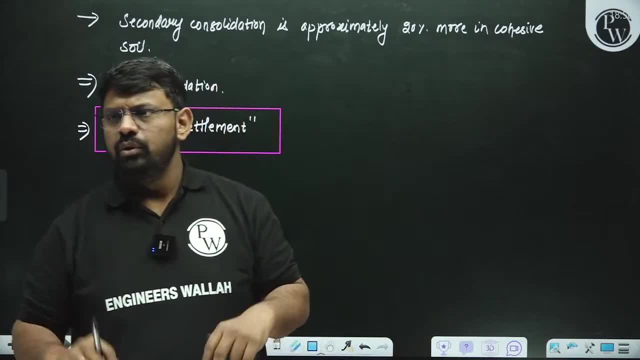 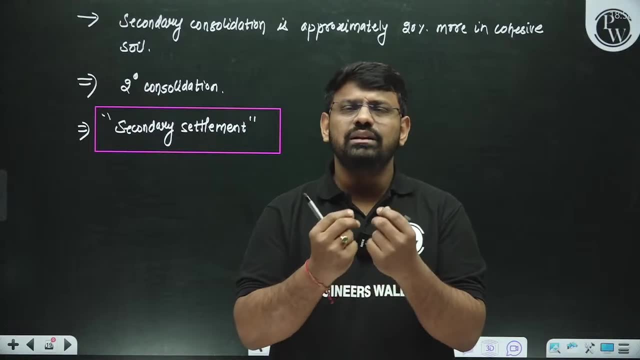 with every finger, I start writing in different languages. Viru Sahastra Budhe. Look, I am able to understand. The serious kid doesn't face all these problems. He doesn't face all these problems. He speaks in a very easy language. 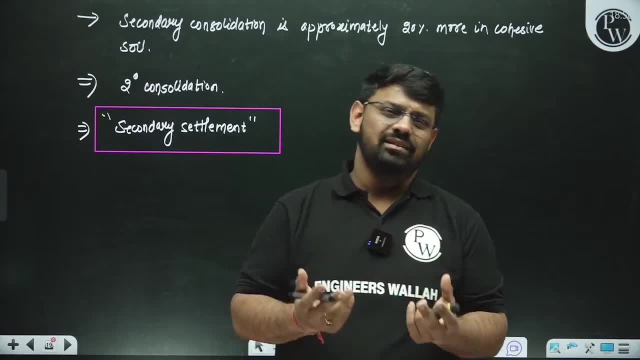 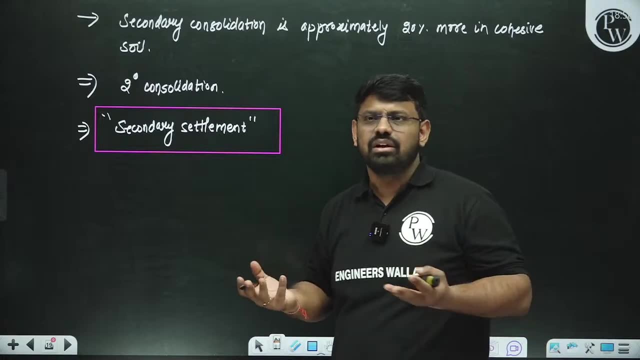 He is explaining things in a simple way, So don't take too much attention to Hindi and English. You are able to understand it very well. What is secondary consolidation? You are able to understand the whole story. When you are able to understand the story, then what is the language barrier? 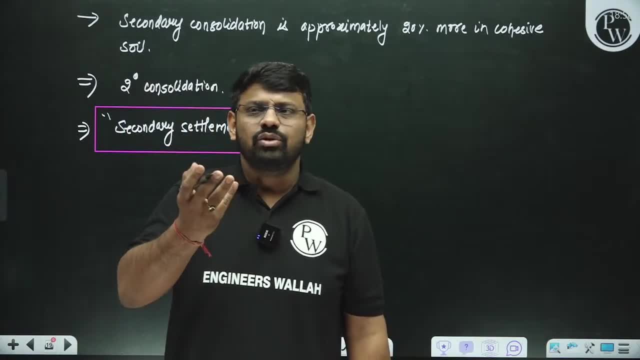 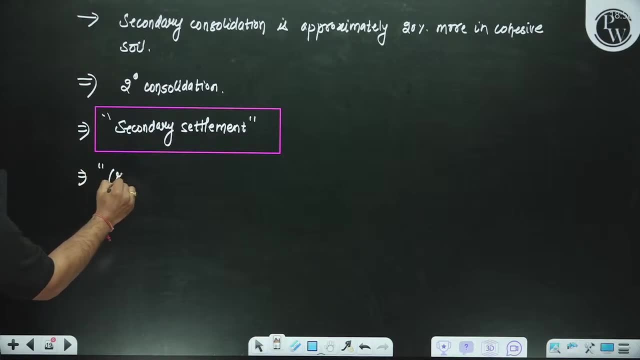 You are able to understand it very well. I have already told you in Hindi: Consolidation, Sanganaan, etc. You are able to understand it very well. Next, we also call it creep. What do we call it? We also call it creep. 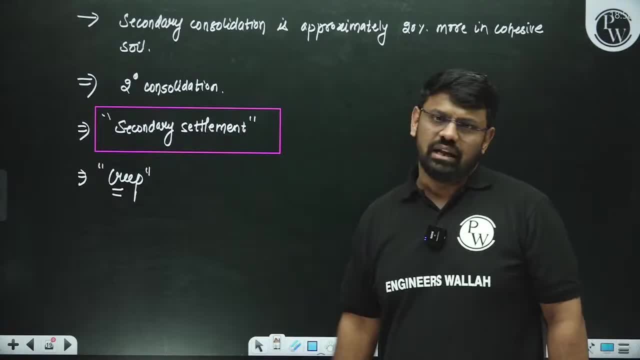 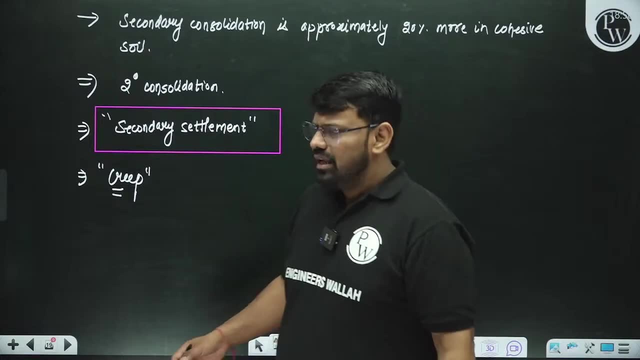 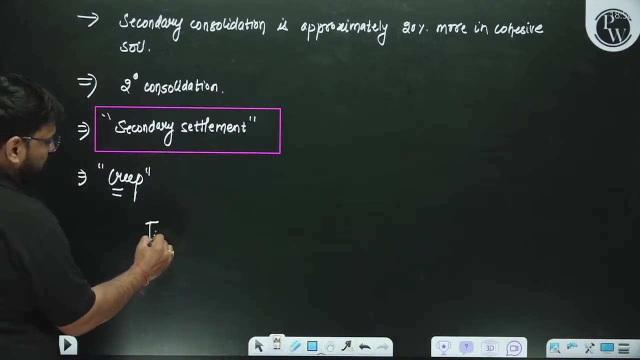 Secondary consolidation. We also call it creep. It is absolutely correct Because of long-term static loading. you are able to understand it very well. You are able to understand it very well. You also read such things in RCC. Further, we have total settlement. 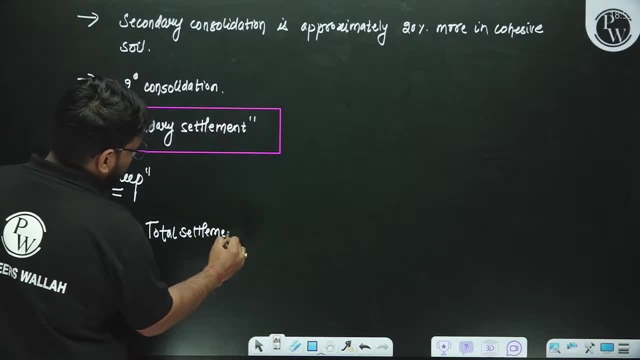 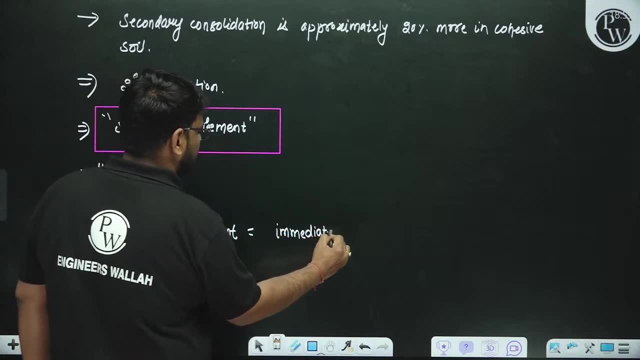 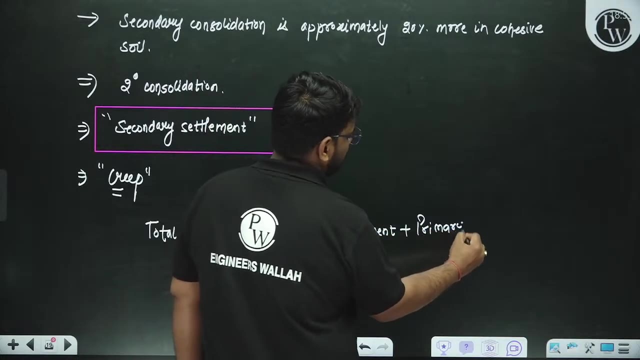 Sir, the total settlement that we get to see. what is that total settlement, Sir? we have total settlement. Now we have understood that you have immediate settlement. Total settlement is nothing but your immediate settlement Plus primary settlement, Plus primary settlement. 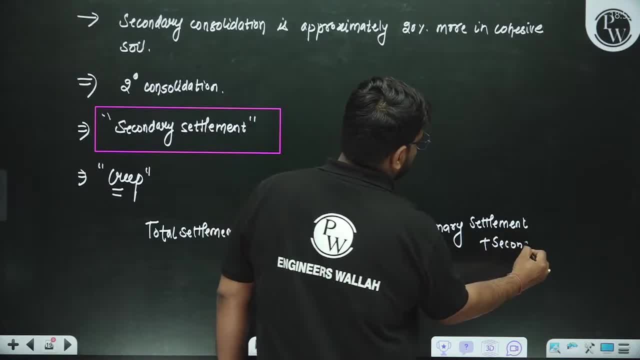 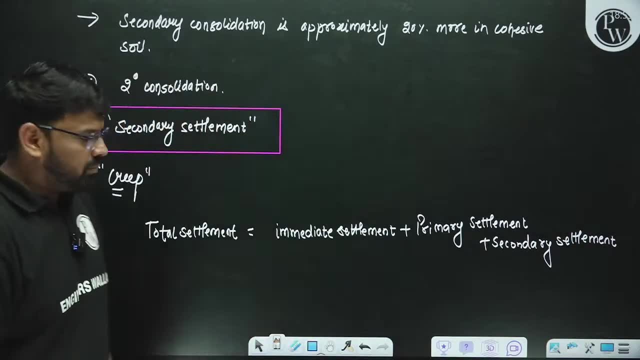 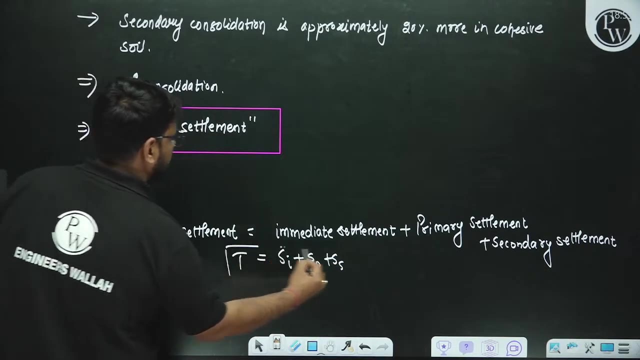 And after that you add secondary settlement. So what do we have, Sir? we have total settlement. This is the total settlement. That means, sir, what happened? That means SI, immediate SP, primary, SS, your secondary. This is your total settlement. 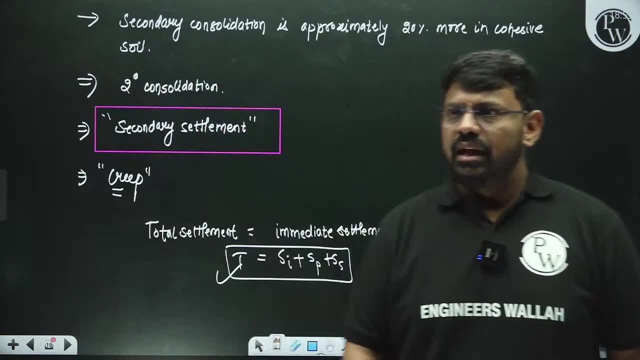 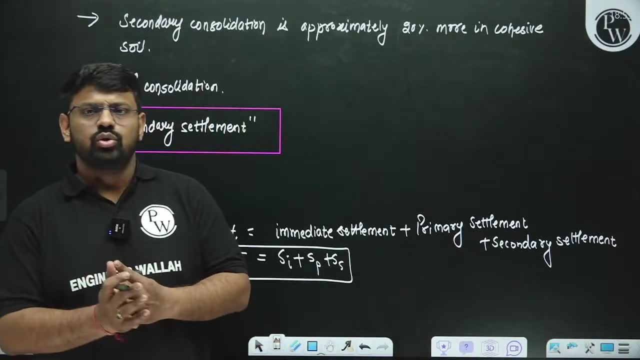 This is your total settlement. It is absolutely clear, sir. So this is your total settlement. You will get to see the criteria here Now. see, sir, further, We will further increase the things further, Sir. the things till here are absolutely clear to us. 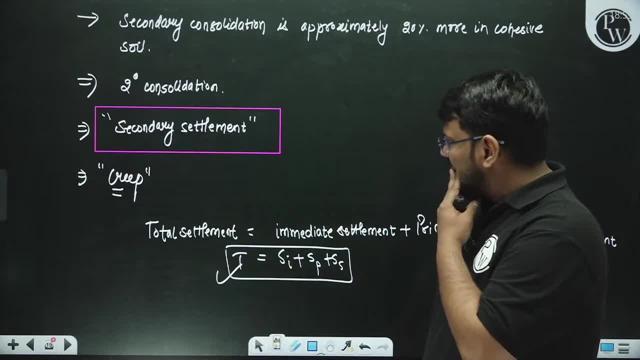 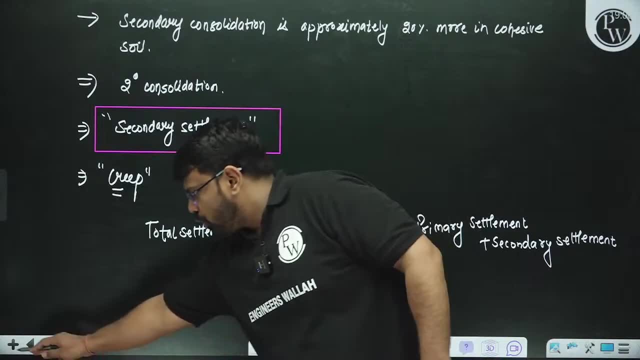 And I am explaining it to you in a very simple language. Okay, Sir, you have understood primary and secondary. Now we will talk about stresses. Okay, Now see, sir, when there is stress on any particular soil, always remember one thing: 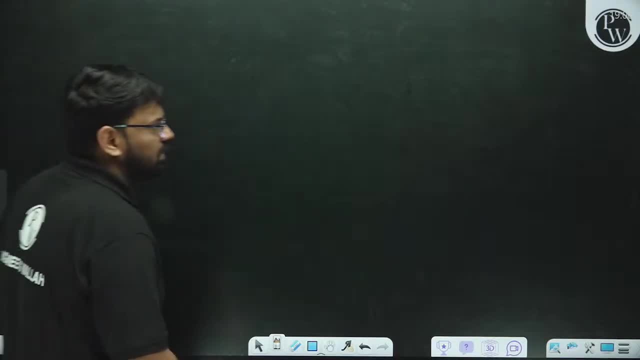 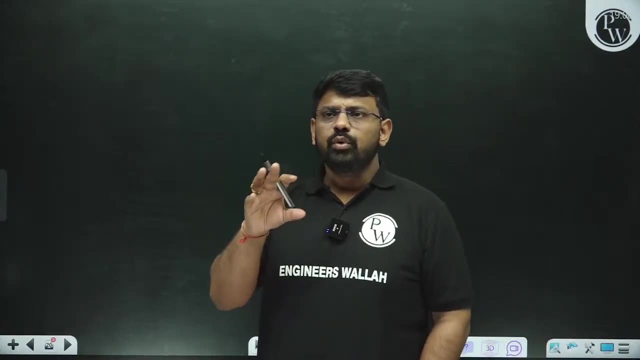 What happened. brother, Always remember one thing here: Whenever we have stress on the soil, whenever we have stress on the soil, whenever we have stress on the soil, then in its entire geological history the soil always remembers the stress. So the soil always remembers the stress. 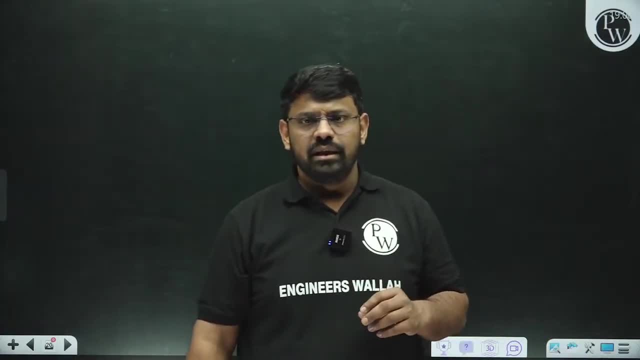 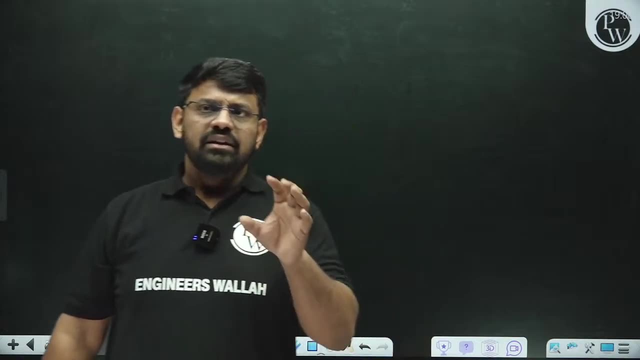 in its geological history. Okay, So in this way you get to see the effect of stresses in a different way. So the first point you have to understand here is that, sir, on any particular soil in its entire history. 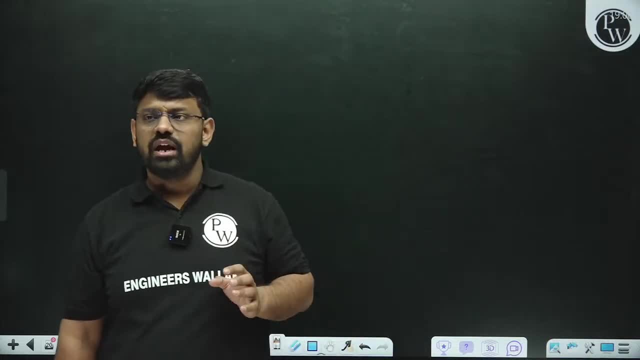 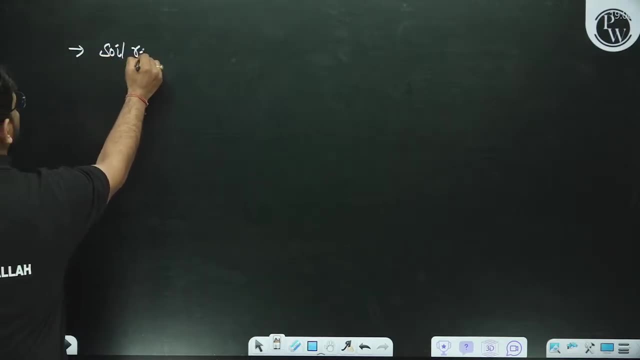 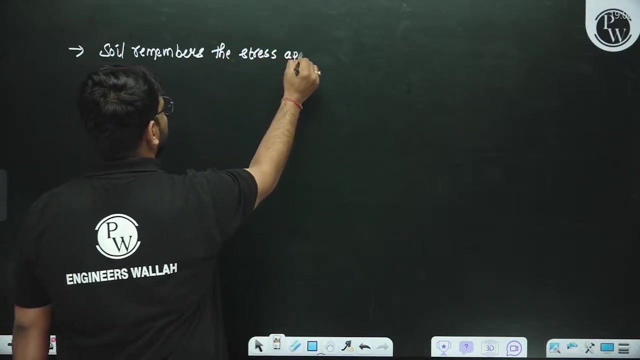 in its entire geological history, the biggest stress that is applied is what we call pre-consolidation stress. The first thing we have to understand here is that, sir, soil remembers, soil remembers. soil remembers the stress applied. soil remembers the stress applied on its. 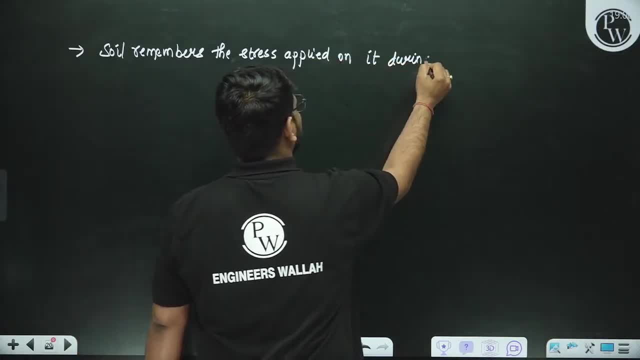 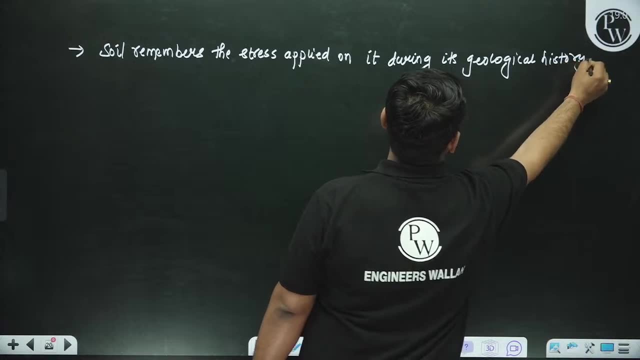 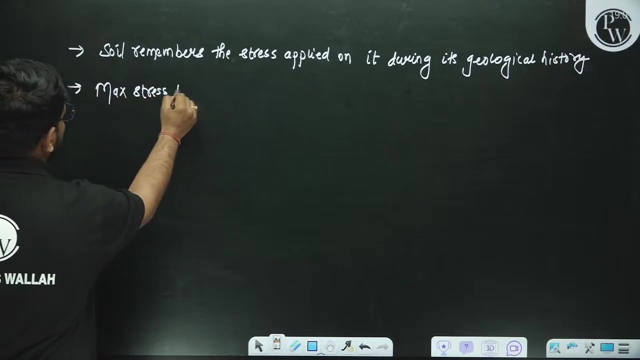 the stress applied on it, on it during during its geological history, during its geological history. Sir, this is the first thing we have to understand. The second thing to understand here is that the maximum maximum stress, maximum stress that is applied on the soil mass, 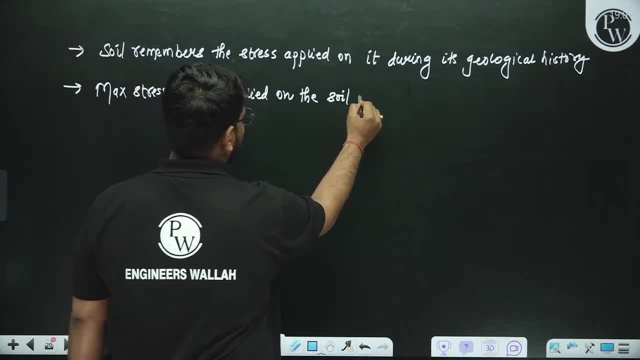 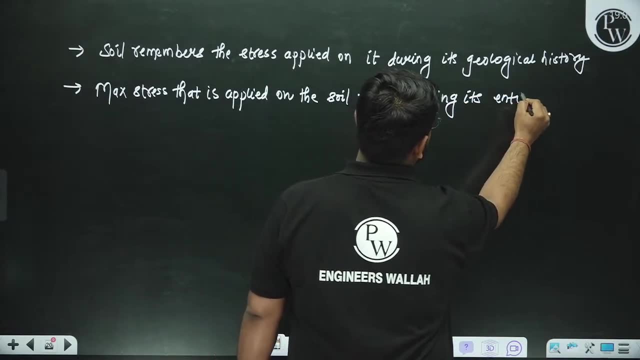 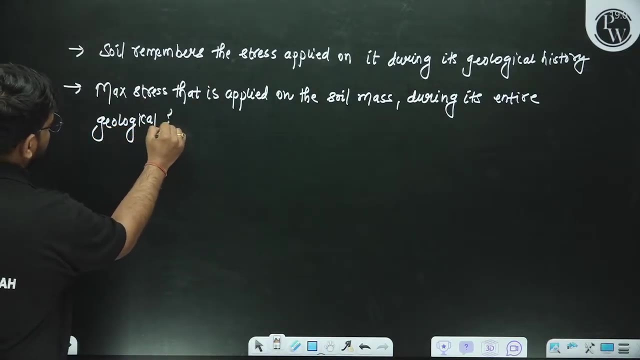 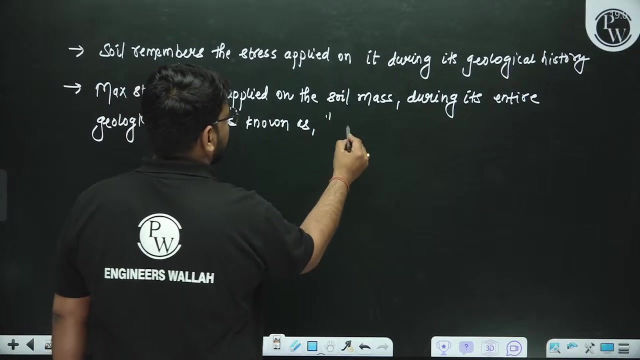 that is applied on the, that is applied on the soil mass, during its during its entire geological history, during its entire, during its entire geological history, is known as. what do we call this stress- We have to understand this too, sir- is known as your. 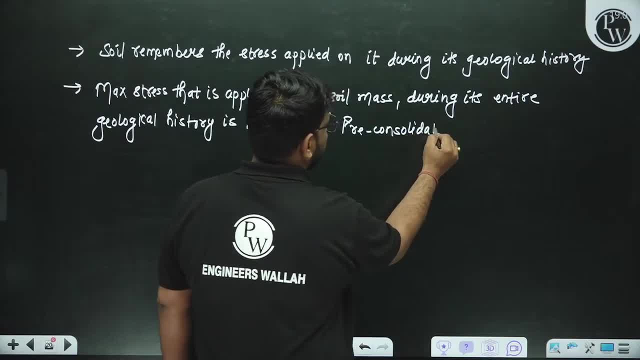 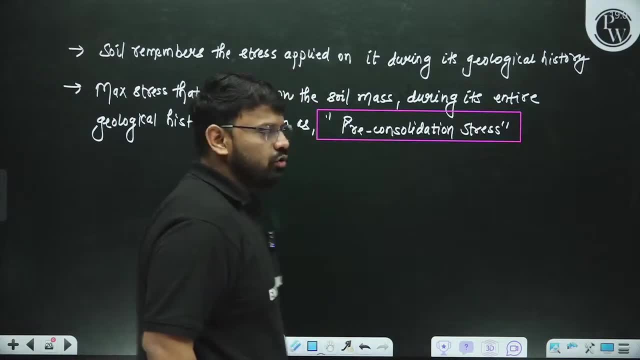 pre-consolidation stress is known as your pre-consolidation stress. Sir, this is what we call pre-consolidation stress. This is known as your pre-consolidation stress. Okay, Which you will represent with sigma c. sigma c bar. 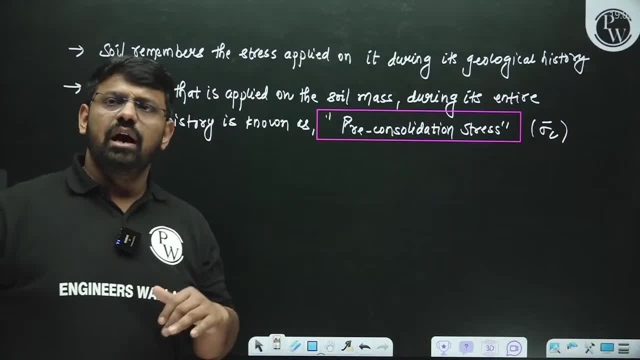 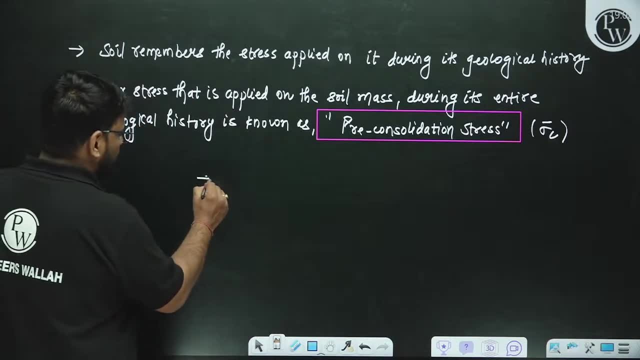 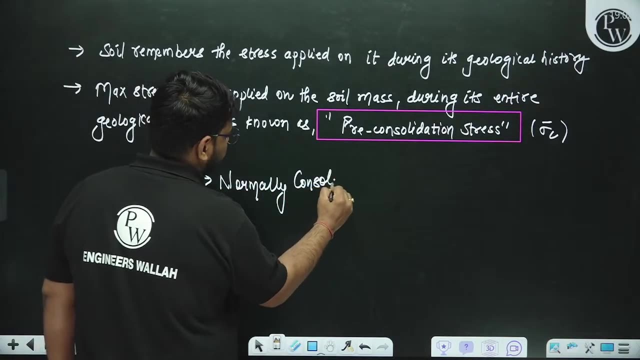 This is pre-consolidation stress. Now, on the basis of this, we divide the soil into different parts, Like we give it different names, sir. Sir, we have: one is normally consolidated clay, Meaning one is normally consolidated soils. 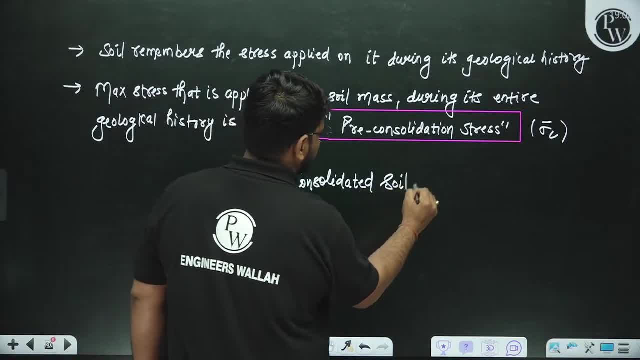 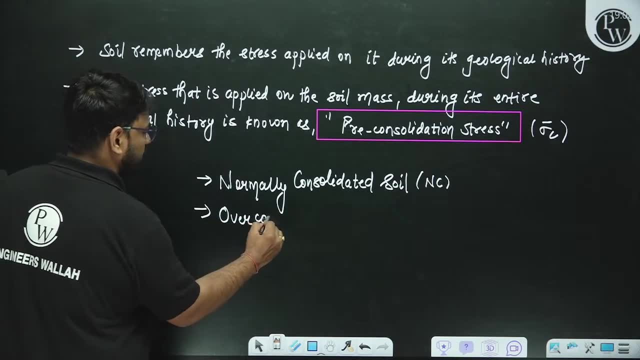 Normally consolidated soils, Meaning NC soil, sir. This is the first thing, Sir. second, we have over consolidated soil, Which one Over consolidated soils? Over means OC, sir. And the third: we have, sir, under consolidated soils, What kind of? 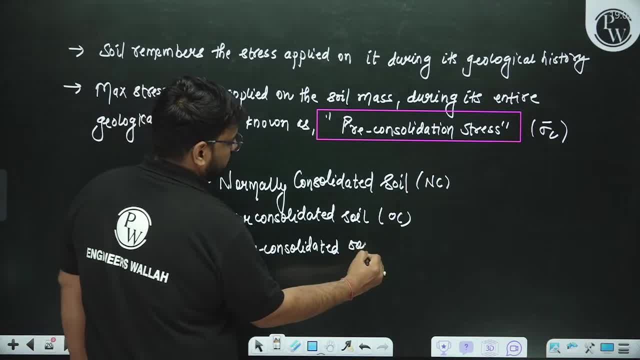 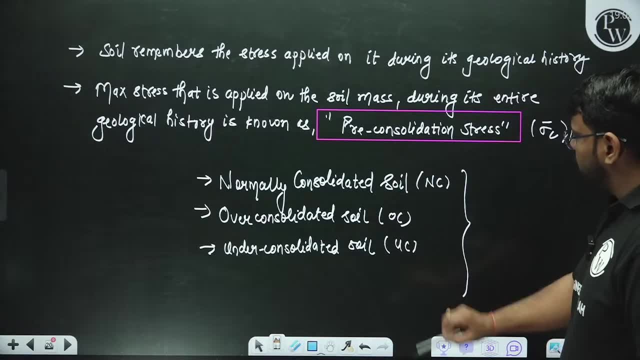 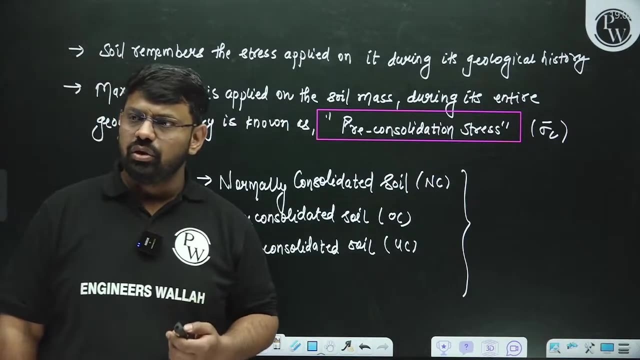 soil Under consolidated soils. And this we have, sir: UC Under consolidated soil. Okay, Now this too, their definition can be asked to you in the exam, Sir: what all things we have normally consolidated over consolidated or under consolidated soils. 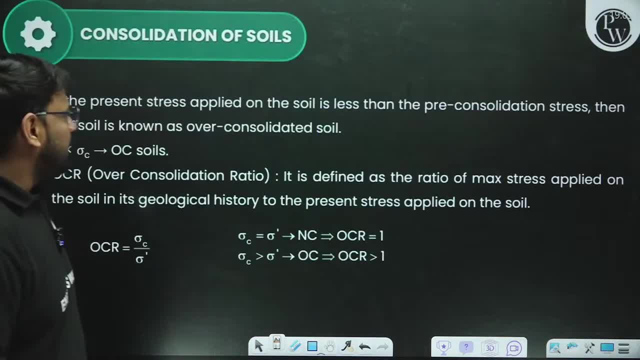 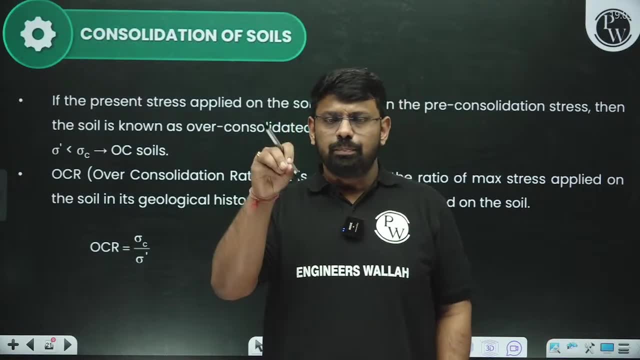 what kind of Sir? the first thing that comes here is that if we have, at any particular time, at any particular soil, if the present stress is applied, meaning I believe that, sir, we have a soil mass Now, on this soil mass, 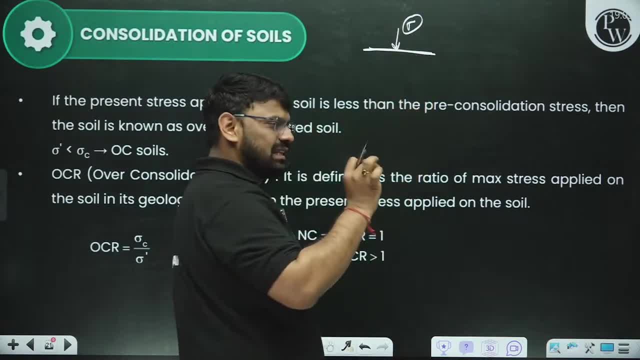 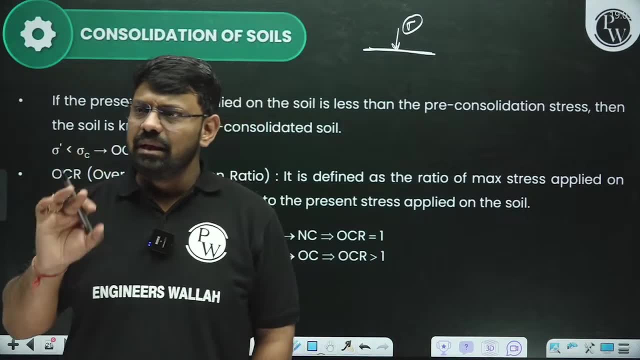 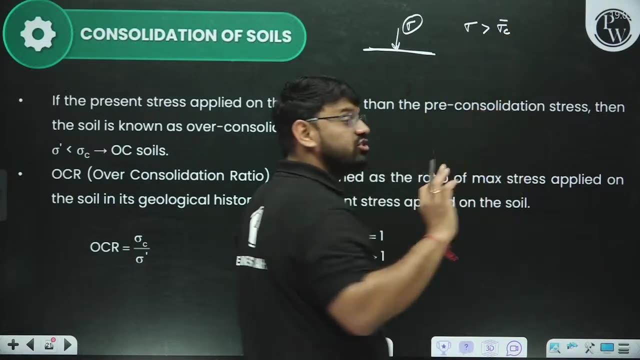 in the present we have a sigma stress. If this present stress, you have the biggest stress applied in the history of the soil, Meaning sir, meaning sir, if the present stress applied to us is greater than the pre-consolidation stress. 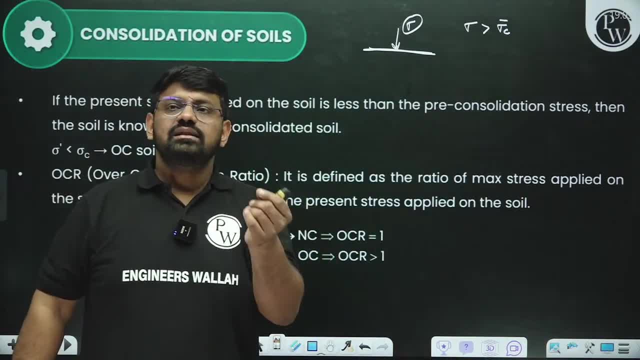 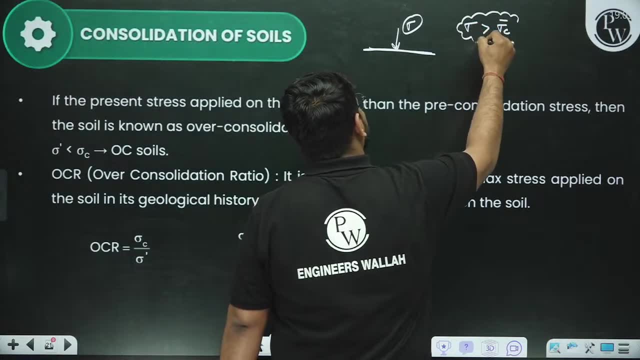 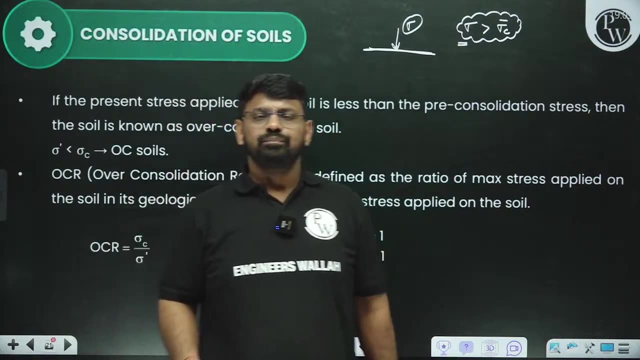 if it is more than the pre-consolidation stress, then this type of soil is called normally consolidated soil. Then what is this type of soil called, sir, Normally consolidated soil? Meaning present stress when it is more than the biggest stress applied to a soil, or 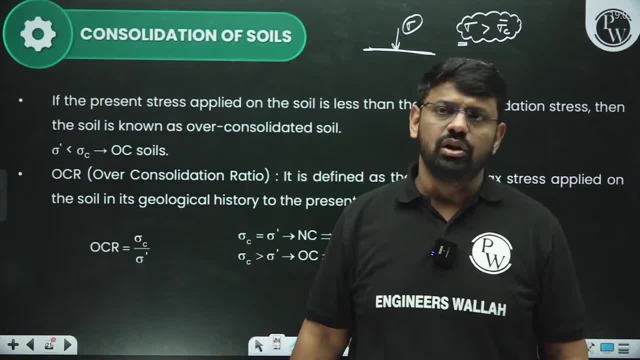 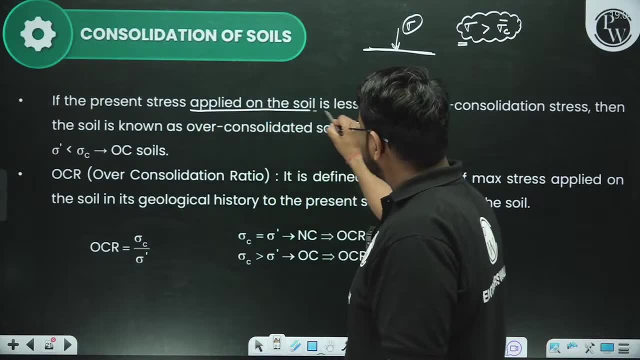 you can say when the present stress is maximum on a particular soil. what is it called, sir? It is called normally consolidated soil. So see, if the present stress applied on the soil is less than the pre-consolidation stress, then 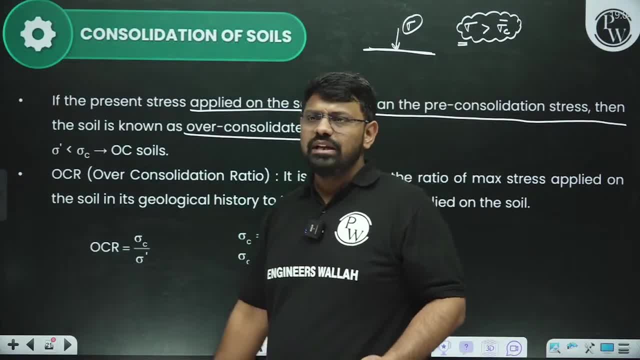 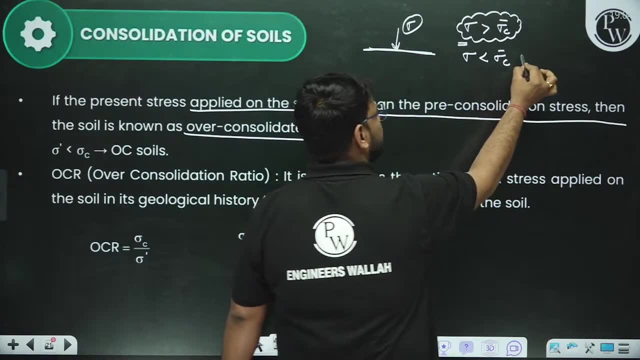 it is known as your over-consolidation. So it is over-consolidated, and normally consolidated means that it is more. So if we have present stress from pre-consolidation, then it is called over-consolidated. So this sir. 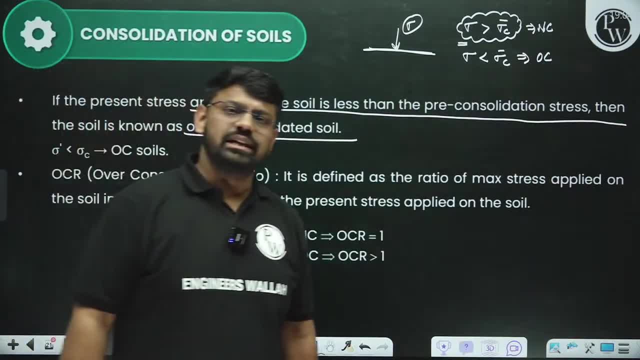 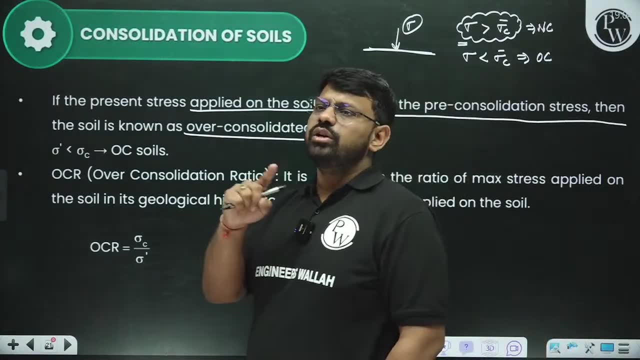 is normally consolidated and the other is over-consolidated. Now understand one more thing, sir. We try to understand this with a ratio, with an analogy, which we call over-consolidation ratio, meaning OCR. So when I talk about 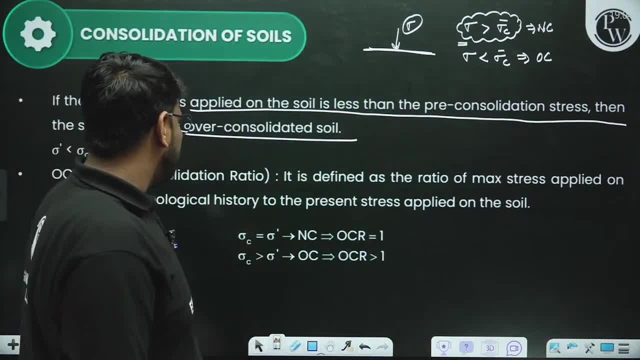 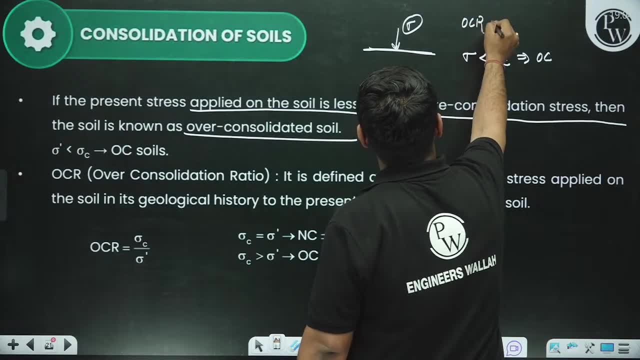 normally consolidated soils. then, sir, in normally consolidated soils, understand one thing here. understand one thing here: in normally consolidated soils, your over-consolidation ratio will be 1, meaning when the present stress is equal to your maximum stress, which is 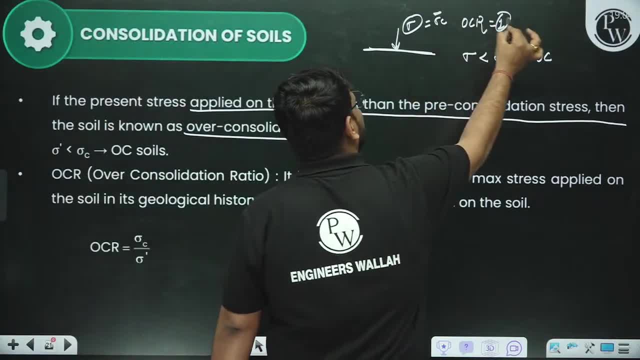 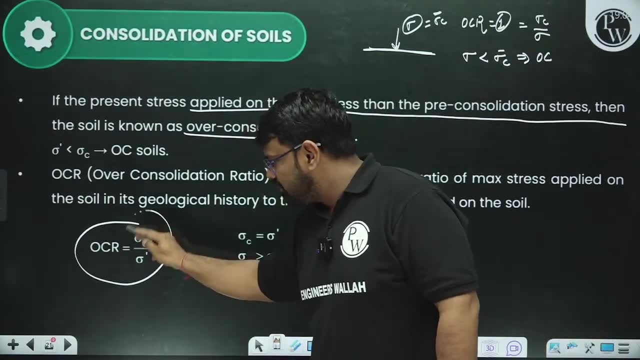 on a particular soil. both will be equal to each other. That means, sir, the ratio of sigma C by sigma, which we call OCR, that is the ratio of sigma C by sigma. both of them are equal. This means we can say: 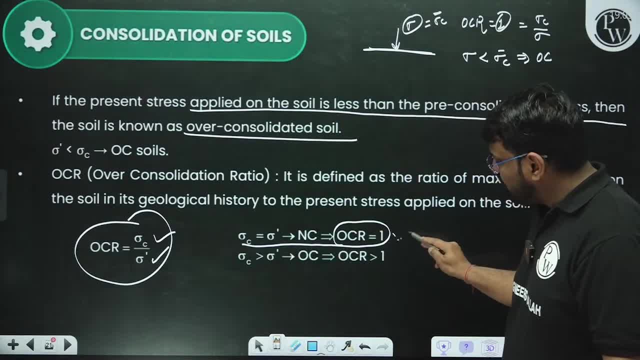 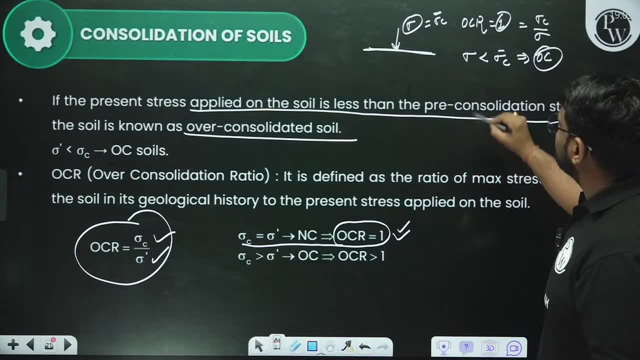 sigma C is equal to sigma 1, then our over-consolidation ratio becomes 1.. But if I am talking about over-consolidated soils where the present stress is less than the previous stress, then when the present stress is less than the previous stress. 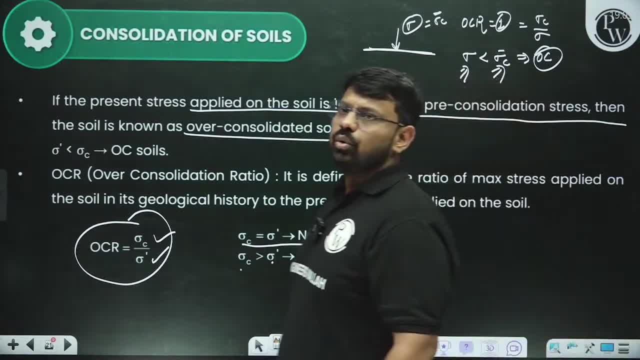 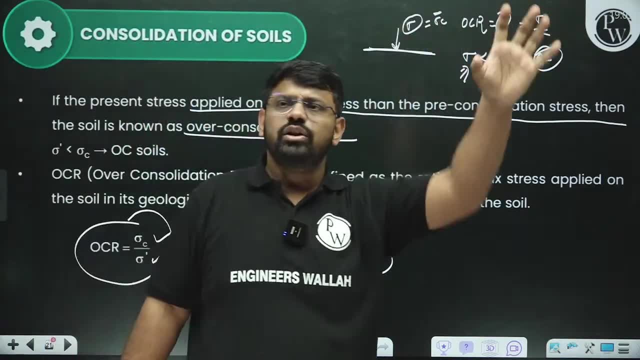 then OCR will also be greater than 1.. So when OCR is greater than 1, then it will be called over-consolidated soil. When OCR is equal to 1, then it will be called normally consolidated soil. When OCR is less than 1,. 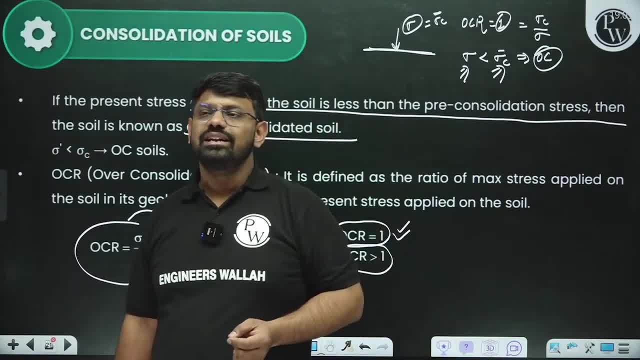 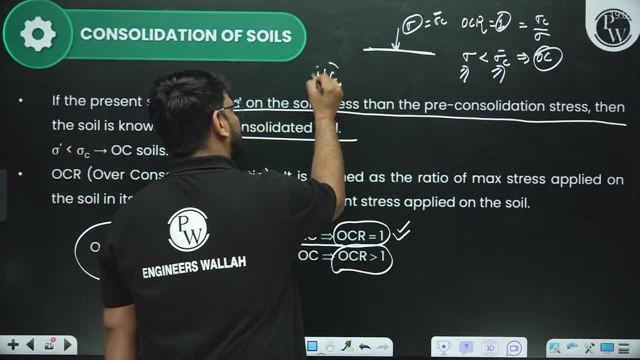 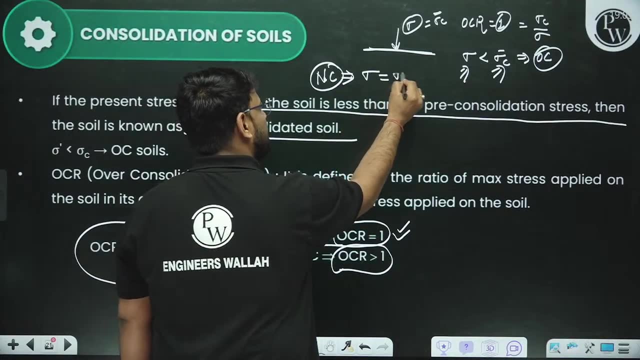 then it will be called under-consolidated soil. It is absolutely clear. So to understand this, sir, in normally consolidated soils, in normally consolidated soils, you have to keep one thing in mind: the present stress is your maximum. And what is the maximum? 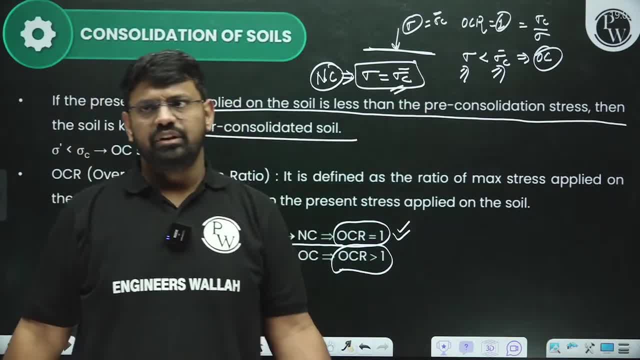 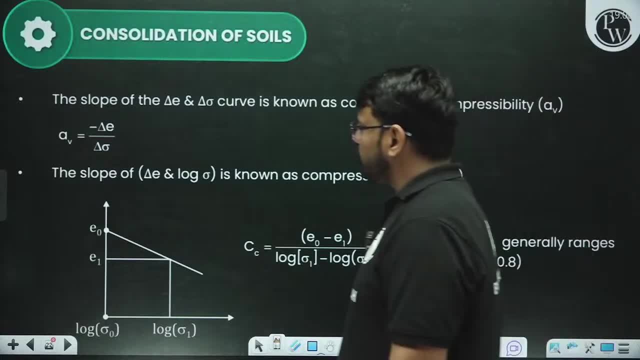 The maximum is your pre-consolidation stress. Okay, sir, This is the biggest part of your stress, which is clear, And this question is asked again and again. Now, sir, look here whenever we make changes in the void ratio. 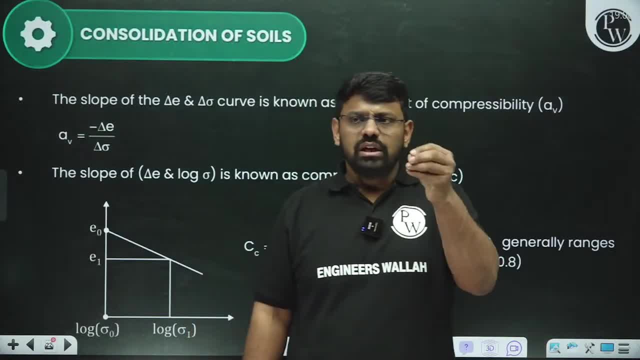 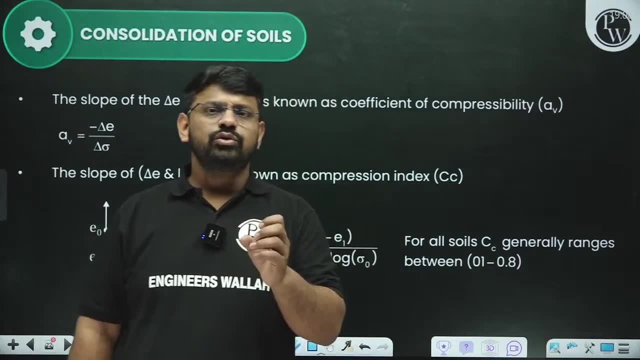 see whenever we talk about a particular soil, then when we put a load on the soil and we try to see the changes in its volume, then, sir, if there will be changes in the volume, then definitely there will be changes in its void ratio as well. 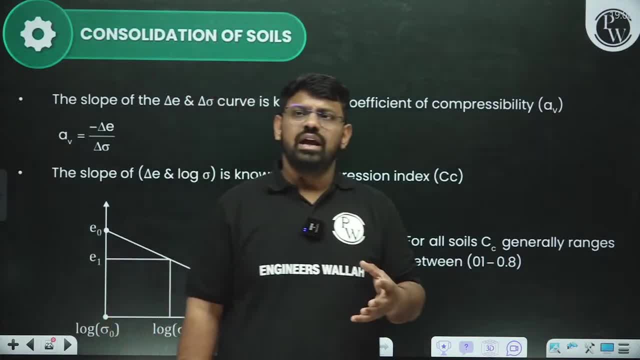 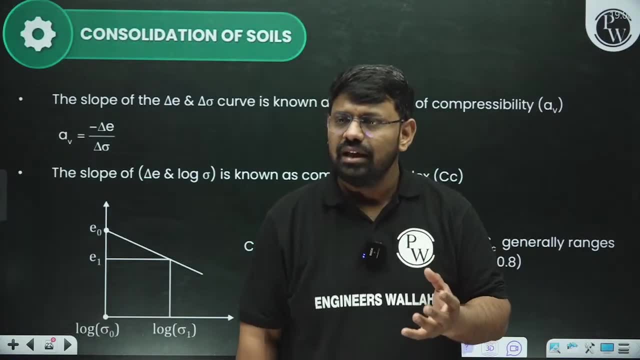 So what do we do, Sir? how much has changed in stress Based on that? how much has changed in the void ratio? How much has changed in stress? Satyendra Karadang says: repeat, sir. Hey son, what do you have to repeat? 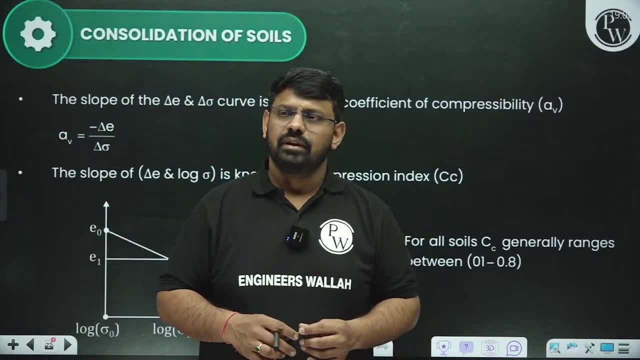 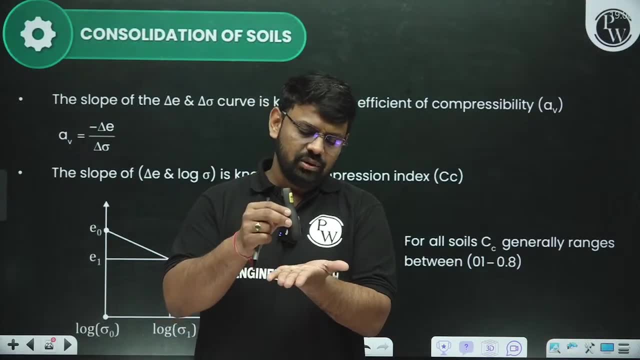 What do you have to repeat? Tell me quickly What did I say? NC soil? Okay, fine, If we talk about NC soil, then this is your present stress. This is the maximum stress on the soil. So if this is equal to the maximum stress, 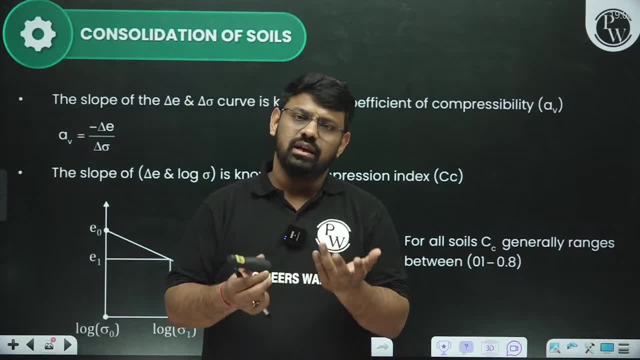 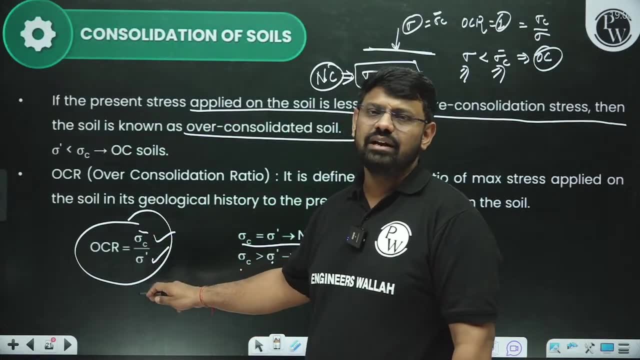 then we call it NC soil. If it is less, then we call it OC soil. Okay, What does OCR have? OCR has: sigma C means maximum stress divided by the present stress. This is OCR. This is called over consolidation ratio. 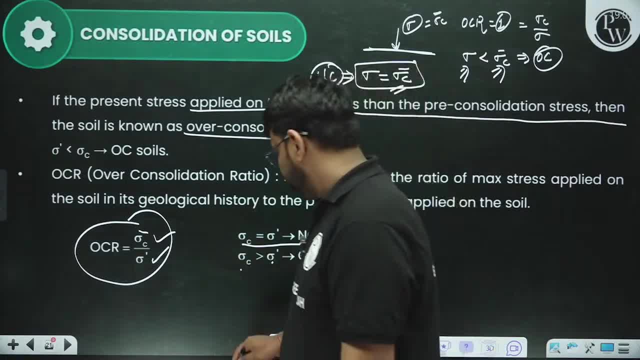 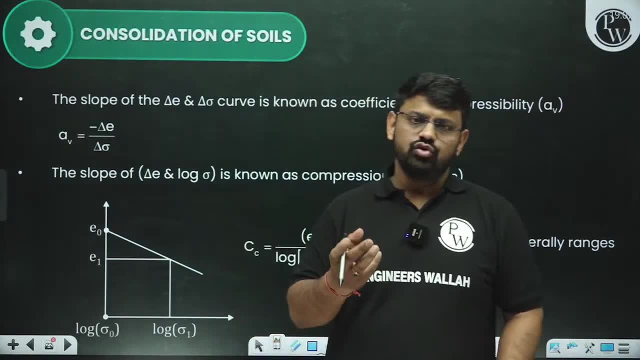 What do we call it, son? It is called over consolidation ratio. Okay, fine, Now look ahead, sir. What is next? sir, Next, as I told you, we have void ratio, So we will get to see change in void ratio. 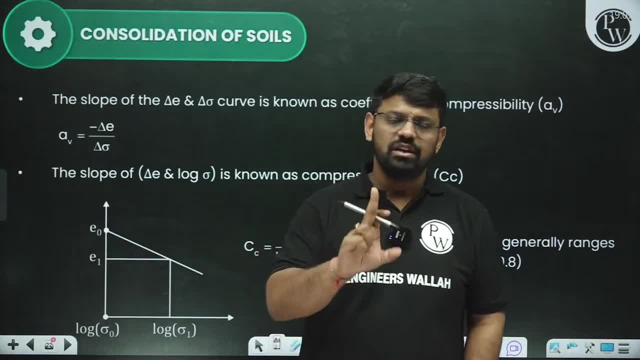 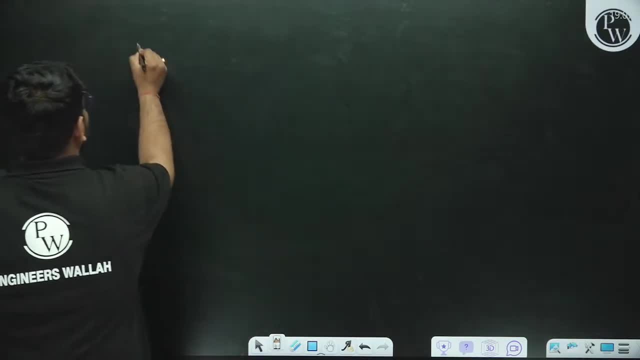 We will get to see change in void ratio And we will also get to see change in stress, Absolutely right. So let's make a graph between stress and void ratio. So, sir, in this graph between stress and void ratio, 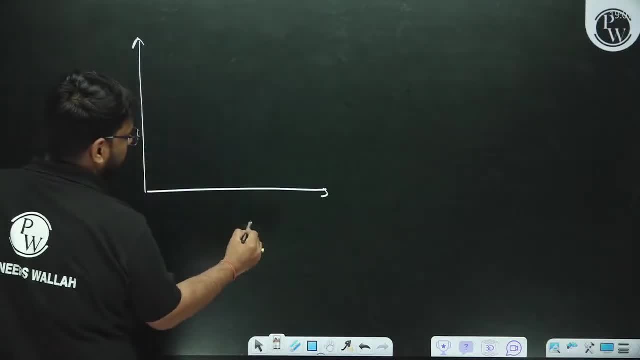 see what will happen, sir, What you do from here, sir, this is void ratio. This is your change in stress. This is your change in stress. Okay, You make this graph in this way. Okay, You make this graph in this way. 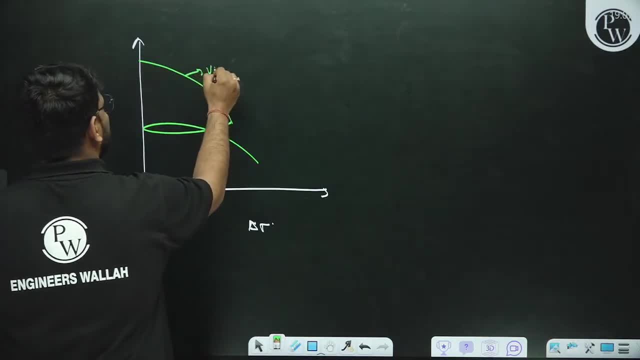 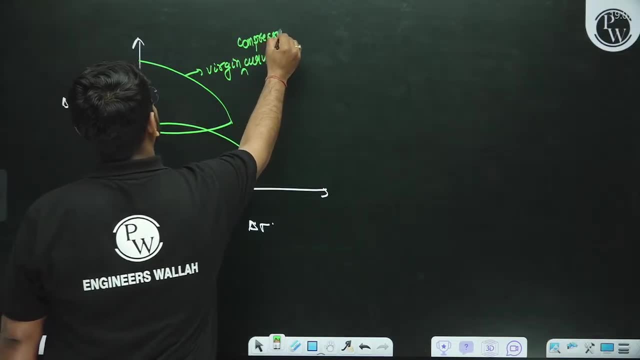 So, sir, here we have the convex shape of this graph. This is known as your virgin curve. This is your virgin compression curve. This is your virgin compression curve. This is your virgin compression curve. We get to see swelling here. When we get to see swelling. 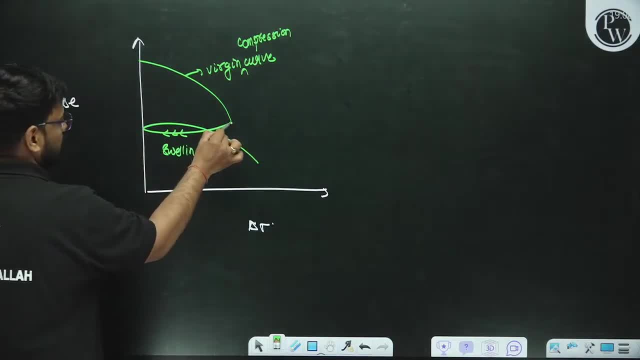 the void will increase. The volume will also increase. here We get to see swelling, We get to see loading. This is a graph for reloading. So what do we do with this, sir? When we take out the slope, we call this slope. 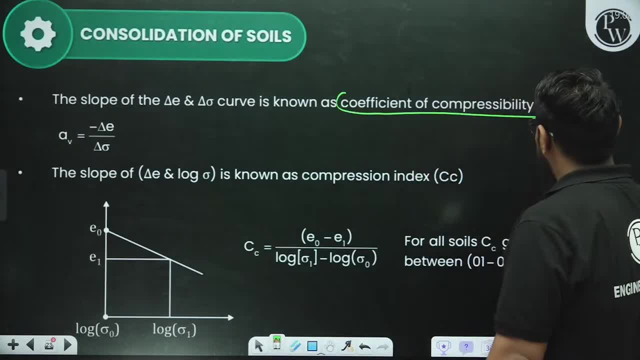 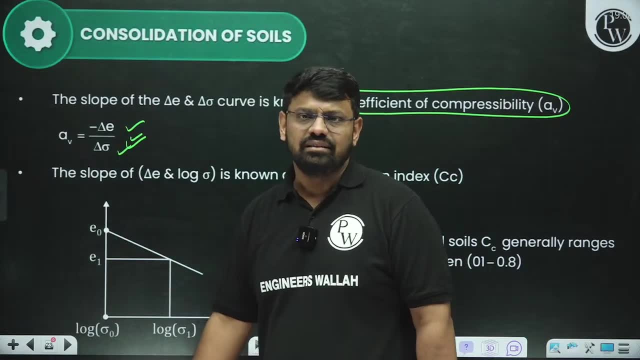 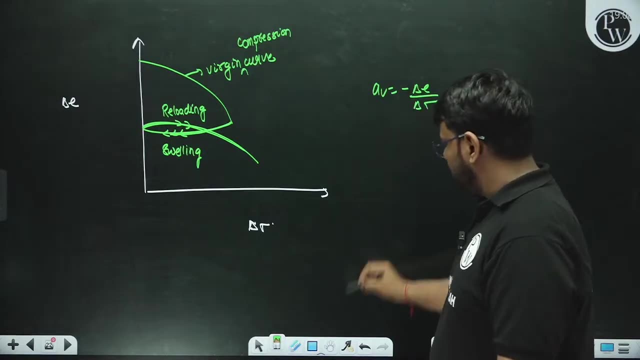 coefficient of compressibility. This slope is called AV. AV means coefficient of compressibility, which is nothing but your minus delta E divided by delta sigma. So the slope of this graph is called coefficient of compressibility, which is nothing but your delta E by delta sigma. 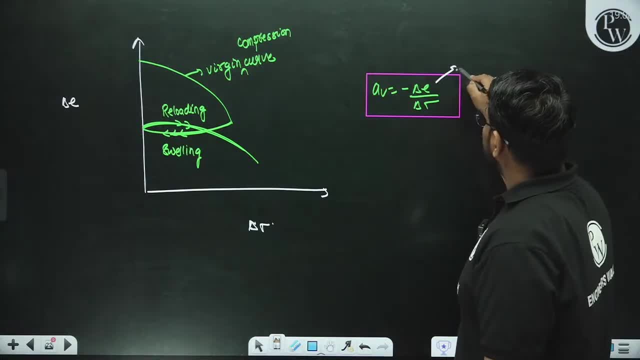 And here, sir, what will happen to delta E? Delta E will happen to us: change in void ratio. So, sir, this is basically your change in void ratio And this will happen to us, sir, when we get to see change in stress. 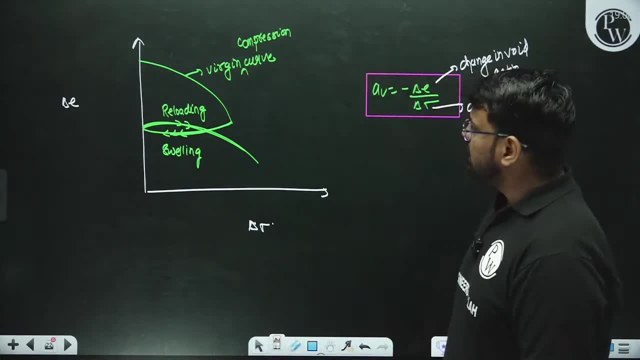 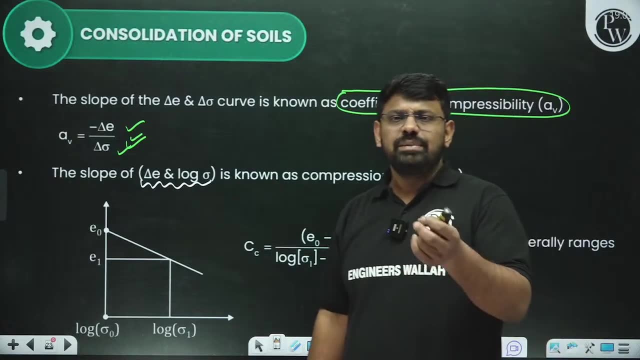 When we get to see change in stress. Absolutely, sir. Now, sir, here delta E and delta sigma are there. If you make this graph in delta E and log sigma, then whenever you put the log, we know that the curvature of the graph is very high. 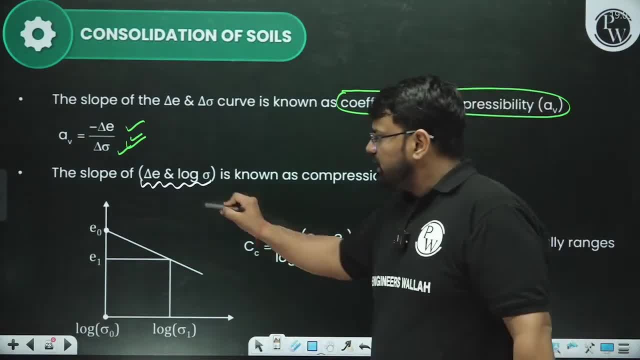 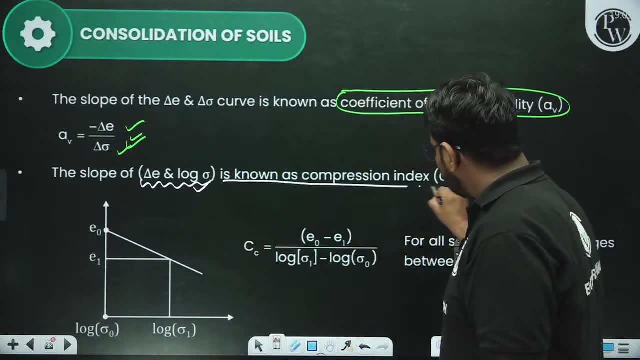 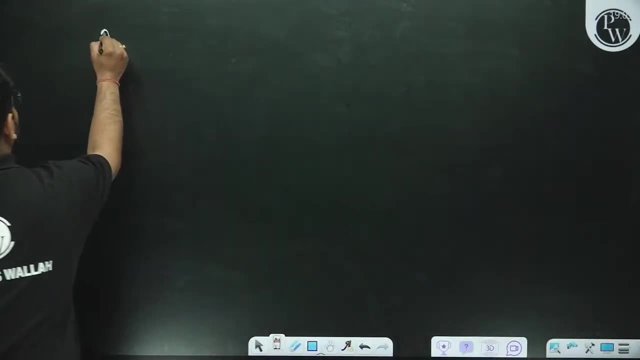 Because if you put the log, then you can accumulate more data on a particular graph. So when you make a graph between delta E and log sigma, then we have this known as your compression index. What do we call this, sir? We call this compression index. 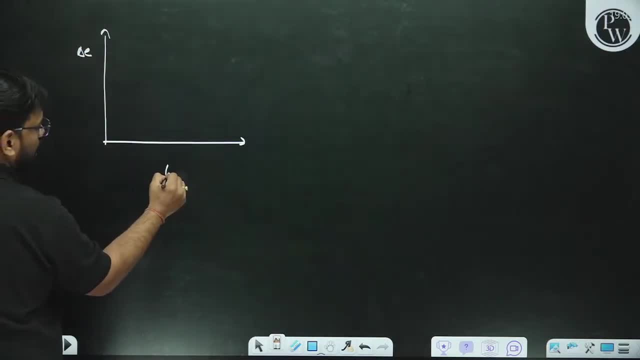 So what did you do, sir? If you made a graph here and we got a graph of delta E and log sigma, then, sir, it becomes a line And the slope of this line, slope of this line slope is known as: 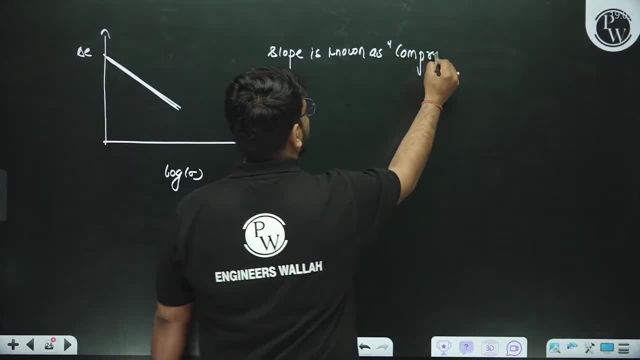 what do we call this slope, sir? We call this slope compression index. We call this slope compression index, Means. we are representing it with cc. This is called, cc means compression index. Now look here, sir Means, sir. 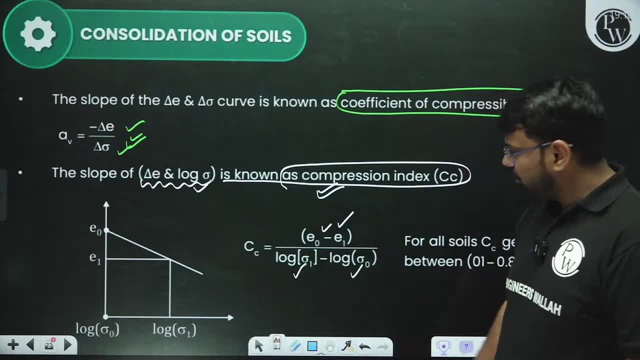 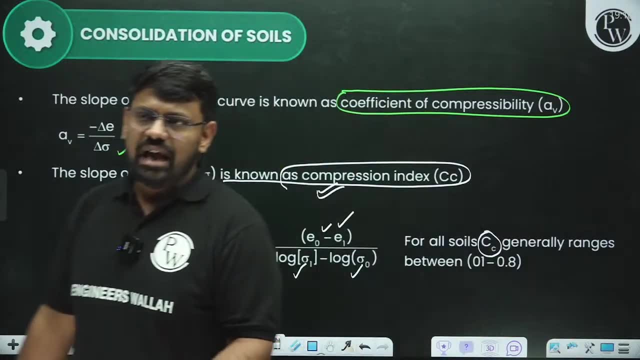 compression index was change in the void ratio divided by log sigma 1 minus log sigma naught. This is your graph. So for all soils, for all types of soils generally, when it is seen then, compression index is equal to 0.1 to 0.1.. 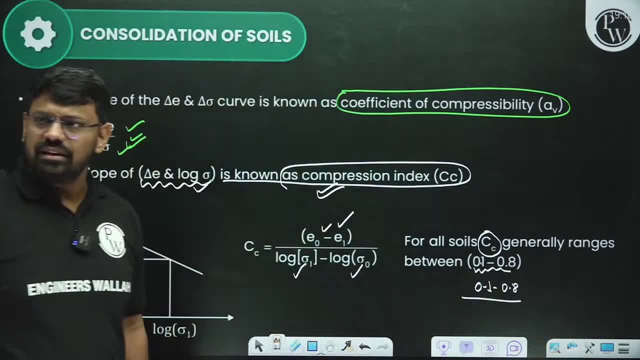 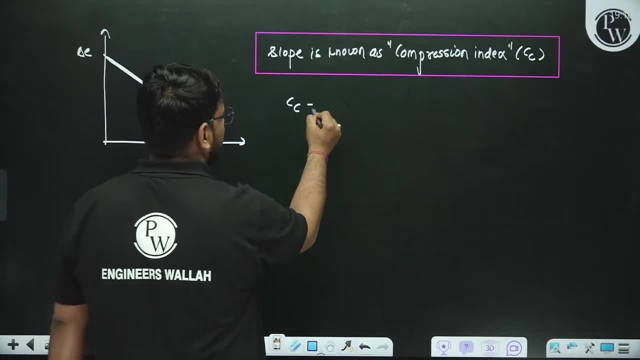 So from 0.1 to 0.8, you get to see. So compression index will be like this. That means, sir cc is basically nothing but your e naught minus e1, divided by log sigma, 1 minus. 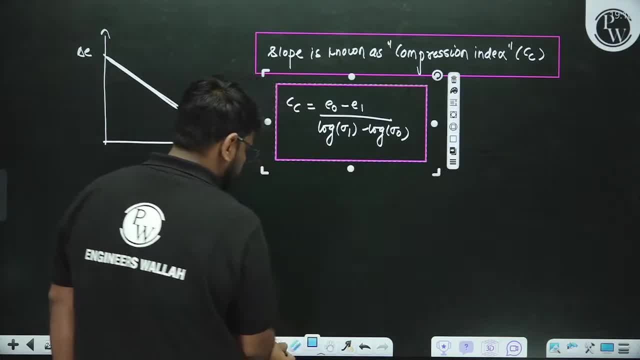 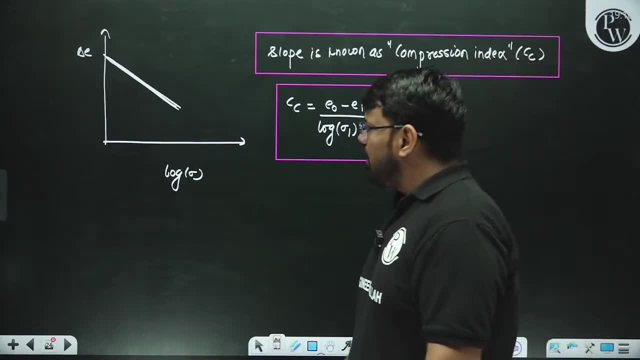 log sigma naught. This becomes the slope of compression index. This is the slope which is known as your compression index. Okay, You have to keep this in mind. Okay, sir. Now, after this, sir understand one thing here. 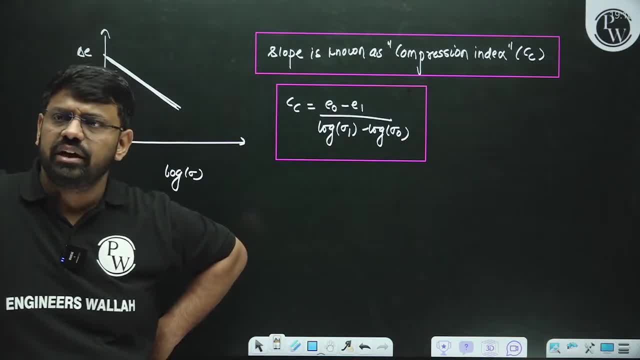 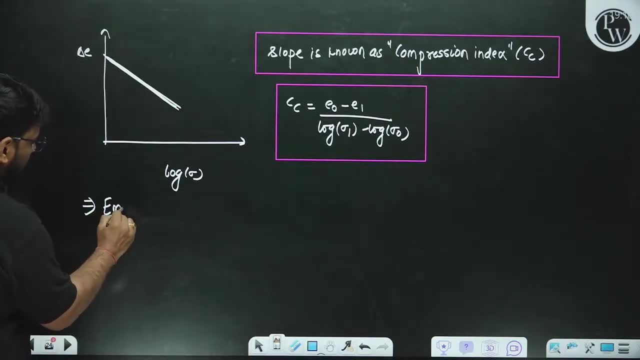 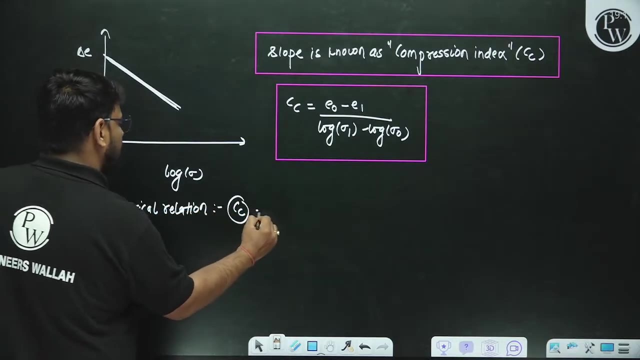 Whenever you talk about compression index. sometimes you are asked about empirical formulas related to compression index. What do you ask, sir? You are also asked about empirical formulas, So empirical relations. Will you quickly comment and tell the children that in compression index 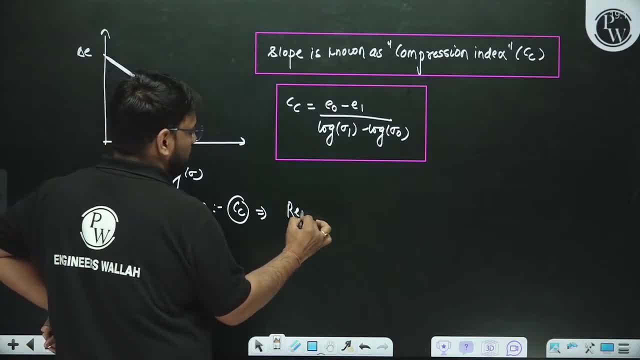 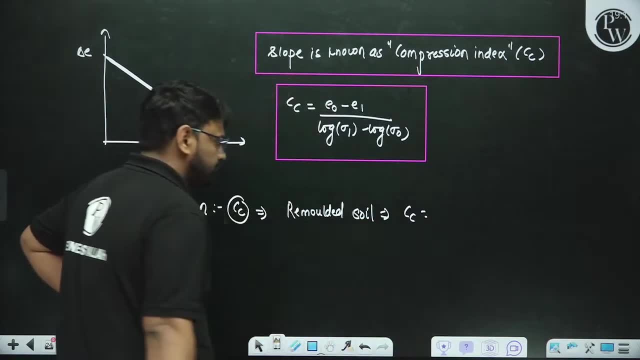 if I am talking about remolded soils. in the case of your remolded soils, how do you measure compression index, sir? Tell me quickly: How do you measure compression index if I am talking about remolded soils? And secondly, sir, if we have 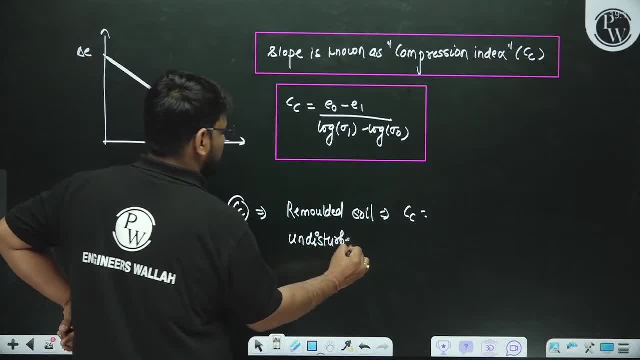 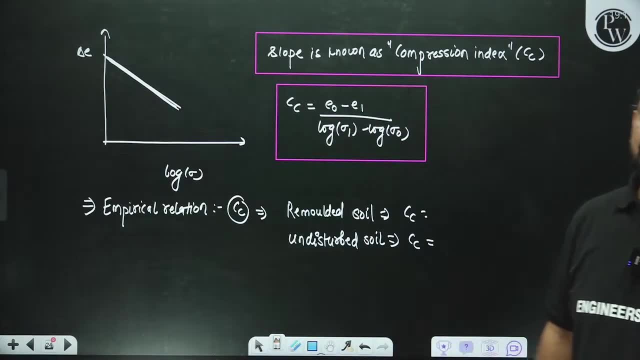 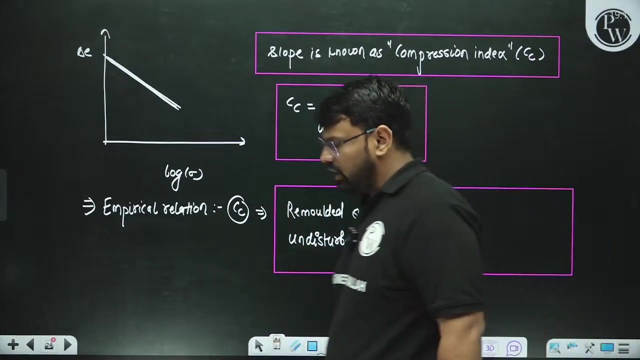 undisturbed soils. in the case of your undisturbed soils, then, how do you measure compression index? Just remember these two formulas here. Remember these two formulas. You will quickly comment and tell me that, sir, remolded soil and undisturbed soil. 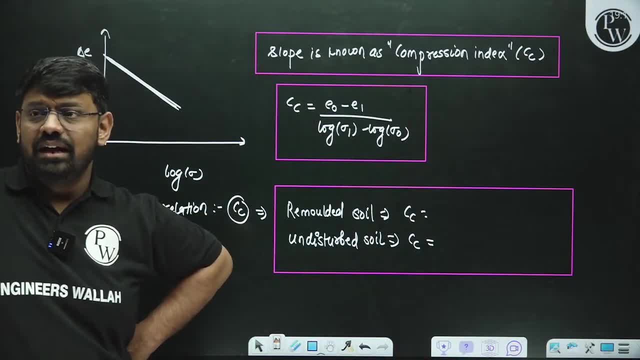 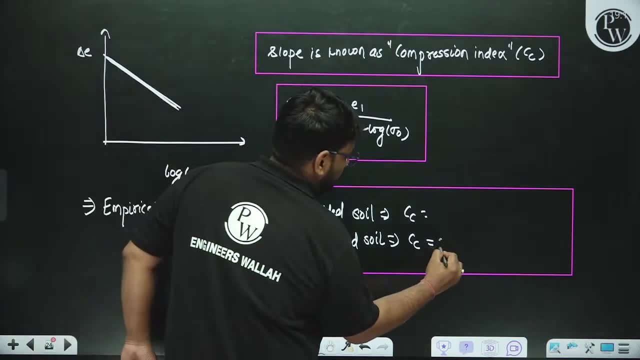 in both cases. will you write and tell separately that, sir? what is the difference between undisturbed and remolded? When it is undisturbed, then it is absolutely correct When you have undisturbed. remember this thing, sir. 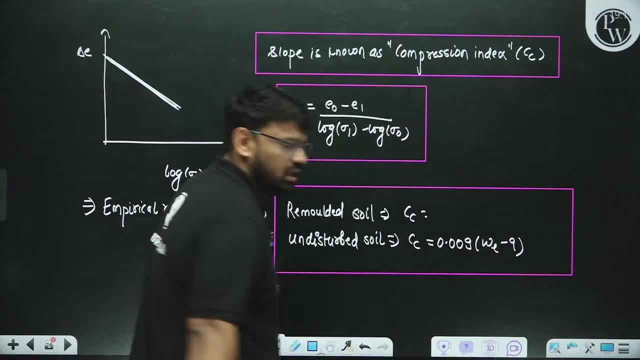 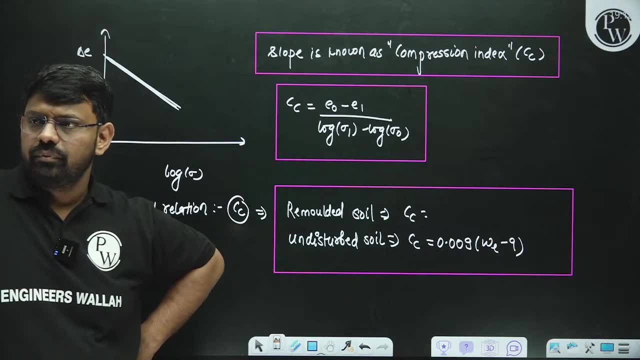 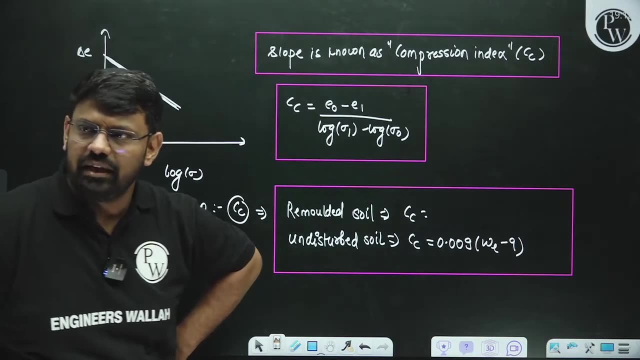 0.009, WL-9.. Right, 0.009,. you have WL- absolutely correct. Yes, 0.009 minus WL-10, you will have. It will not be 9,, it will be 10.. It will not be 9,, it will be 10.. 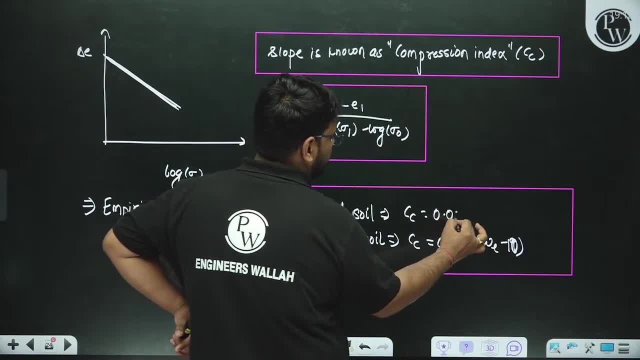 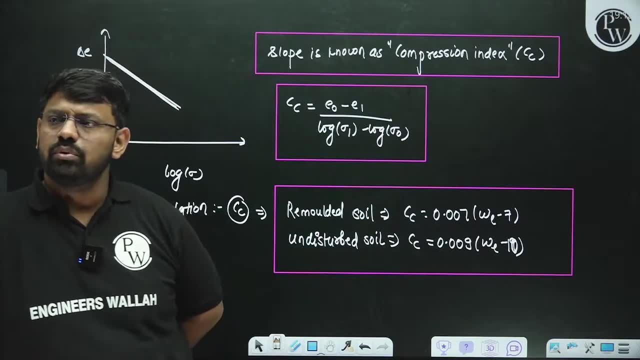 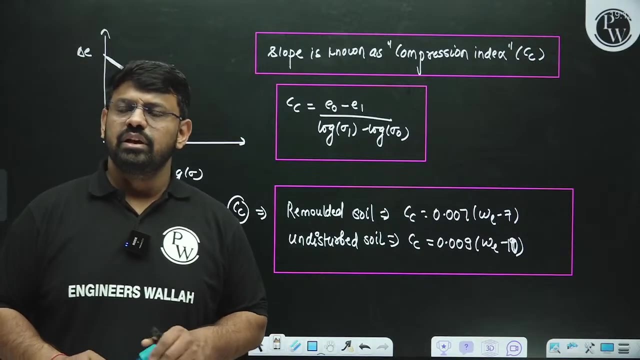 Here you will have WL-10.. Similarly, 0.007 WL-7. you have it here. So these two formulas, you have to remember these two formulas. You have to remember these two formulas. It is absolutely clear, sir. Tell me quickly. 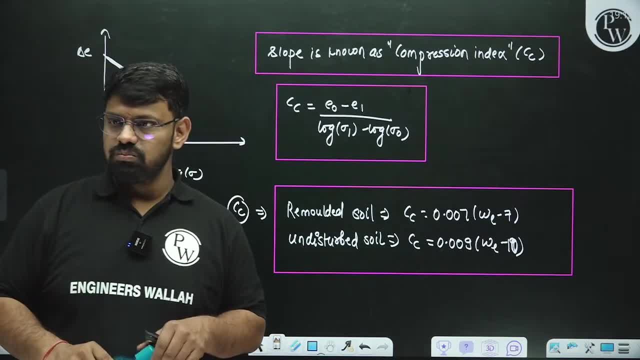 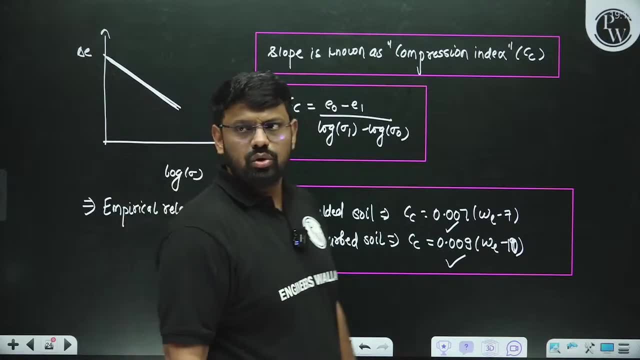 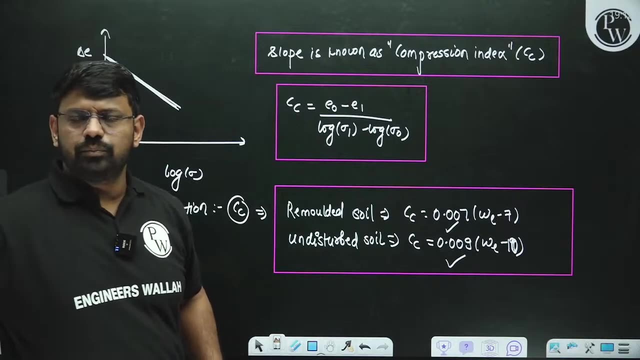 You have to remember these two formulas, Right, So, undisturbed, Undisturbed, And you have remolded in both, Absolutely 0.007 WL-7 and 0.009 WL-10. You have to remember these two formulas. 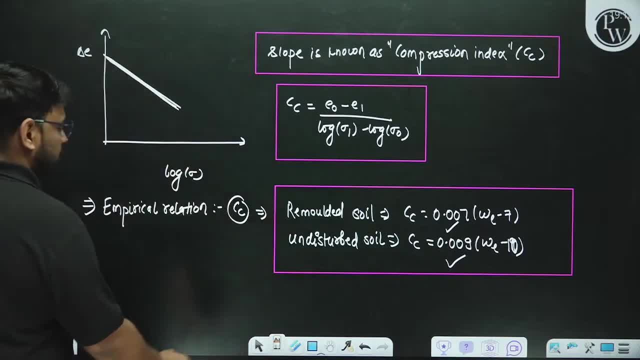 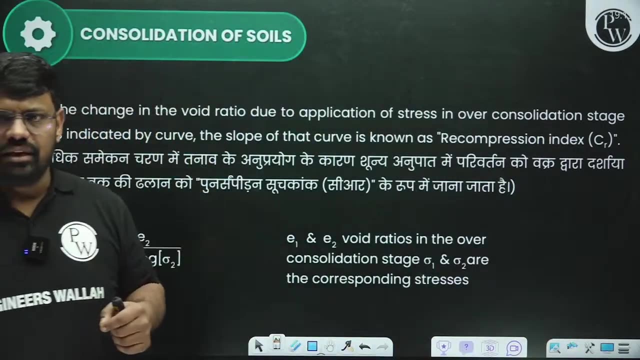 That is clear, sir. So this is your basically empirical relation. This is basically your empirical relation which we get to see here. You will be asked the same question in the previous series. Now, if we talk about recompression index, then what does it mean? 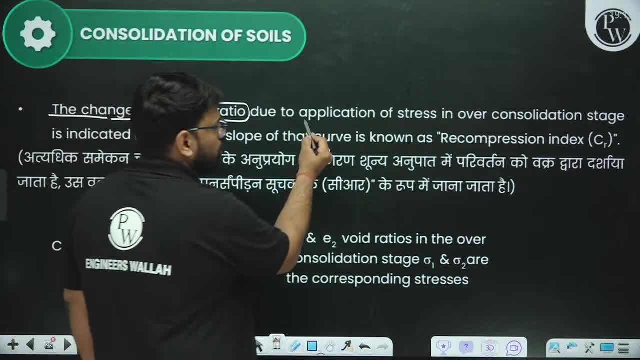 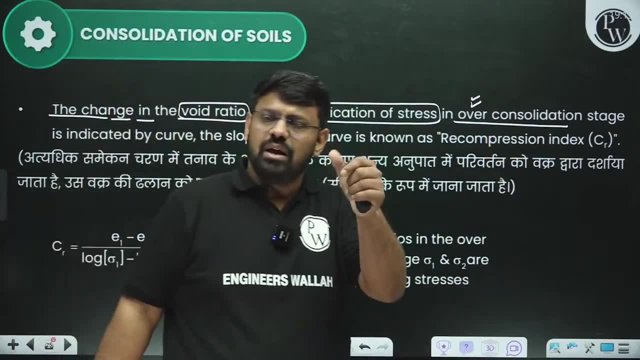 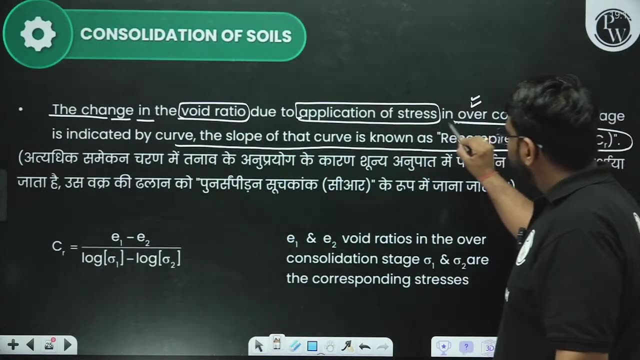 The change in void ratio. If I talk about change in void ratio due to application of stress in over consolidation stage, Sir, when we are talking in over consolidation stage, at that time it is represented by a curve which we call recompression curve. 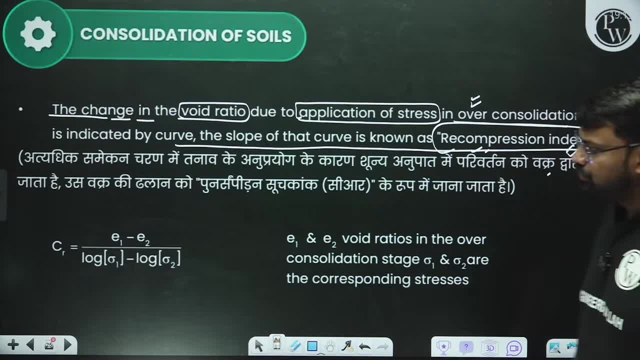 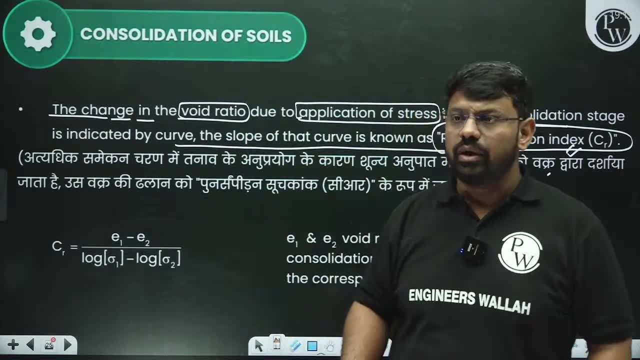 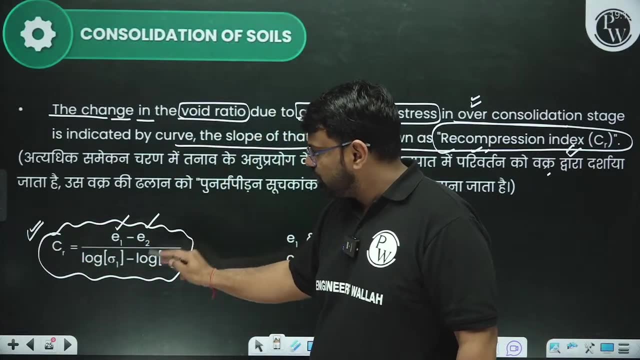 And the slope there is known as recompression index. That means if you go to over consolidation stage, then when you take out the slope of the recompression curve, that will be your CR, which means recompression index. So you have to remember this formula as well. 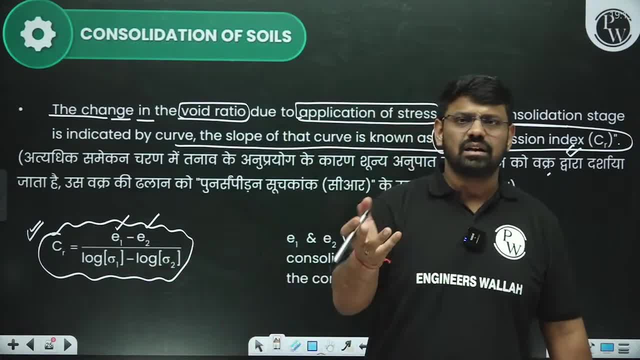 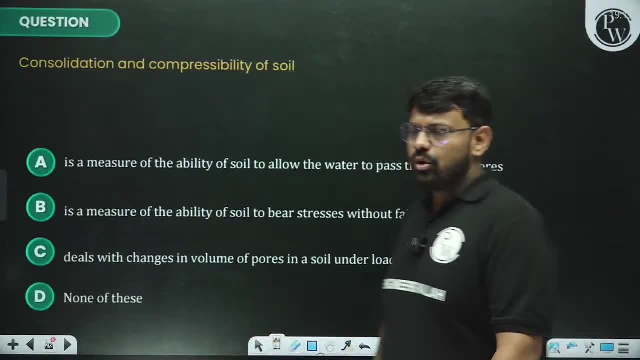 Sigma E1 minus E2 is the formula of over consolidation stage. It is exactly the same as the compression index. Similarly, you also get to see recompression index. Now we will quickly do one question and all students should participate in it. 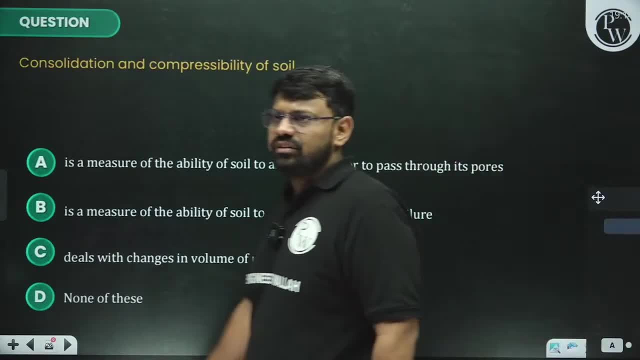 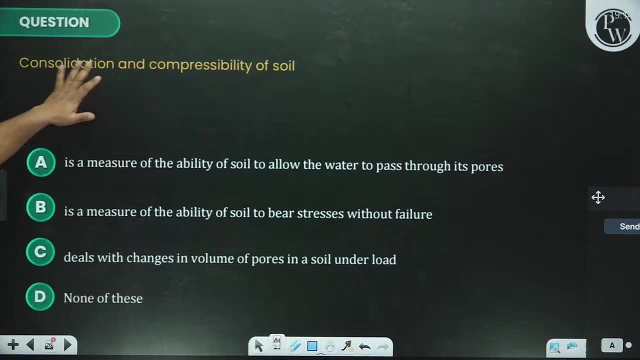 You will tell me the first question. This is the question you have, Then we will move ahead. We have read a lot of theory. Solve one question first, Then we will move ahead quickly. Consolidation and compressibility of the soil: What happens? 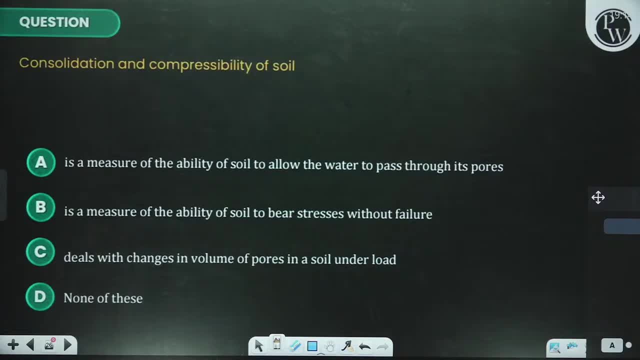 Read the statement quickly and tell me the answer quickly. What should be the right answer for this particular question? Sir, will we get the correct answer for this particular question? What should be the right answer to this question? Answer directly. All kids will comment and ask. 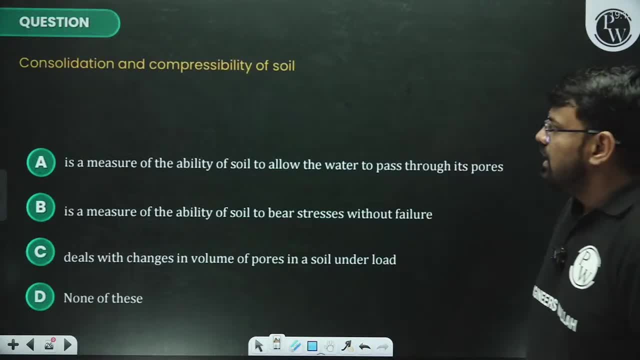 that. what should be the right answer, Sir, is a measure of the ability of the soil to allow the water to pass through it. Sir, this is not consolidation. this is permeability we have. It is a measure of ability of soil to bear stresses without. 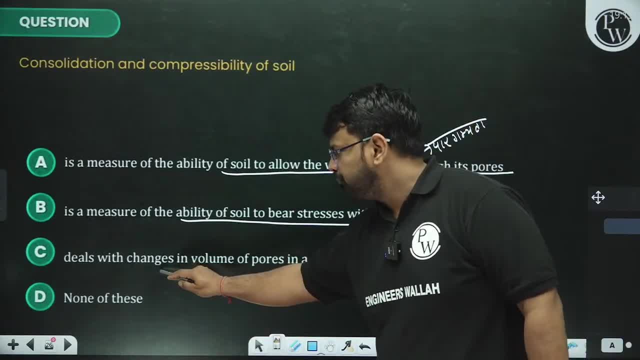 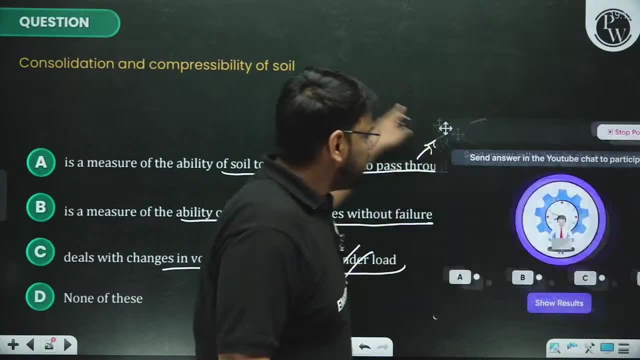 flaring. This is its ability to bear weight, and load bearing capacity Deals with the changes in volume in pores under load. So it is absolutely correct. C is the right answer for this question. All children should remember it in a good way. Sir, what will be? 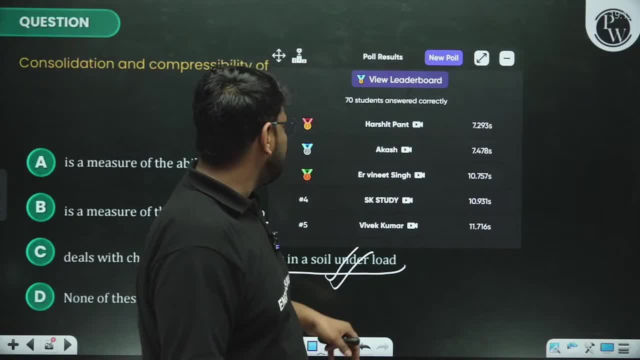 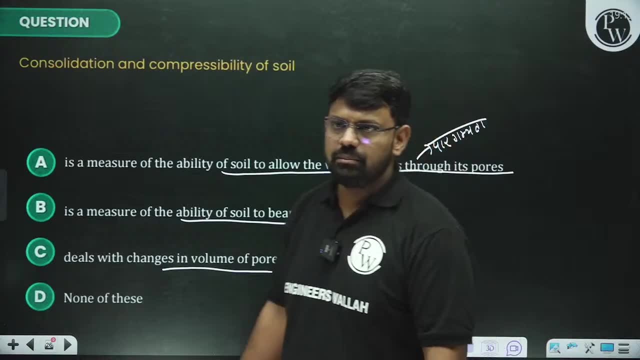 the correct answer for this. C will be your correct answer. 99% of children are correct: Harshit Akash, Engineer Vineet, SK Study and Vivek Kumar. Very good, Very nice, Sir, you have remembered these things in a good way. 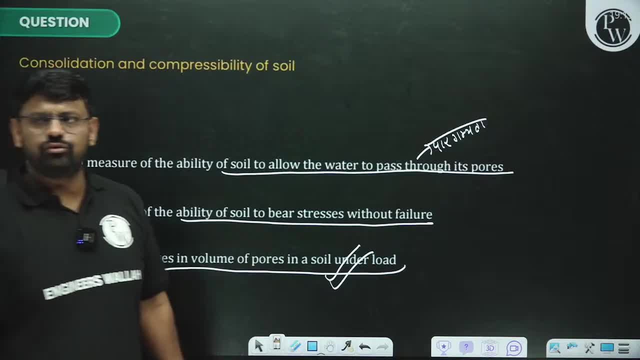 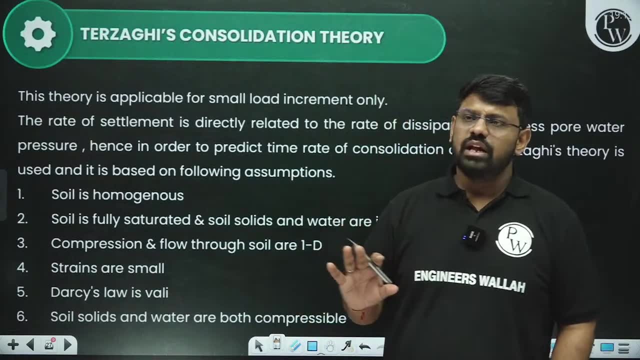 Now see, sir, after this, keep one thing in mind, sir. Now we are going to read. the next topic That you have- assumption point of view or all kinds of point of view- is the most important topic, That is known as your Tarzaghi's. 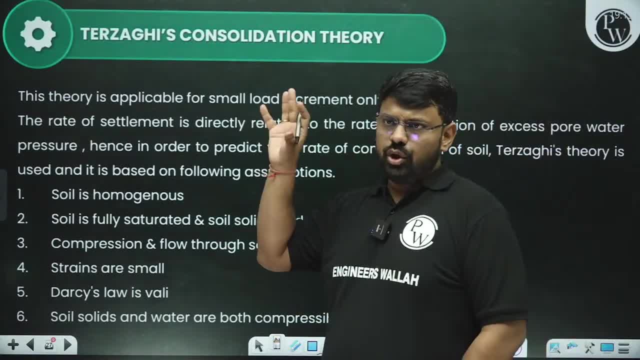 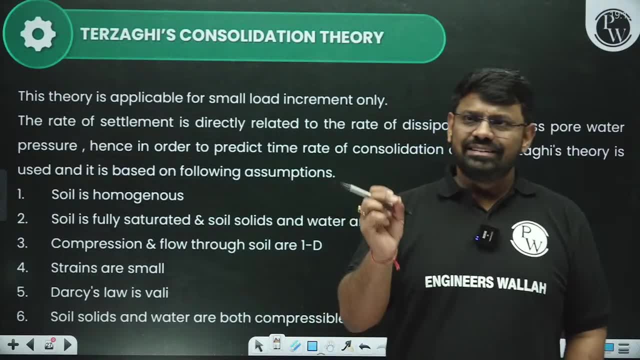 Theory of Consolidation. So Tarzaghi's Consolidation Theory, its assumptions are also important, sir, And the product results that come out of it are also as important to us. Before that, one more thing to understand here. that, sir, the consolidation that you all calculate. 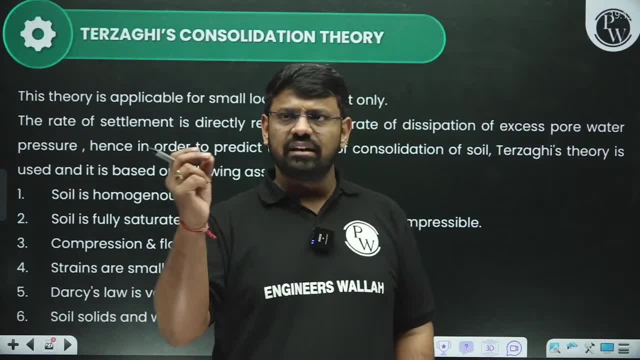 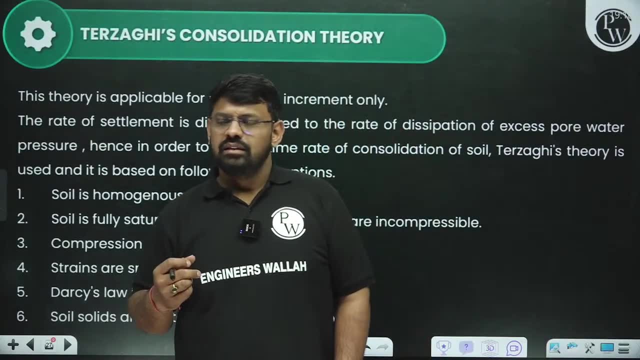 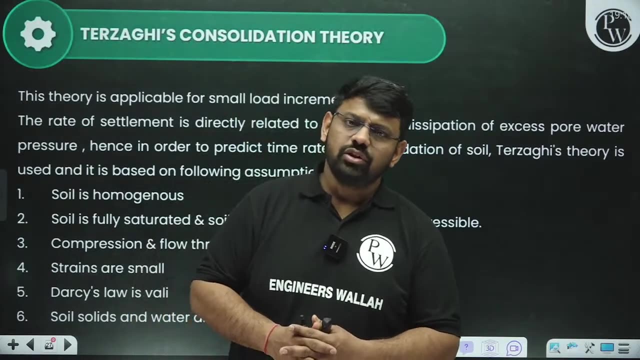 is calculated by an apparatus. Quickly comment and tell me that consolidation, from which device do you people quickly take out? Quickly take it out, sir. Quickly tell me. Quickly tell me Which device do you calculate consolidation from Consolidometer and what else is called a consolidometer? 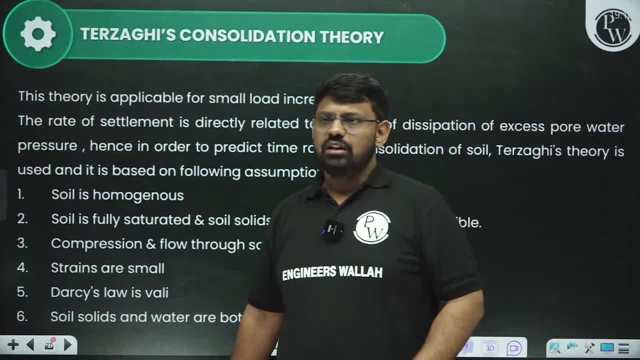 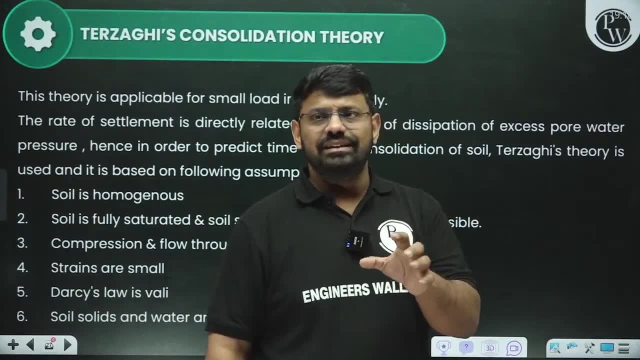 What else is called a consolidometer? Quickly tell me What else is called a consolidometer: Oedometer, Very good, So you have to remember this as well, sir: That Oedometer and Consolidometer. With this you can calculate. 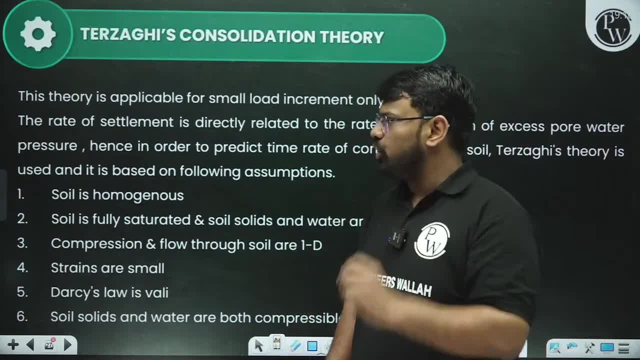 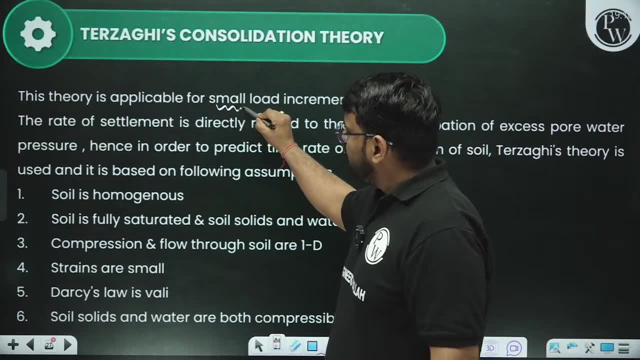 consolidation. Now let's come to Tarzaghi's theory. Sir Tarzaghi's theory. the first and most important thing is that Tarzaghi's theory is basically applicable for your small load increments, only When we have small load increments. 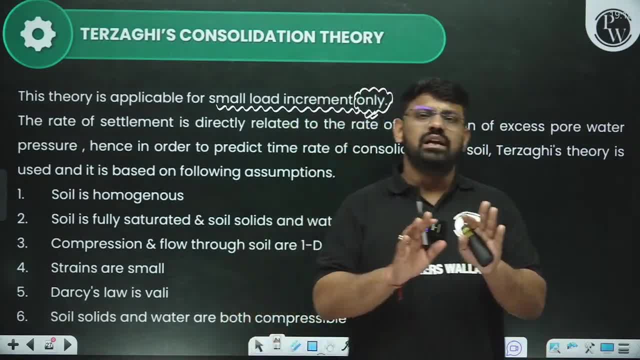 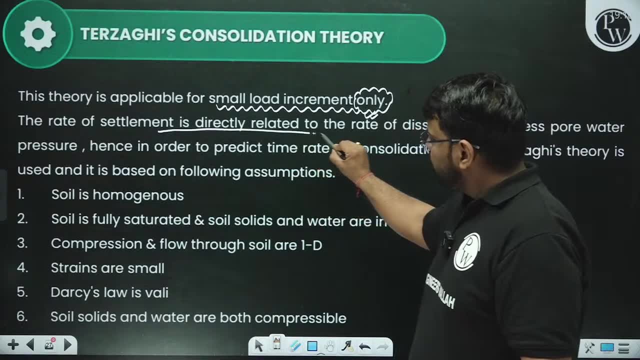 when there are small load increments, then only we consider Tarzaghi's theory applicable. The first point should be clear in our mind. Second: look, sir, the rate of settlement that we have is directly related to the rate of dissipation of. 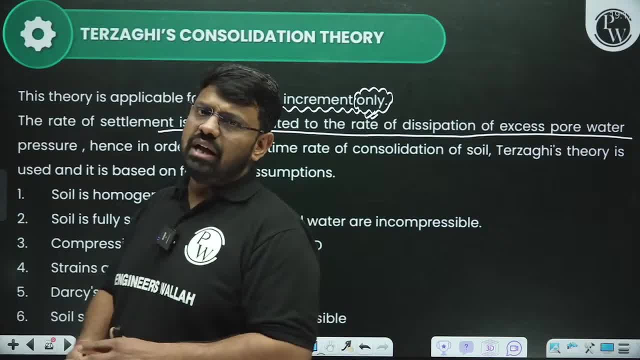 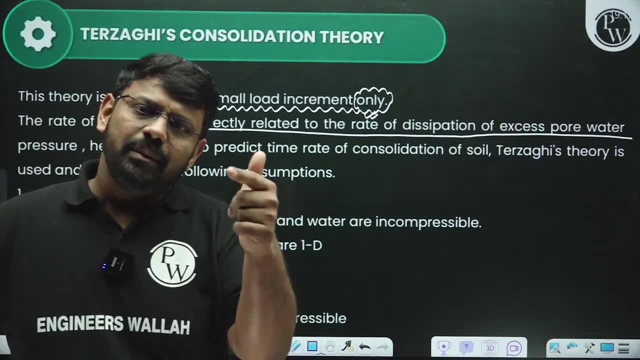 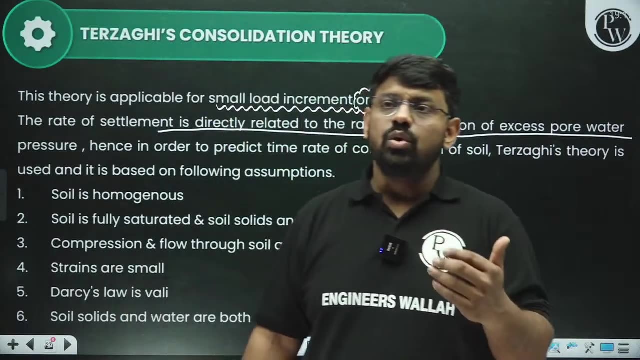 excess pore volume. Sir, consolidation was basically depended on the excess pore volume. So the earlier the excess pore volume dissipates, the earlier the rate of consolidation and the greater the rates of consolidation will be Correct, sir. So the rate of settlement. 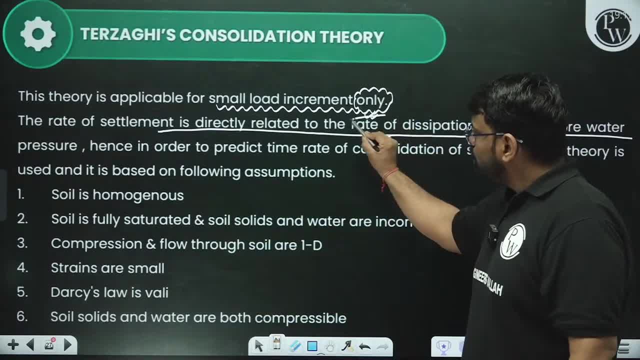 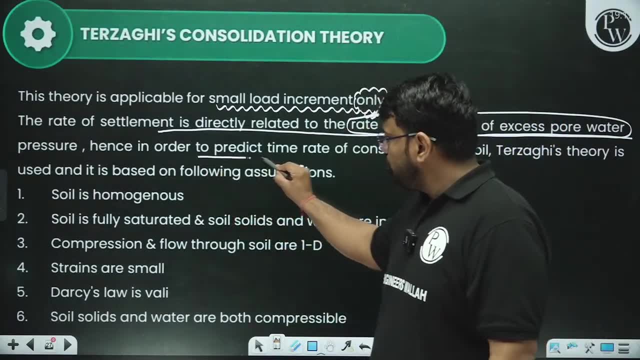 is depending on the rate of dissipation of excess pore volume. It depends on the rate of dissipation of excess pore volume. It means that, Hence, in order to predict the time rate of consolidation, what did the Terzaghi theory say? It accepted some assumptions here. 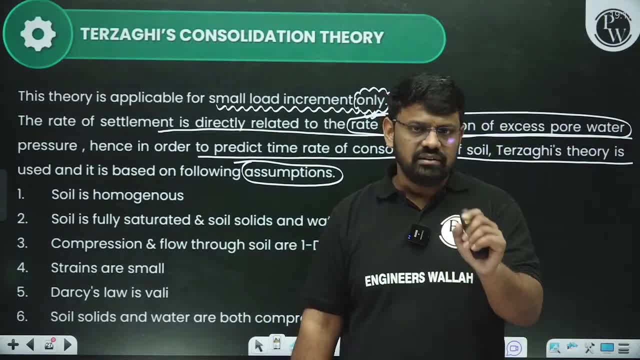 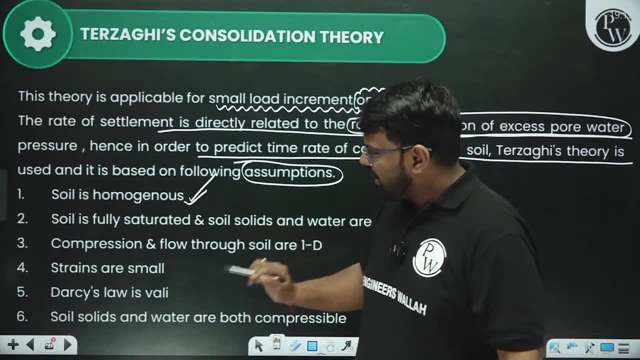 And what are those assumptions, sir? The first assumption, the most basic assumption, which we have to remember, Sir: your soil will be homogeneous. Sir, we remember so many things. Look ahead, Sir. our soil will be fully saturated. 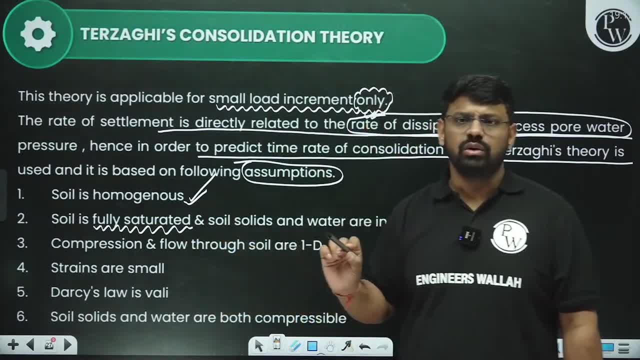 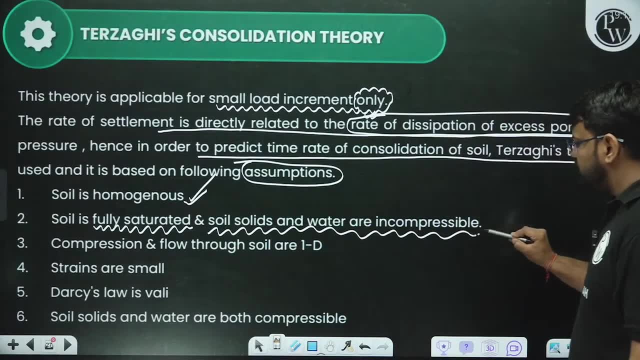 Because consolidation is happening, it is necessary to have completely saturated soil. Soil will be completely saturated And soil solids and water are incompressible. And what are the soil solids and water that we have, Sir? they are incompressible. The Terzaghi did not tell us anything new. 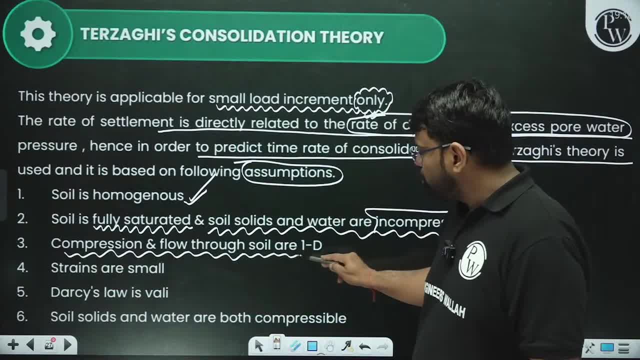 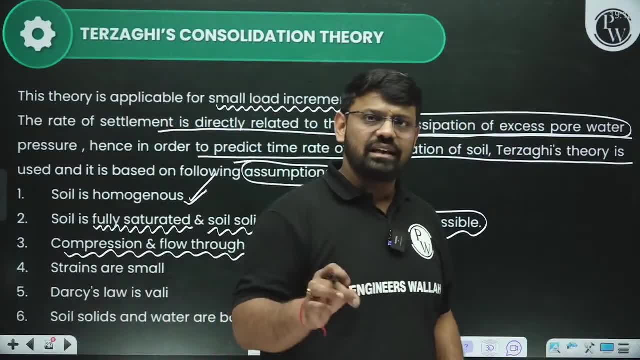 We knew it, sir. Next look: Compression and flow through soil are 1D. Here you have to remember that Terzaghi has a one-dimensional theory. What do we call it? We call it Terzaghi's One-Dimensional Consolidation Theory. 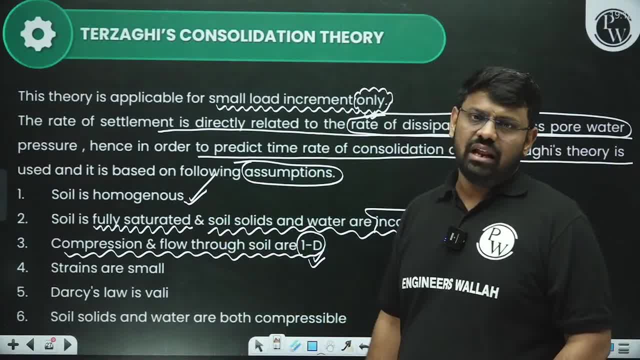 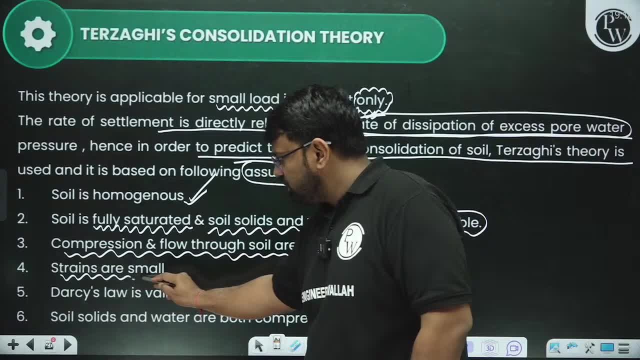 In this one-dimensional theory, we generally allow drainage. That is the water that will come out. it will be from the same direction. OK, Strains are small, So we will take small strains here. We also consider Darcy's Law to be valid. 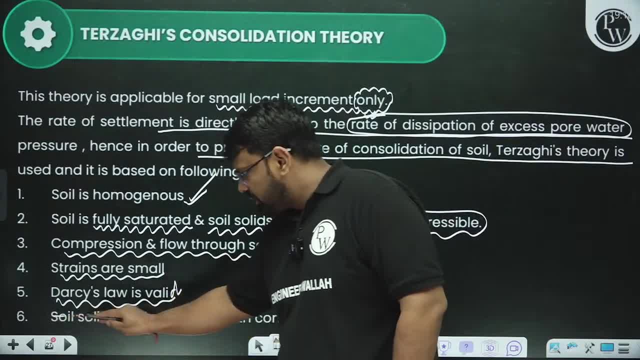 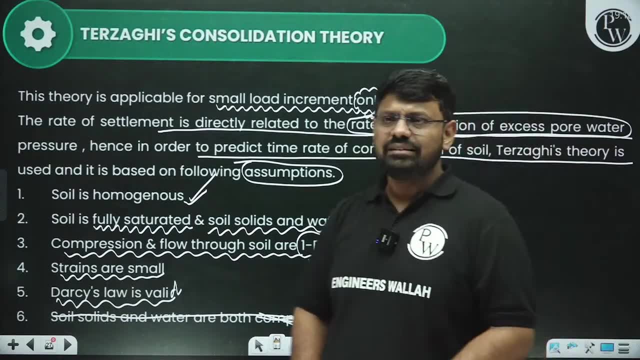 Here, Darcy's Law is valid And I have already told this statement Not compressible. Both will be incompressible. OK, So this is not compressible. This statement is here, So we have some assumptions that it should be homogeneous. 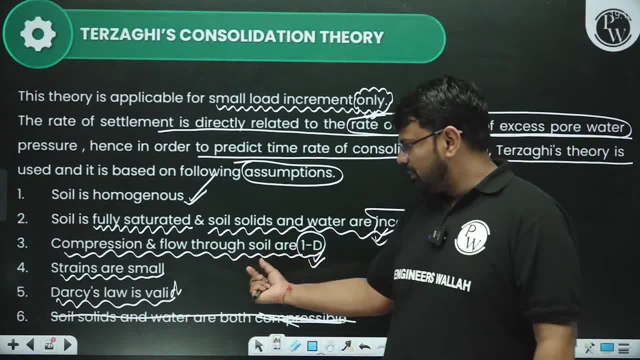 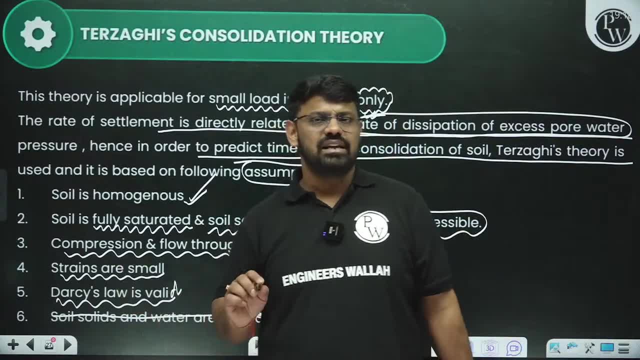 You should have saturated. here We have compression. You should have 1D one-dimensional soil. The strain will be small, sir. Similarly, Darcy's Law will also be valid here. On the basis of this, what has he done, sir? 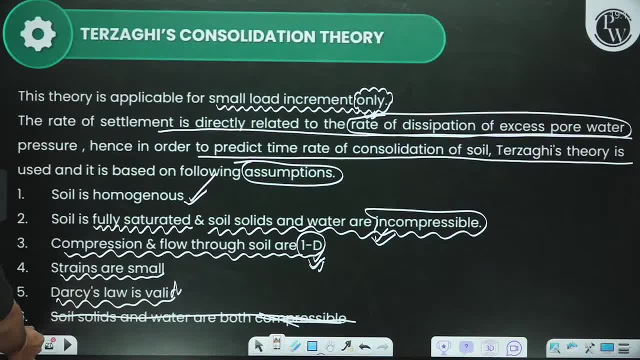 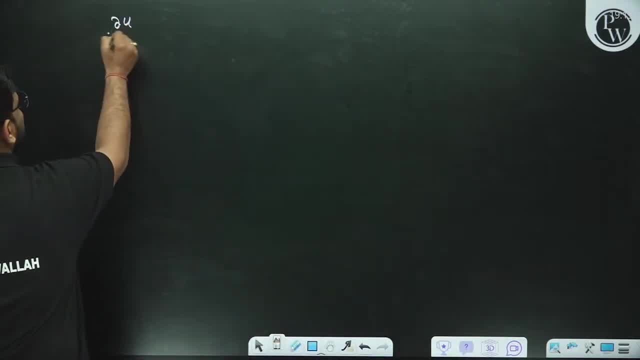 On the basis of this he has calculated the consolidation. OK, On the basis of this he has calculated the consolidation. Now, if you see here, Sir, the consolidation equation that he has given has been given along with the dissipation of the pore water pressure, sir. 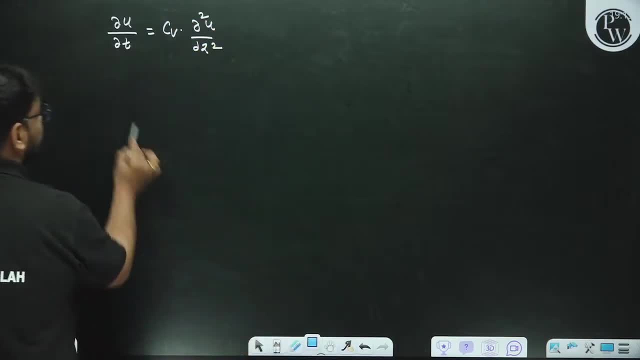 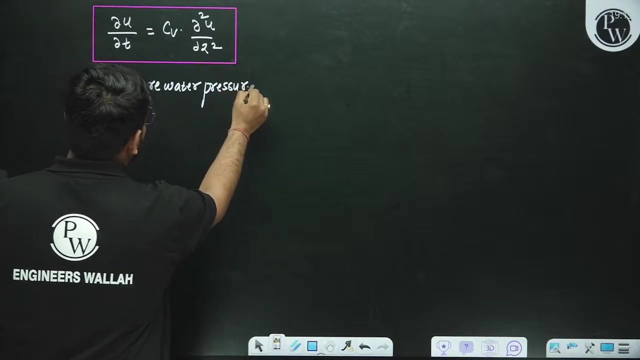 That is, del square, U by del Z square. What do we have here, sir? We have the equation of consolidation here. This is the equation of consolidation In which you can see, sir, U is basically your pore water pressure. So, sir, we have U pore water pressure. 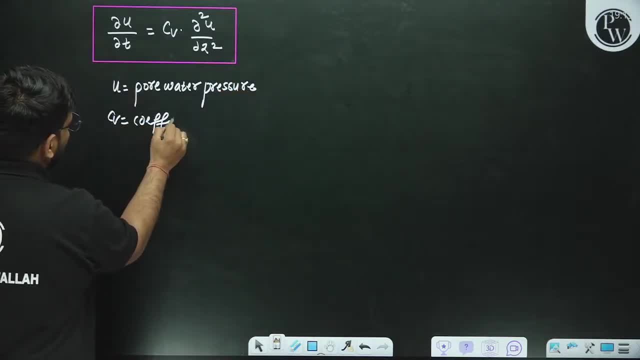 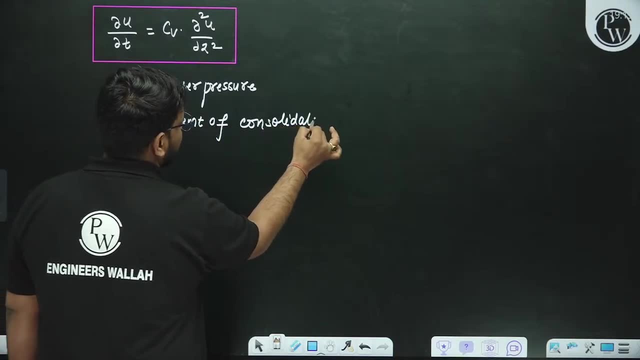 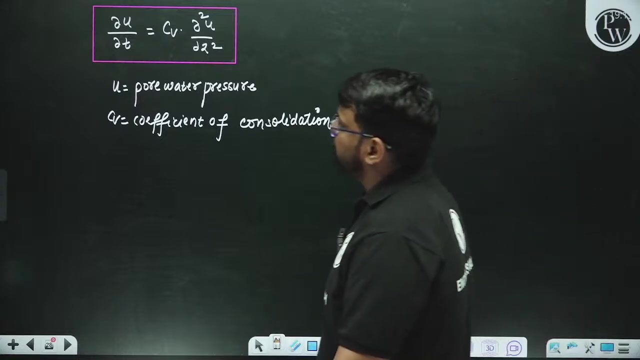 And Cv. this is known as your coefficient of consolidation. This is known as your coefficient of consolidation. Is it clear? This is known as your coefficient of consolidation. OK, This is what we call coefficient of consolidation: Cv And Cv, which we have see. I have told you two things. 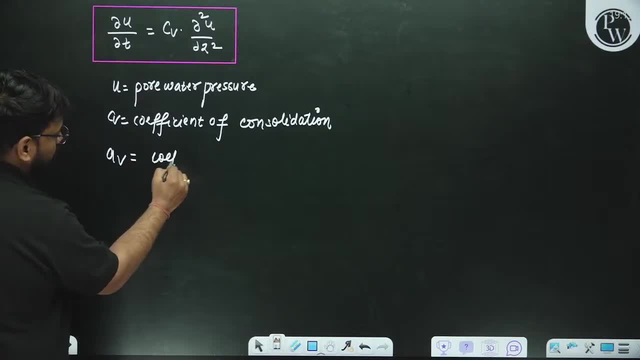 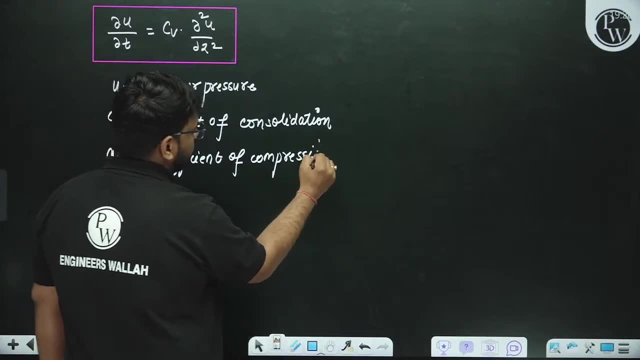 One. I told you: Av, Sir, we had the coefficient of compressibility, Isn't it Sir? we had Av Coefficient of coefficient of compressibility. So, sir, this was the coefficient of compressibility And this, sir, we had the coefficient of consolidation. 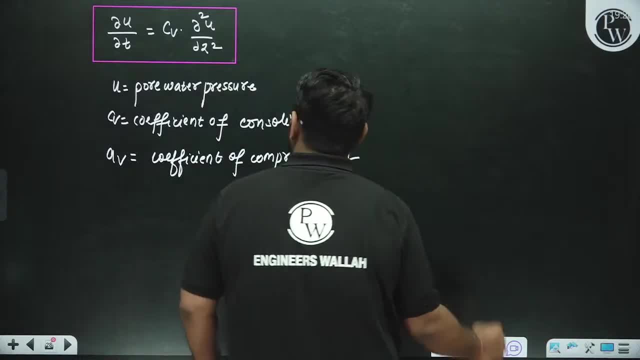 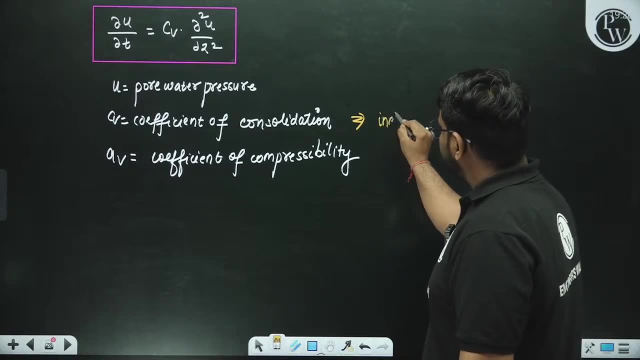 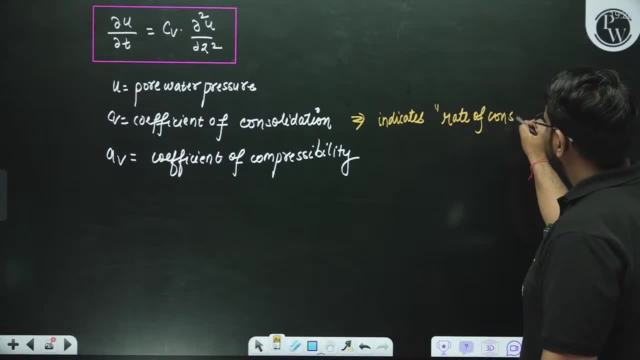 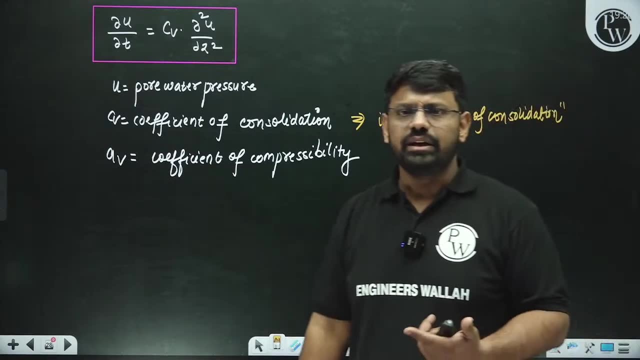 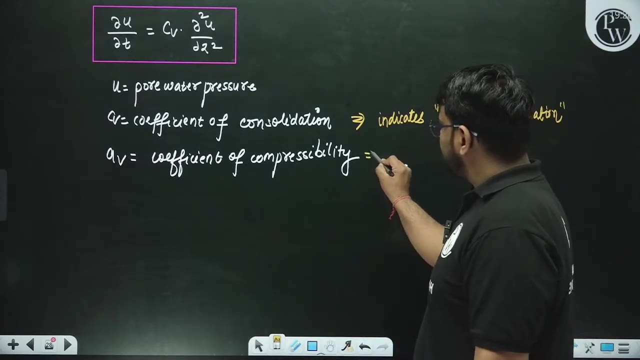 Means how fast the consolidation is going on. it is generally referred to, It indicates the rate of consolidation. So, sir, this indicates the rate of consolidation. The first thing, it is clear. Second, sir, coefficient of compressibility. 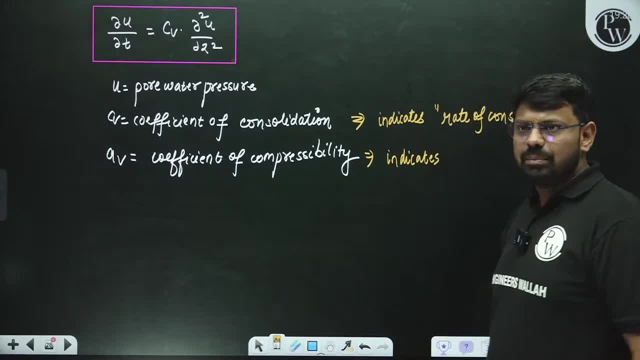 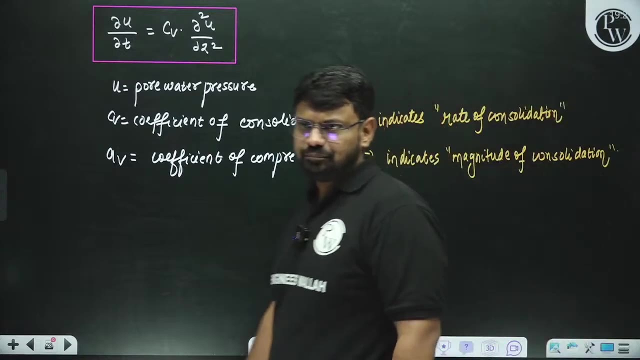 Sir, what does coefficient of compressibility indicate? Sir, coefficient of compressibility indicates the magnitude of consolidation. It indicates the magnitude of consolidation. So, sir, he considers the magnitude of consolidation. It is clear now. Now let us see here. 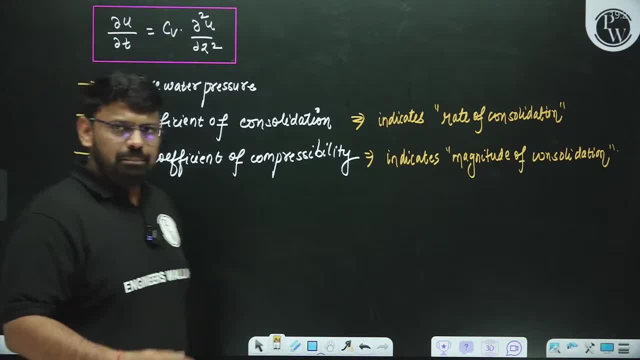 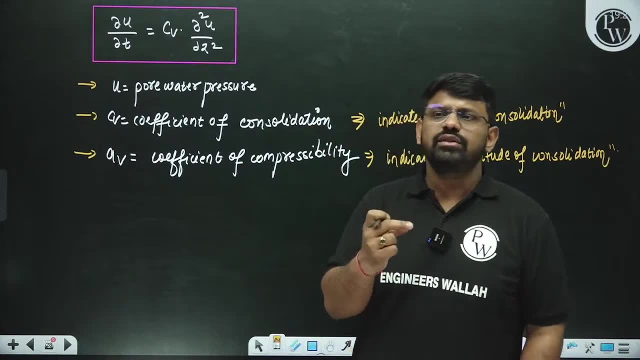 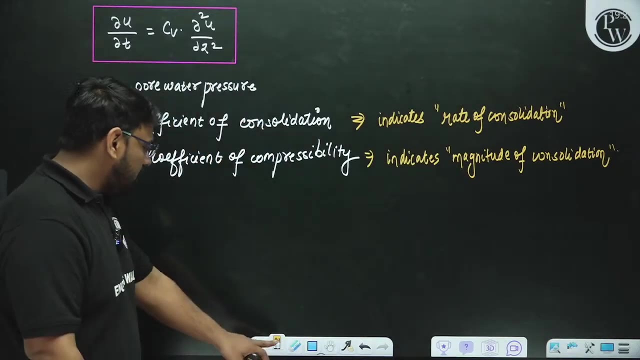 One thing to understand That Tarzaghi said in his theory. Tarzaghi said in his theory That, sir, the change in void ratio and the change in stresses, You get to see a unique relationship in between. You will get to see a unique relationship. 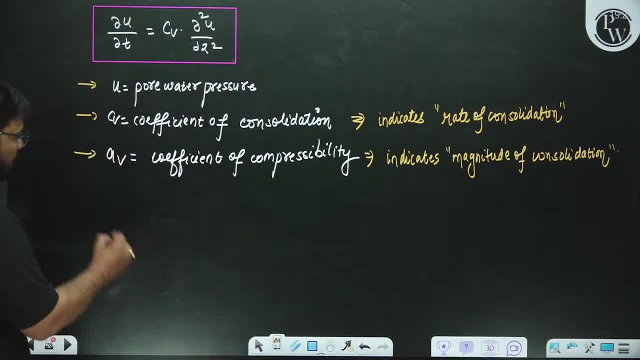 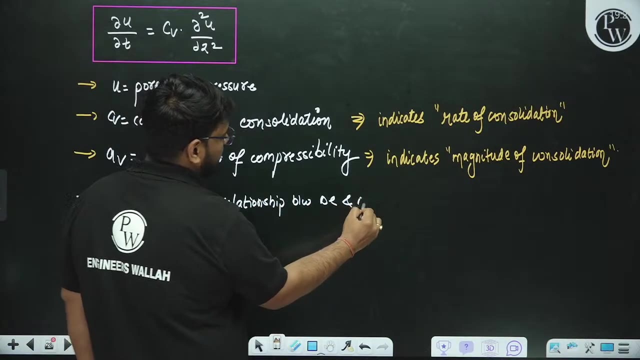 It means he is talking about the coefficient of compressibility. Okay, Keep this thing in mind. Tarzaghi said there is a unique relationship. There is a unique relationship between delta E and delta sigma. It is clear, sir. It means he is making AV a constant. 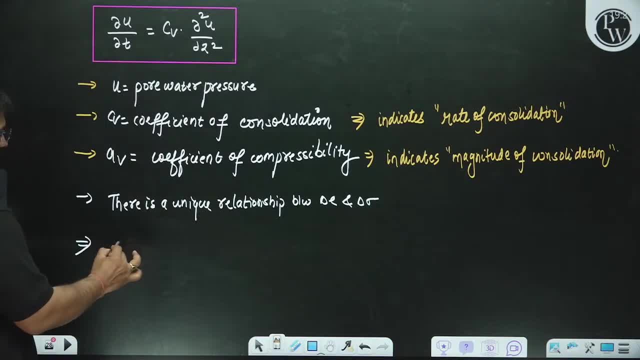 Throughout the constant. And along with this, sir, You get to see a unique relationship, One thing to keep in mind, sir. You get to see two types of names in it, Sir. one is hydrodynamic lag, One is hydrodynamic lag. 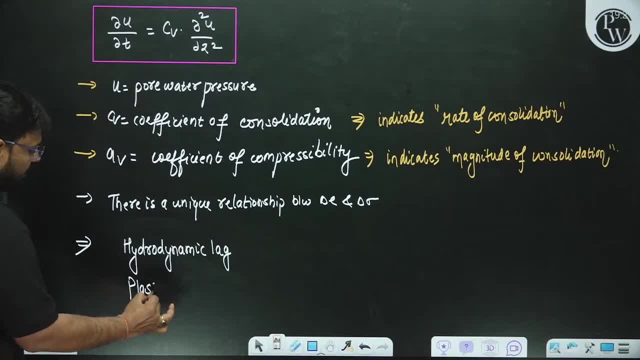 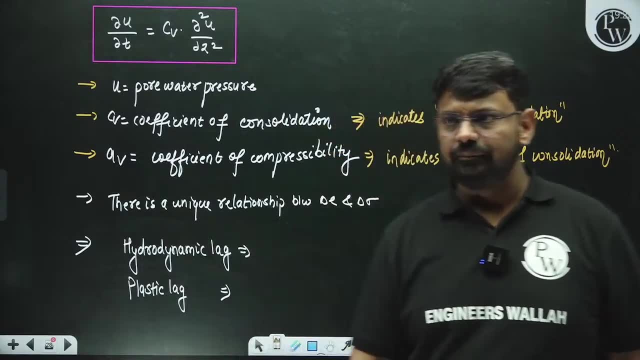 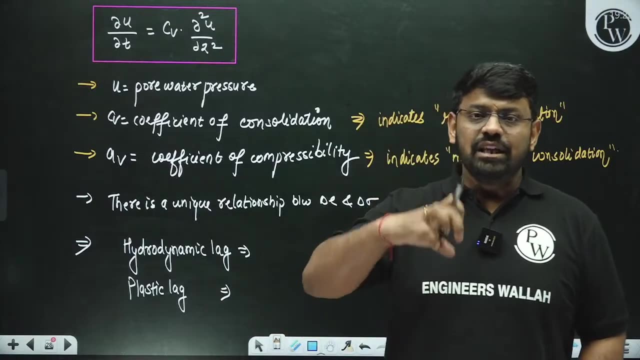 And one is plastic lag. You have to understand these two words now. One is plastic lag. Tell me quickly What is hydrodynamic lag. What is hydrodynamic lag, Sir? hydrodynamic lag means How much time does it take water to transfer from a particular soil mass? 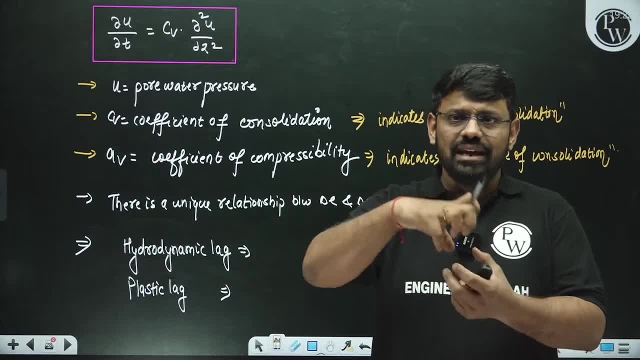 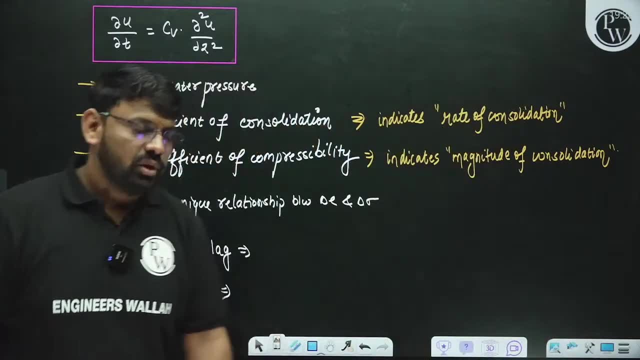 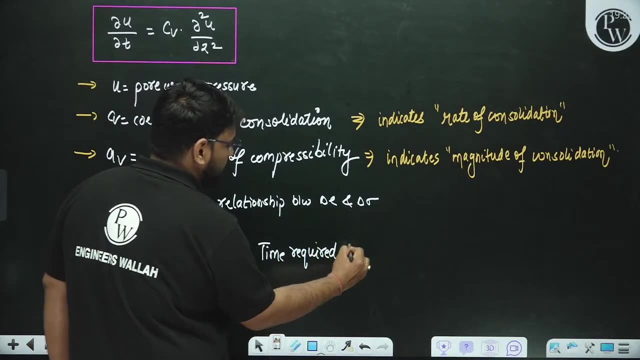 to another soil mass in the same place. squeeze out with a particular soil mass. squeeze out means how much time does it take to get it out? that is called as hydrodynamic lag. So look at the definition: time required. this is basically time required, time required to. 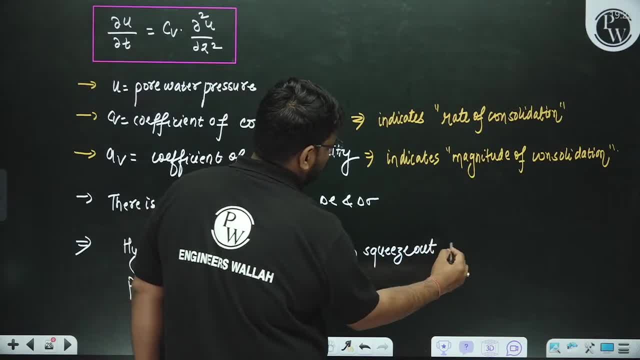 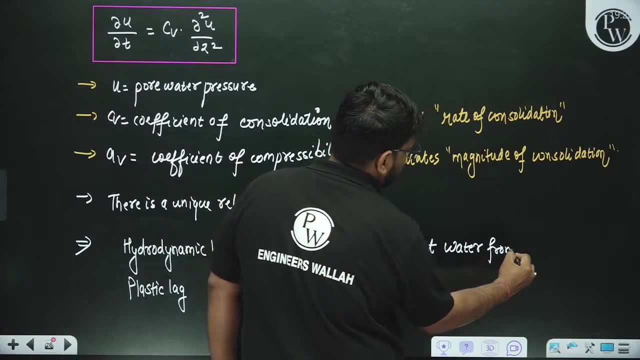 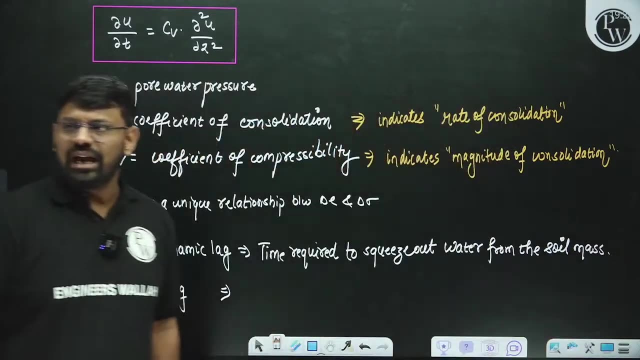 time required to squeeze out. squeeze out water from the soil mass. squeeze out water water from the, from the soil mass, So from the soil mass to squeeze out water, the time it takes. what do we call that? That is called as hydrodynamic lag. 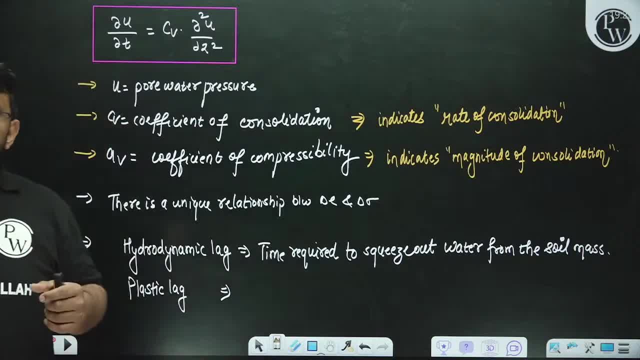 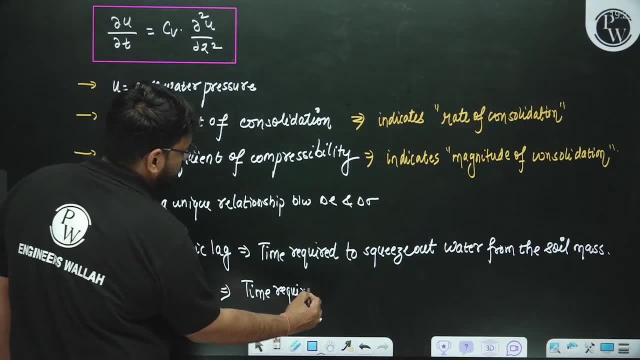 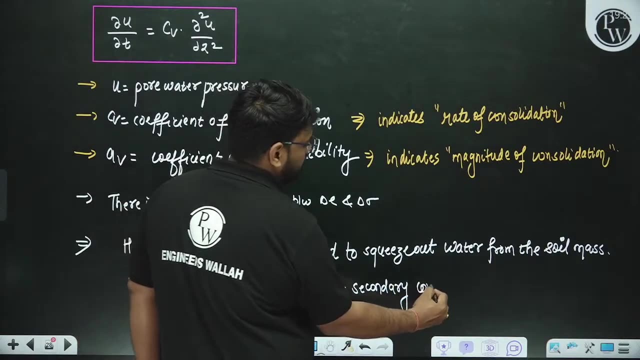 And what is plastic lag? What is plastic lag? Plastic lag is the time required for secondary consolidation. This is basically your time required, time required for time required for secondary consolidation. So the time required for secondary consolidation is called as plastic lag. 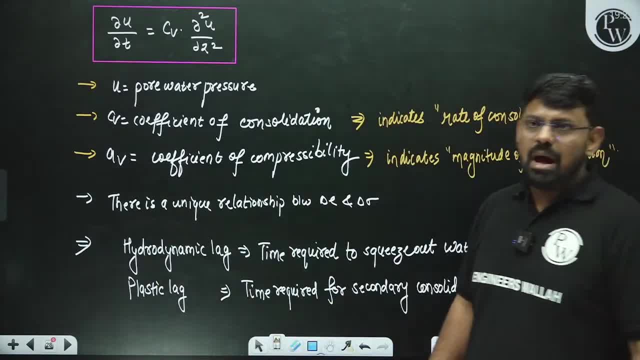 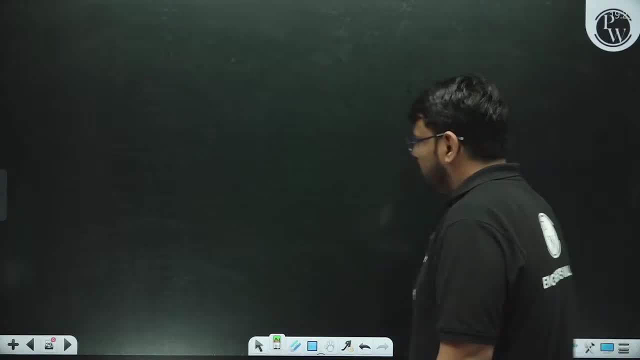 That is basically known as your plastic lag. Now you have to understand one thing here: that sir Tarzaghi Tarzaghi has told you one more thing. what did he tell you, sir? I will tell you in a good way. 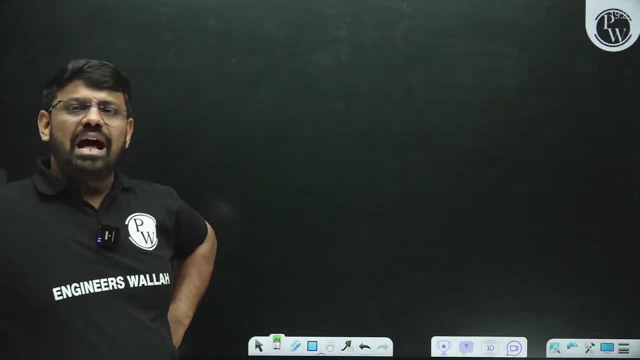 Sir, here he said, Tarzaghi, that Tarzaghi has neglected plastic lag. So Tarzaghi only considers the hydrodynamic lag and, neglecting it, He neglected the plastic lag. You have to write this point in a good way in a note. 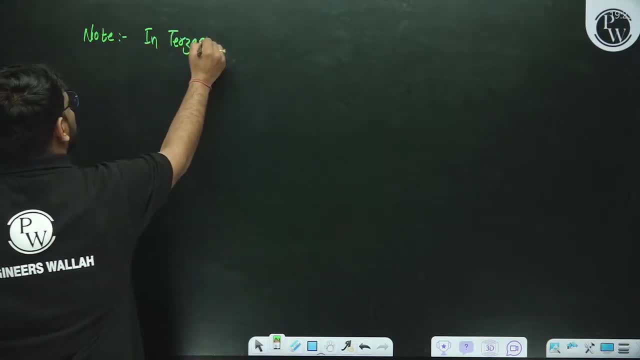 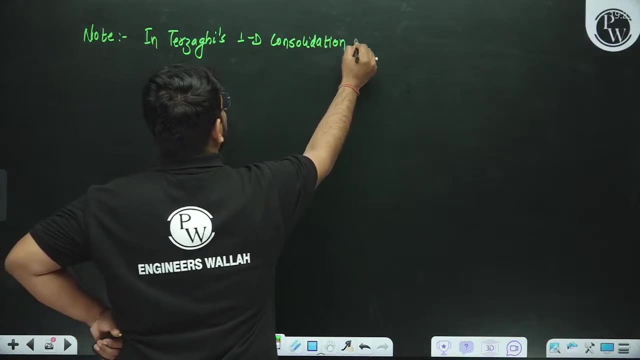 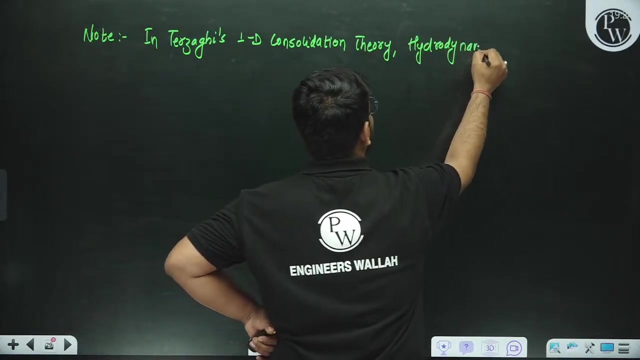 That in Tarzaghi's theory, in Tarzaghi's, in Tarzaghi's 1D consolidation theory, in Tarzaghi's 1D consolidation theory, consolidation theory, hydrodynamic, hydro hydrodynamic lag is considered. 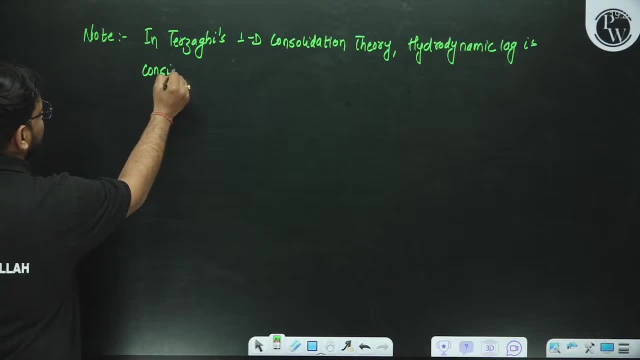 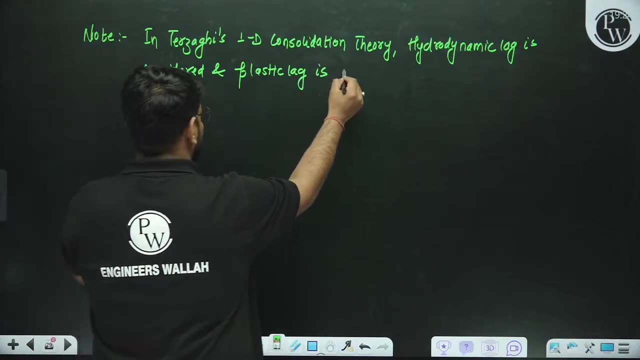 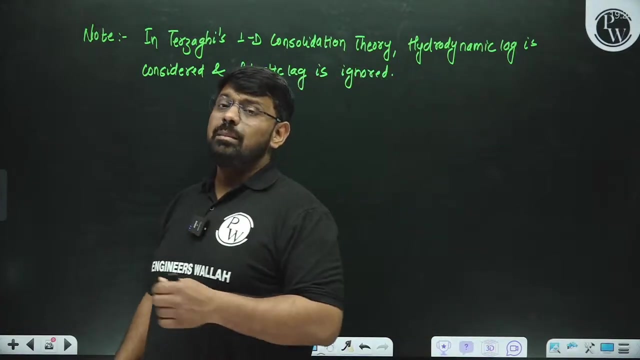 So hydrodynamic lag is considered, lag is considered and plastic lag- plastic lag is ignored or neglected. So we have ignored or neglected plastic lag. You can understand one more thing from this, sir, What This means. sir, he is explaining primary consolidation. 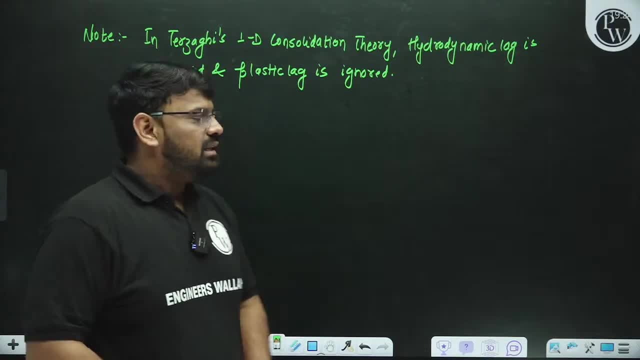 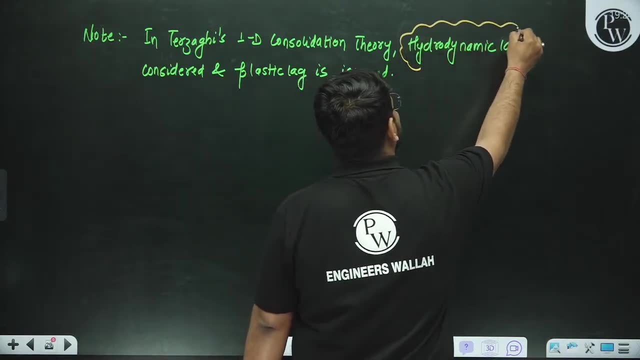 and he is neglecting secondary consolidation. It is absolutely clear. That means, sir, primary consolidation is being discussed. So you can write this point here also, that, sir. this means, sir, what is the main focus of this? Sir, what is the main focus of this? 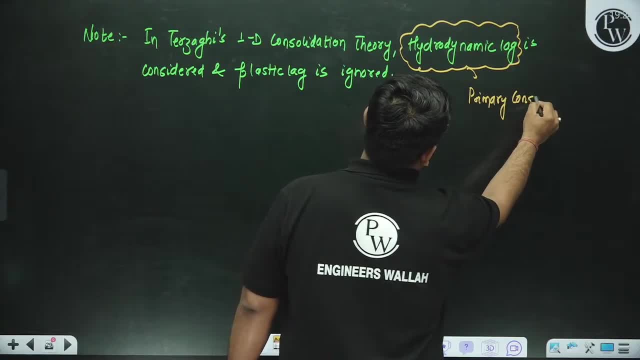 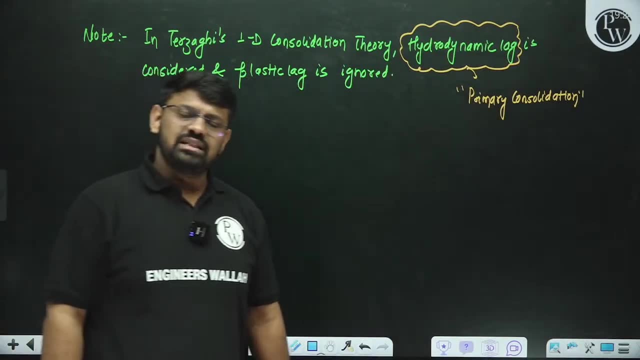 It is on primary consolidation and not on secondary. So if you ever get to see this point then, sir, you have to understand this point here also. It is absolutely correct, sir. So this Tarzaghi's equation came to us. 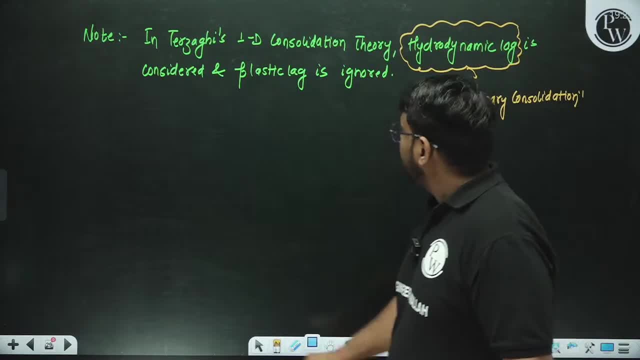 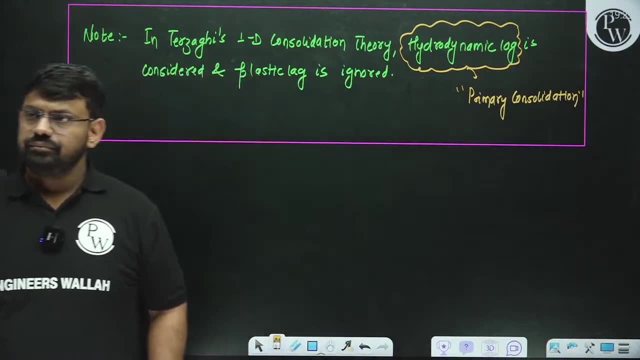 In this Tarzaghi's equation. we have understood all these points. We have also covered up some important points, sir. Now see sir further. Now see, sir, further. Sir, the last part of 3 minutes is a little less understood. 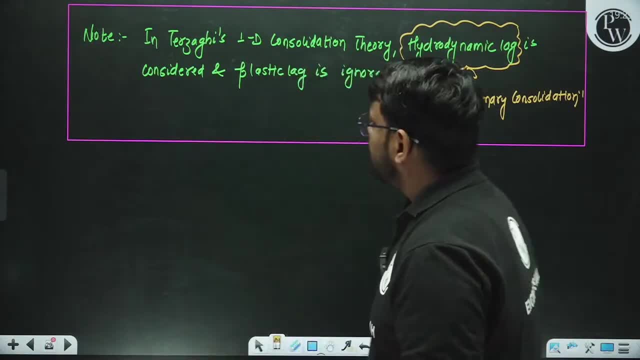 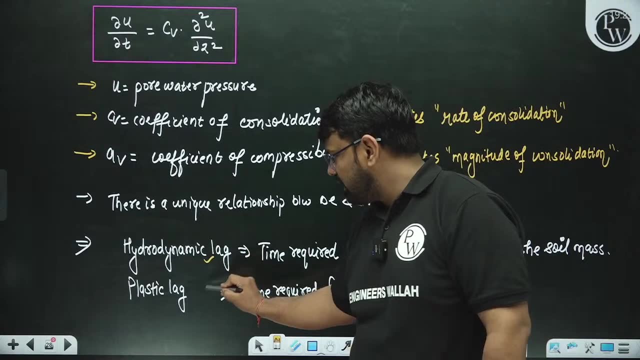 Exactly. SK knows 3 minutes. See: SK understand 3 minutes. what do I know? where is your 3 minutes, 3 minutes. I would have told you this only, Sir. we have Hydrodynamic lag and Plastic lag. So Hydrodynamic lag means till the time water is coming out. means: how much time does it take for primary consolidation? That is your Hydrodynamic lag. How much time does it take for secondary to happen? Sir, what is that? 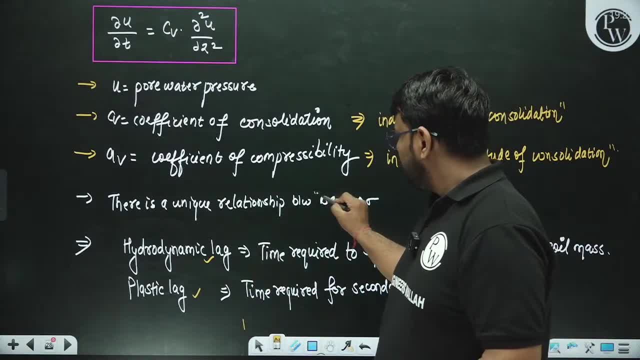 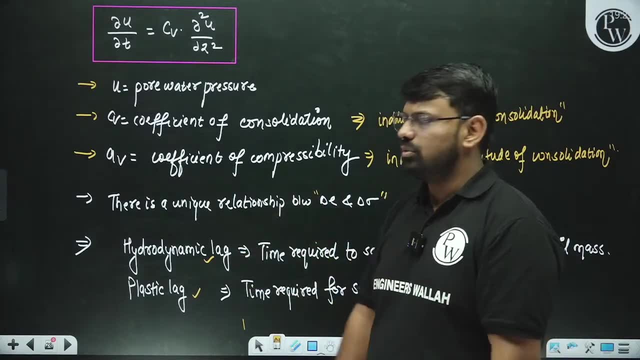 That is Plastic lag. That is Plastic lag. There is a unique relationship means in the void ratio. as the amount of stress changes, the same amount of void ratio also changes gradually. There is a unique relationship between the two. We have to take care of this thing. 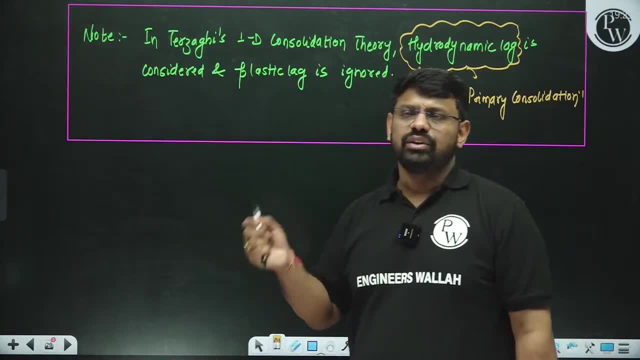 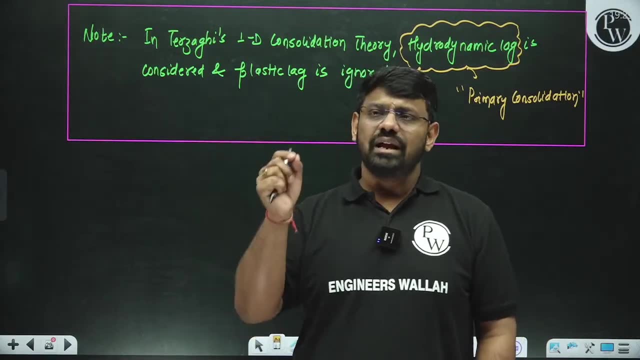 I have told you these two things, And I have told you these two things, so I have written this to you in a statement- that, sir, the theory of Tarzaghi- we have it- considers the Hydrodynamic lag- means in total. you have to keep in mind, sir, 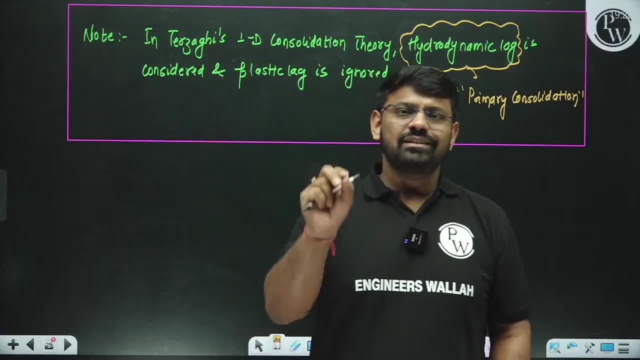 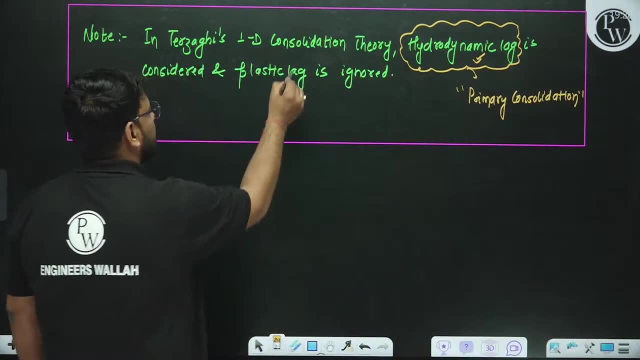 that he is talking about primary consolidation. He is talking about primary consolidation. So, sir, primary consolidation is considered, It does not do secondary. Okay, I have told you all these things here. Okay, sir. So Plastic lag means: 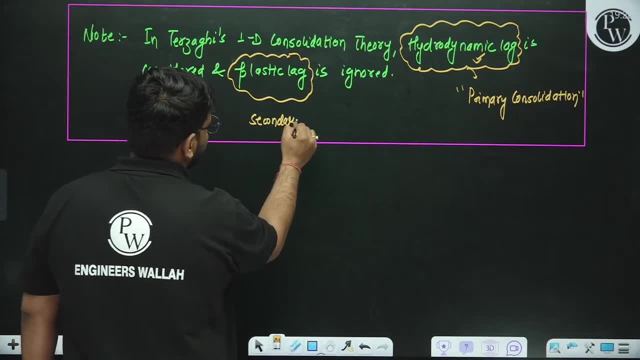 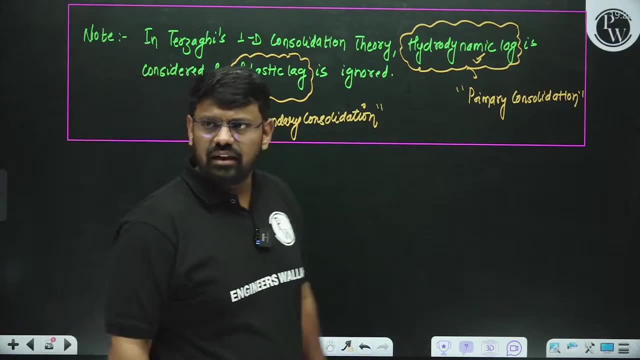 basically, you have it indicates about secondary consolidation. Okay, sir, So SK study. I have told you all these things till now. Okay, The last three minutes, I have told you again. Okay, sir, Look ahead Sir, now, if you understand here. 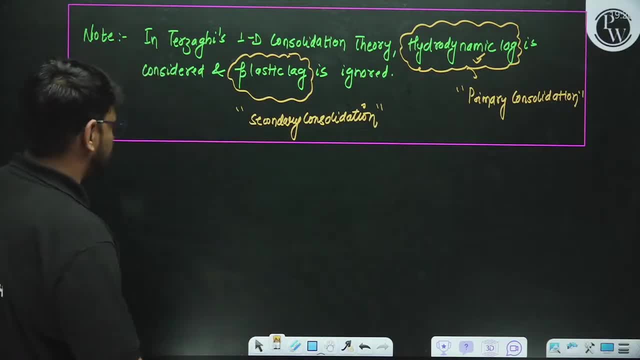 so, sir, we have, we have a term which we call Isochrones. What is it called? Tell me quickly, what are Isochrones? You must have heard this term. So, sir, what is the meaning of Isochrones? 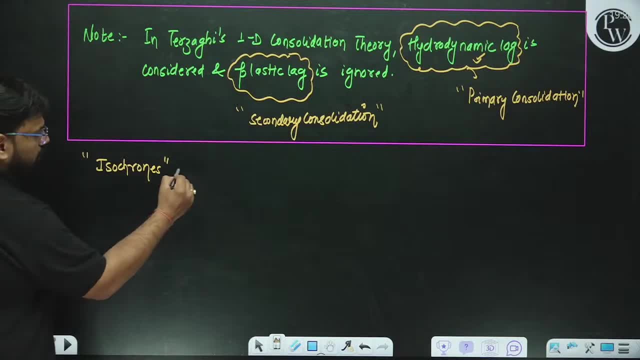 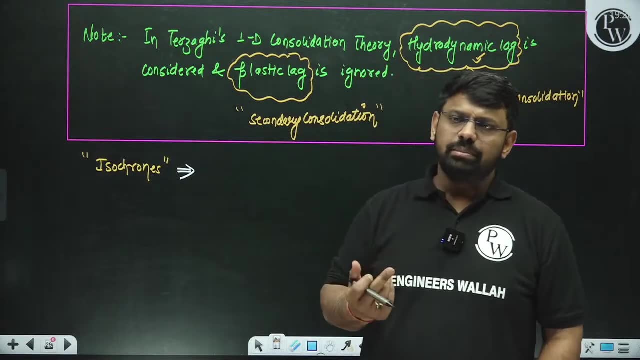 What is the meaning of Isochrones? What is the meaning of Isochrones? So look, Isochrones which we have. basically, what does it show? It shows the variation of the pore water pressure with time and depth. 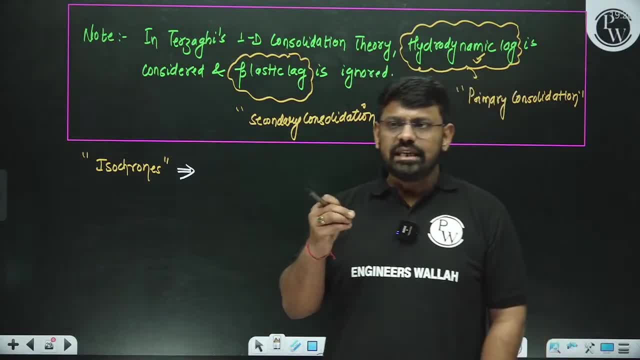 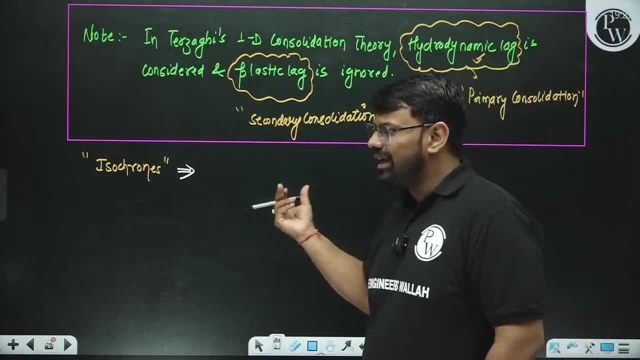 We call it Isochrones. So Isochrones basically indicates the change in pore water pressure with respect to time and depth. What do we call it? We call it Isochrones, So basically it indicates. it indicates. 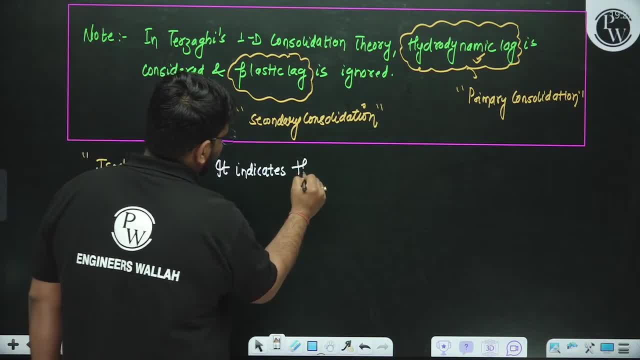 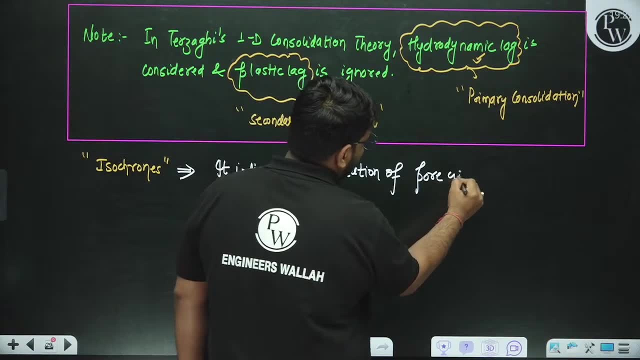 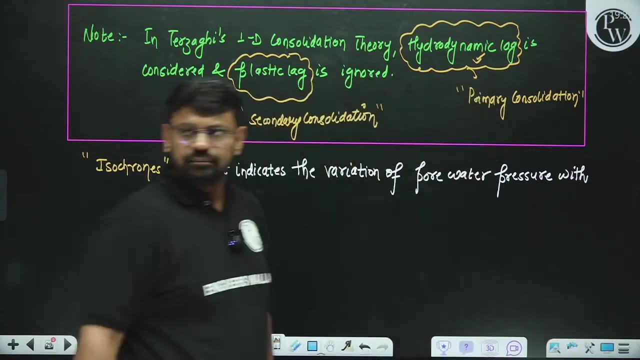 it indicates, indicates the variation. it indicates the variation of variation of pore water pressure, with variation of pore water pressure, with time and depth- Okay, With time, So here you have to understand this. with time and depth, so here you have to understand that. 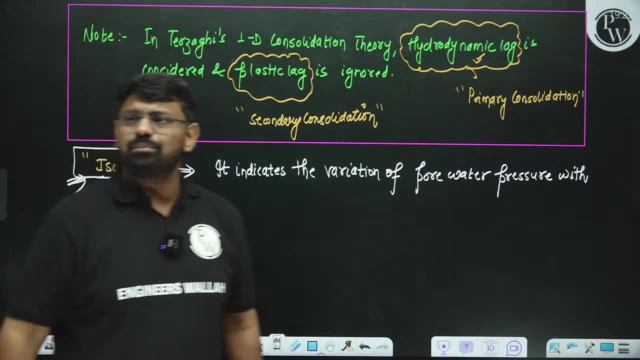 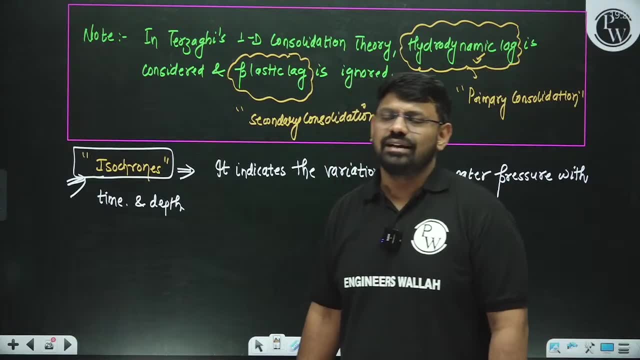 Isochrones does not mean that you have the same pore water pressure, right. Isochrone does not mean that the same pore water pressure is fine. Let's join equal height. Look, Sakshi is telling Son, there are contour lines where you join the points of equal elevation right. 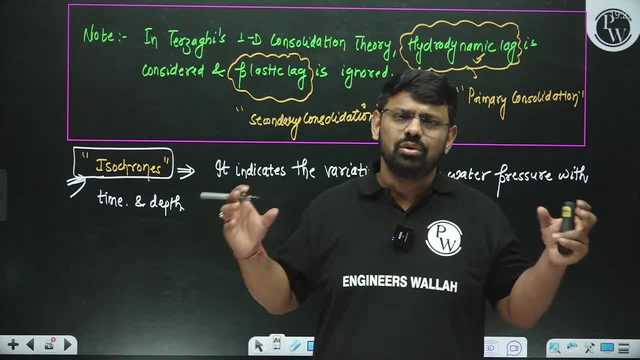 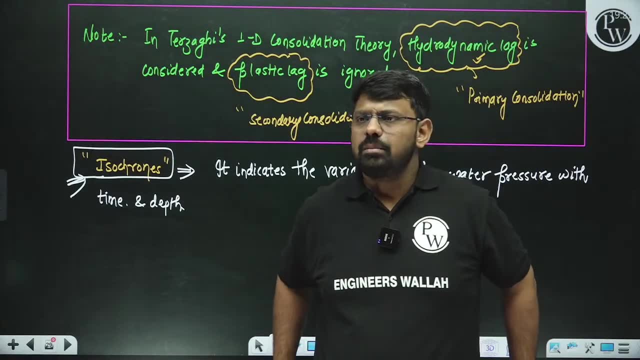 You don't have to mix all the things- Surveys, soil- you don't have to mix everything. If you mix all the fluids like this, then if you mix mud and water, it will become dirt. right, We don't have to fall in dirt. 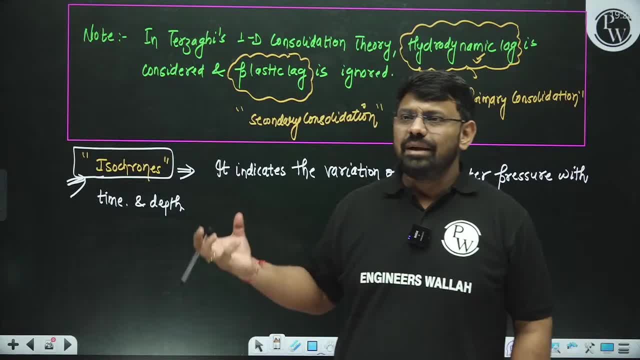 So the equal height that you are telling is what They are: contours. Here I am telling you isochrones, okay, So isochrones, if your language is written. try to understand the statement, Sir. it tells the variation, Whose variation. 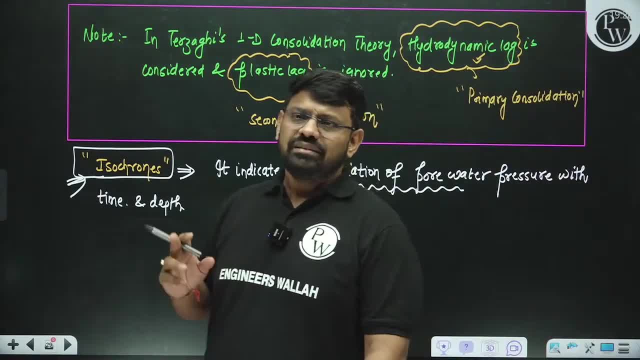 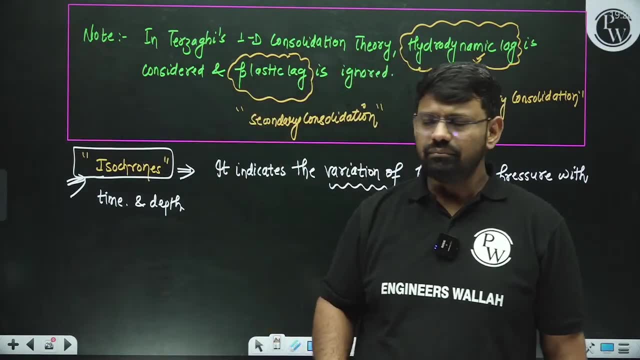 It tells the variation of pore water pressure with time and depth. But here the confusion should not be that, Sir, we have that, both are equal. But this should not happen Right, And when you hear iso, you remember the equal one. That is why I have told you separately. 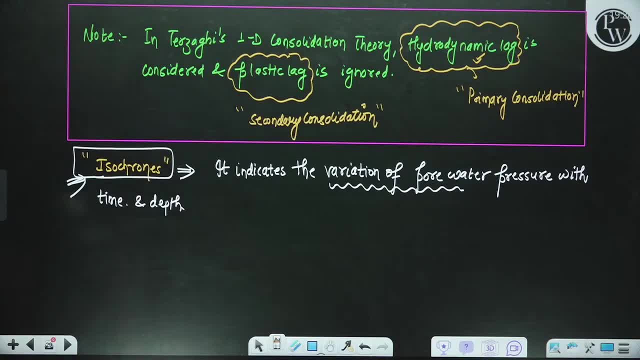 It means we have this. Okay, sir, The things are absolutely clear. Now, look, I have told you the equation of this type, Sir. the equation of this type, when you solve this differential equation, when you solve this differential equation, 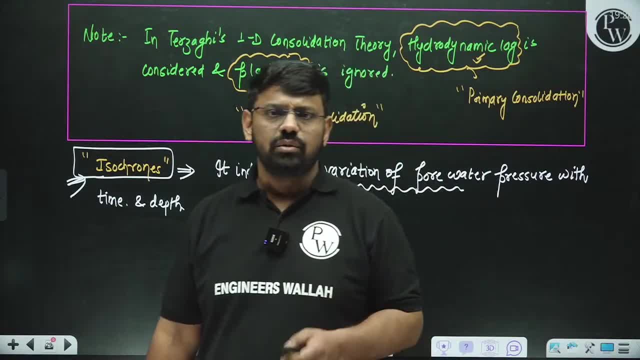 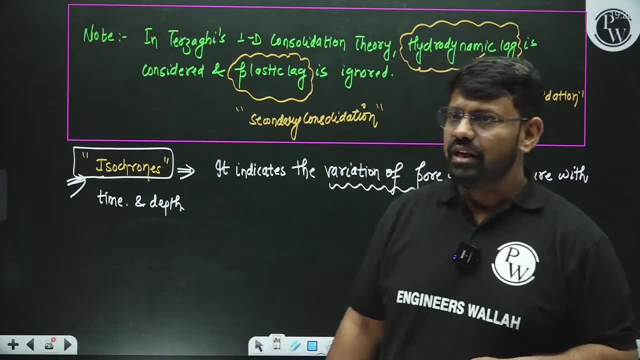 then you get to see different types of parameters, Some different types of. what do you get, Sir? we get to see different types of dimensionless parameters. So when we solve the equation of the type, then we get to see three types of parameters. 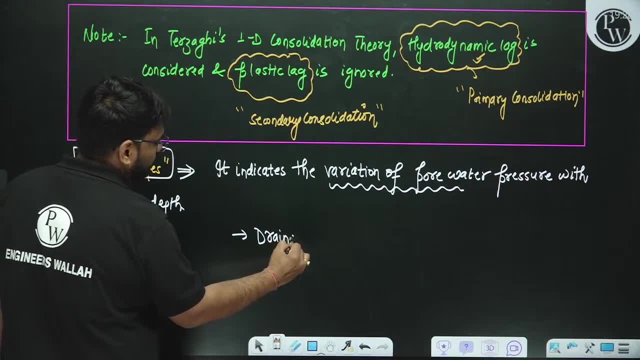 Sir one is the drainage path ratio. What is this, sir? Sir one is the drainage path ratio And sir one is the time factor. Time factor And sir one is the degree of consolidation. What is it? Percentage consolidation or degree of consolidation? 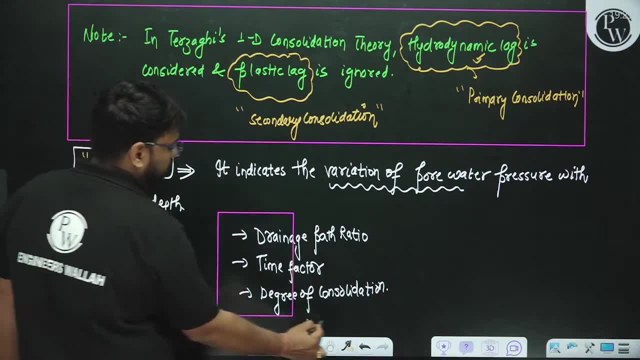 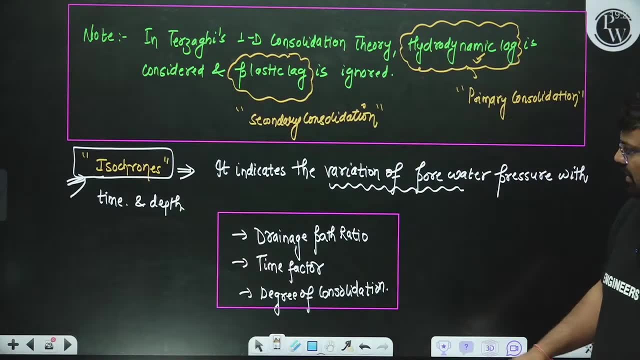 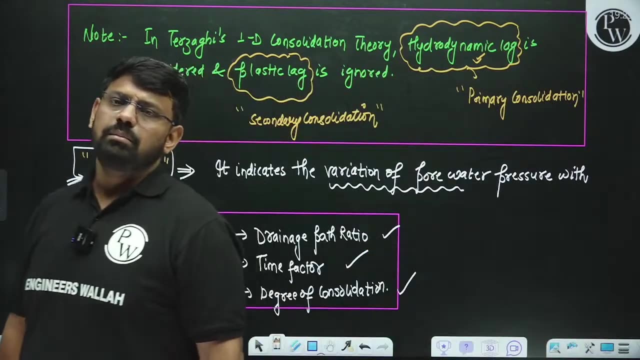 And what will these three be, sir? These three are dimensionless. We have these three dimensionless parameters here. Okay, we have this: Drainage path, ratio, time factor and degree of consolidation. We get to see these three dimensionless factors. 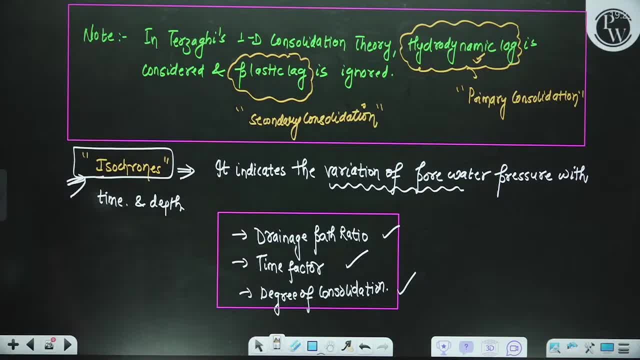 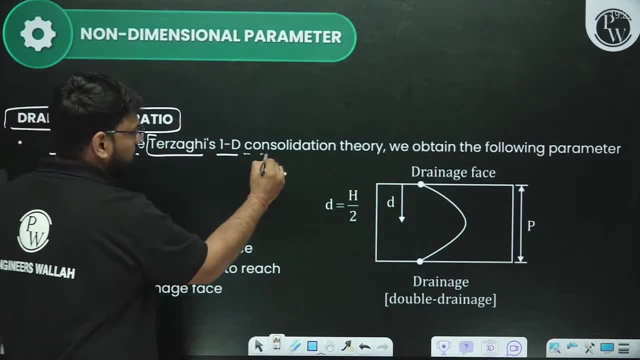 The thing is absolutely clear. Okay, sir, Now look ahead. Now, first of all, let's talk about the drainage path ratio. So what happened, sir? By solving the Terzaghi's 1D consolidation theory, we obtain the following parameter: 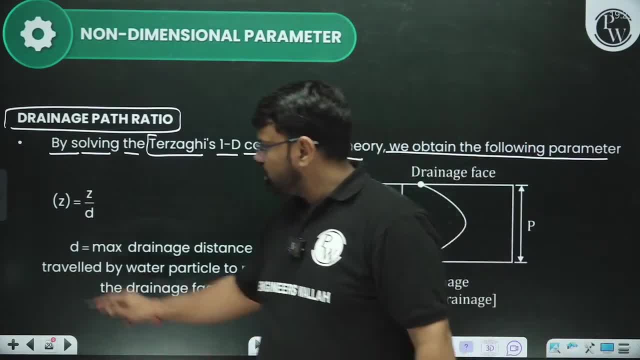 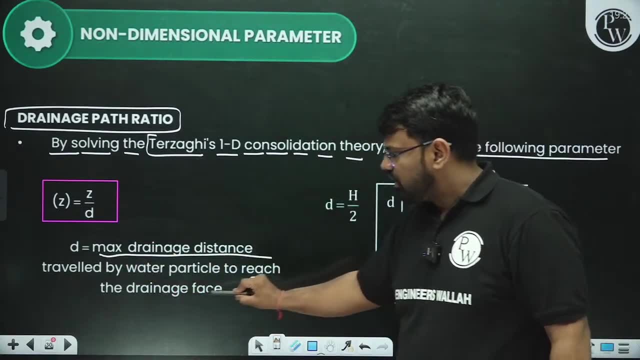 First of all, you have the drainage path ratio And this drainage path ratio that you make, that is basically Z by D. What will D be? D is basically the maximum drainage distance travelled by water particle to reach the drainage face. Sir, we talk about two types of things here. 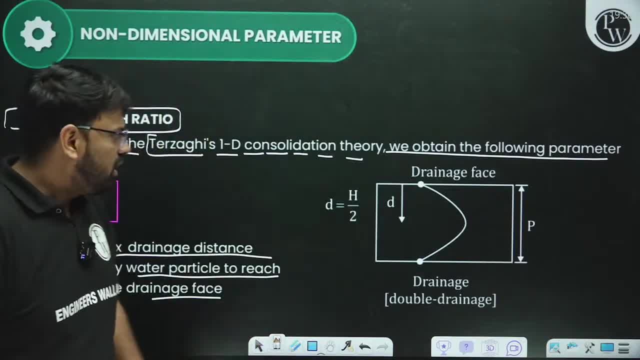 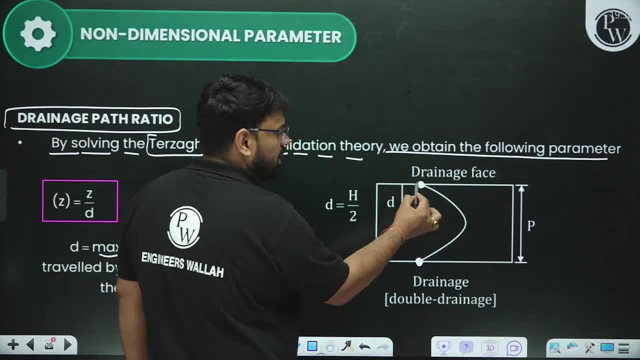 One. we have single drainage, One we have double drainage. So if you have see, if this is also a drainage face, and this is also a drainage face, meaning water can go from here to here, at both the places. it means, sir, the drainage path. 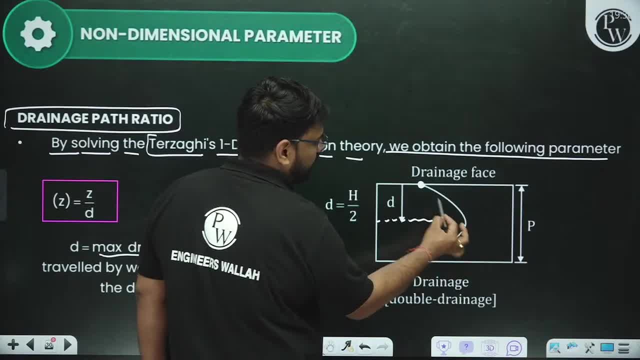 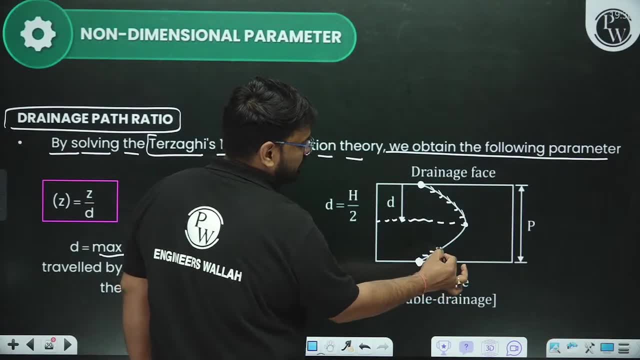 see now how far will any particle go to the maximum. Here also drainage is allowed, so the particle can reach here at maximum, And here also drainage is allowed, so the particle will go from here to here at maximum. Sir, how much drainage will you have at maximum? 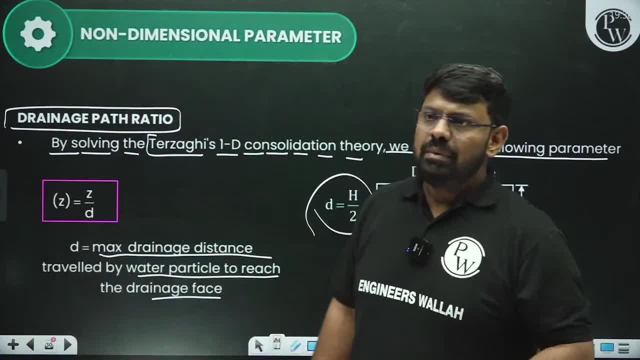 Sir, your drainage will be equal to H by 2.. Sir, how much drainage will you have at maximum, Sir? what will you have at maximum, Sir, the drainage will be equal to H by 2 at maximum. Okay, So D is equal to H by 2.. 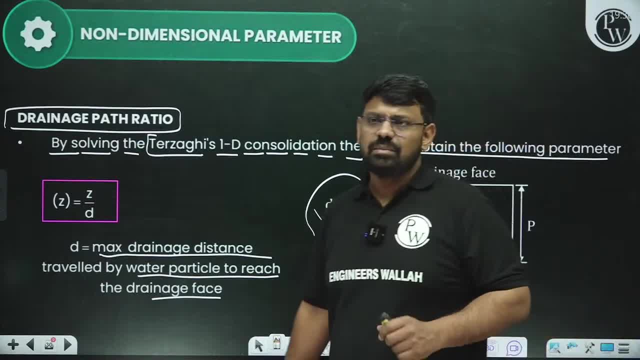 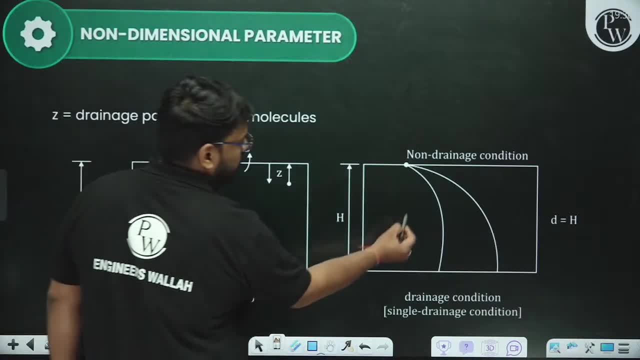 We get to see maximum drainage here If we talk about single drainage. Okay, Vineet, no problem. Okay, If we talk about single drainage, then what will we have in single drainage, sir? In single drainage we have this non drainage condition. 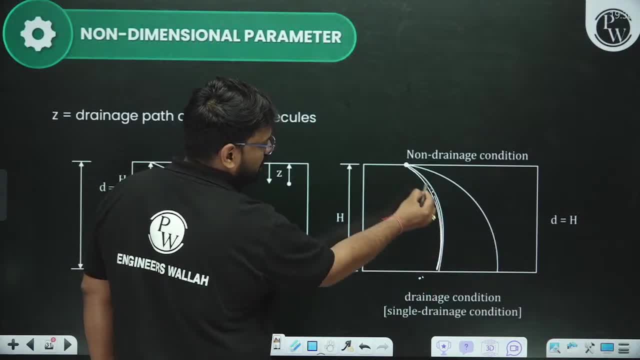 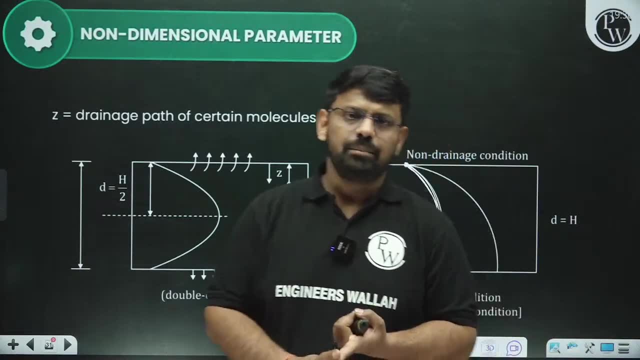 and this is your drainage condition, so the path will have to follow it completely. So here D is equal to H. We have to pay attention to these two things here. So the maximum drainage path that we have that will be equal to H by 2 in double drainage. 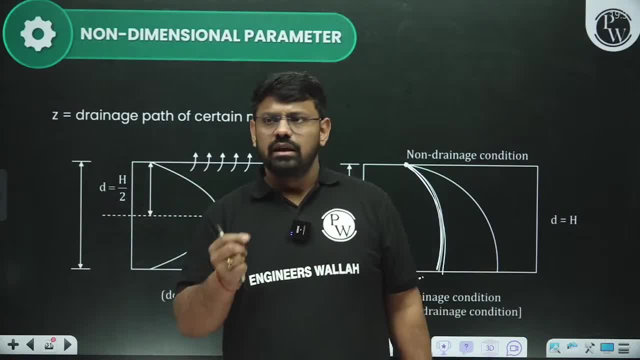 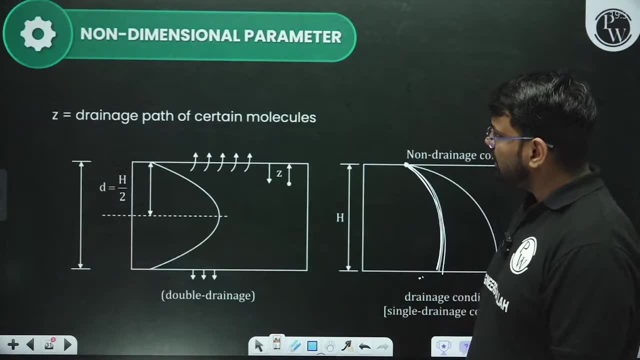 and in single drainage you will have to go completely. So this is first your. what do we have here, sir? This is called drainage path ratio. This is the drainage path ratio. Okay, And what is Z, sir? We have Z. 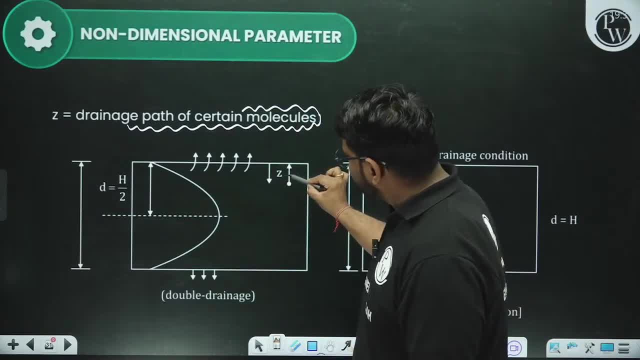 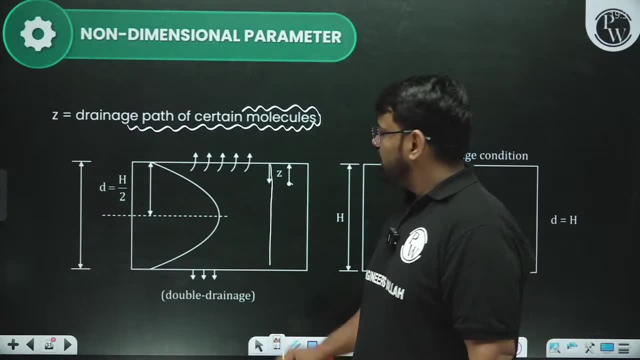 Drainage path of certain molecule. Drainage path of any particular molecule, For example. this is a molecule. Its drainage path is going: You have Z. Okay, This is how you get Z. So what does Z have? A molecule of a drainage path. 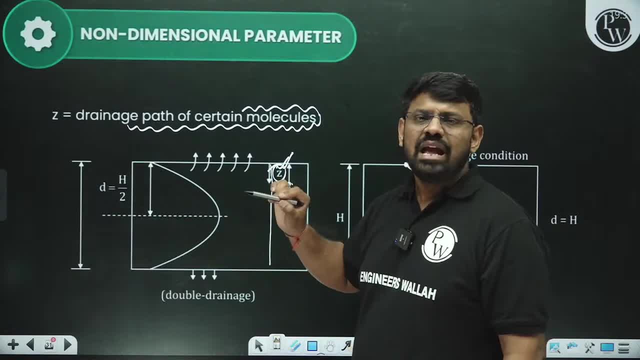 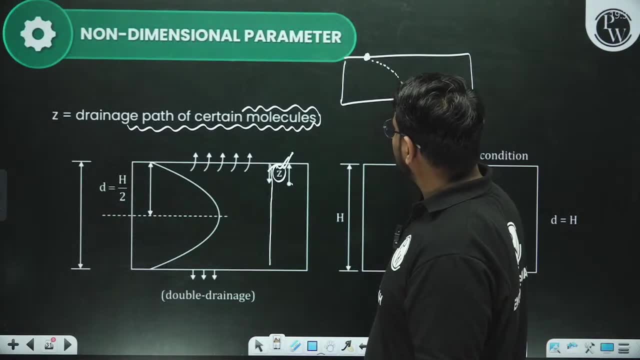 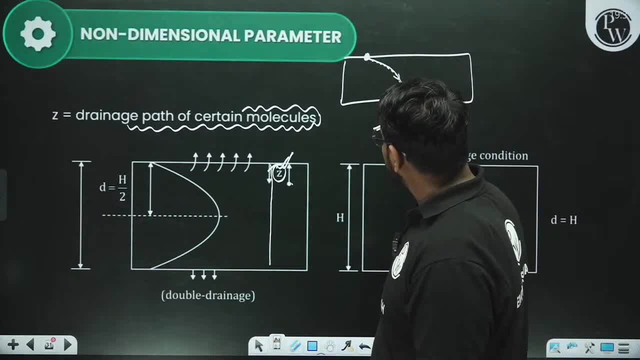 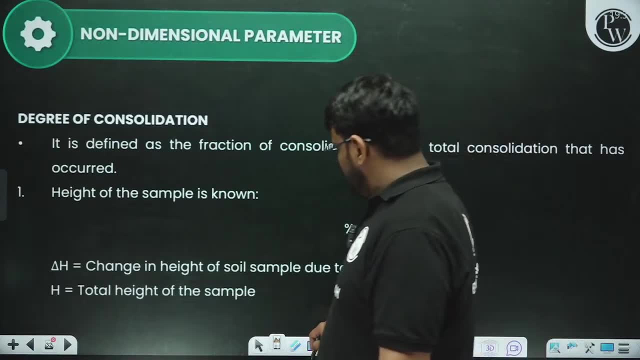 must be going somewhere. So this is its path, The direction in which the drainage is showing. that drainage path is called yours. We take out the ratio of this. The first thing is that this is understood. Second, sir, degree of consolidation. 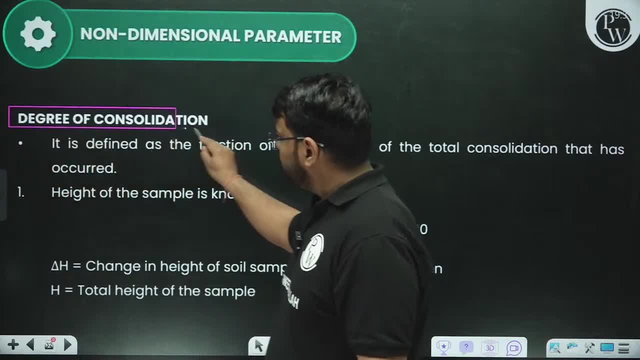 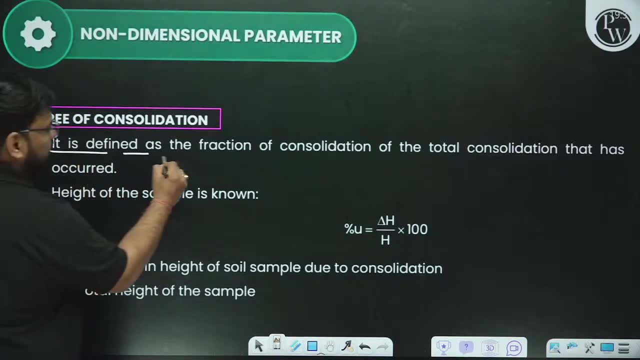 Degree of consolidation means how much percentage consolidation we have. Now what does percentage consolidation mean, sir? Understand this thing carefully. It is defined as the fraction of consolidation To the total. It means the percentage has been done in a way. Now the first way we have in percentage is: 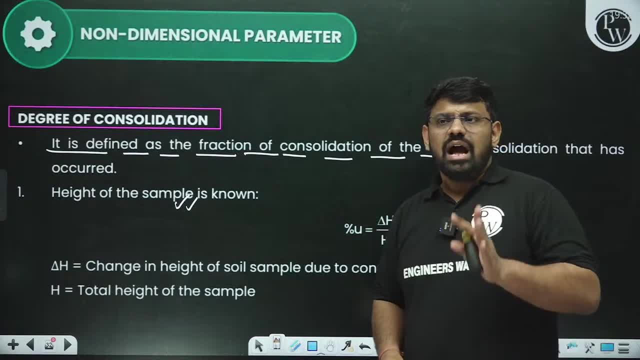 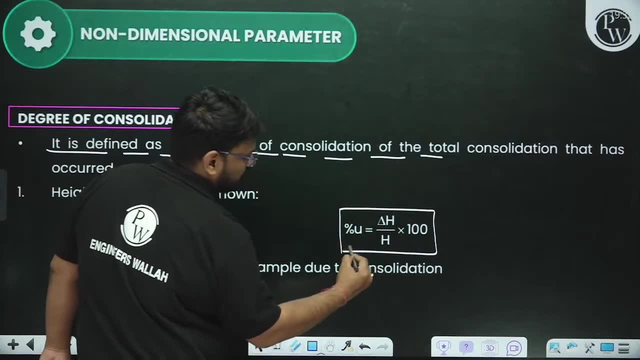 the height of the sample is known. If I have to calculate the height of the sample in this way, then see how the percentage consolidation will be Delta H by H. It means the height in which the variation came Divided by the total height. 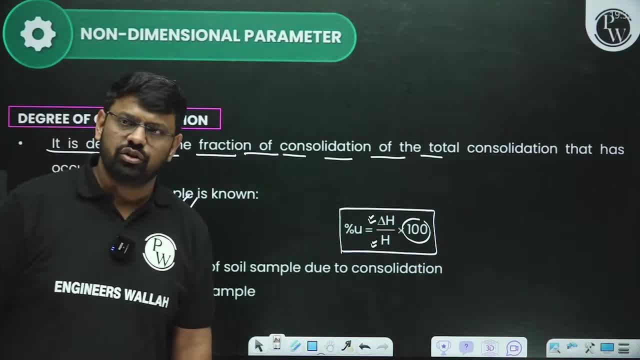 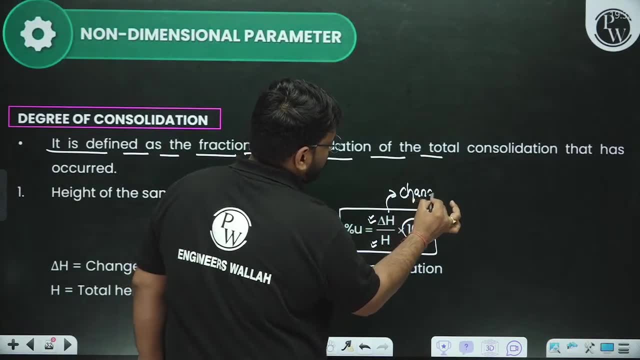 Multiply by 100.. We have this, sir, Percentage consolidation. Our first formula is clear: What is delta H, sir? Delta H is that change in height due to consolidation. So, due to consolidation, the change in height we have, the change in height we have. 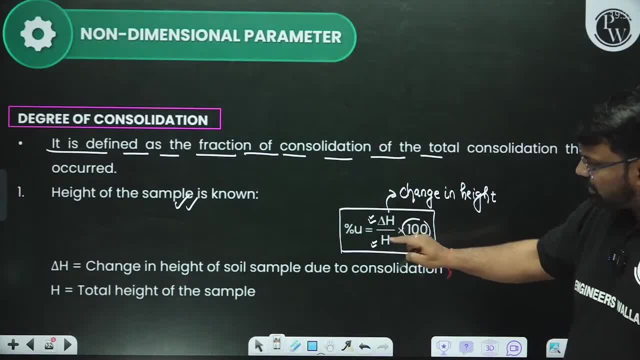 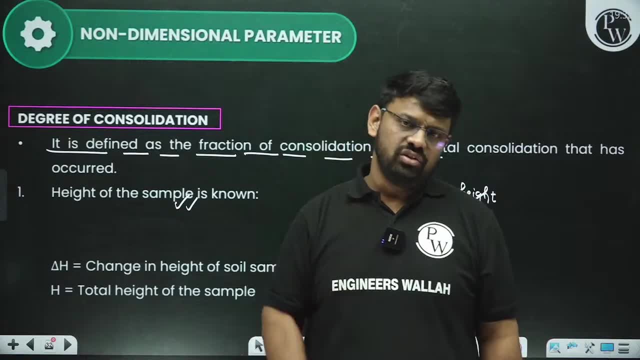 that is your delta H. So the change and the total height was: you took out the percentage, You took out the percentage. so from here you got to know the degree of consolidation or the percentage consolidation. This is the first method. The second method we have is: 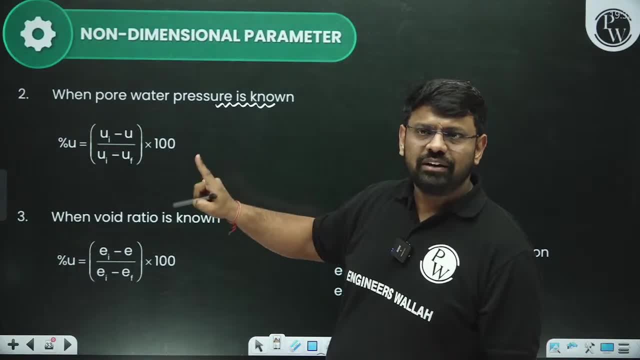 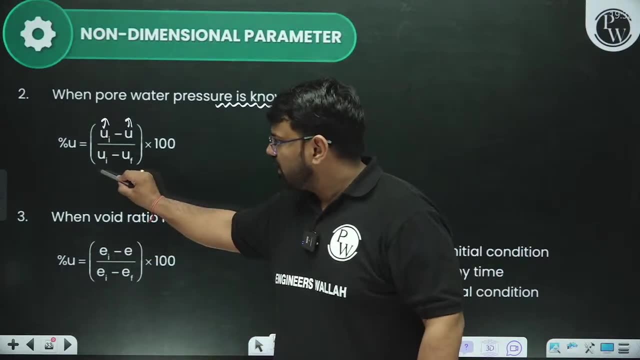 when you know the pore water pressure. So pore water pressure, like Sir, this is the initial pore water pressure. This is your present pore water pressure. It means from where to where it reached First thing And from where to where it reached total. 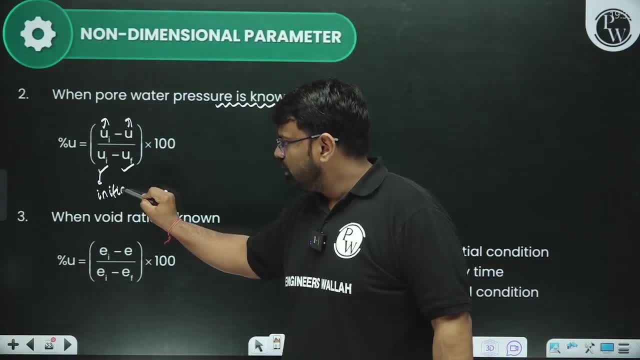 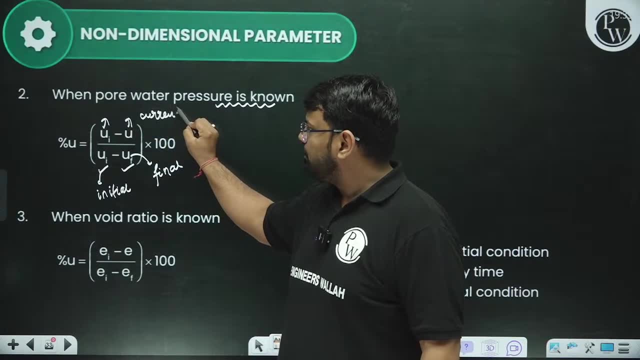 Means initial. We have Ui, sir, Initial, Ui is initial, And we have Uf, sir Final See Ui is initial And this is your current. The present pore water pressure will be. So what will you do from here? 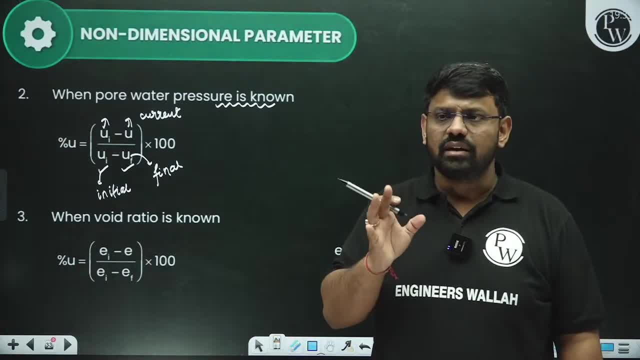 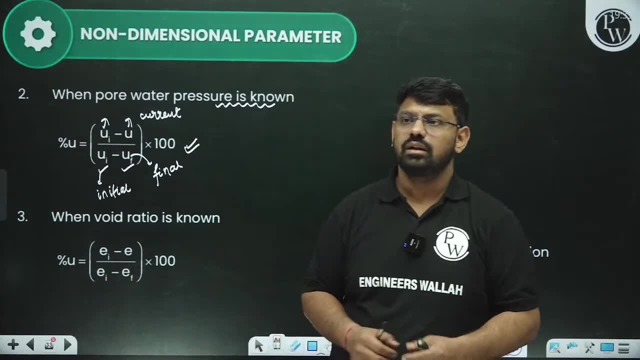 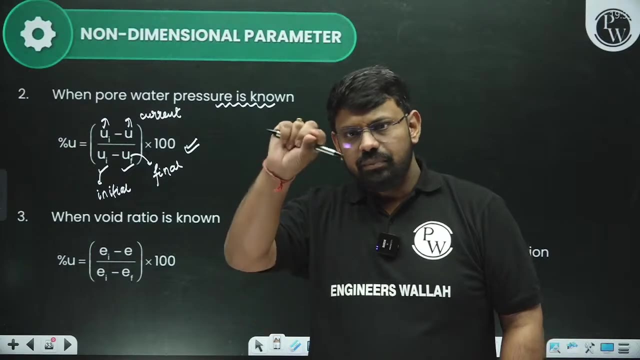 Here at any particular point. what will you calculate, sir, At any particular point? you will calculate here that how much percentage is coming out? Kishri comes in, Comes in right. Yes, You must be seeing the drainage path of the particle inside the soil. 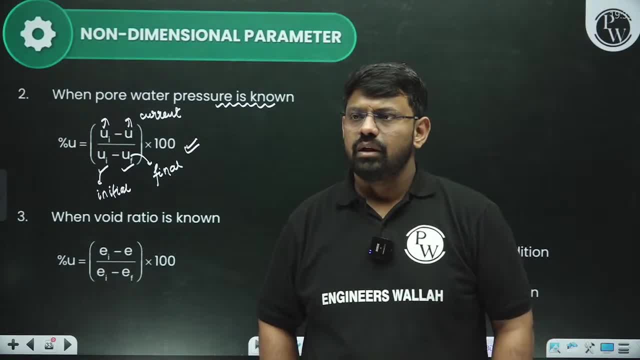 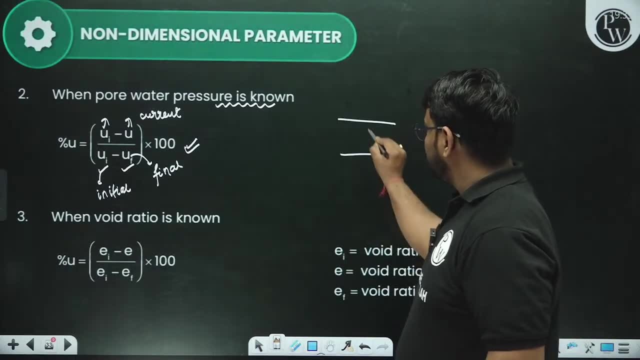 How will it go out? Yes, Is H the ultimate consolidation? No, What do you have? H? See, Understand. What do you have H? You have H. This is the total distance. Now, if vertical load is applied, then there must be some difference in height. 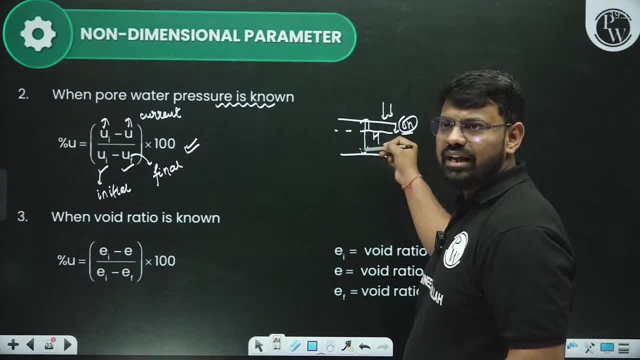 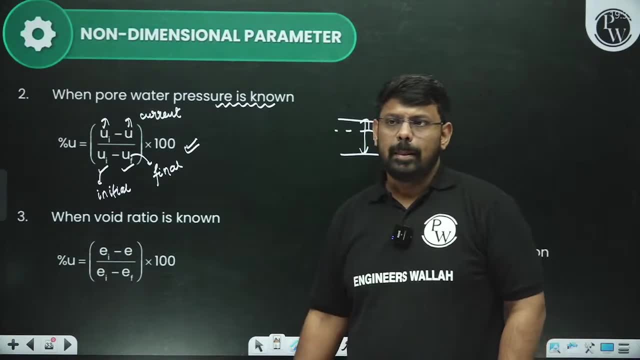 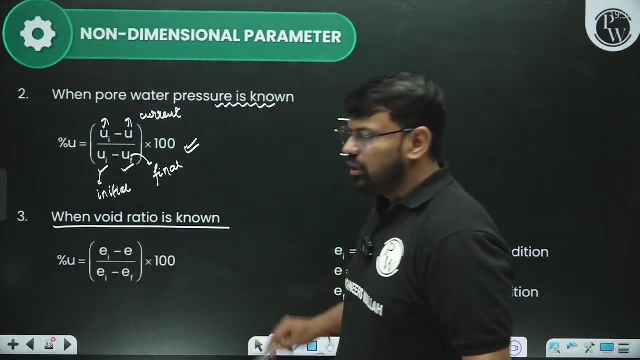 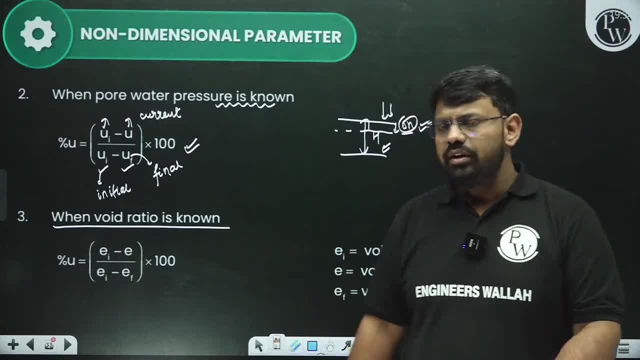 Sir, now the void ratio will be known. See the load you apply. it is directly true. We are getting to see changes in the void ratio too. So changes in the void ratio, like initial void ratio minus that current one, Initial minus final, and multiply by 100. 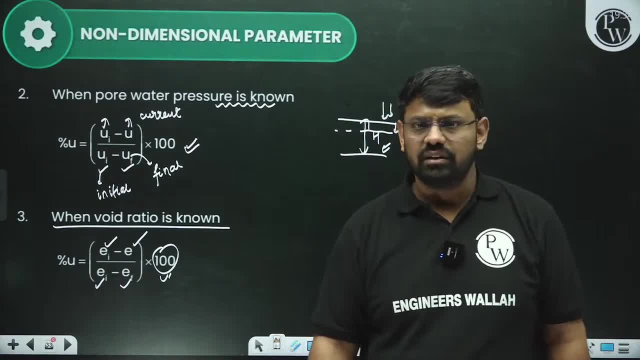 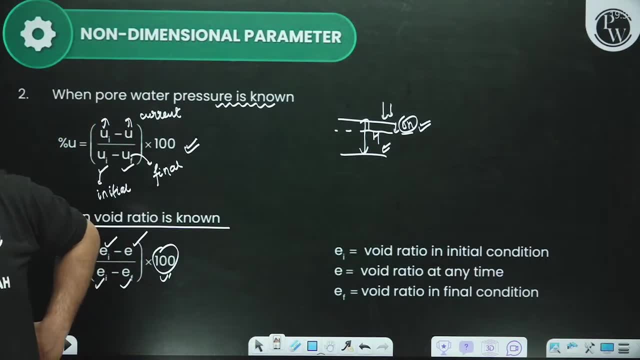 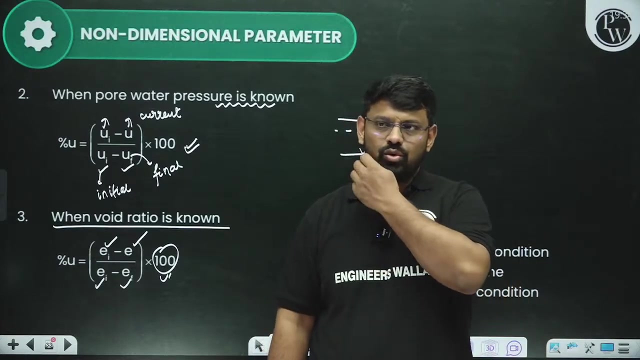 What do we have, sir? What do we have, sir? What do we have, sir? We have percentage consolidation Here you can see, This is the percentage consolidation. Okay, Okay, Okay, Okay, Okay. Drainage through the soil. Shubham Khorwal. drainage through the soil. 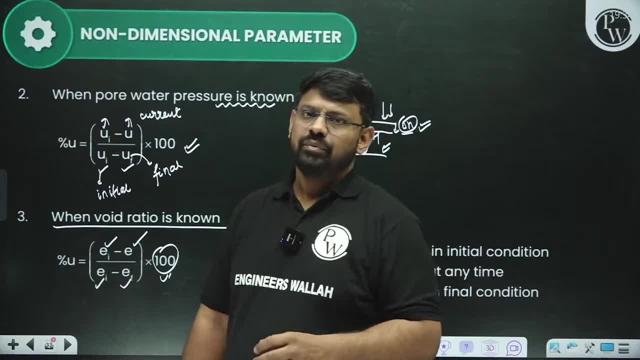 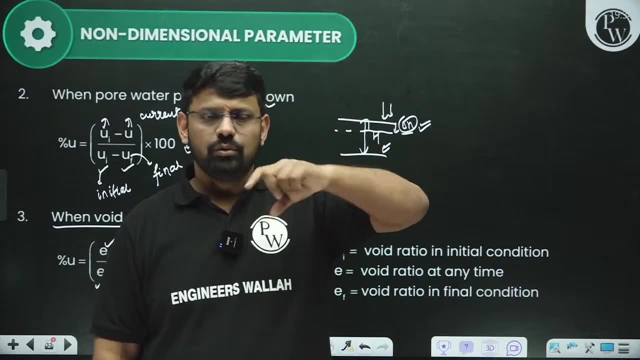 How will consolidation take place? Tell me, how will consolidation take place in this? Consolidation will take place when water is coming out of the soil. Water is coming out of the soil, So the path will go inside the soil. Water will go inside the soil, outside the soil, wherever it goes. 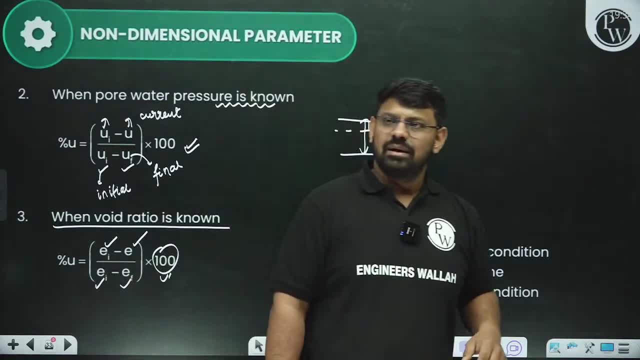 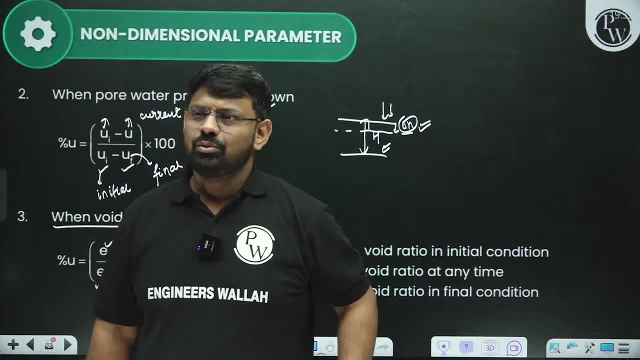 Tell me, what do you mean by that? What do you mean by that? There is a wise man among us, Ocean of Knowledge Study. He wrote a message and deleted it- That if everything happens by luck, if it happens by knowledge, then Birbal Bajshah would be there. 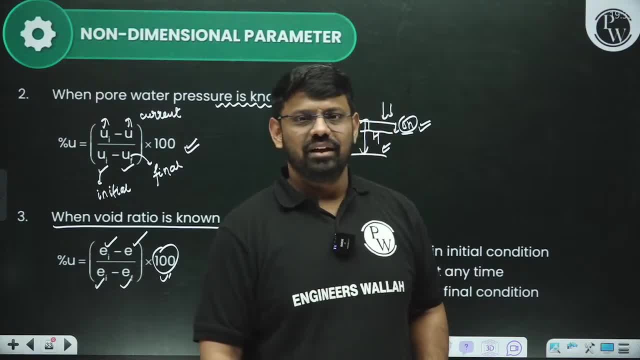 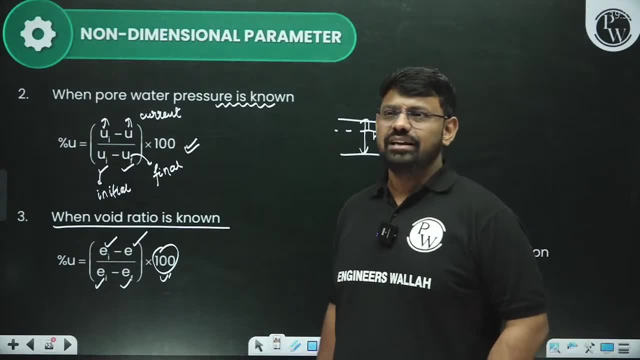 No, son, knowledge is good. It is not by luck. There are not many things by luck. Knowledge is good, Education is good, Knowledge is the light and it will take you forward in life. It will take you forward in life. 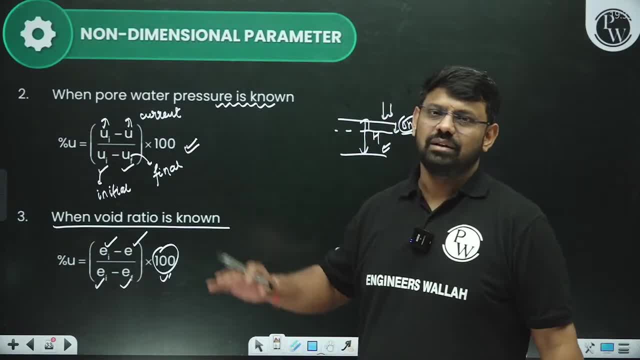 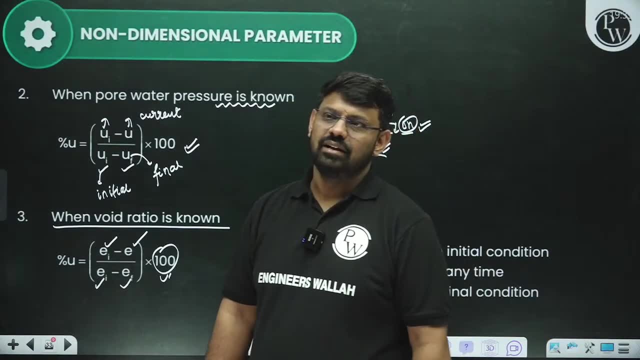 All the rest of the things are useless. All the rest of the things, by luck, by knowledge, by knowledge, are useless. Come on, okay, He says right. What does he say? I remembered one thing about your saying. I remembered about the matter of luck. 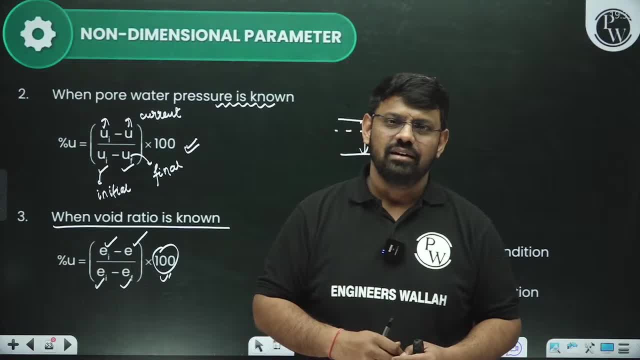 That neither there is a shine of stone nor there is a shine of stone. Okay, right, People wear stones and stones. I have worn one, So this does not mean that there is a shine of luck going on. Nothing like that is happening. 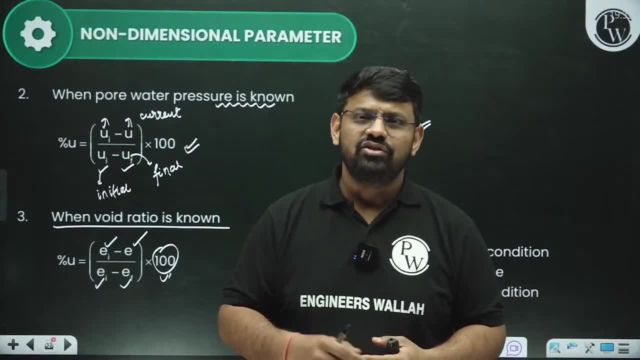 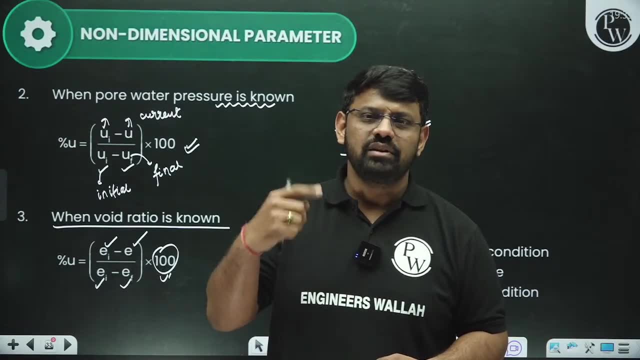 That neither there is a shine of stone nor there is a shine of stone. There is a shine of living on the face, And we heard nothing from the ancestors in inheritance. What we see is a shine of life and blood. So when you see this shine of somebody, 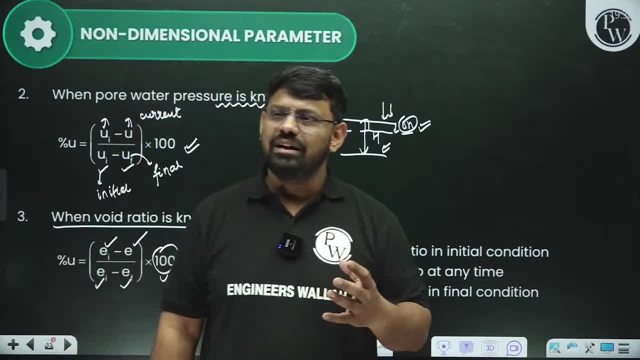 If you see a shine on your face who is working hard, then you will see a shine on the servant too, Do you understand? So this is the matter. So you get to see things only by working hard. So there is a shine of stone. 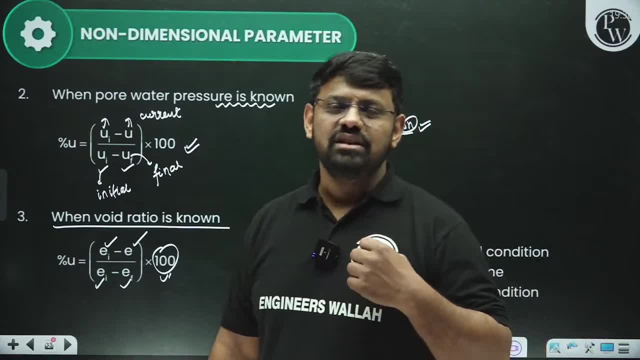 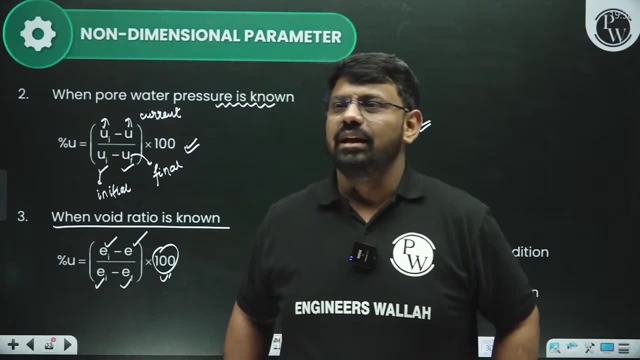 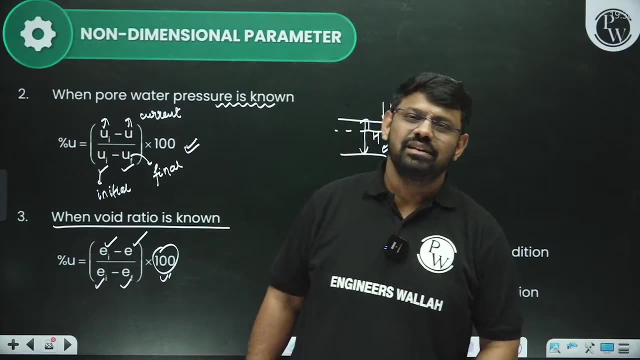 there is a shining flower. There is a shine of life and blood on the face, And we heard nothing from the ancestors in inheritance which we can see the shine of life and blood Right? Yes, Absolutely So there is a spark of blood and sweat. that is your real spark. 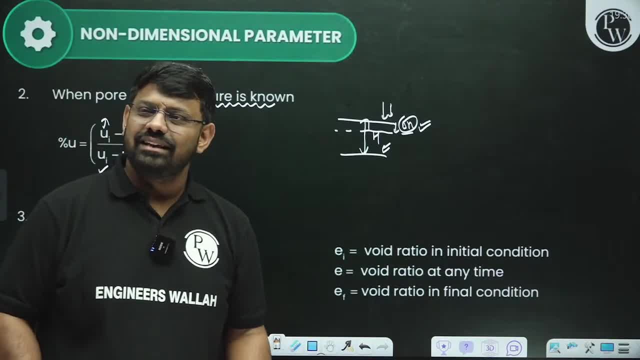 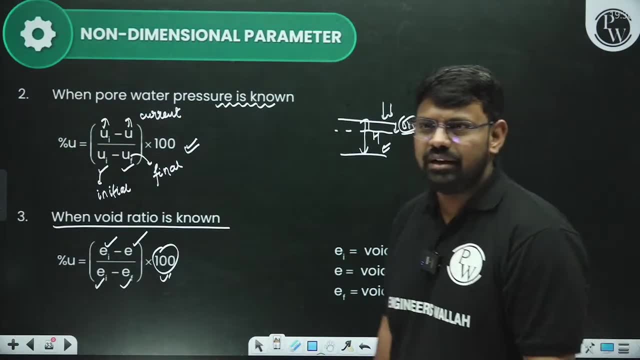 That is your real spark. See Rohit kumar, Dolly chai wali. Rohit wants us to say something or the other. Everyone has their own life. brother, He does not work hard, that he sits free and does something. 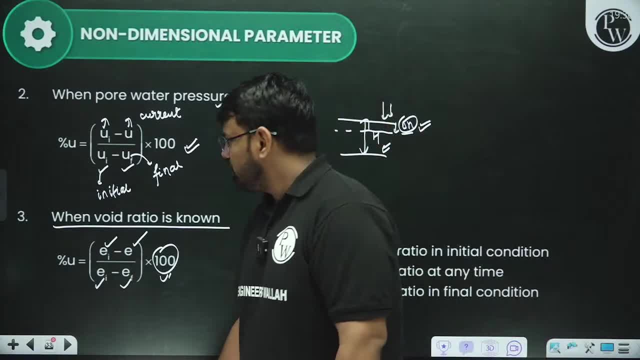 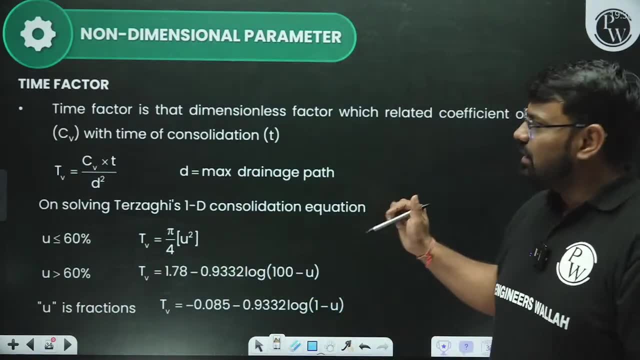 He has also worked hard. Right, He has also worked hard enough. Okay, sir, Degree of consolidation is done with us. Now come to the next. Come to the next line, Sir. next we have time factor, And this is very important. 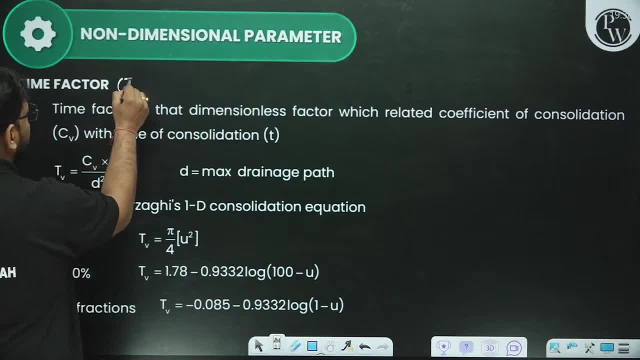 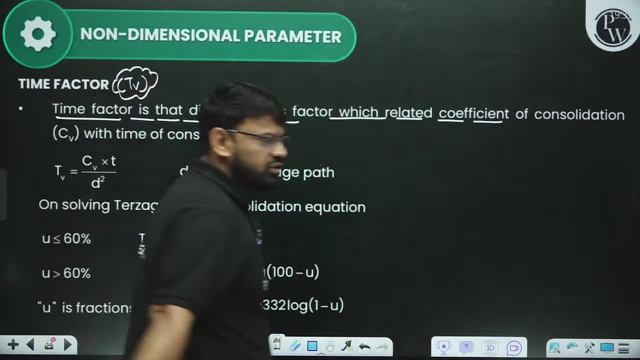 The question is definitely asked to you from here. Okay, Sir, you talk about time factor, about Tv. This is time factor. Now, time factor is that dimensionless factor which is related to coefficient of consolidation, Which is related to Cv, With time of consolidation means T. 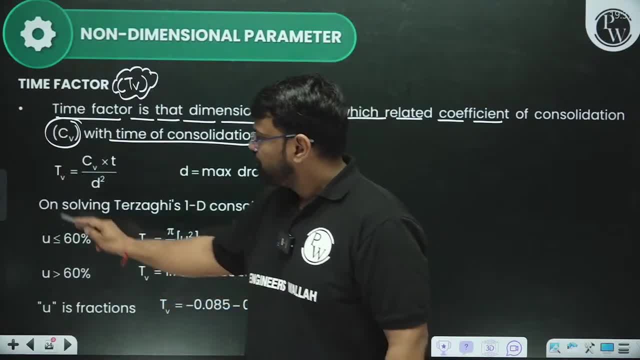 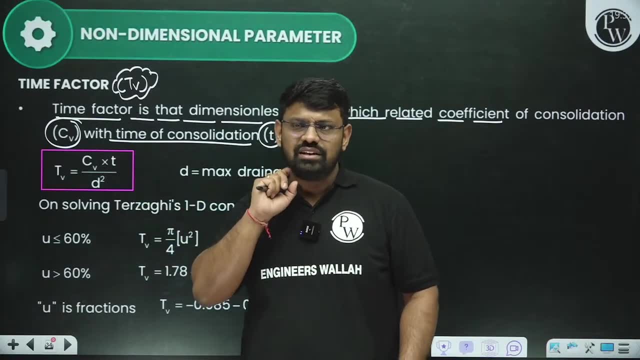 So remember one formula here, sir, in a good way: That Tv is equal to Cv, T by D square. Now, how do you get questions from here, sir? Right From here you are asked questions. of what kind? From here, you are asked questions. 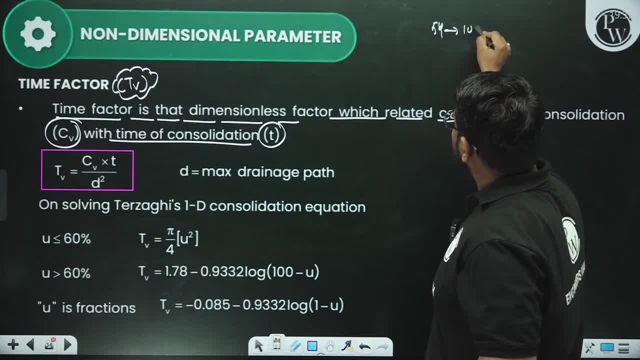 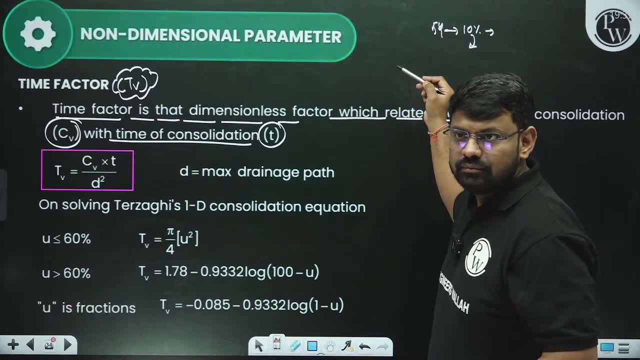 Sir, if in 5 years so much percent- suppose 10%- consolidation happened, He took so much time, So in the same percent consolidation. Okay, In the same percent consolidation if you have 10 years means single drainage. 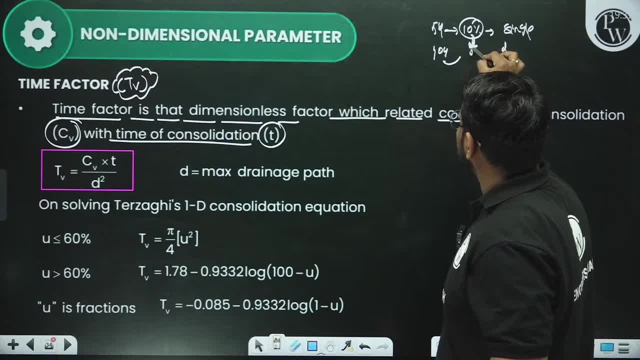 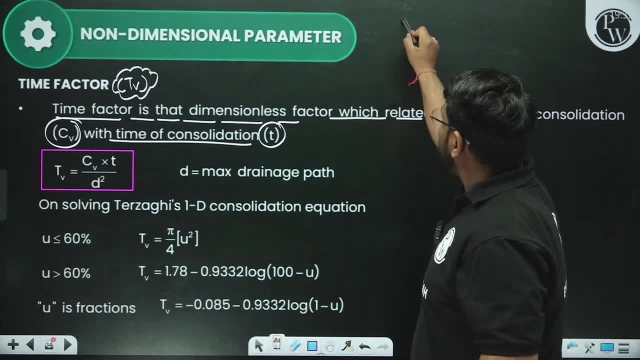 So how much time will it take in the second double drainage In the same percentage of consolidation? These kinds of questions are asked to you. So what do we have to do, sir, If in 5 years, suppose 60% consolidation happened? 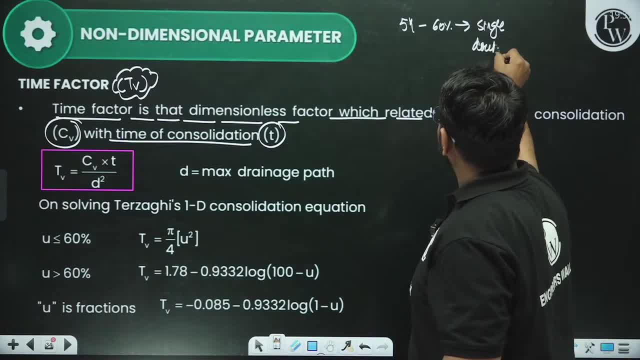 And it happened in single drainage condition. So tell me, in double drainage condition, how much time will the same percentage of consolidation take? These kinds of questions are sometimes asked to you in exams. So where will you solve that? Sir, you will solve this formula. 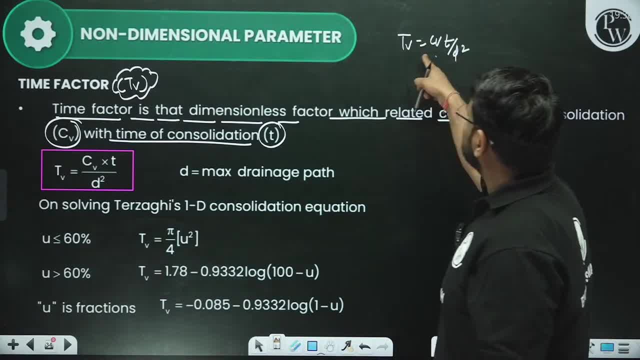 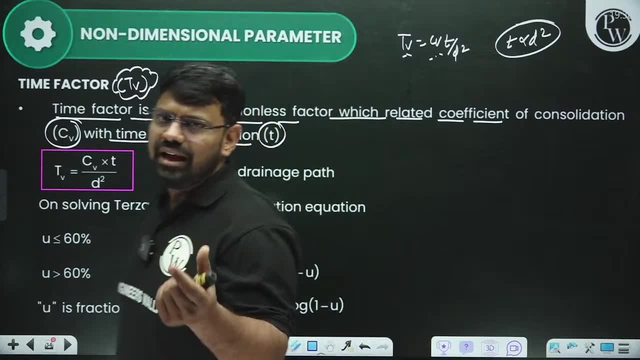 Tv is equal to Cv, T by D square, So these two are equal for any particular soil. So your time will be directly equal to which It will be equal to drainage path. If you have single drainage condition, then, sir, it will be equal to H. 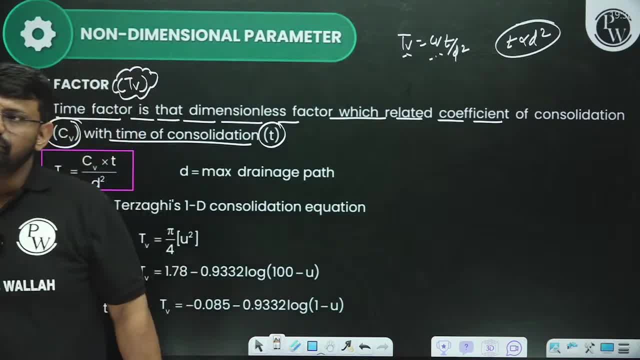 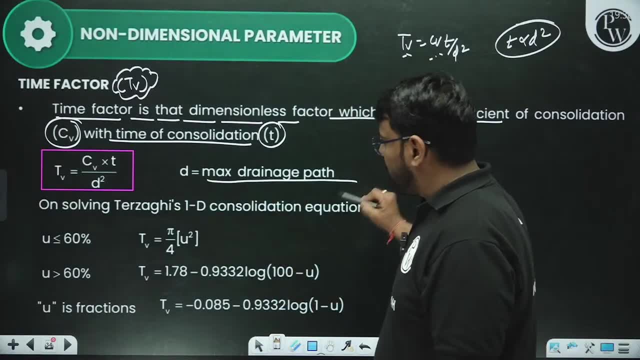 If it is double drainage, then it will be equal to H by 2.. Okay, So this is what you have. It is absolutely clear. So here see D drainage. maximum drainage path is done. Now, if you solve this and you come to know that degree of consolidation is less than 60%, 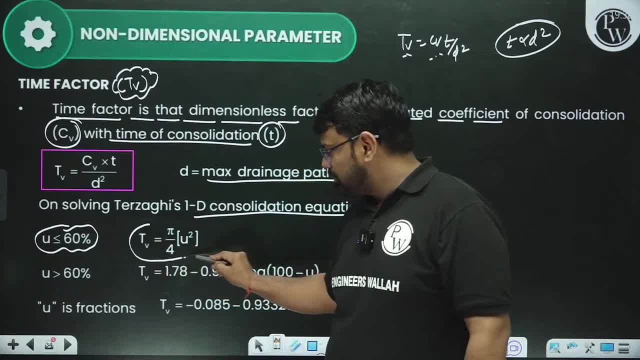 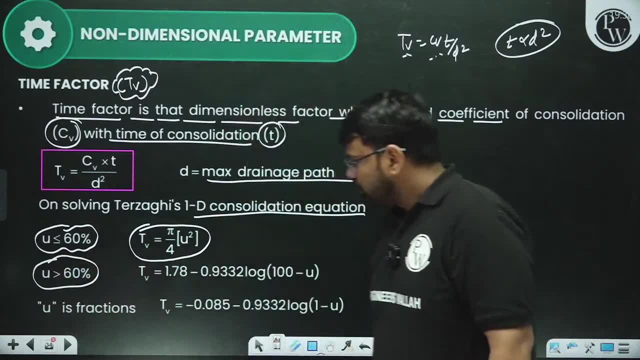 then how will you find Tv? So we have Tv equal to pi by 4 into U square. This is the Tv, Isn't it? Second, if the percentage of consolidation goes above 60, then, sir, Tv will come to us 1.78 minus 0.9332. log 100 minus U. 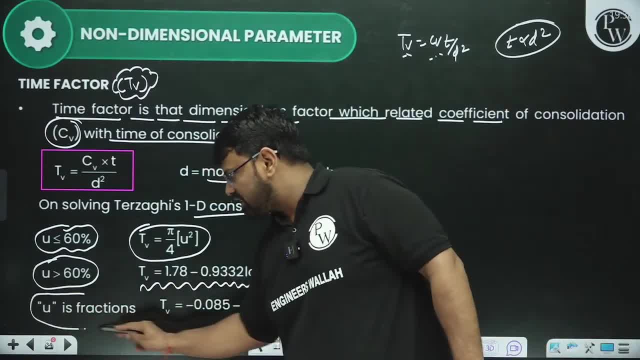 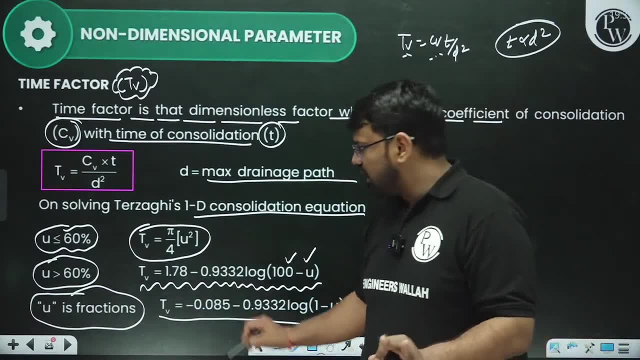 This will be with us, And if the percentage comes in our fraction, then you can see it in this way. So you can remember three formulas from here. The most useful formula for you will be this formula. From here, you can also be asked for numericals. 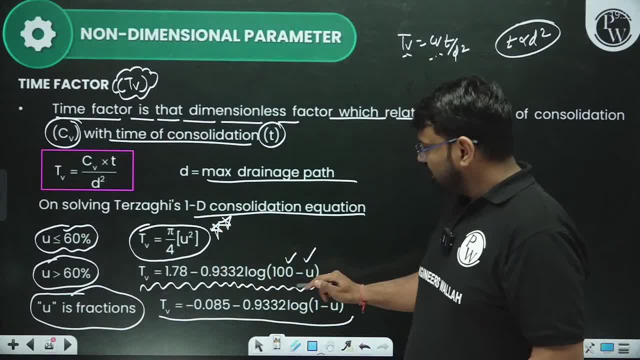 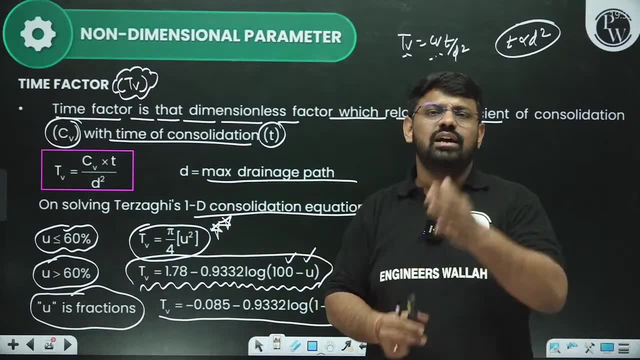 So remember this formula: pi by 4 into U square. And along with this formula you can be asked that: tell me is this formula correct or not? They will give you the formula directly. You will be asked: tell me four options. 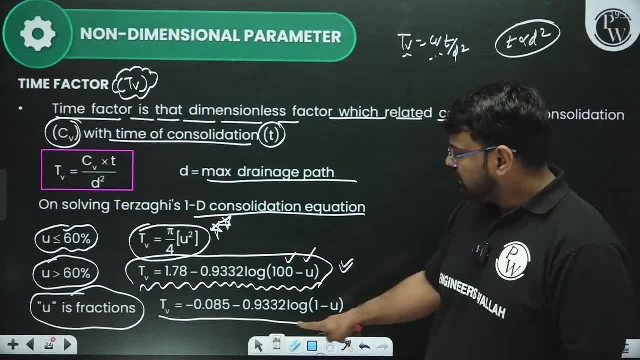 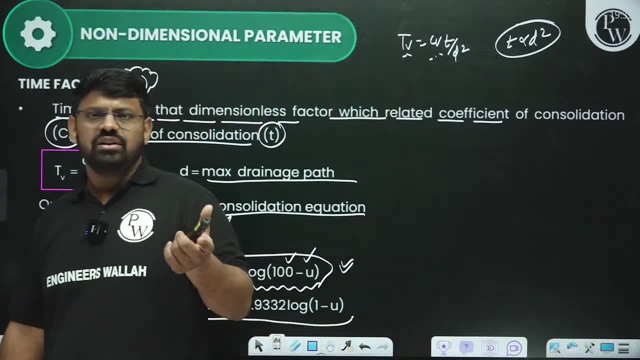 Which one is the correct one among them, Isn't it? So remember this formula too. This has not been asked much yet. This has not been asked much yet. Absolutely, Akash. very good. When the time factor is 50%, then some children have also remembered. 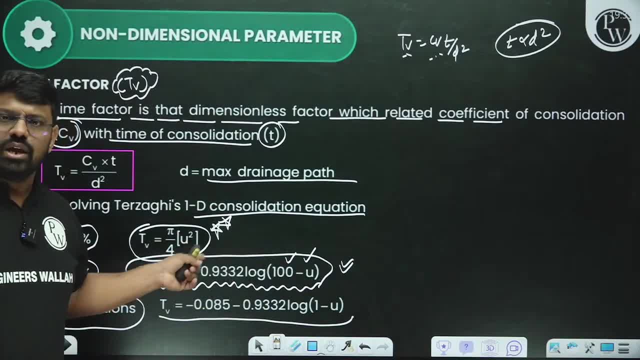 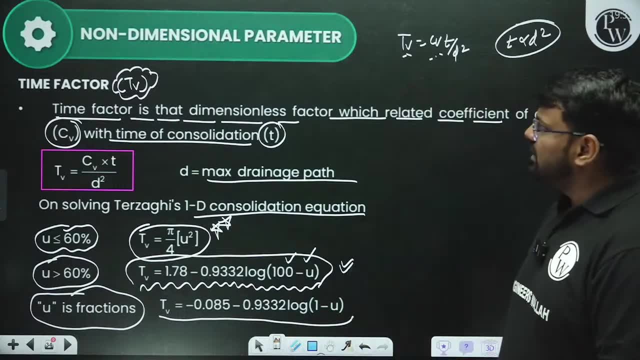 Sir, if you put the value of U here as 50%, then you get this value as 0.196.. So if you remember some data in this way, then you benefit in the exam. Okay, We have to understand all these things. 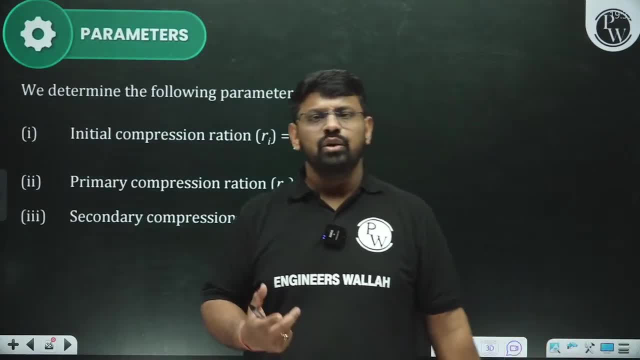 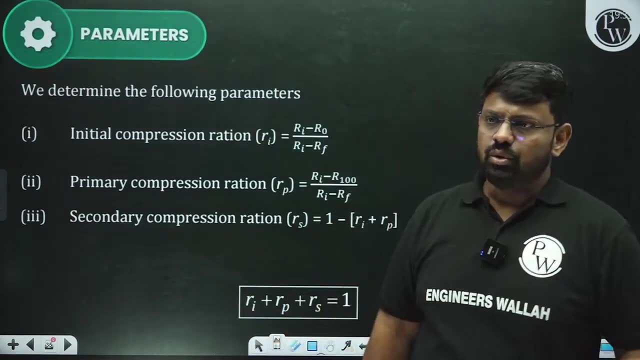 So we have seen all three factors, Sir. we have seen percentage consolidation, Sir, we have seen degree of consolidation And we have also discussed the time factor here. It is absolutely clear. Now look further here, sir. What do we have further? 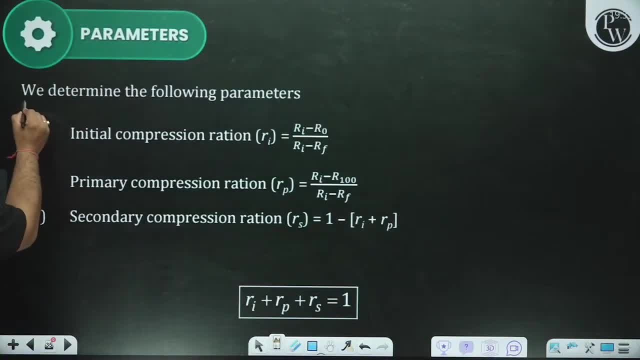 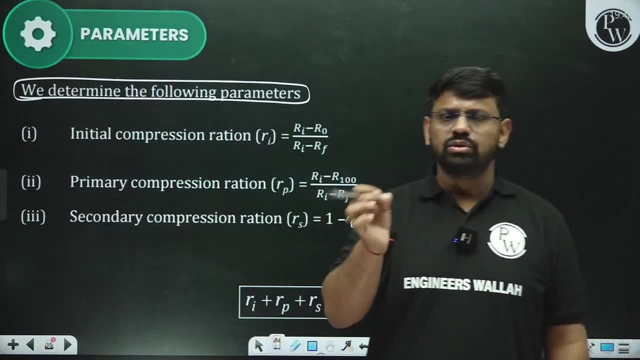 Okay, What do we have further? See, we take out some parameters. We take out some parameters, Okay, From the curve fitting method. Okay, From the curve fitting method. There are two types of curve fitting methods. We calculate some parameters from them. 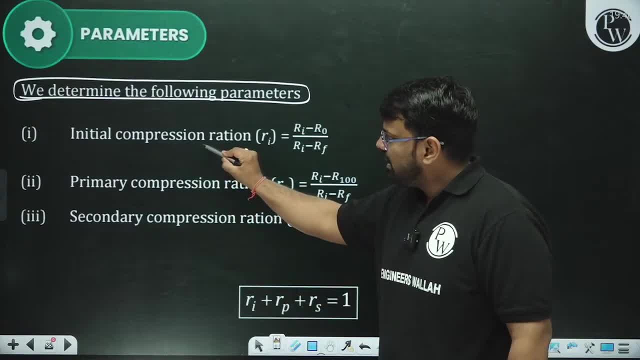 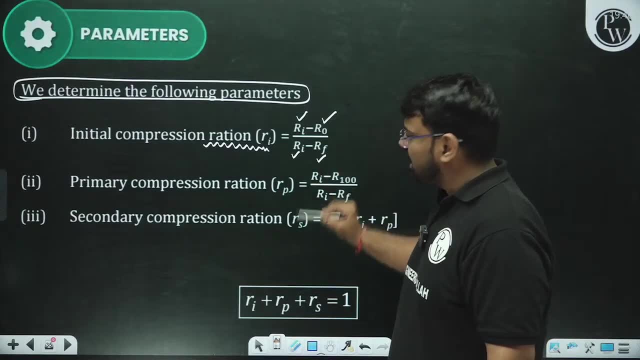 And how do we understand those parameters, Sir? first, we have the initial compression ratio. Okay, Which is nothing but your R? i minus R naught divided by R? i minus R f. Sir, what is R i R f R naught? 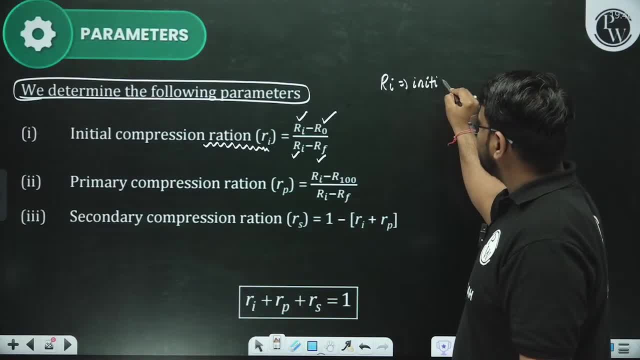 Sir, you have R i as initial dial gauge reading. What is that, sir? This is basically your initial dial gauge reading. So this is initial. Sir, you have R naught as dial gauge reading on 0% consolidation. Okay, 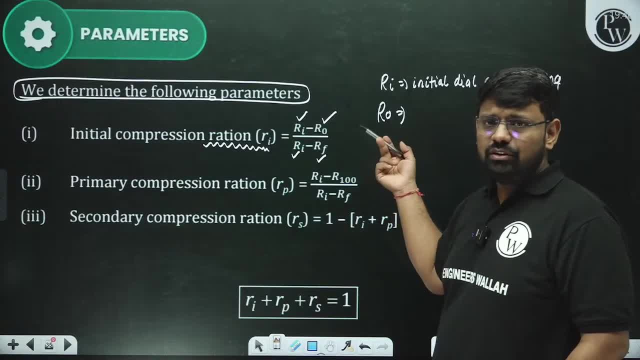 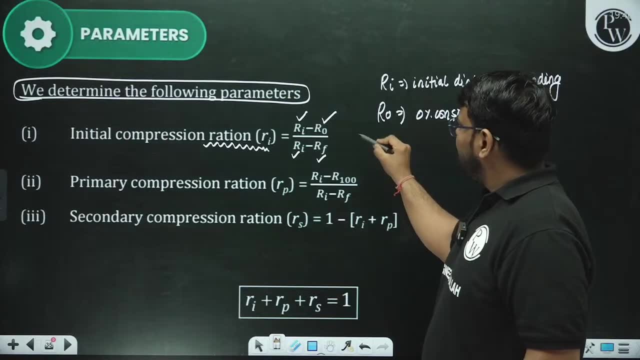 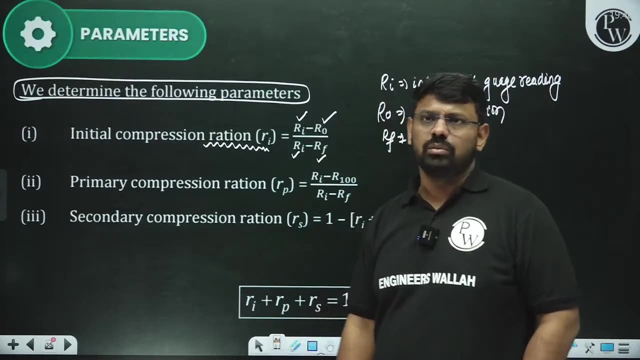 So when R naught is there, you will get dial gauge reading on 0% consolidation. So you will get 0% consolidation. Okay, So when R i becomes initial, you will get R f as final reading. So when R i becomes final, you will get R f. 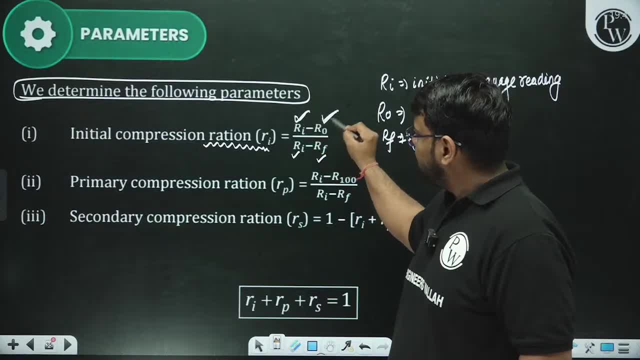 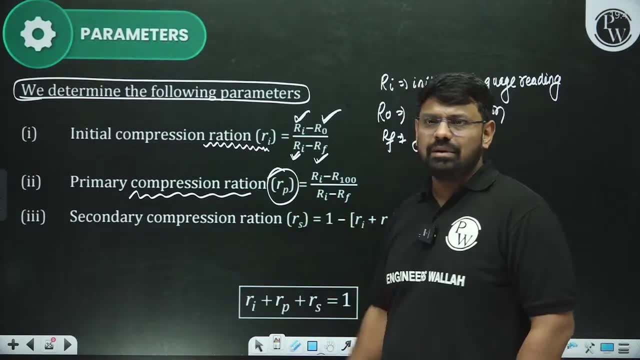 So initial compression ratio is R i minus R naught divided by R i minus R f. Look at the second point. If I talk about primary consolidation ratio, that means the ratio of R p. we have R i minus R 100 divided by R i minus R f. R 100 is equal to R? i minus R f. divided by R? i minus R f. R i minus R 0. divided by R? i minus R f, R i minus R 0. divided by R? i minus R f, is equal to 1.. 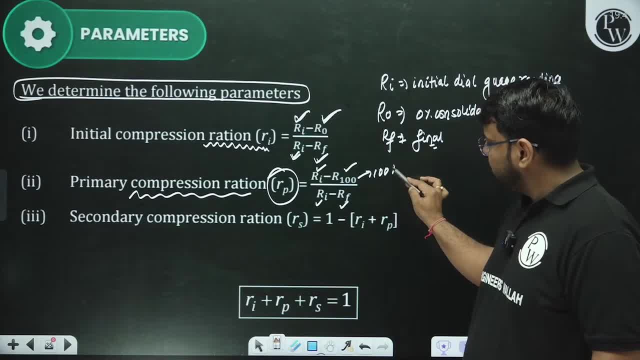 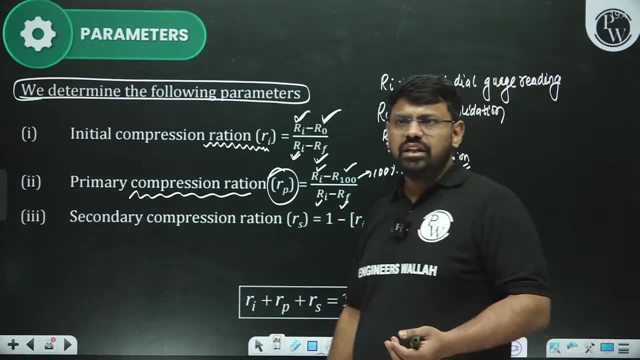 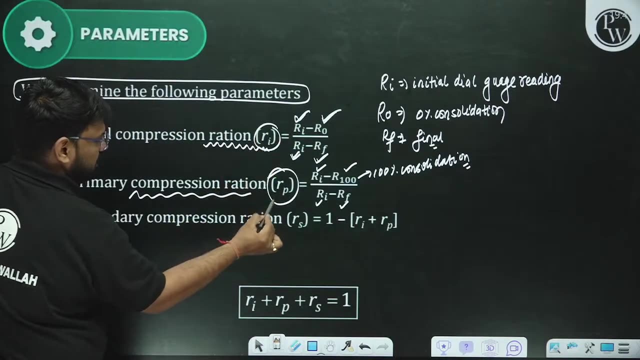 Ri minus Rf R100 is the corresponding reading of 100% consolidation. This reading is corresponding to 100% consolidation. We remove this from the curve fitting method, but you have to remember this formula directly. So, sir, this compression came. this initial compression came this: 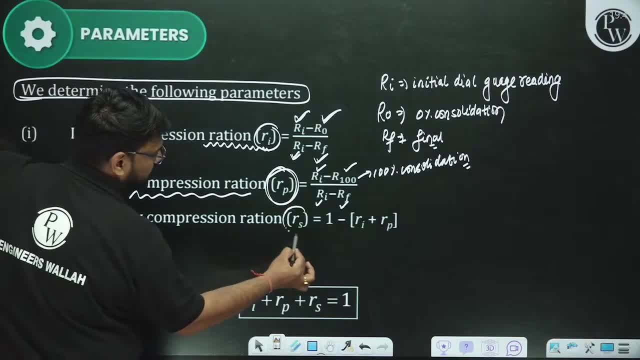 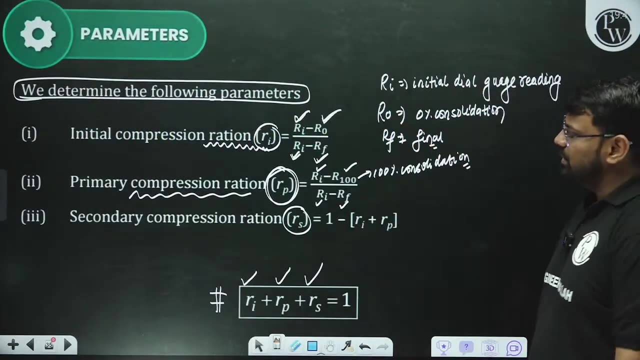 primary compression came and this is secondary compression, And the relation of secondary compression will be like this: that, sir, initial compression plus primary compression plus secondary compression, equal to 1.. So this can also be asked by you in the objective. So these are the different parameters that you can calculate from here. We generally 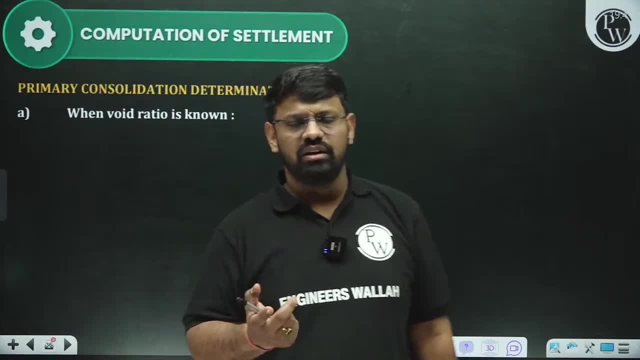 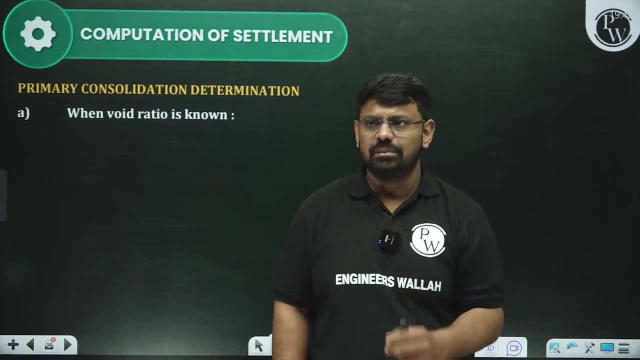 remove this from the curve fitting method. What kind of grande is this? It is a logarithmic tailor's curve fitting method. We have these two points. It is a very clear thing I understand. Now see what are the points ahead. We have the point of computation of settlement. 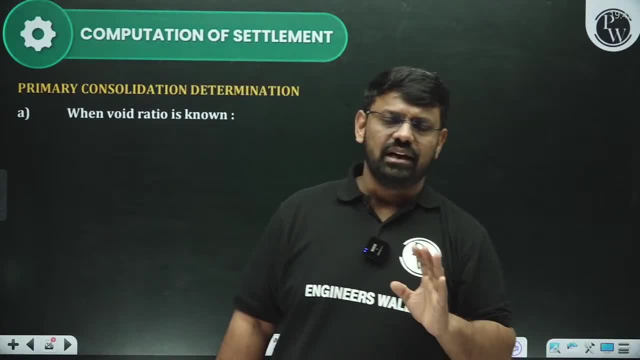 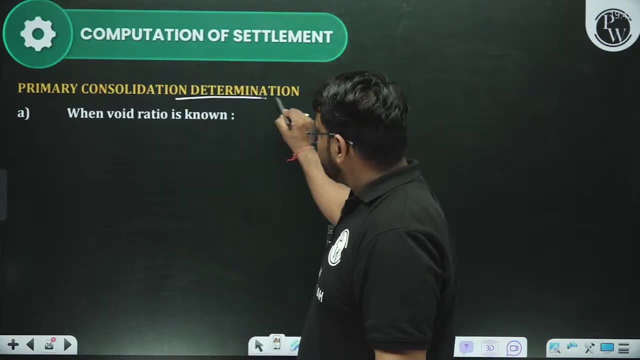 Many points ahead and doubtfulexisting. besides, what are these points? Can't listen to both. Now we hot to calculate settlement. then here you have to remember some formulas. What? what formulas do you need to remember? Okay, what formulas do you need to remember? 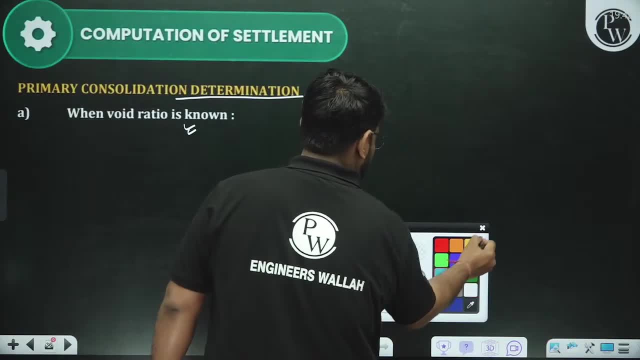 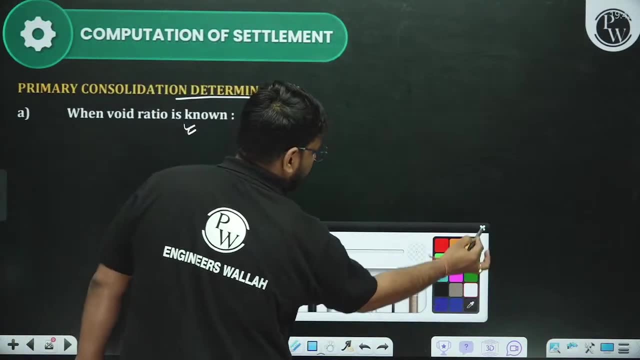 Sir, look here: primary consolidation determination when void ratio is known. When we get the void ratio, then we find out. do understand carefully, Sir. the very first point: when you know void ratio means You must have seen this formula. You must have seen this formula. 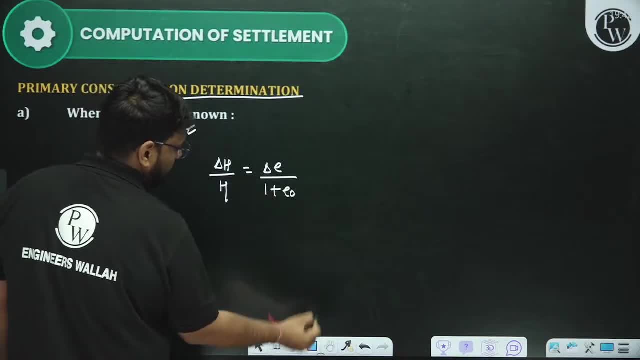 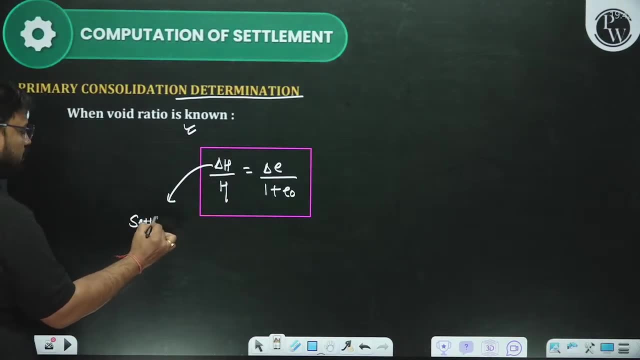 equal to delta E by 1 plus E. naught, This is the formula we have, sir. Now look inside this. This is delta H, which is the change in height. Basically, we are calling this settlement. So this is our. 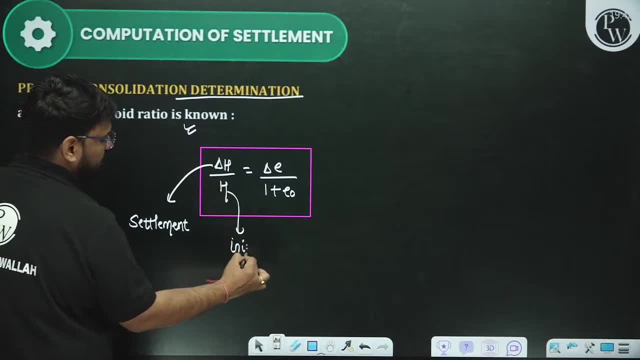 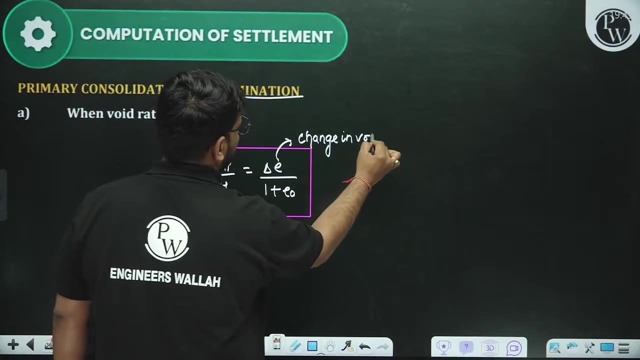 settlement. This is the initial thickness, sir. I mean say initial or total thickness. This is basically the thickness of the soil. See, this is the thickness of the soil. Delta E is the change in void ratio, Because we know, sir, there will be a change in the void ratio when you have 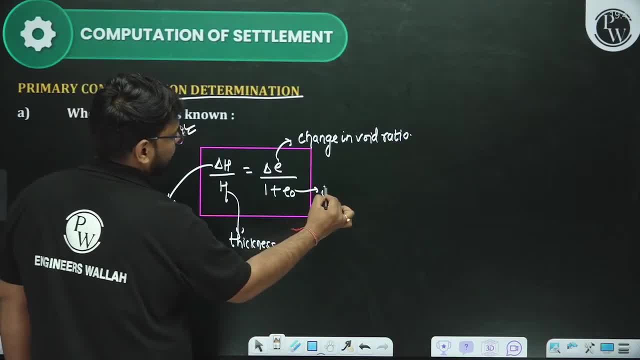 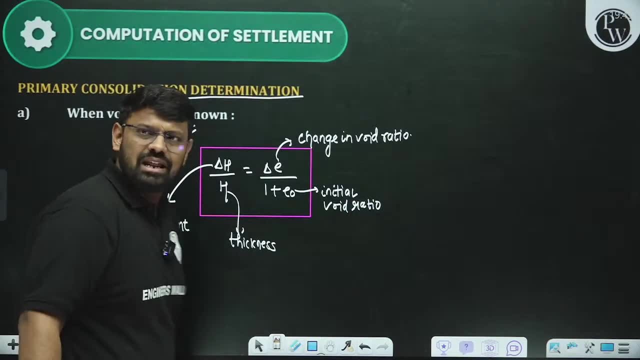 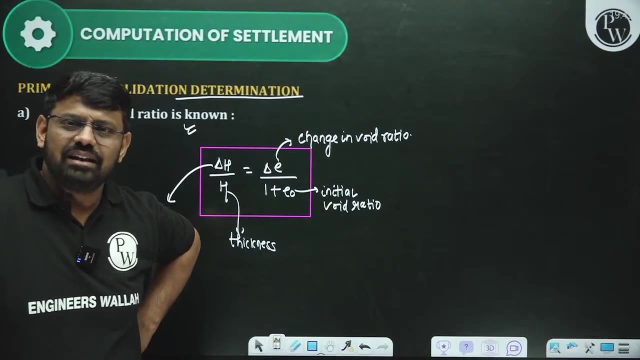 consolidation. And E naught, sir, we have. This is basically your initial void ratio. So, sir, this is our initial void ratio. So this is the first formula that we have to remember. Raju Yadav- Raju Yadav has come here with tea in a different way. Yes, Rupak, sir, you teach very. 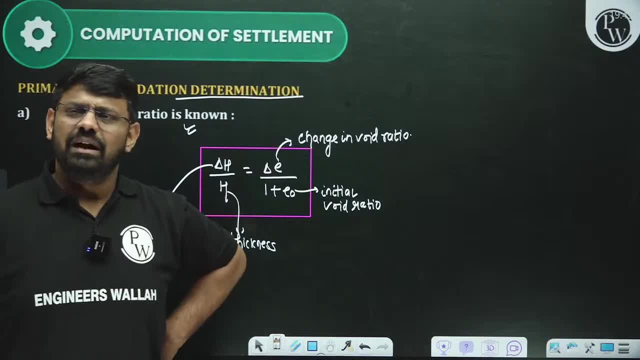 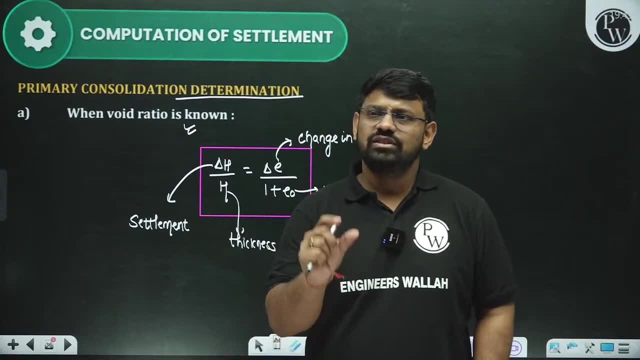 well, Raju Yadav says: sir, I am not able to understand anything. Something goes in my mind: Son don't say anything. You say, sir, I don't understand this topic, Tell me something like this: Yes, You know what happens in something I don't know. See, sometimes you go to order food, So 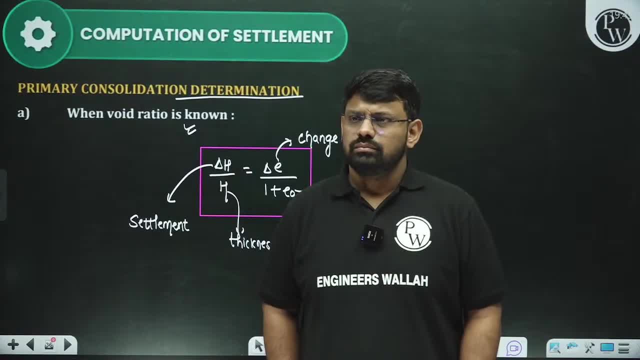 what will you eat? Bring anything, man. Now, what should I bring in? anything, Isn't it? I don't understand right, What should I bring in anything? Okay, if you say, sir, what should I write in this? I say: write anything, man. 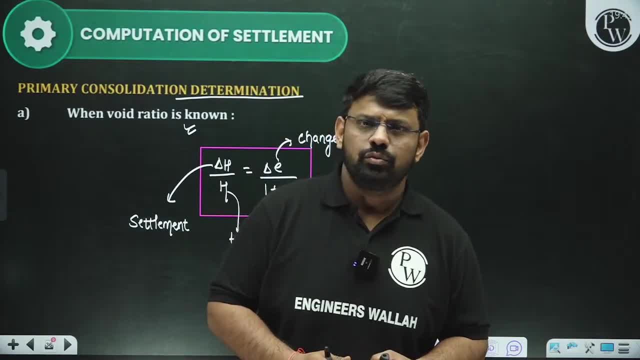 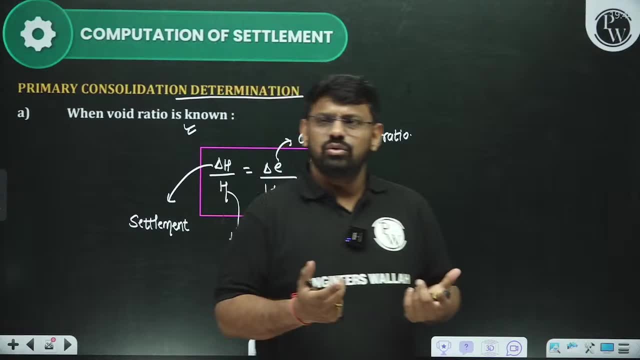 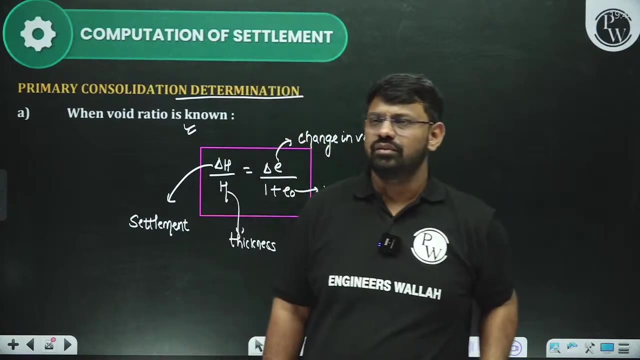 Write any answer So you will understand. Will you understand anything? Yes, No, it will come. What does something mean? What does something mean? And if something means everything, then you are in the wrong situation in life. You are at the wrong point, right? 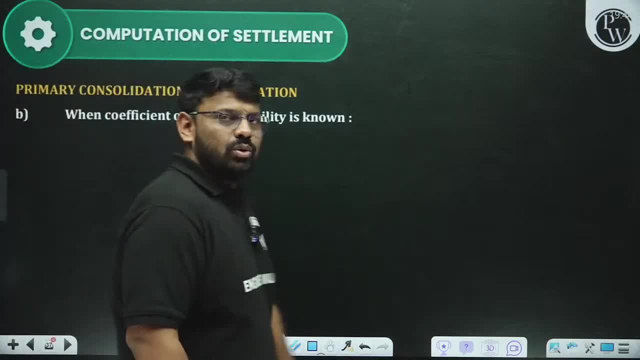 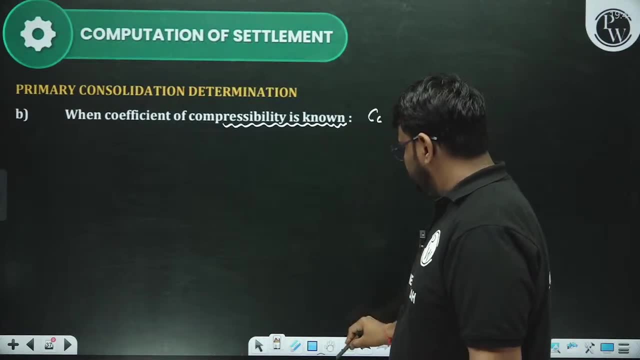 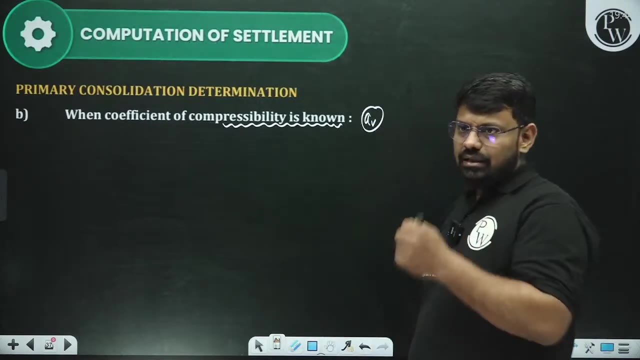 Okay, sir, The first point we understood here, this one. Look at the second. Look at the second, sir. Second, we have: when coefficient of compressibility is known, When we know coefficient of compressibility. Coefficient of compressibility means when we know AV, here Now, AV which we have, sir, this is coefficient of compressibility. 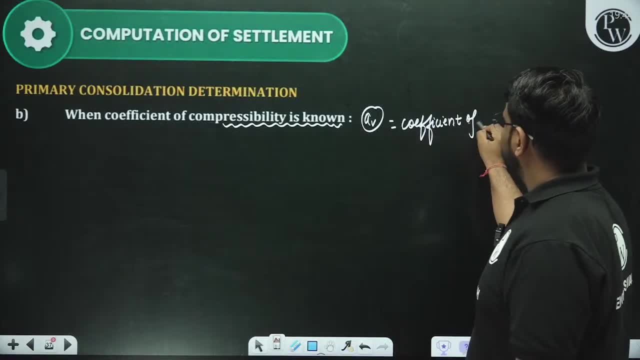 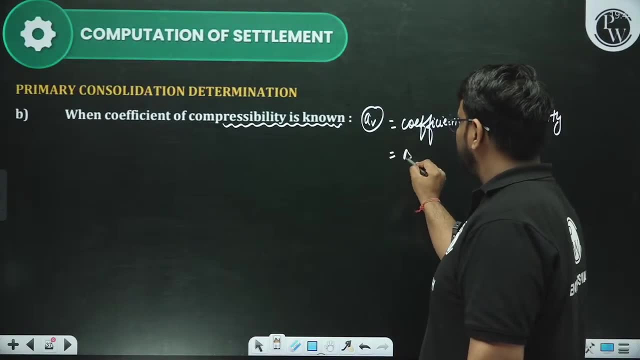 I told you just now, This is known as your coefficient of compressibility. So, sir, when we know coefficient of compressibility, which basically happens, you have delta E by delta sigma. So, sir, what can you do? You can write the change in void ratio, ie, delta E. sir. you can write AV into delta sigma. 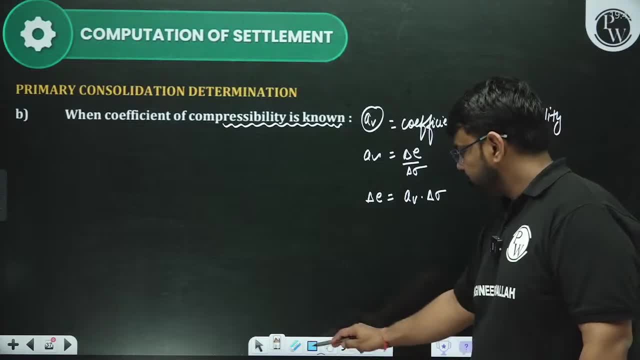 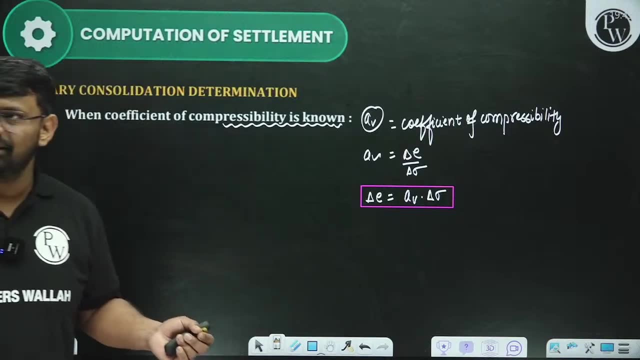 You can write this, sir AV, into delta sigma. Absolutely right, sir AV into delta sigma. You can write. So this AV into delta sigma. So this AV into delta sigma. So this AV into delta sigma. Yes, 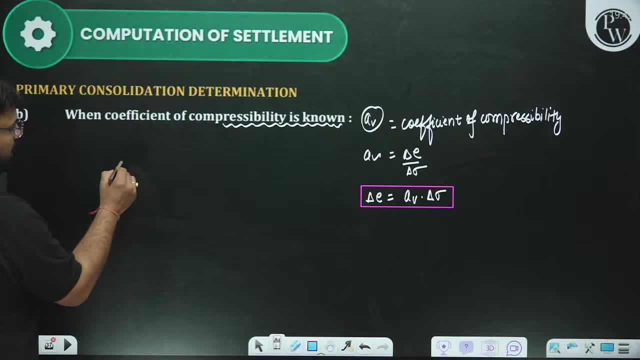 AV into delta sigma. AV into delta sigma. You will write here how, Sir, delta H divided by H is equal to delta E divided by 1 plus E. naught. So this delta H, sir. this is the settlement we have. 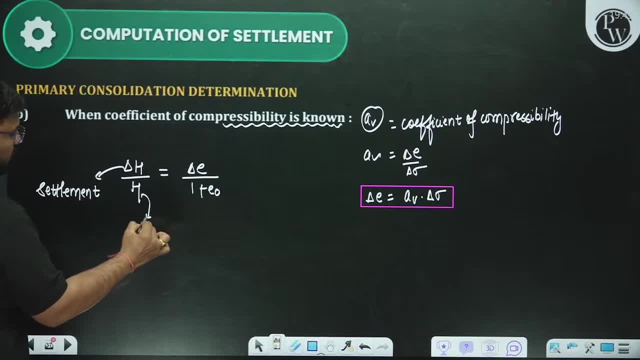 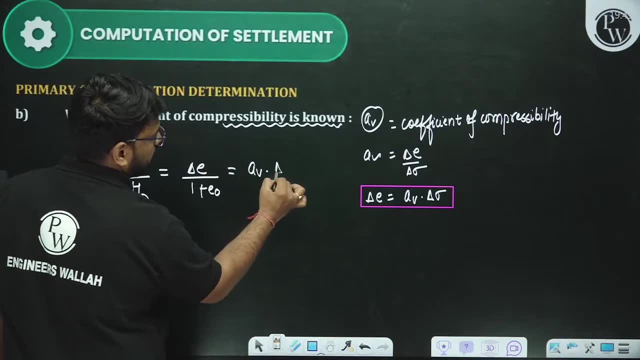 Right, We can call this the settlement. This is the same thickness which was the previous thickness. Now, what to do? Keep this in place of this. delta E Means AV into delta sigma divided by 1 plus E: naught, Yes. 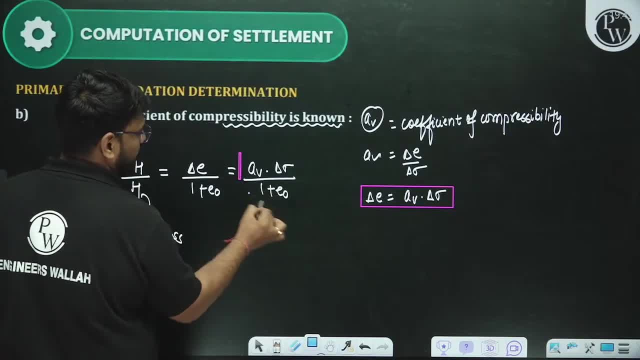 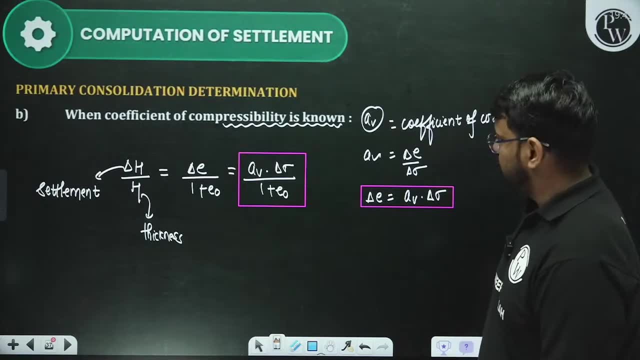 AV into delta sigma divided by 1 plus E. naught, Yes, Yes, Yes, Yes, Yes. So this is also our formula, from where you can calculate the settlement. Yes, Yes, Yes. Here also you can calculate the settlement. 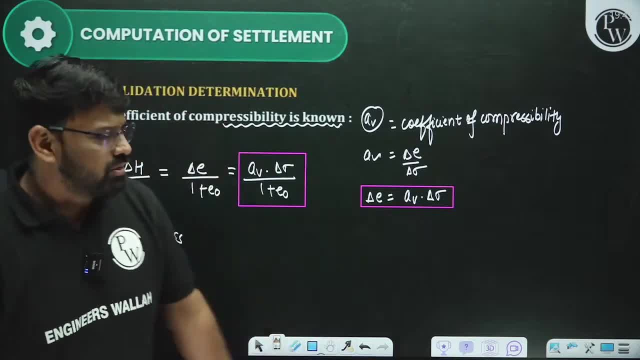 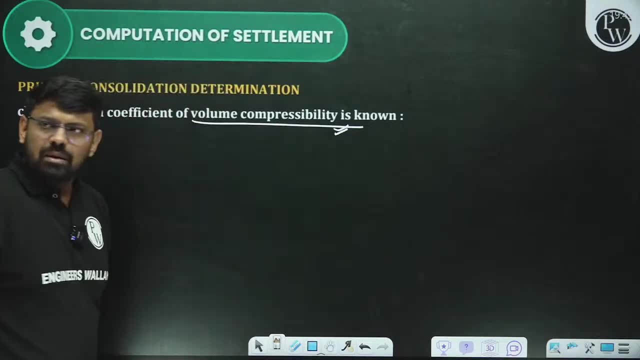 Right, Sir, one is telling the volume of coefficient of volume compressibility. Absolutely right, We will talk about it now. See when coefficient of volume compressibility is known. Means, Sir, coefficient of volume compressibility means that you have MV. 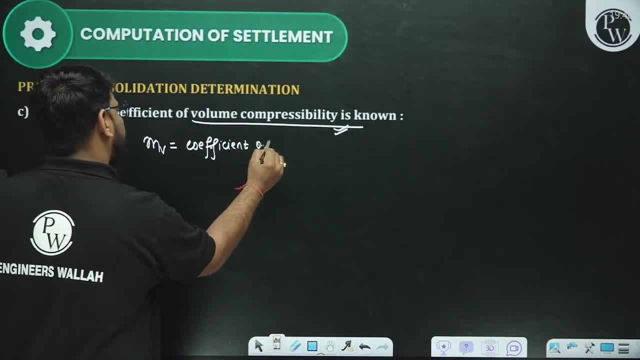 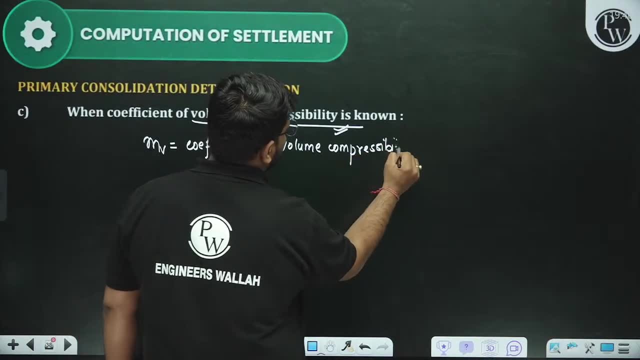 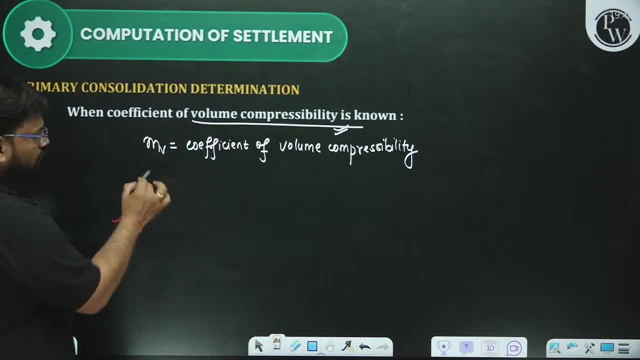 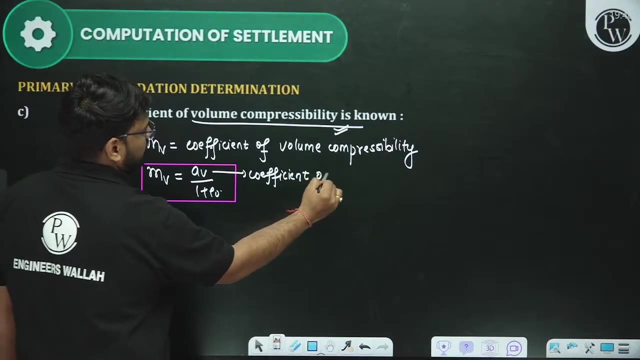 volume compressibility. Now the coefficient of volume compressibility is A? V divided by 1 plus E naught. This is your A V divided by 1 plus E naught, Where A V is coefficient of compressibility. Here A V is 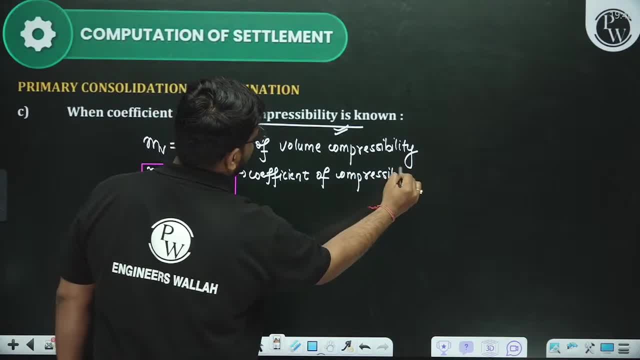 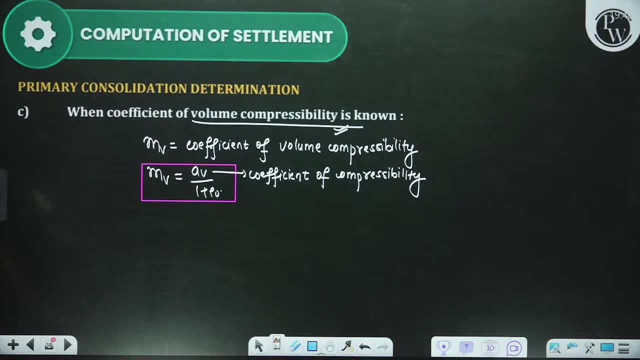 coefficient of compressibility. So we have to keep this thing in mind. And if we keep this thing in mind, A, V divided by 1 plus E, naught. So what do we do, sir? Now, you don't have to do anything. 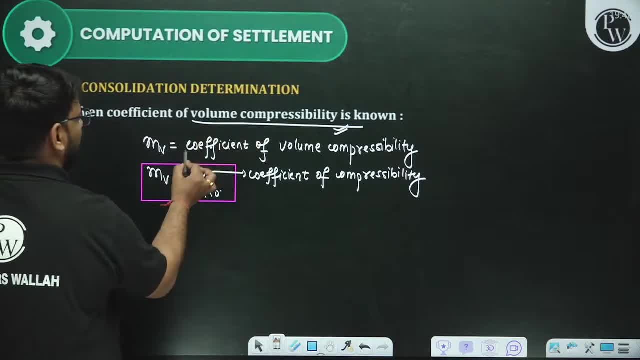 Now you don't have to do anything here, You just have to know volume compressibility. So look, Delta H by H is equal to delta E by 1 plus E. naught, This is our formula. The first thing is fine, sir. 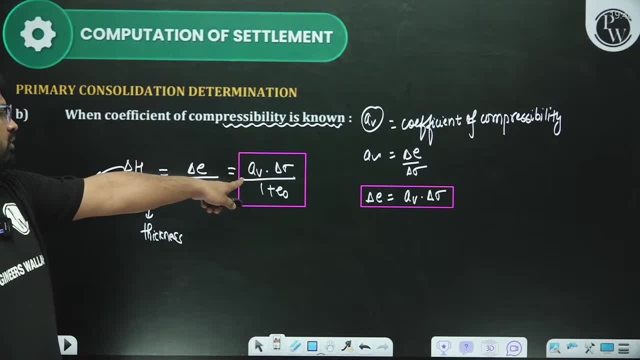 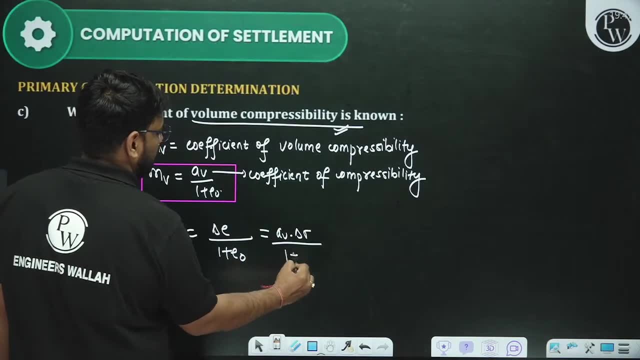 Now, when you know this formula and if you look here, then, sir, what we have? A V into delta sigma upon 1 plus sigma naught. That means you had written this only: A V into delta sigma Upon 1 plus E naught. 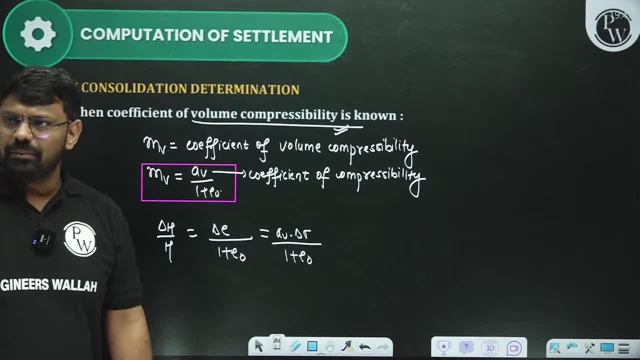 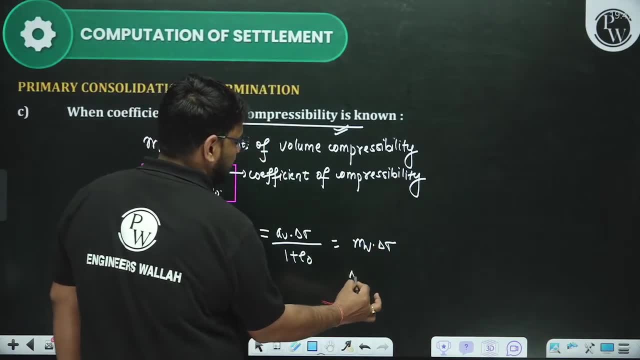 Now I am saying this, sir, A V upon 1 plus E naught which we have, this is M V. That means, sir, you can write this M V into delta sigma. So, sir, here the delta H which will come. 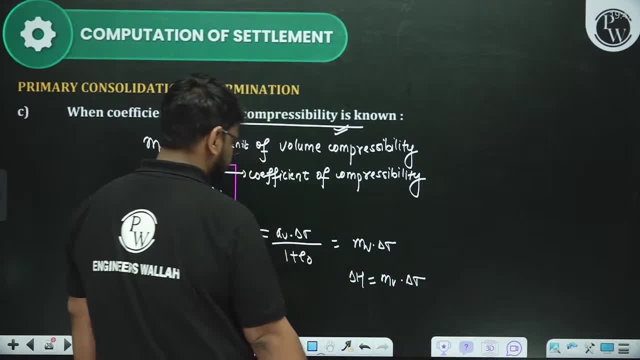 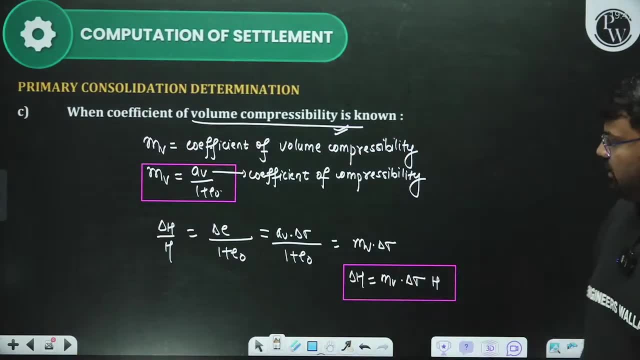 that will come, sir M V, into delta sigma. Okay, Multiply by H. What do we have so far, sir? This much we have. That is known as your settlement. So, even with coefficient of volume, compressibility, you calculate these things. 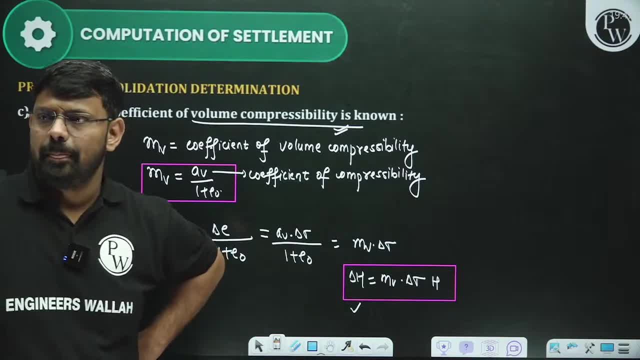 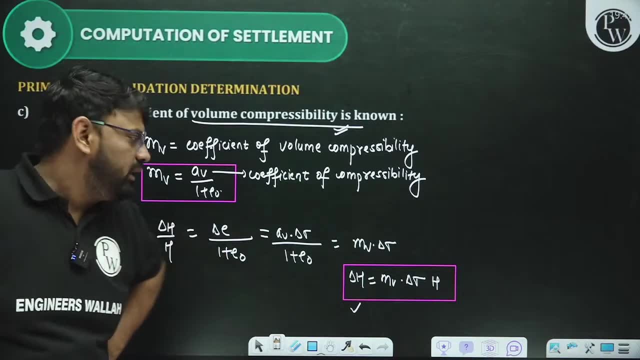 Change in volume upon effective stress change. Absolutely correct: M V upon delta sigma. Okay, It can come Okay. So this is what we have, sir. Coefficient of volume compressibility. Now, last thing, sir, we have 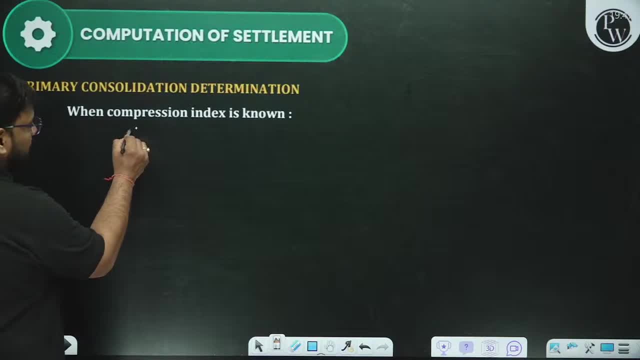 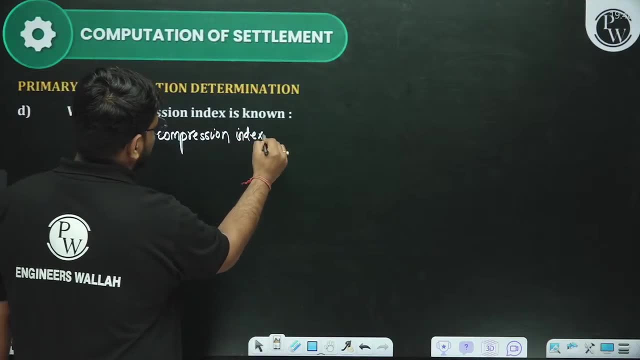 when compression index is known. When we know compression index, that means we know CC. Now, CC is what we have, sir, We have compression index, CC. sir, we have compression index And sir, what is compression index? 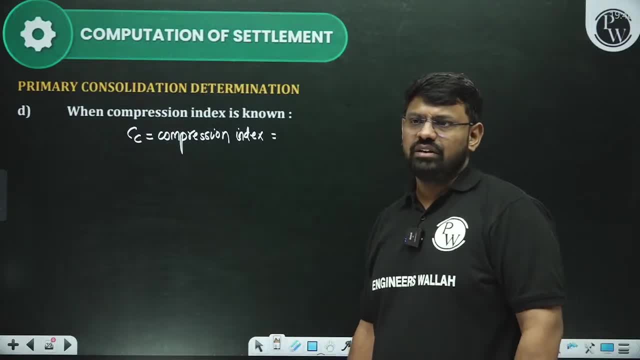 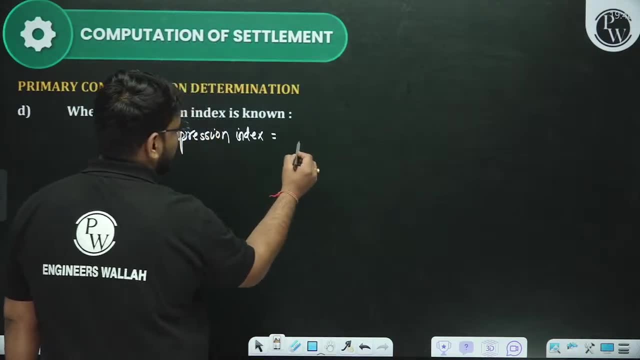 Sir, tell me quickly What is compression index? What is basically your compression index? Yes, we had studied K there also. You are absolutely correct. You are right, Sir, in compression index. I had told you that change in void ratio. 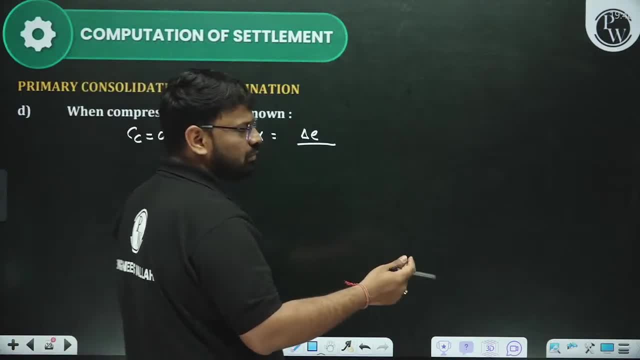 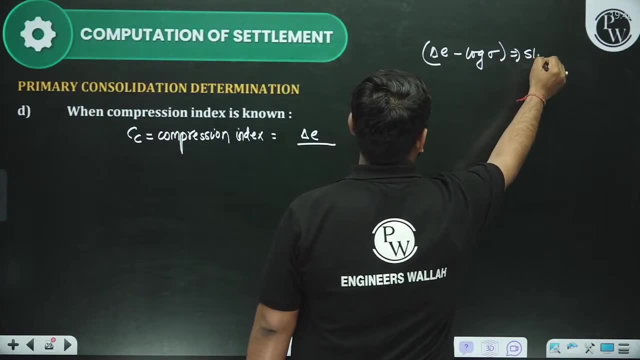 change in void ratio. the compression index you had, whose slope was that, Sir, delta E, and log sigma, the graph which was made the slope of this you had called compression index. So, sir, compression index, we had delta E by. 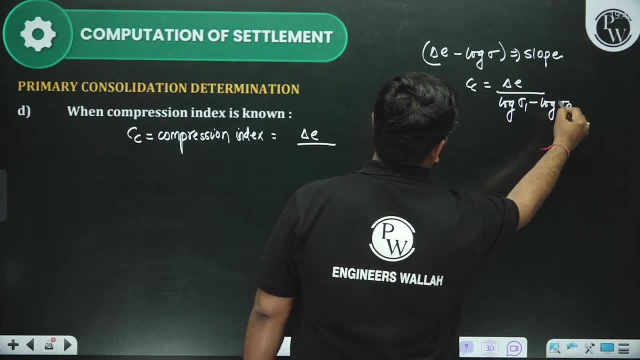 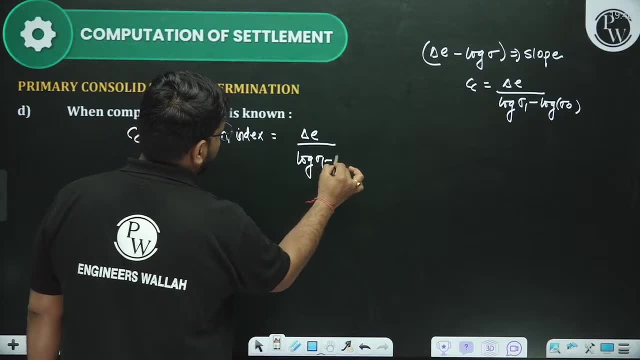 log sigma 1, minus log sigma 0.. We had compression index here. It is absolutely clear, sir. So delta E by sir. you can write here: log sigma 1, minus log sigma 0,. this is compression index. 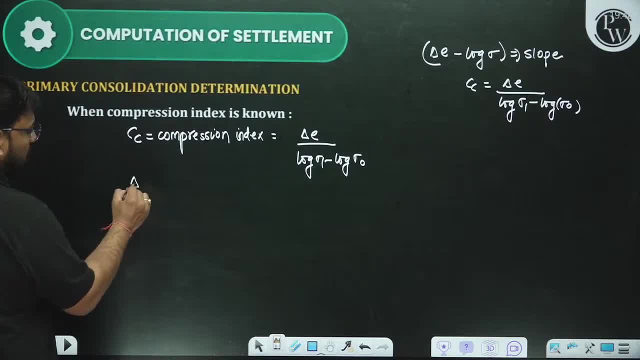 This is basically your compression index. So here, if I have to find delta H by H, how will I find it? sir, I will find it from delta E by 1 plus E naught. Now you can write delta E as CC into this. 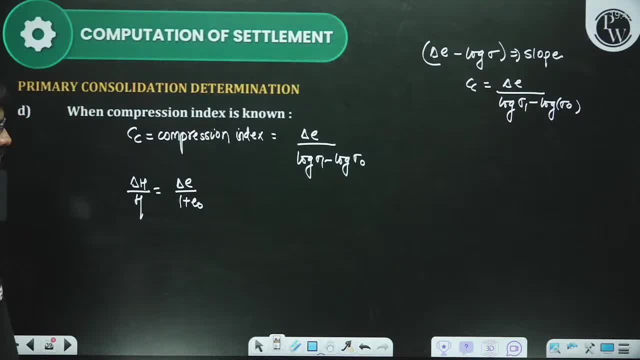 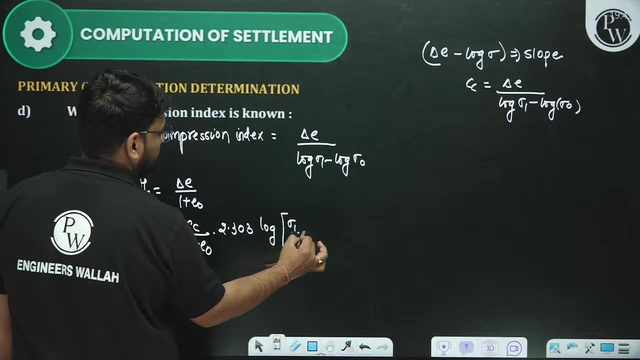 Okay, You can write CC multiplied by this. So, sir, write CC multiplied by this also. So I can write it instead of delta E. So I can write, sir, CC divided by 1 plus E naught: 2.303. log of sigma 1 by sigma naught. 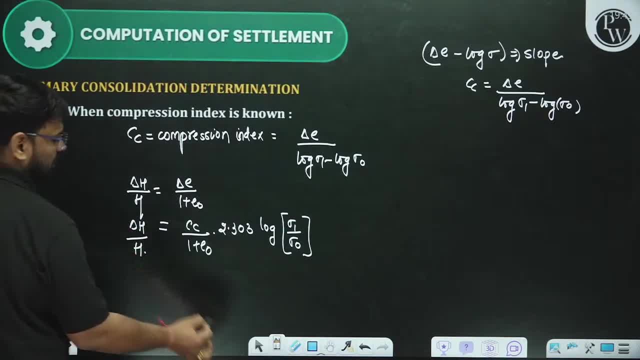 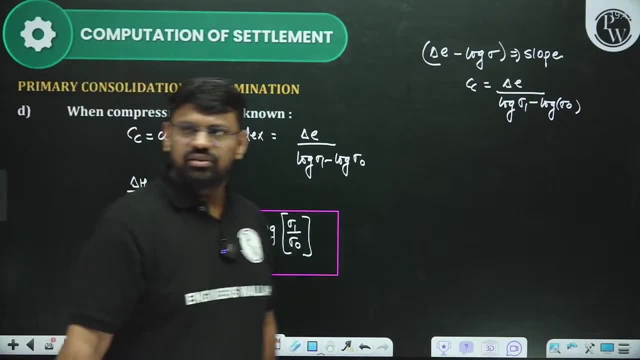 So from here, sir, what do we get From here? we get one more formula of settlement from where you can calculate settlement. What happened to CC here, sir? What happened to CC, sir? CC is basically your compression index. 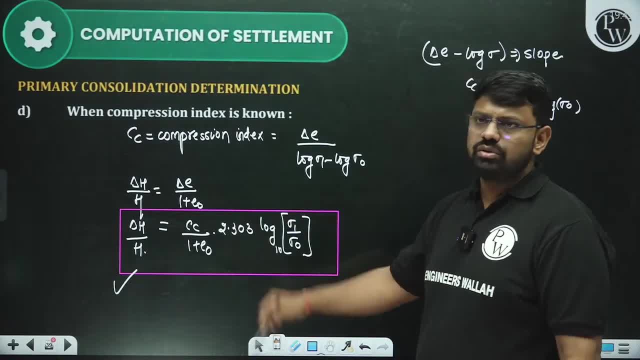 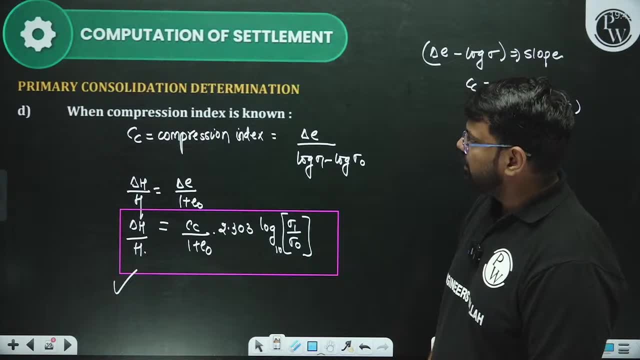 Okay To convert this into log base 10, we can log this 2.303 here. Okay, sir, Till here we got compression index 1 plus E. naught is done. When compression index is known, then it will be done. 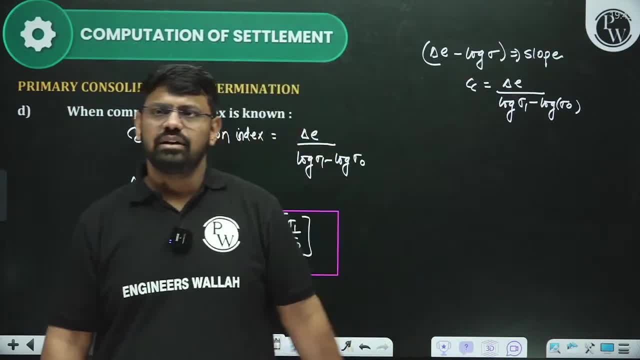 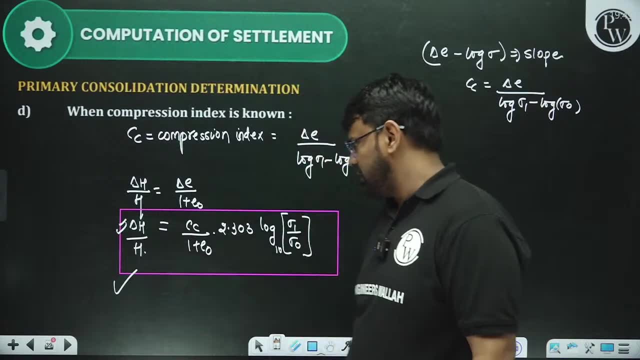 Okay, sir, Till here the things are absolutely clear. So what can you do in this way, sir? In this way you can calculate compression index or settlement criteria, That is, you can remove delta H settlement from here. One thing to keep in mind here is that 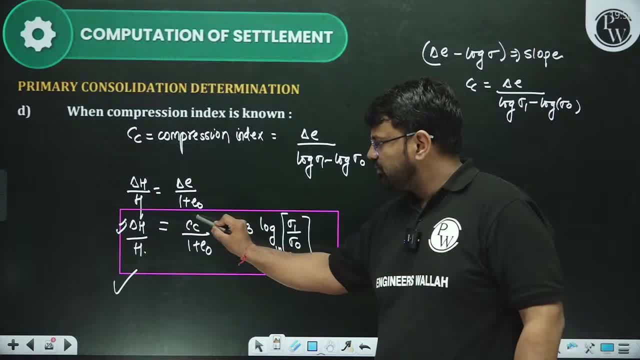 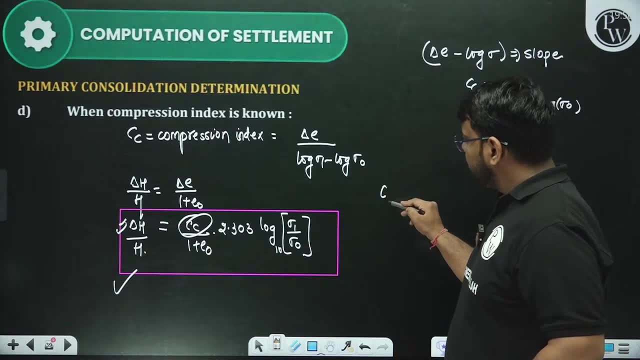 when you have soil that is normally consolidated, then only use this compression index. If you have soil that is over consolidated, then what do we have to use there? There, you have to use recompression index Means, you have to use CR. 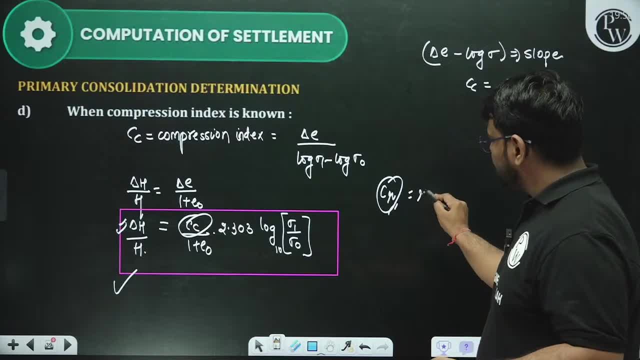 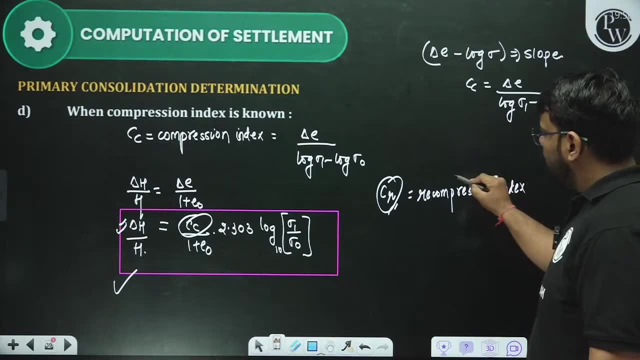 Okay, Because I had already told you the ratio. What is recompression index? Okay, When you have over consolidation, when your soil goes to over consolidation stage, you have to use CR. at that time You have to use recompression index. 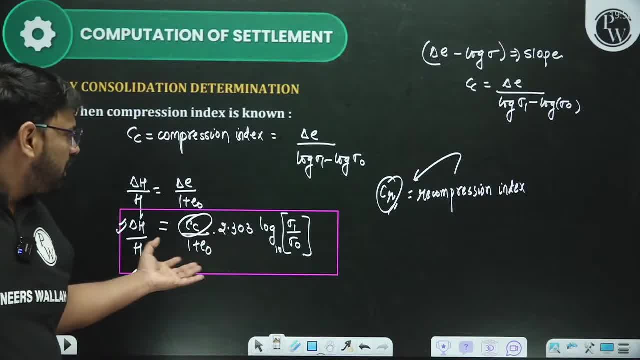 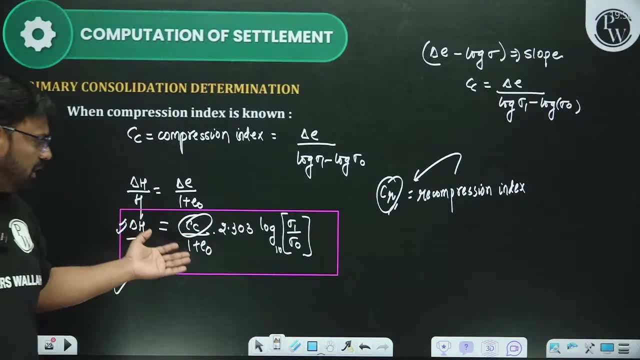 And when your soil is normally consolidated, then you have to use CC Means, you have to use compression index. This particular question comes absolutely numerically. Delta H by H is equal to delta C by means. CC by 1 plus C naught. 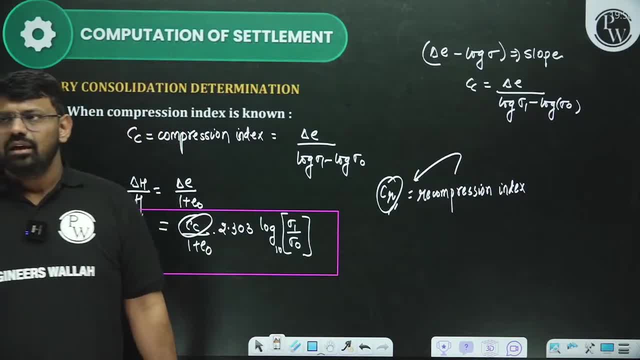 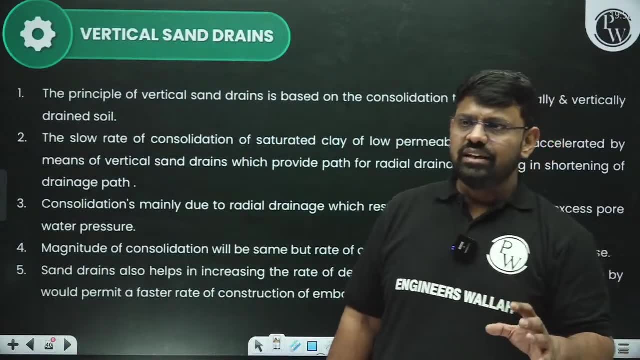 2.33 log, sigma 1 by sigma naught. Okay. So from here you have to remember all these formulas. From here you can remove the settlement. Okay, sir, Now in consolidation. sir, in consolidation, we have one more topic. 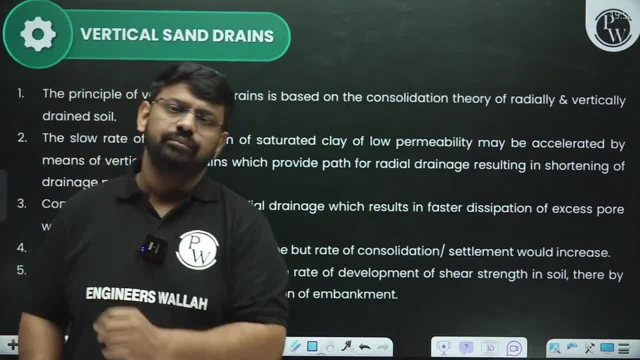 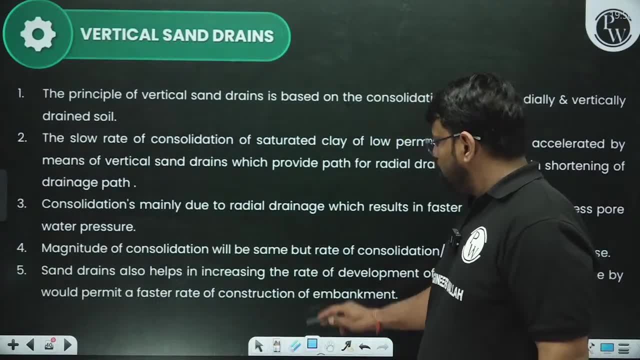 One more topic, sir. We call it vertical sand drain. Sir, what is the meaning of vertical sand drain? You will tell me quickly See what is the meaning of vertical sand drain. Assume that you have a clay deposit. Okay, 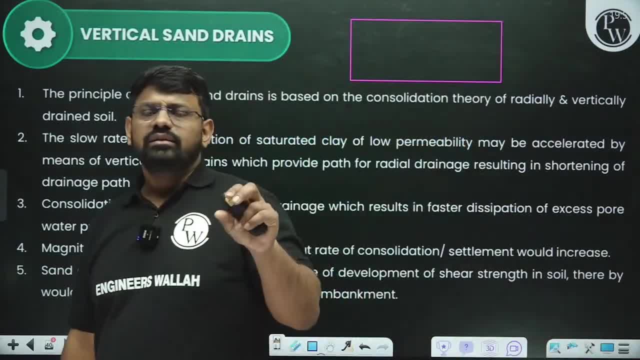 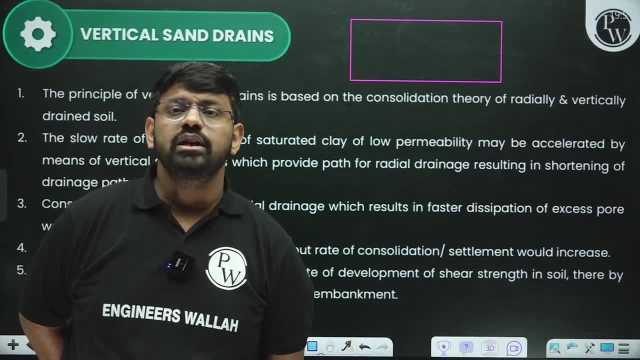 This is a very interesting concept, Sir. you have a clay deposit. Now, when you put a load in the clay deposit, then the consolidation that happens. that consolidation, sir, you get to see very slowly, slowly, slowly, Means you get to see consolidation at a very slow rate. 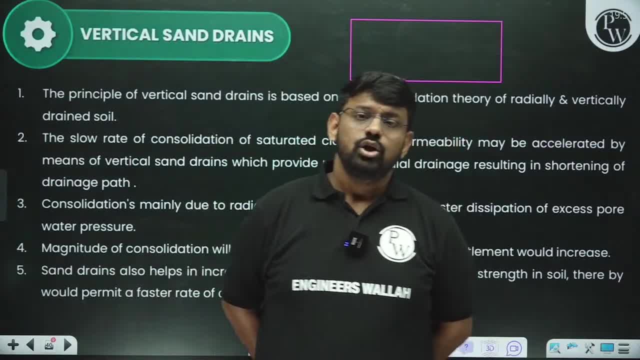 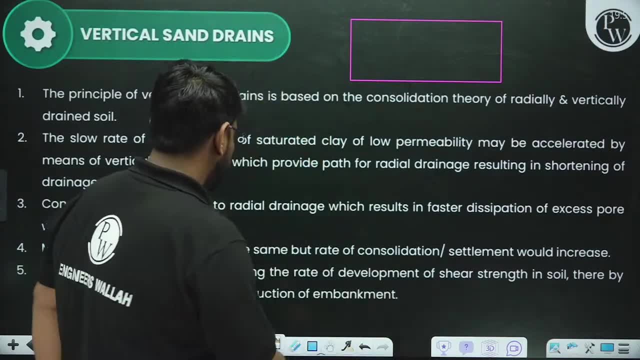 in the cohesive soil, in the clay. So if I put a sand drain in the clays, if I put a column of sand means, sir, what will you do? You will excavate here First. what will you do, sir? 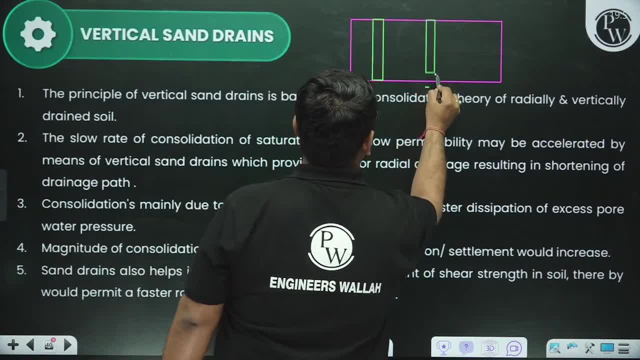 Will you excavate in the middle like this? By excavating, sir, you will fill the sand in it And in this. when we around here, sir, all the clay is there. What did you do in the middle, sir? 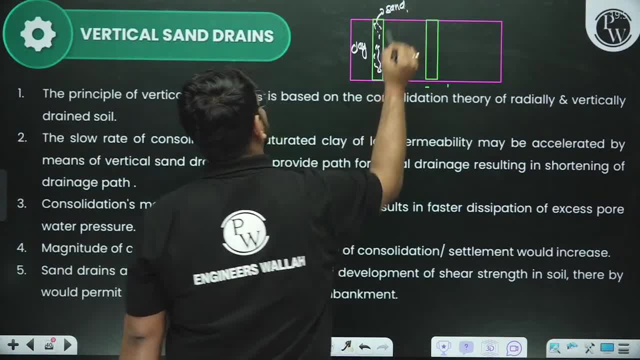 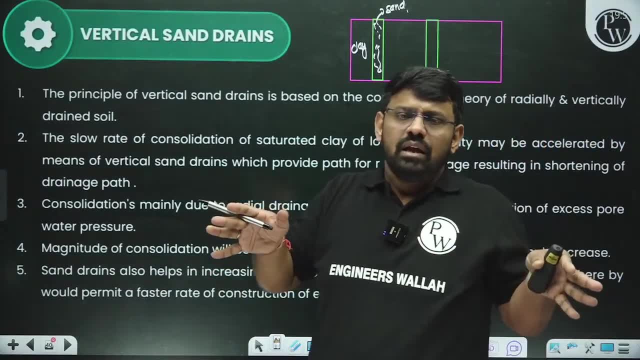 You filled the sand, So this is called sand drain. Now we know, sir, we know that in the sand it is very easy to get out of the water. sir, It is very easy to get out of the water in the sand drain. 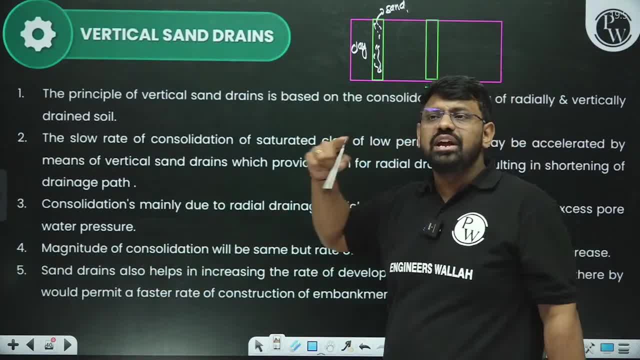 So the water will come out here. So what will happen here? The rate of consolidation will be fast. So, sir, this will increase the rate of consolidation. So, sir, this will increase the rate of consolidation. So, sir, the rate of consolidation will increase generally. 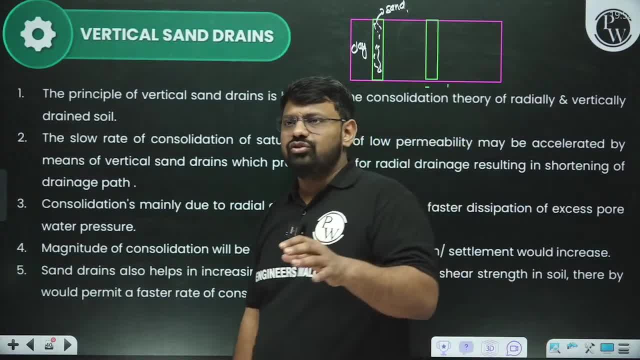 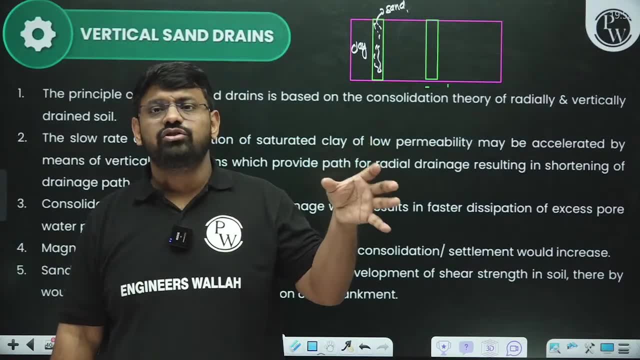 So, sir, why did this happen? Because sometimes we have to see in the structure that, sir, what will happen now? What load am I applying? I want to see how much our structure can settle maximum right. So if I get to know that quickly, 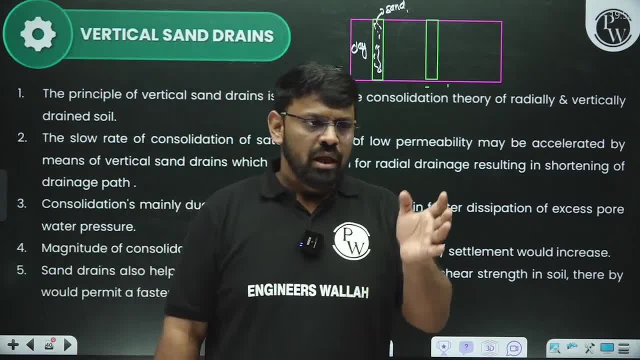 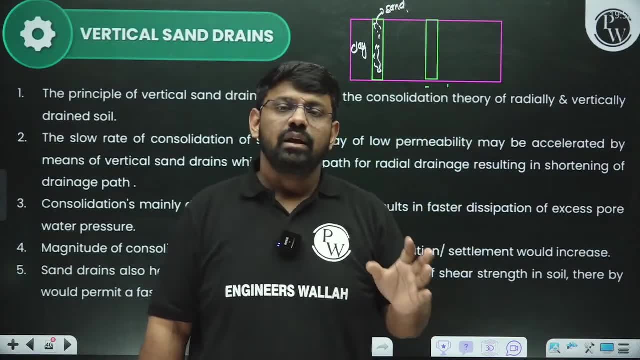 then I will understand things very easily there. So what will I do if I put it on cohesive soil or clay soil? So, sir, you will get to see that consolidation after a long time. That is why we put sand drain, So that we increase the rate of settlement. 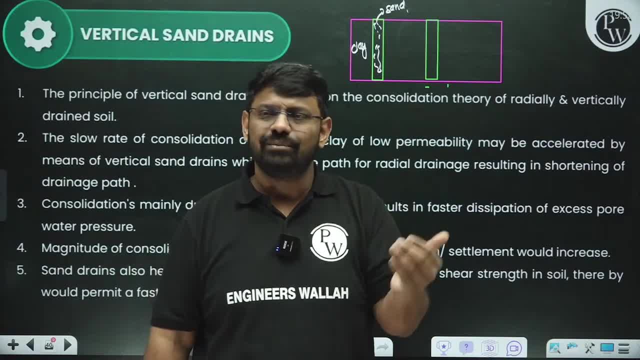 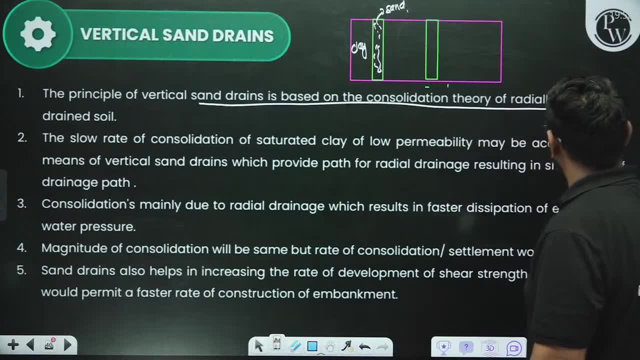 So that the settlement that had to be done in 10 years can be done in 2 years or 1 year, And we will know how much the final settlement has to be done. Okay, So look, the principle of vertical sand drain is based on the consolidation theory. 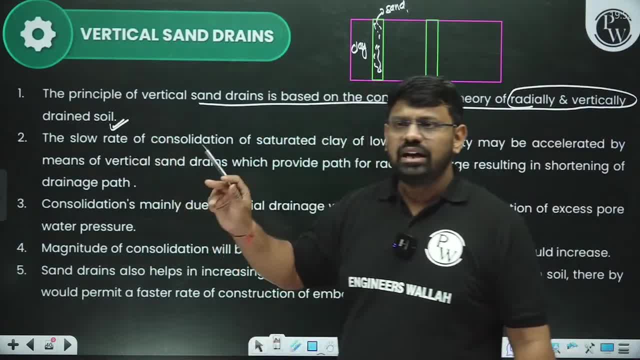 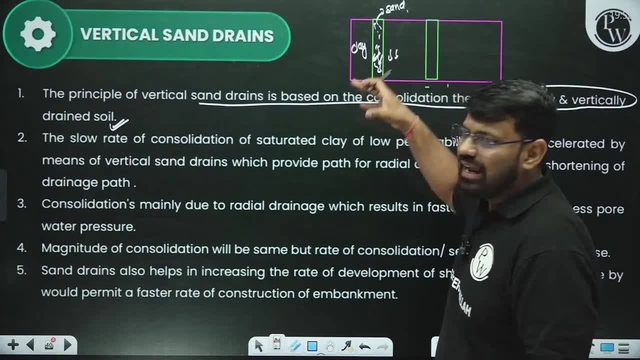 of radially and vertically drained soil. You get to see in radially and vertically drained soil. It means that now you are not only having vertical drainage, sir, now the drainage is also being done in radial, Because in sand it is possible in every direction. 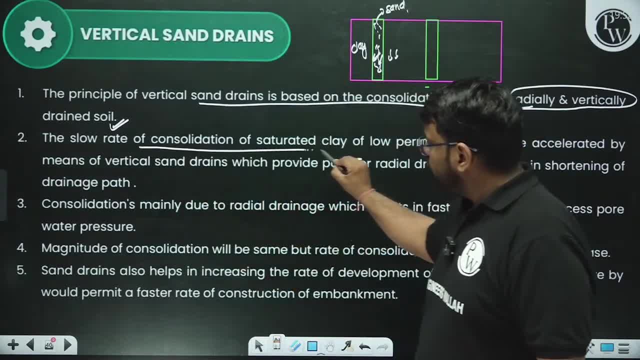 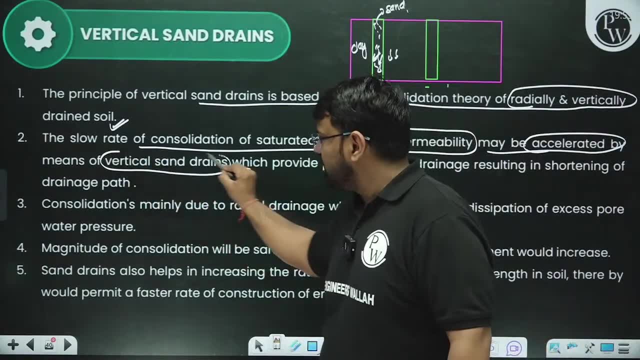 Absolutely right Now. look, the slow rate of consolidation of saturated clay of low permeability may be accelerated. We accelerate this by vertical sand drain. So, sir, with vertical sand drain, what can we do? We can accelerate it. 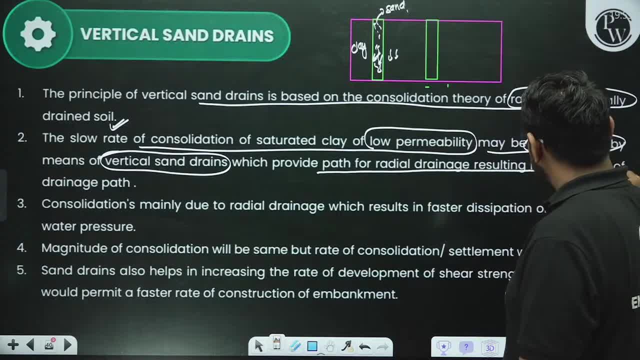 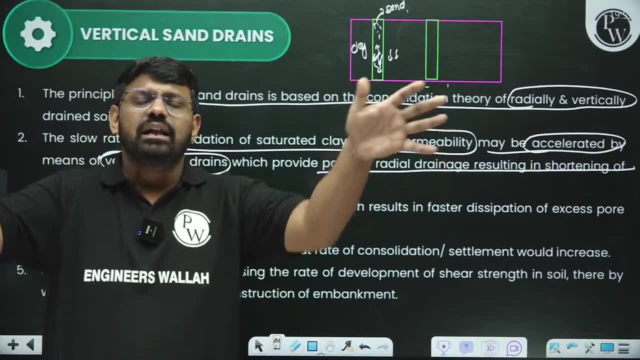 Okay, Provide path for radial drainage, resulting in shortening of drainage path. It means, sir, our drainage path will become smaller And we are allowing water in every direction, So that water can flow out from there in every direction. This is vertical sand drain. 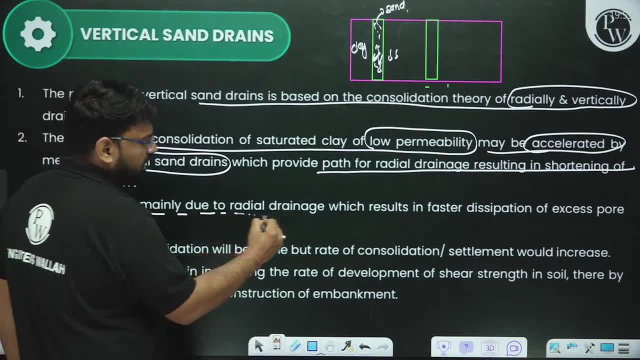 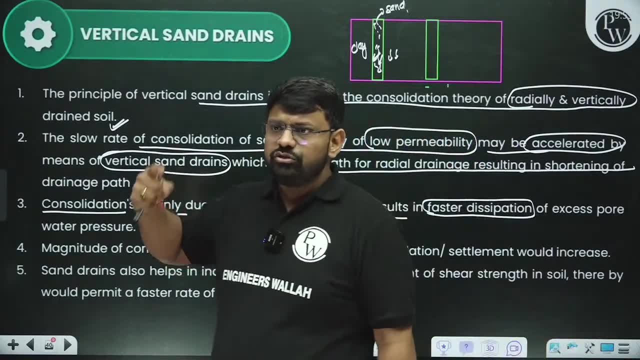 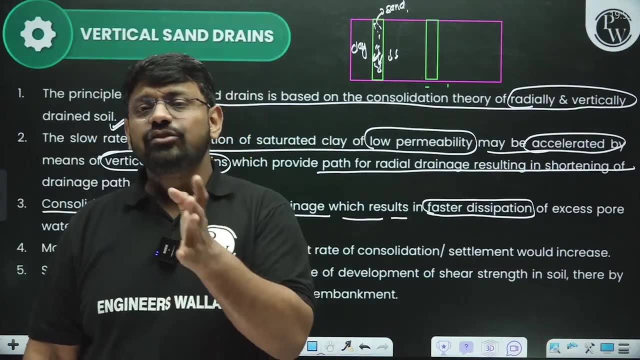 Now look. consolidation is mainly due to radial drainage, which results in faster drainage. I had told you in a statement that the rate of dissipation we have depends on how much or how fast the excess pore water pressure dissipates. I had told you earlier. 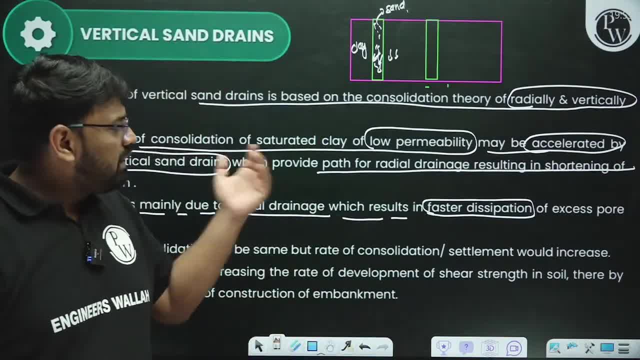 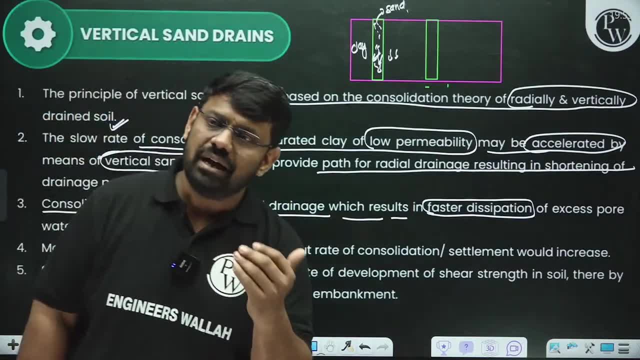 It is the same. So what are we doing here? We are fastening the dissipation here. So when the excess pore water pressure dissipation will be fast, then the rate of consolidation will also increase. Okay, Look ahead, Sir, the magnitude of consolidation we have. 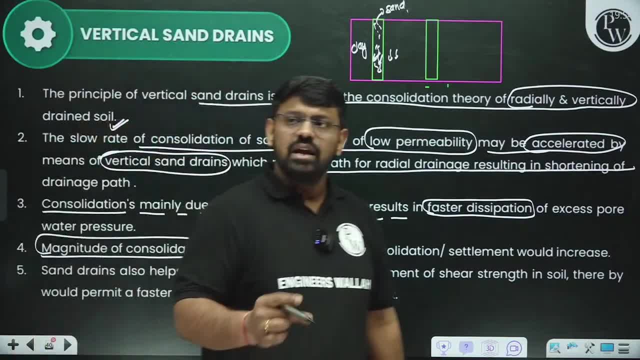 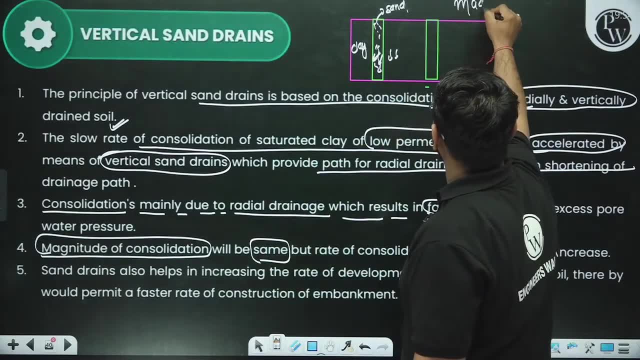 will be same. We just have to keep in mind that, Sir, the magnitude will not change here, Only the rate will increase. Sir Right, Not the magnitude. Sir, in any particular soil, if we have total settlement, suppose it has to be of 15 mm. 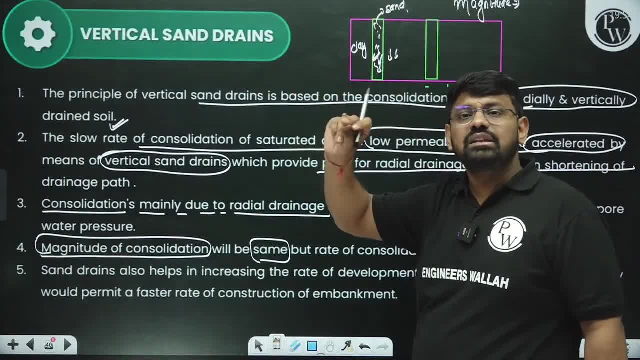 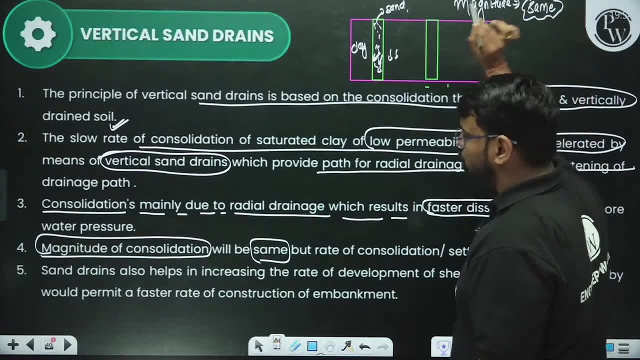 then 15 mm will remain. It will not be more than that, But that 15 mm will be achieved in less time. This is vertical sand drain, Sir. So, Sir, the magnitude of consolidation will remain the same, as it has to be. 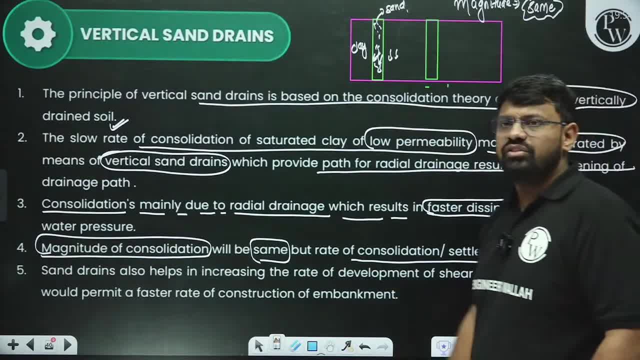 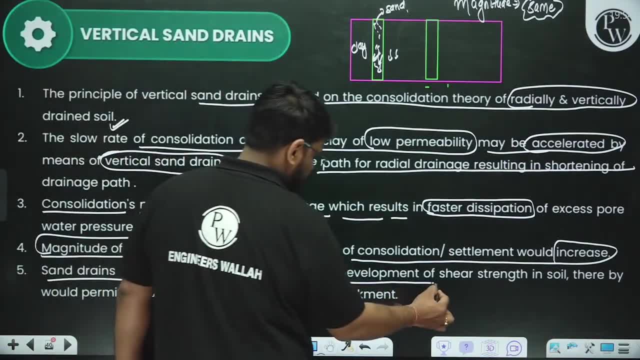 But rate of consolidation will increase. So the rate of consolidation will increase. We have to keep in mind this. Now look ahead, Sir Sand drain also helps in increasing the rate of development of shear strength of the soil And thereby would permit the faster rate of consolidation and embankment. 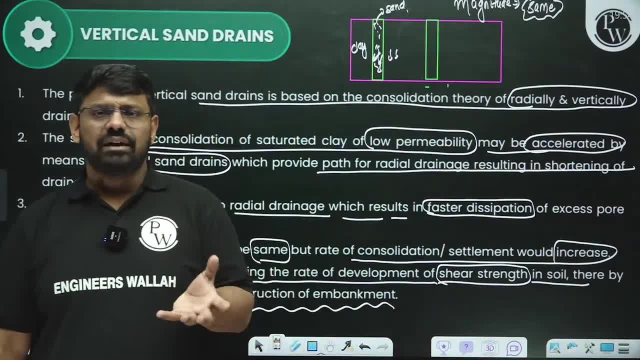 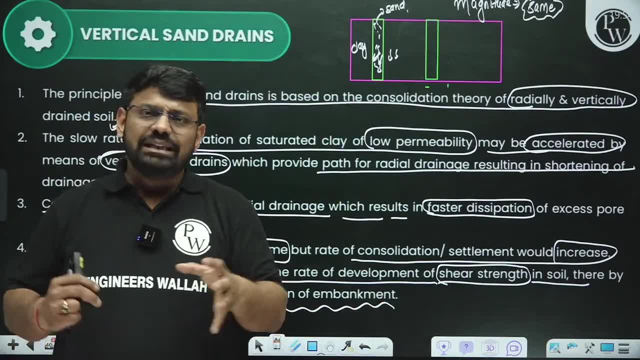 It means, Sir, from here your total capacity also increases. It means shear strength will also increase here, Because as the faster water is coming out from there, then the particles will come in closer contact with each other. When they come in closer contact, 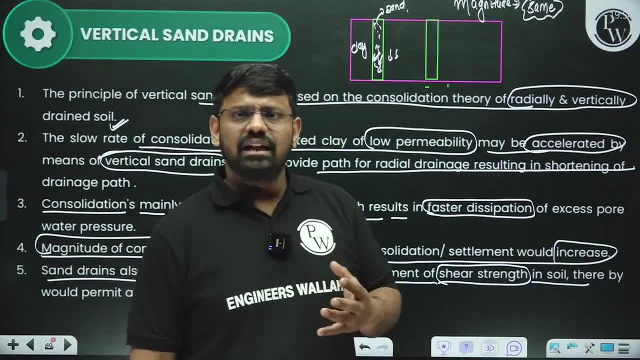 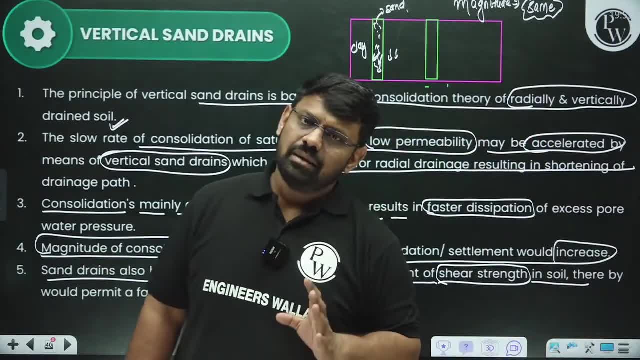 then the effect of stresses will increase And at the same time the value of shear strength will also increase. It means you will also get to see the improvement and capacity of the mixture increasing. The matter is absolutely clear. So, Sir, we apply this vertical sand drain in this way. 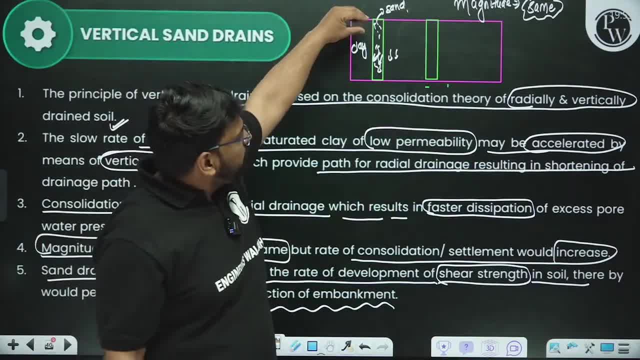 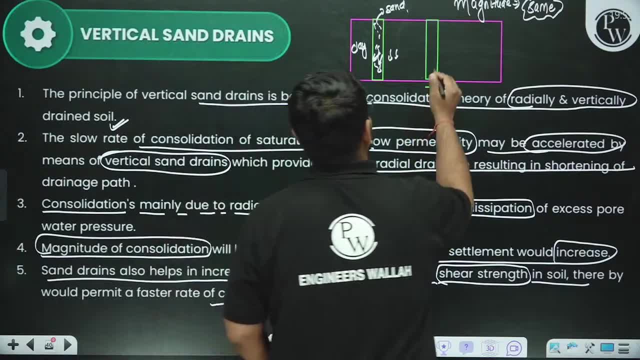 Now one more thing to understand here. What do you understand, Sir, When you install the vertical sand drain, when you install the vertical sand drain while installing, Sir, the soil around it? what do you do in this soil around it? 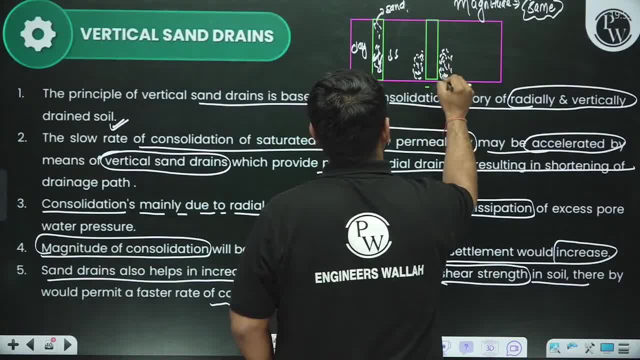 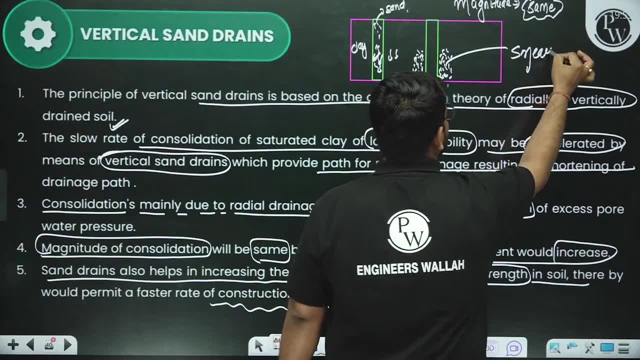 Sir, you do densification. What do you do, Sir? You do densification in the soil around it, And this is known as your smear effect. What do we call this, Sir? This is known as your smear effect. This is what we call as smear effect, Sir. 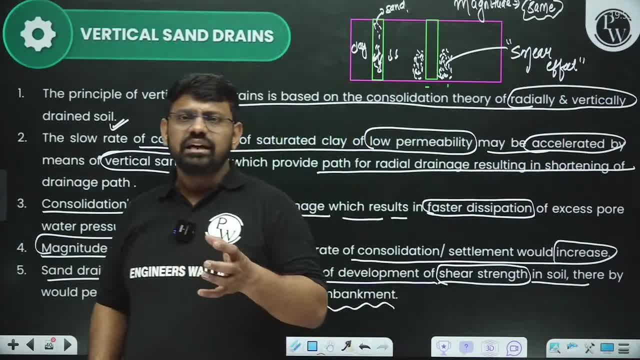 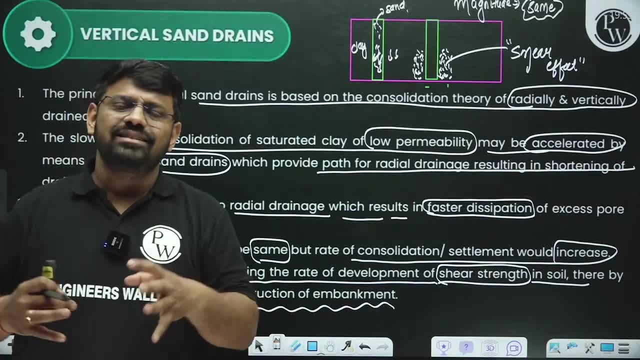 Densification of the soil that is created by placing the sand drain. When we are placing the sand drain, then we will do excavation. The soil around us goes into a dense state. It becomes compact, So the soil's denseness improves there. 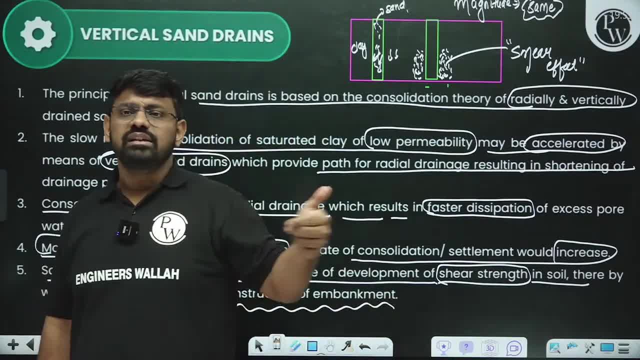 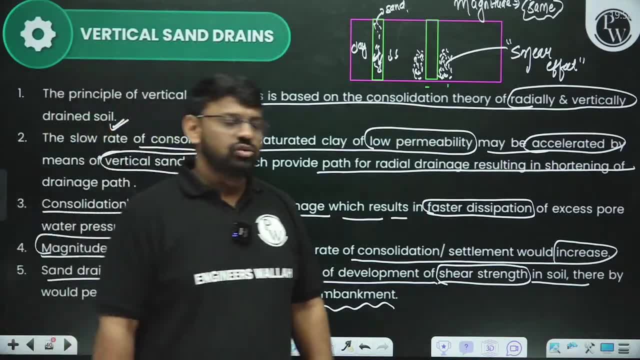 The strength of the soil improves, And that improves, Sir, because of your smear effect, So that is known as your smear effect. in the vertical sand drain Is everything clear. So, Sir, this is what we call as complete consolidation. 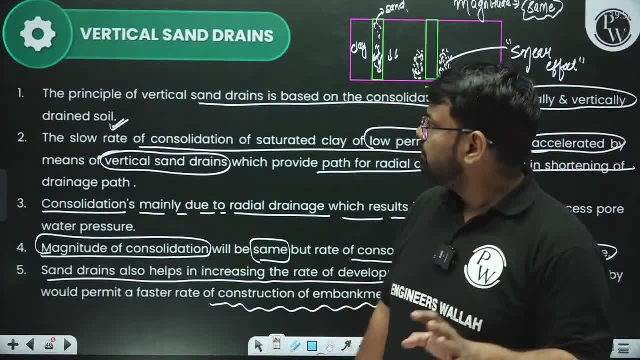 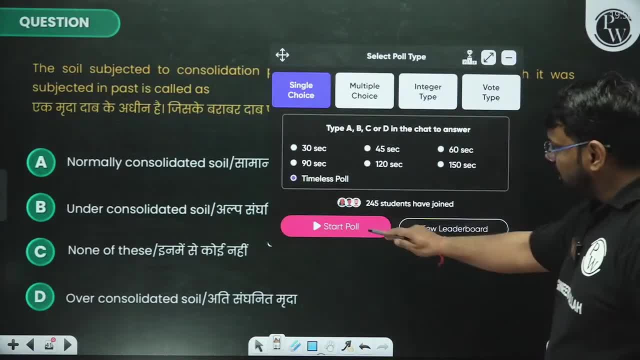 In which we have covered a lot of important things. We will do three questions. Fill the comment box with the questions. First of all, we have the answer. First of all, we have this: The soil subjected to consolidation pressure equal to. 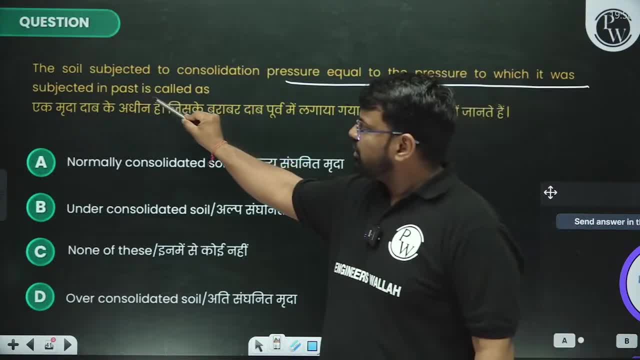 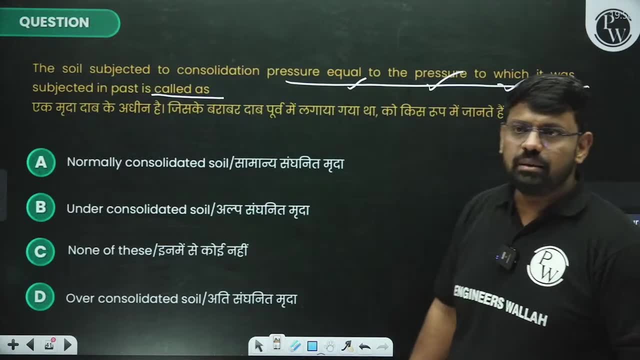 pressure to which it was subjected in the past is known as The soil subjected to consolidation pressure equal to the pressure subjected to which the soil in the past is known as What is said. I had told you Now normally consolidated soil in over consolidated soil. 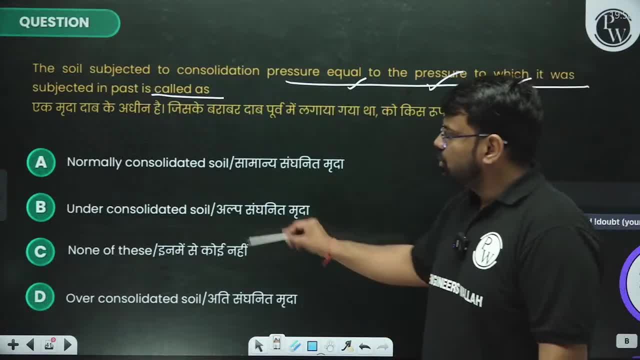 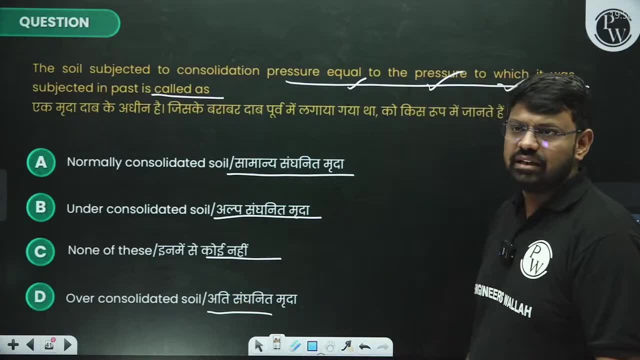 Okay, Tell me in both. So normally consolidated soil is done, Under consolidated soil is done. None of these, or over consolidated soil. What is the correct answer? Normally consolidated soil. When Sir sigma is applied to us, Sigma is equal to sigma C. 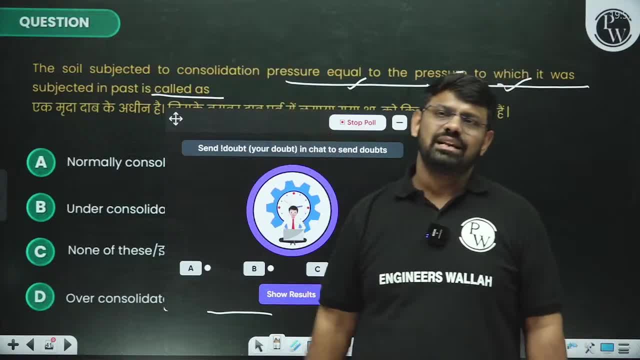 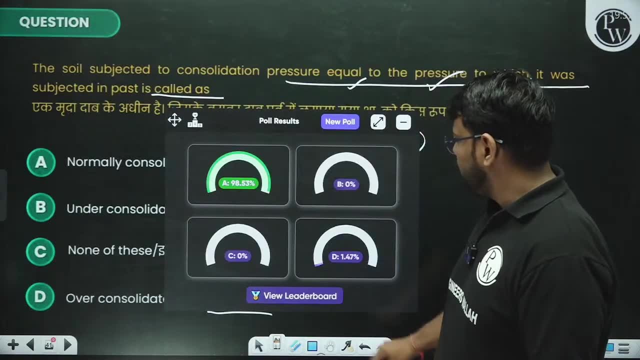 So A is the right answer. Fill all the children quickly. Okay, Tell me the answer quickly. A should be the right answer for this particular question. Let's see, Sir, how many children did it. Ninety-eight percent of the children did it, right. 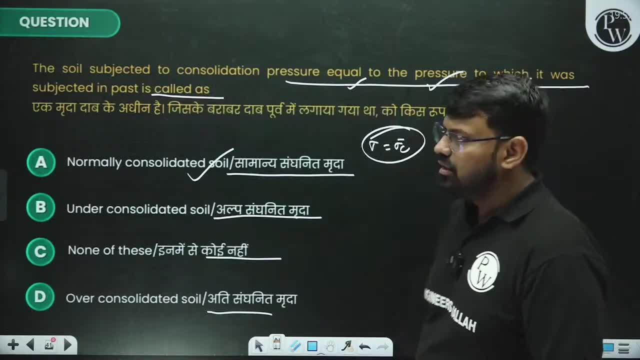 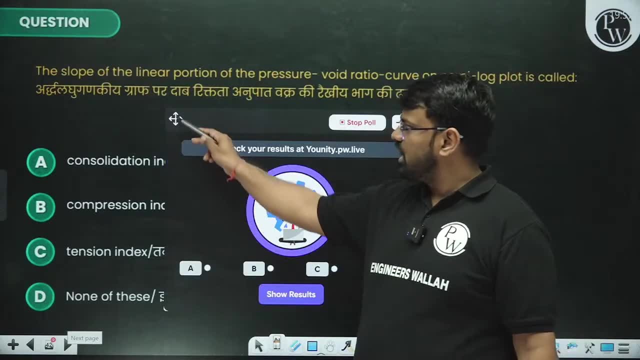 Aakash Harshit, Vivek, Prince Ankit. It's me All the children are telling Sir, it is absolutely correct. Come on to the next point. Second Second option, Second question, in front of you On your computer screen. 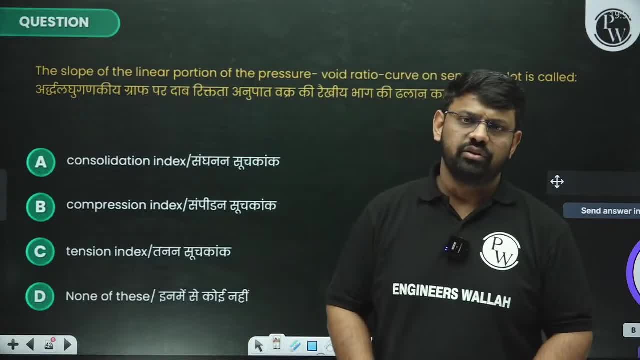 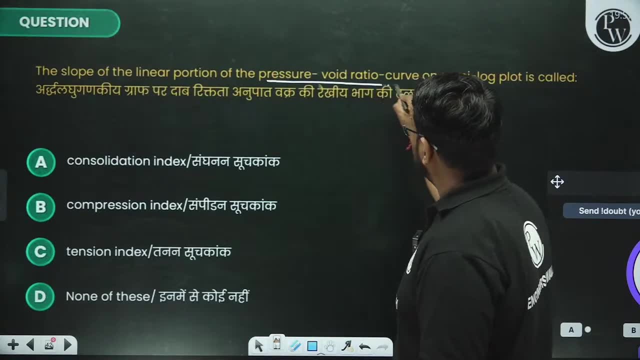 Here it is. Second question. Second question, Second question: Who plays crore-patim In the voice of Amitabh Bachchanji? What do you say, Sir? The slope of the linear portion of the pressure-void curve on semi-logarithmic plot is known as: 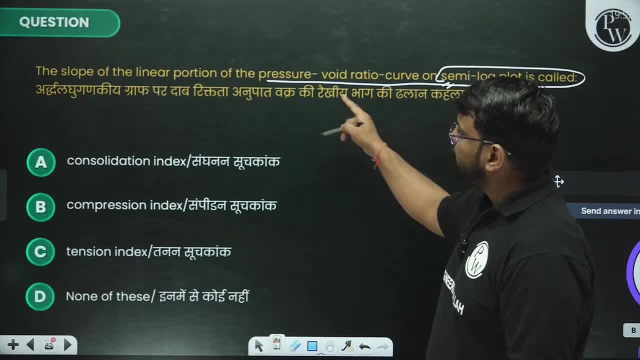 I have just told you. What is it called, Sir, What it is known as, What is it? Slope of the linear portion In which Pressure and void ratio on a semi-log graph Means delta, E and log sigma. 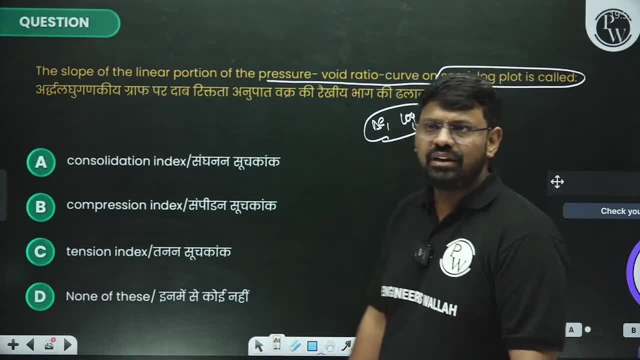 The graph of this is called slope compression index. What is it called, Sir, Sir? compression index? It has been filled in a great way. Let us see who wins 7 crore. Tell me quickly, Sir. consolidation, Not consolidation index. 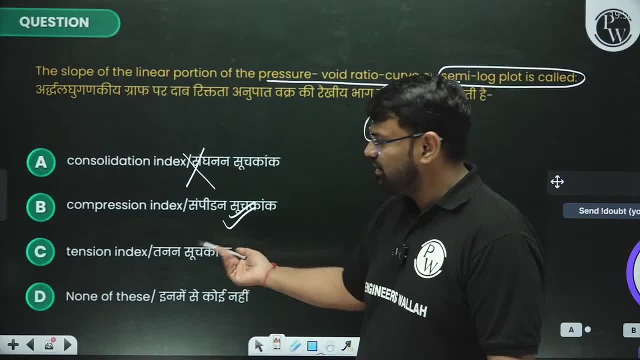 Compression index is absolutely correct. Tension index: Nothing happens, We do not take tension. So, Sir, B is the right answer. B is the right answer for this particular question. It is absolutely correct. B is the correct answer. 91% of the children have told. 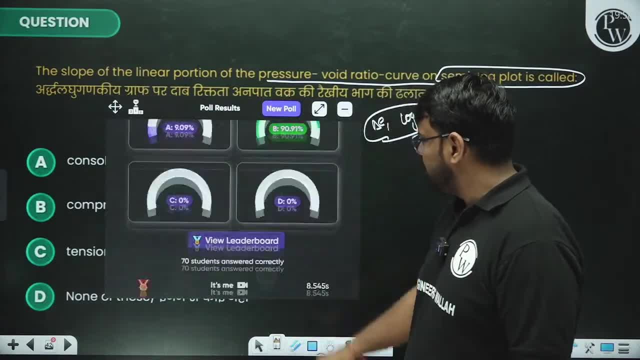 It is me, is the fastest? Harshit Bhaskar, Vivek, Prince, Ankit. Very good, And now the last question of today's class. Here is your last question, Sir. what is it called, Sir? 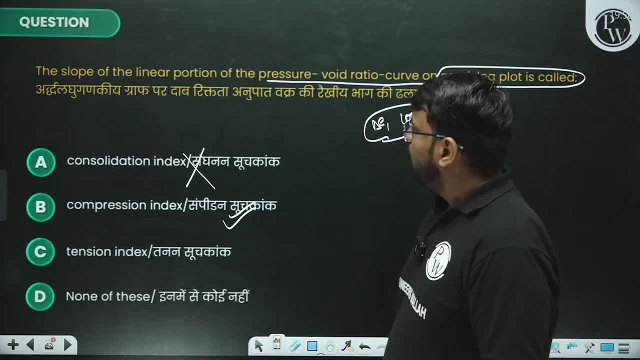 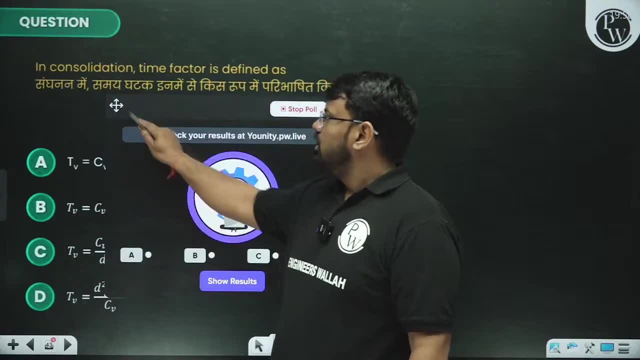 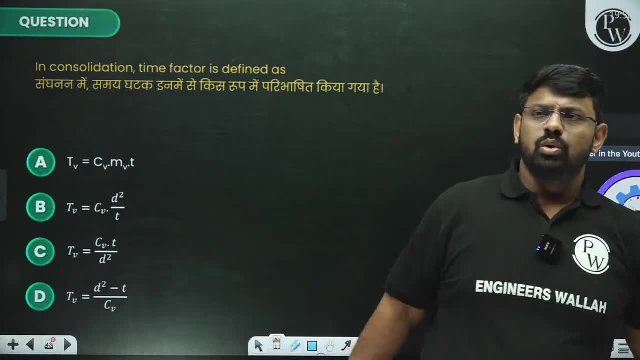 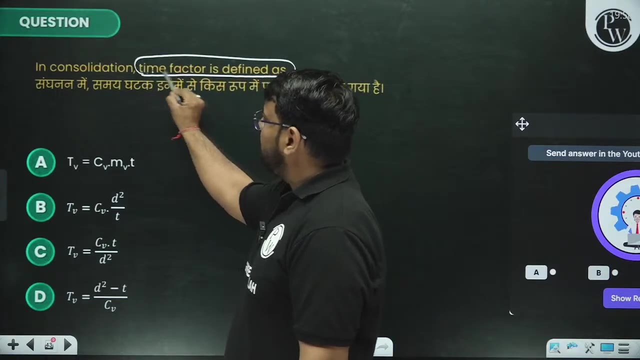 Answer it quickly And take the reward of your crores. Become a millionaire today. Tell me quickly What should be the right answer for this question. It is a formula-based question, Sir. In consolidation, time factor is defined. as I had told you about time factor. 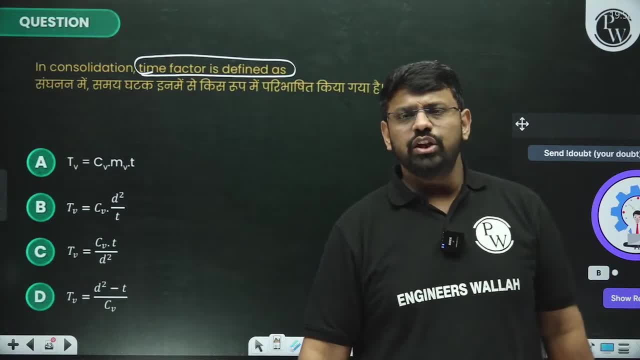 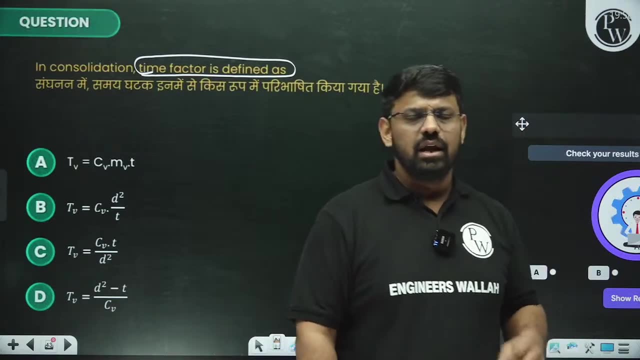 When you solve the equation in consolidation theory, then three dimensionless parameters come out. One of those three dimensionless parameters is a time factor, And the time factor is Cv, That is the coefficient of consolidation, And time of consolidation is related to each other. 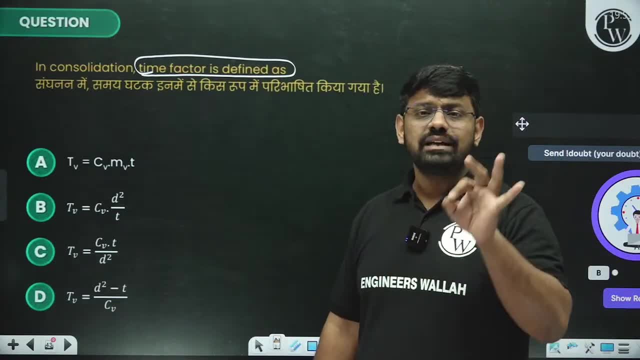 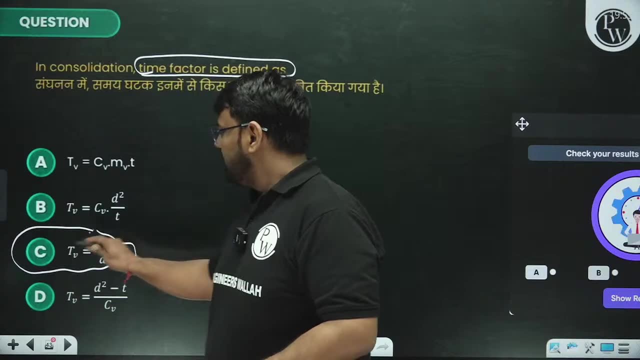 That is CvT by D square. We call it time factor. It is absolutely clear, Sir. So we have CvT by D square Where D is your drainage path. That means C is the right answer for this question. 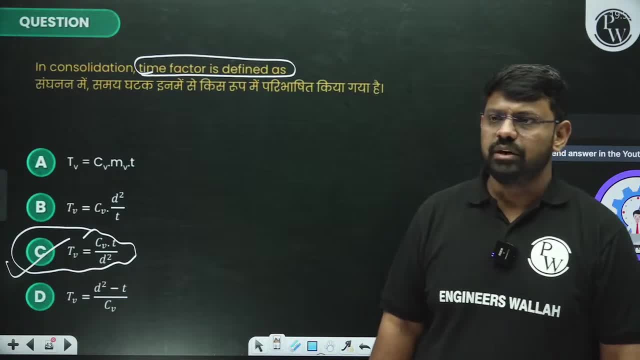 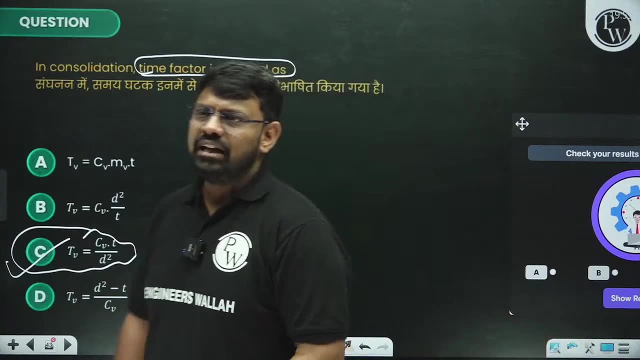 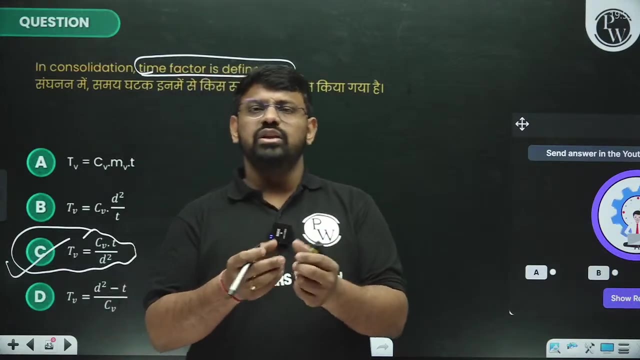 For this particular question. For this particular question, The answer is absolutely correct. Sir Kaushik says Spring piston model, Son. spring piston model is a representation of consolidation theory. Where in spring the soil is solid, In between the pores are pore water. 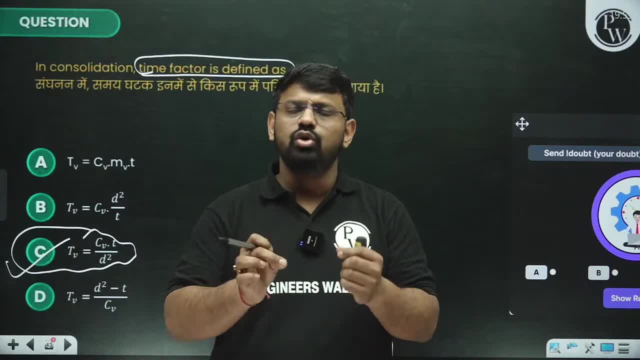 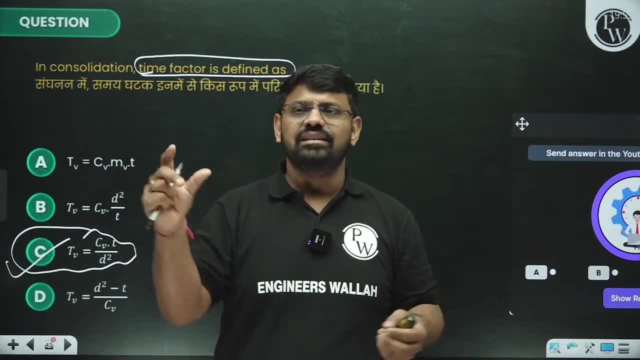 And what happens in the piston above? There are pores in it. It represents the porosity of the soil. It represents the voids. So when you press the piston, the water expels out, Just like the water expels out in the soil. 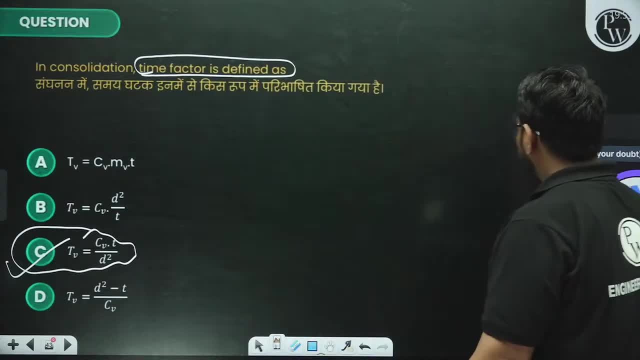 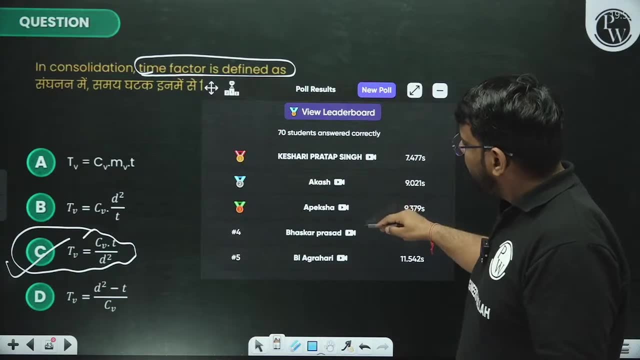 Absolutely correct. Absolutely correct, Sir. So here, Sir, we will have the correct answer. C will be the right answer for this question. 80% of the students have done it. K Sripatav Singh. Very done. 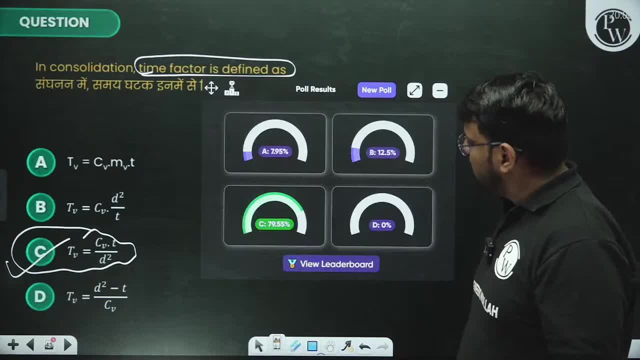 Very nice: Akash, Apeksha, Bhaskar, BI, Agari Vartika, And these are all our top 10.. Who is today's overall topper? Let's see once. The overall topper is Akash today. 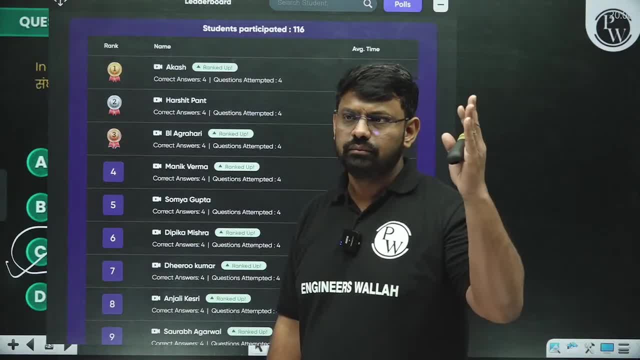 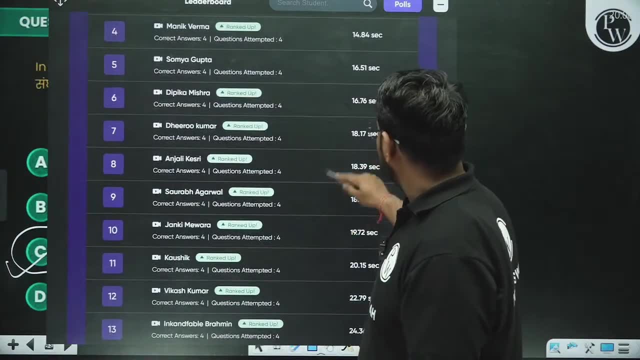 Congratulations, Akash. You have won 7 crores. Okay, Harshit Mann is second, Absolutely correct. And Manik Soumya. Deepika Dhiru- Wonderful. See, everyone's average time is also coming. 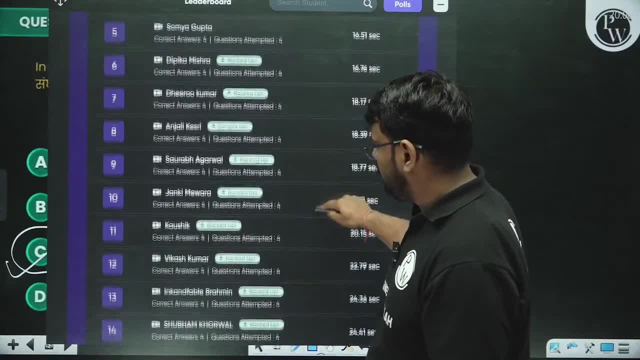 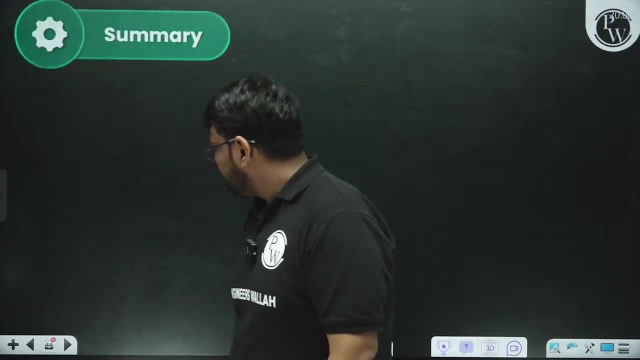 Great Attempted 4 questions. All 4 were correct: Saurabh, Janki, Kaushik, Vikash. It is a very long list, Brother. Okay, Sir, Very good Sir, we have talked about it till here. 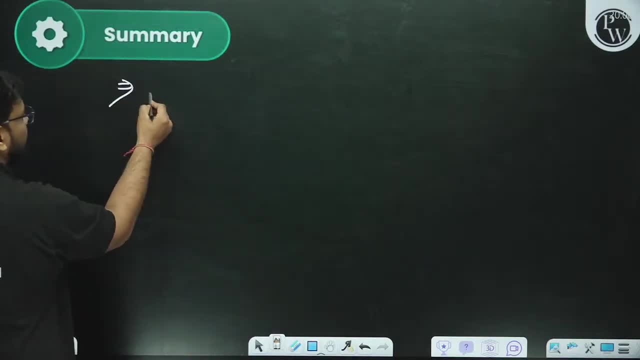 So what was today's summary, Sir? Today's summary was that, Sir, we have read the stress distribution, We have read the stress distribution And Son, out of 7 crores, put 1 crore in my account as well, Akash. 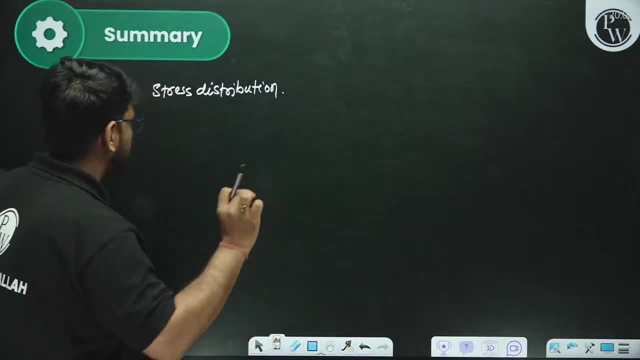 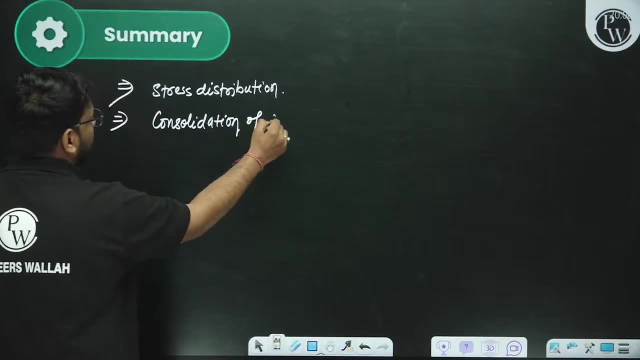 You have worked so hard. Out of 7 crores, put 1 crore in my account. And Second, Sir, we have Consolidation. What will you do with so much money? Give some money to Sir. Consolidation of soil. 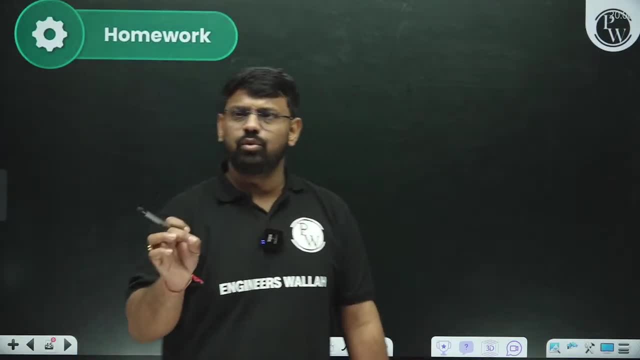 Okay, Tomorrow, Sir, what are we going to read? I am telling you, Tomorrow, you have to read. You have to read and come, Sir. Very important topics. Both of them are important topics. One, Sir, we have shear strength. 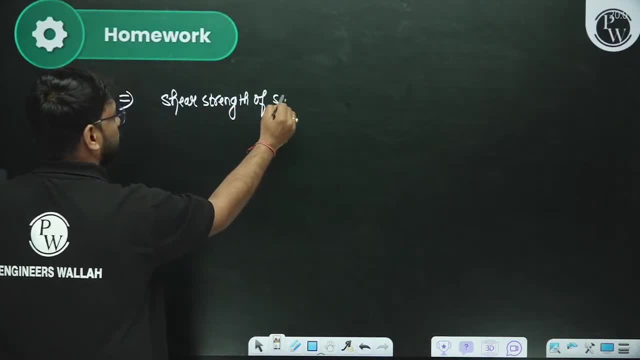 And I am warning you from the beginning, Sir, that you have to read a little bit of shear strength of soil, Otherwise you will not be able to pace up. Okay, If you will not be able to pace up, Next see, Sir, Earth Pressure Theories. 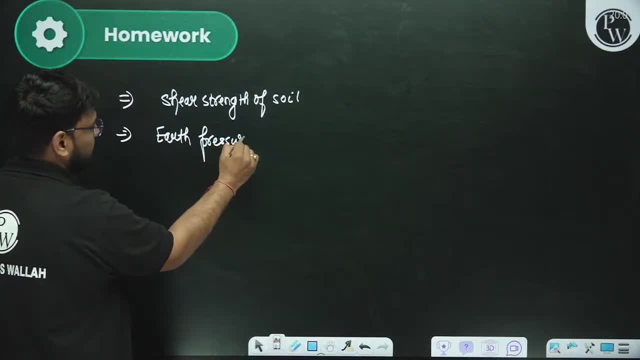 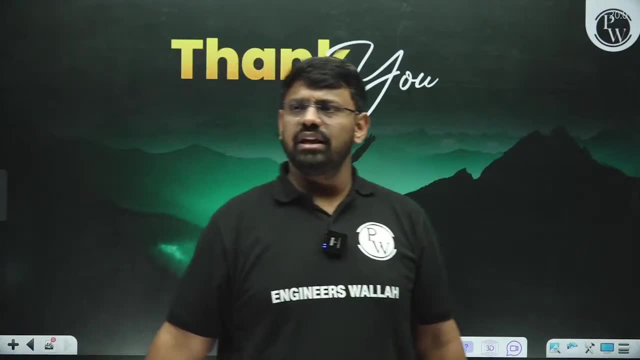 Tomorrow we are going to read these two topics in a great way: Okay, Earth Pressure Theories, And tomorrow is Sunday, So I am fully hoping that more children, because they get free in every way, get free from all kinds of classes. 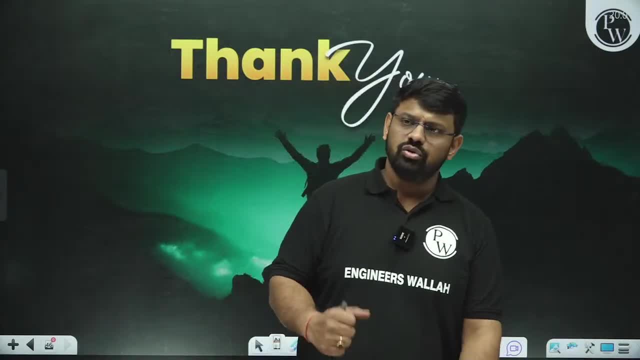 So tomorrow all the children will also be present And they will show enthusiasm And they will revise in a good way. Tomorrow is Sunday time And there cannot be better topics than this on Sunday. Shear Strength and Earth Pressure Theory. 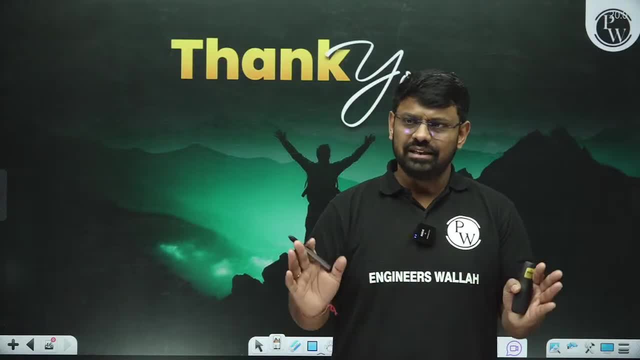 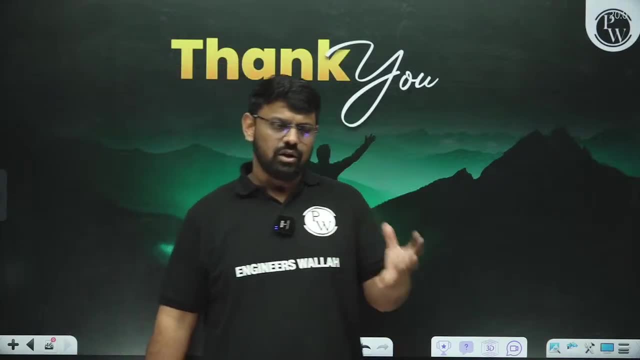 Both are very conceptual topics. It is going to be fun in a very good way. Once, make a heart symbol and tell us, Sir, how did you like today's session, And do comment in the comment box And tell us that. 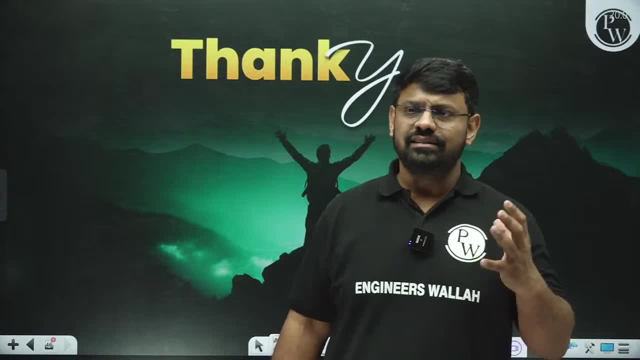 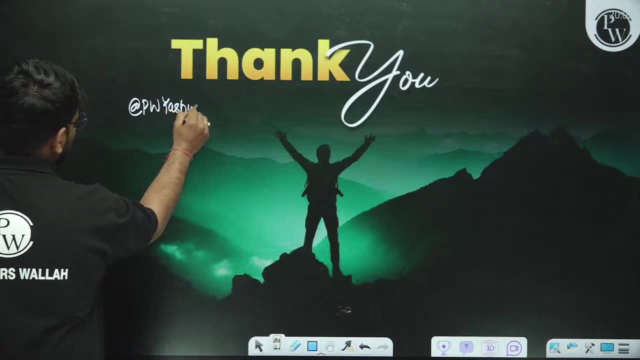 Sir, we are liking the sessions very much And continue with this enthusiasm, with this energy. Okay, So at the rate PW Yashwant Sir. You all know this Telegram channel. At the rate PW Yashwant, Sir. 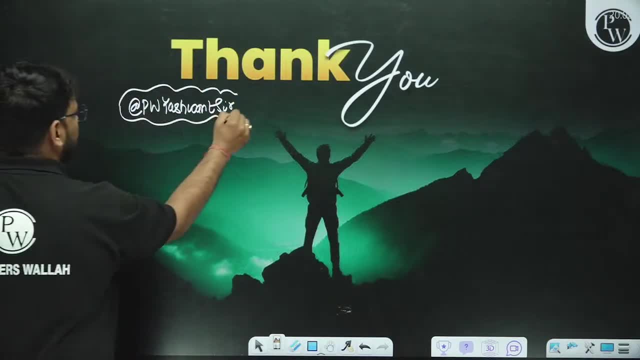 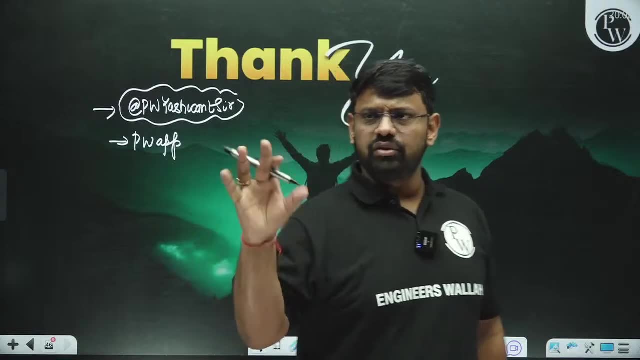 You will get a PDF on this Telegram channel. You will get a PDF on the official application of PW, Sir Okay, And here you can also ask your doubts. I am available for you 24x7.. Here I tell you all kinds of doubts. 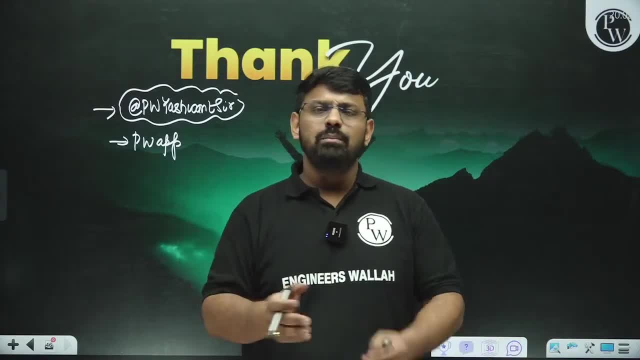 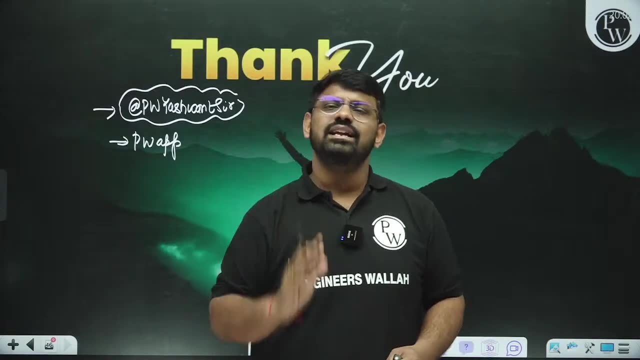 If some doubts are very small and simple. So there are a lot of kids in the group, See. there are a lot of rankers too, Who are selected students of SST. They are also connected to this group So they also keep answering you from time to time. 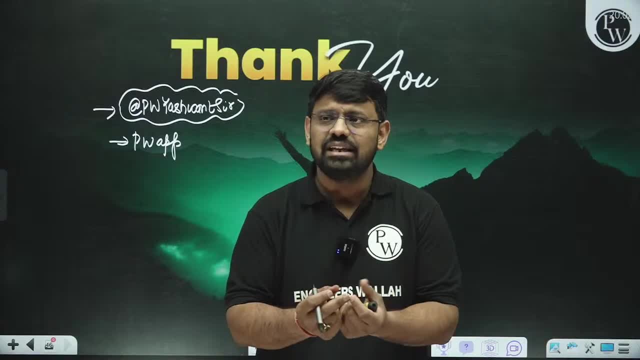 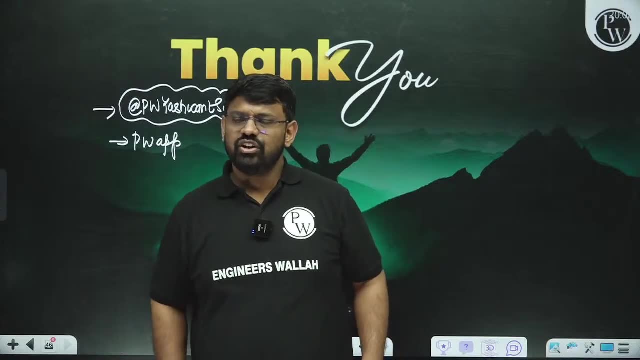 Okay, So you don't have to think that Sir Sir did not answer this question of mine, Because there all other kids also answer you. Okay, Sir, Very good. Okay, Sir, Let's meet in the next class. 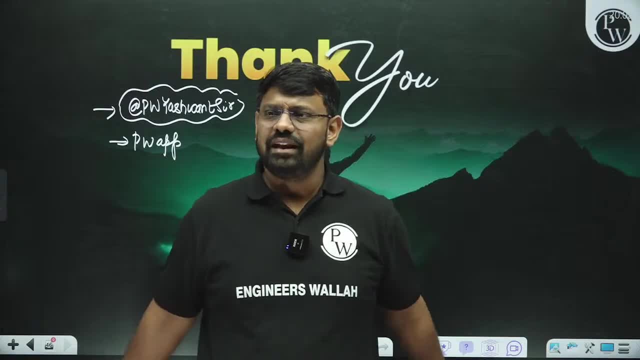 Sir, with full energy, The girls are going to study with sheer strength and freshness. Till then, all the kids will say together: Keep learning, Keep rocking. Thank you so much.